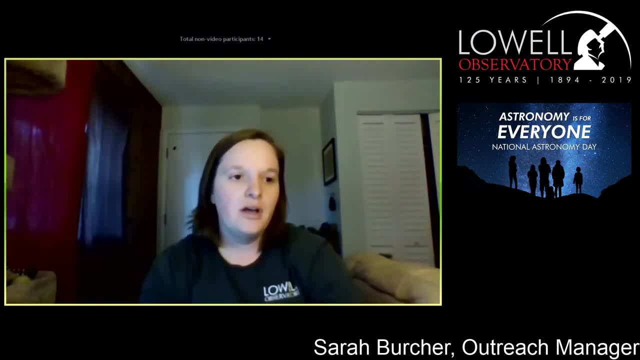 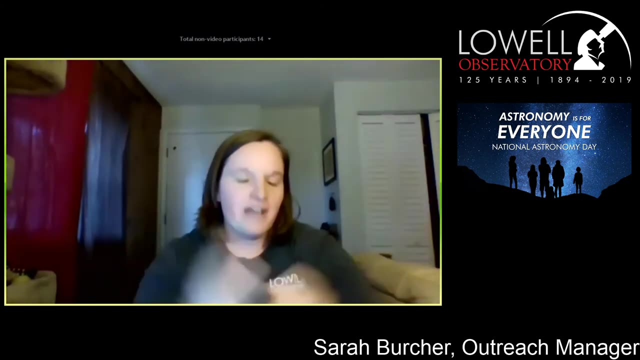 So we have a whole slew of people to talk to you tonight, including some of our educators talking about their own personal experiences. We have some of our astronomers talking about what astronomy means To them and how you can get into it. We have more educators giving you activities you can do with your kids and kind of some insight into how you can start your own backyard astronomy program. 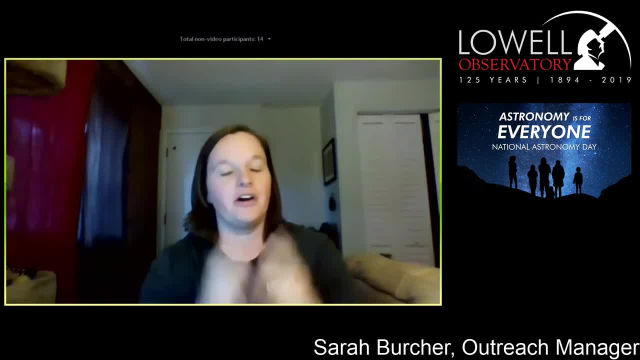 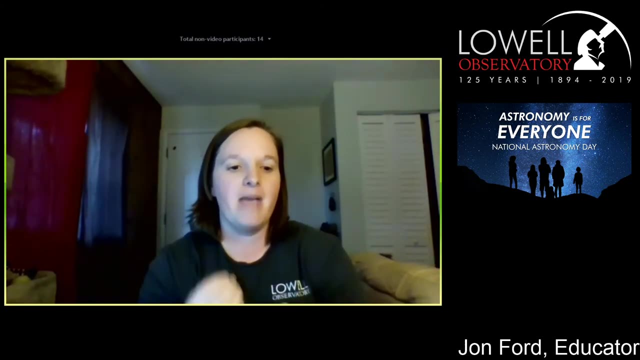 So with that we are going to start, our astronomy is for everyone presentation with one of our senior educators, John Ford, And he's just going to start us off by telling a bit about his childhood experiences in astronomy, That that made this such an important part of his life. So, John, are you ready? 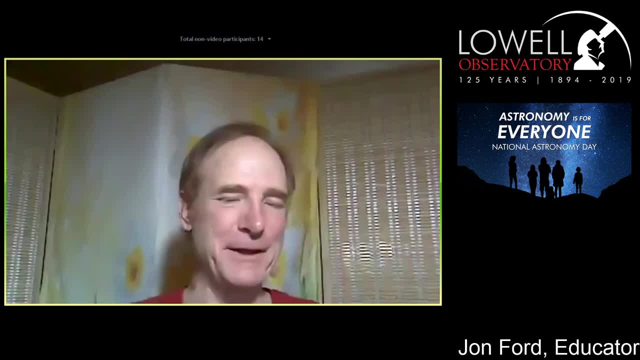 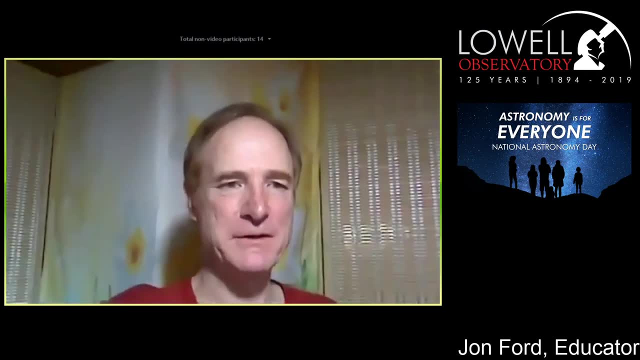 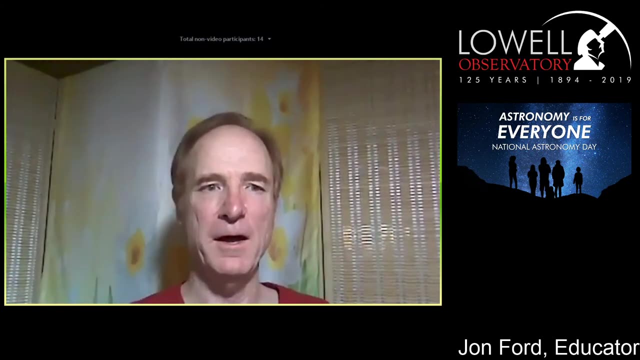 Hello, how are you doing? My name is John, I am a senior educator at Lowell Observatory And, yeah, I just want to share a little bit about how I got into astronomy, And a lot of it has to do, as Sarah was mentioning, about some of my experiences early on in life. 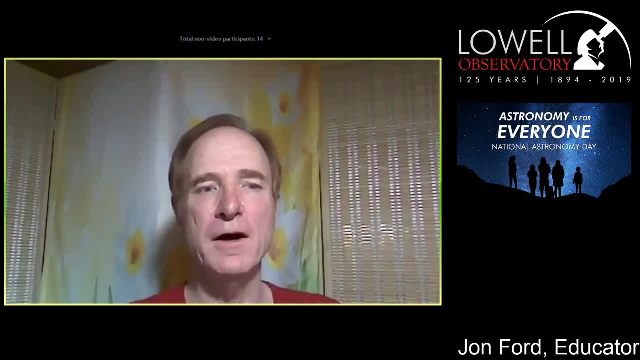 I did grow up during the time period of the space missions, the manned space flights including Mercury, Gemini and Apollo, And I have very vivid memories of that happening, you know, on my television set back in the 1960s. I would say that was probably the first major influence in that regard. 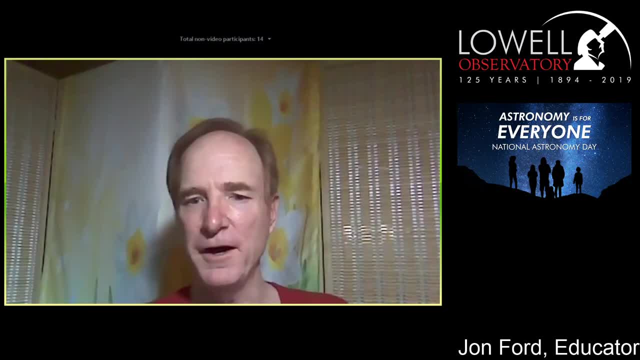 Of course, that's when I first realized at a very young age that astronauts were Up in space, orbiting the Earth and eventually reaching the destination of the moon. Other experiences I had during that point in life that I remember was having a 2.5 inch refractor telescope. that was in our family at that time And that was a pretty big deal. 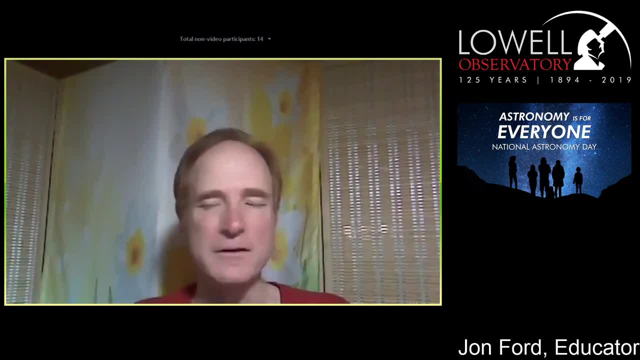 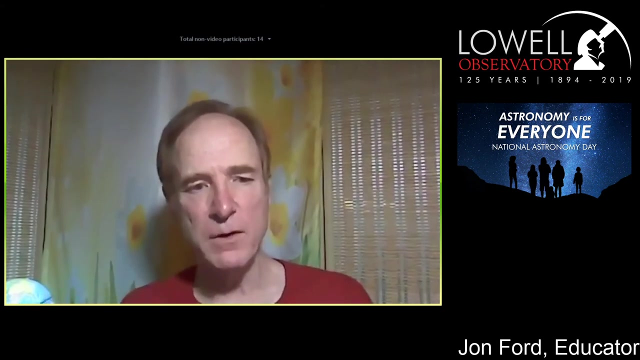 I would say that was the first opportunity I had to look through a telescope And once again, it evolved At a very early age. I remember watching a solar eclipse from the year 1970. And using a refractor telescope, we actually projected the shadow of the eclipse onto a screen and got the opportunity to see the moon, the shadow of the moon moving across. 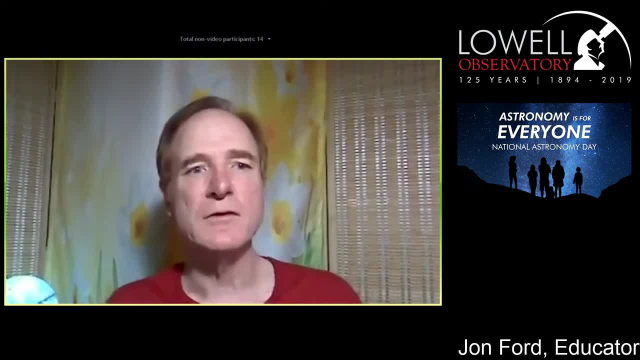 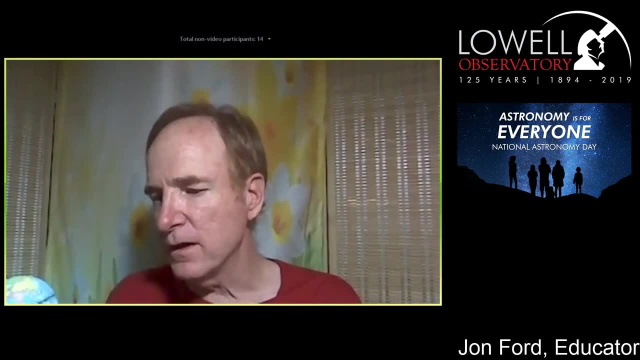 Changing the appearance of the sun and darkening the sky. So that was really one of those moving moments that really inspired me to get into astronomy. At that point in my life I was living in Chicago And I have to say that Chicago is interesting because you would think as a big city you wouldn't really have many people. 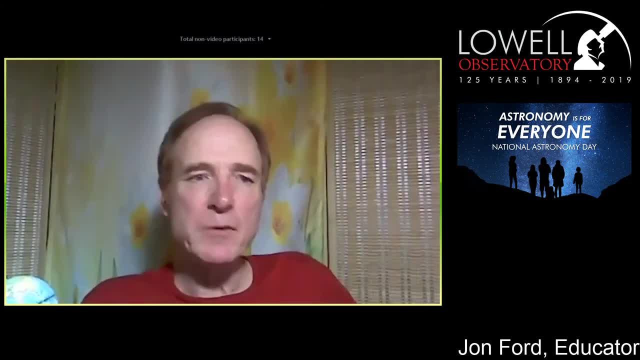 You wouldn't really have many opportunities for astronomy, But that really wasn't the case. We had world-class museums in the city, including the Adler Planetarium, And once again, from that point in my life, I can remember the amazing opportunity to go to the planetarium to look at the projection of the night sky that they created on the ceiling of the dome. 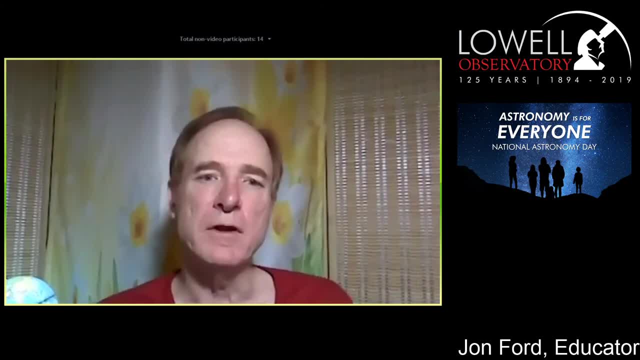 And just being kind of Captivated by that experience. I'm very thankful that I've had the opportunity to work at Lowell Observatory these years, Because now this becomes my opportunity to share some of those same experiences that I had as a child with visitors that are now coming through the observatory. 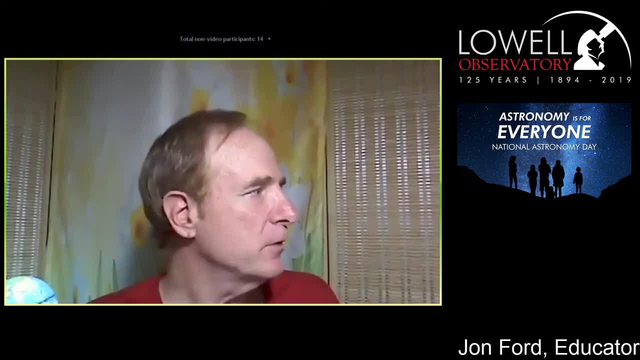 Of course we don't have a planetarium like the Alford Planetarium, but what we do have is the actual night sky, So we can actually use the night sky in much the same way to identify the different constellations and the different objects that we can see. 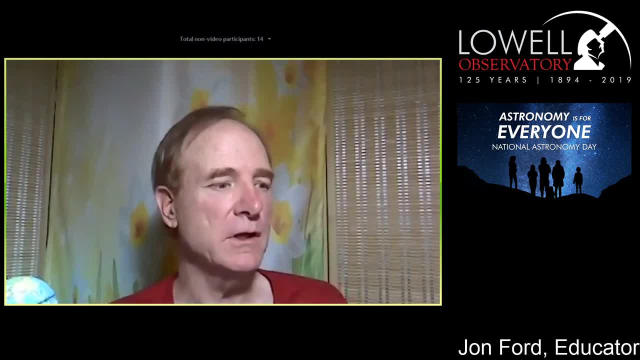 And once again, I'm just so thrilled that I have that opportunity to be able to kind of convey that experience to the next generations of visitors that we have at the observatory. So that's all I have to share. That's all I wanted to kind of share with you guys about the observatory. 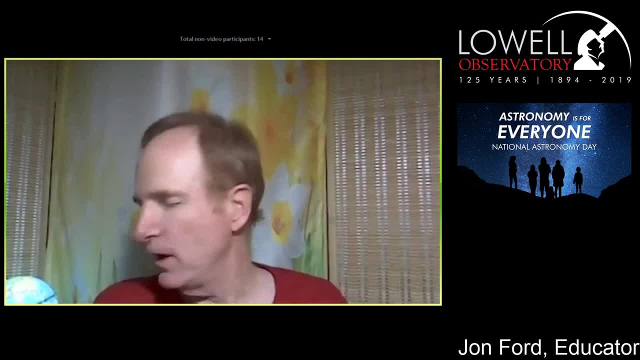 So that's all I have to share. That's all I wanted to kind of share with you guys about the observatory. So that's all I have to share. That's all I have to share with you guys about the observatory. I'm glad to have you guys with me on this. 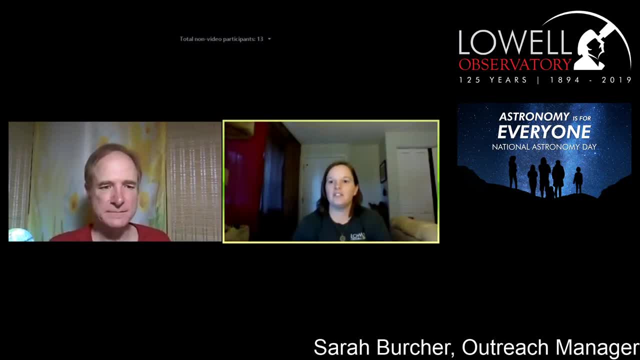 That's all I have to share, All right, Thank you so much, John. Oh, I'm going to give time for questions, though. Anything to say while we wait for questions? Nope, not really. Let me take a look real quick up here. 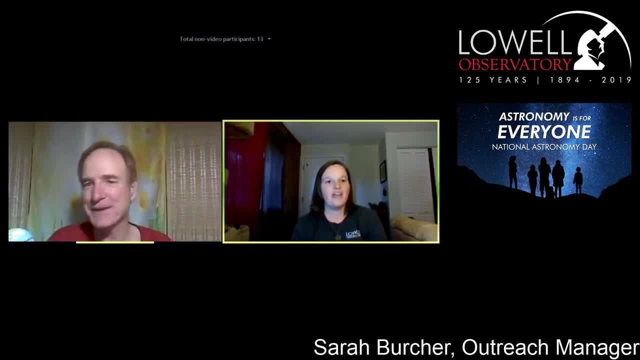 All right, All right, I don't think we have any. So thank you, John. So yeah, I love those kinds of stories that tell us. you know that people give me because everybody has their own anthropology, So that's great. 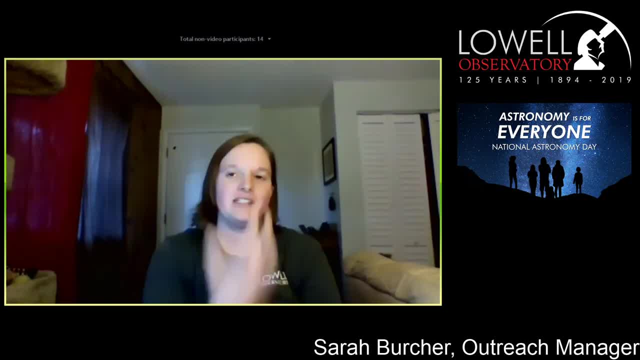 those stories. Like John was saying, he grew up in Chicago. There's no night sky there, yet he still managed to find that passion And I love that kind of stuff so much. So to kind of switch gears slightly but stay in the same realm I'm going to introduce 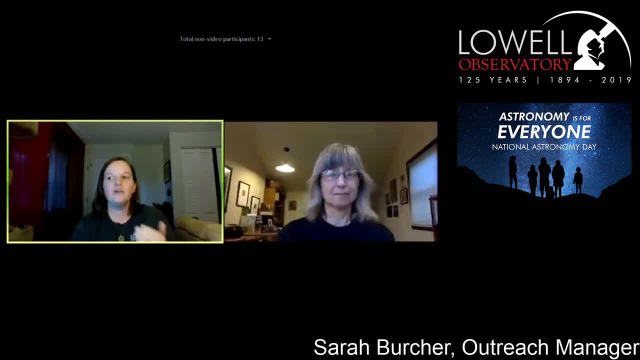 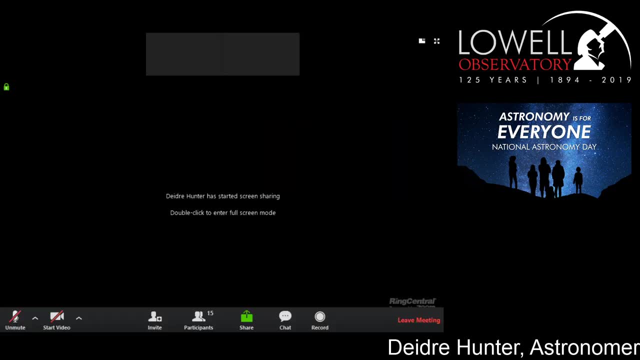 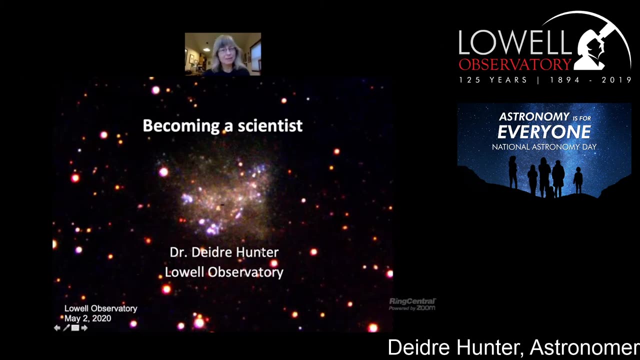 one of our astronomers, Dr Deidre Hunter, who's going to talk to you about becoming a scientist and what that means to her. So, Deidre, take it away. Well, thank you, Sarah. So I want to take a few minutes to tell you about how and why. 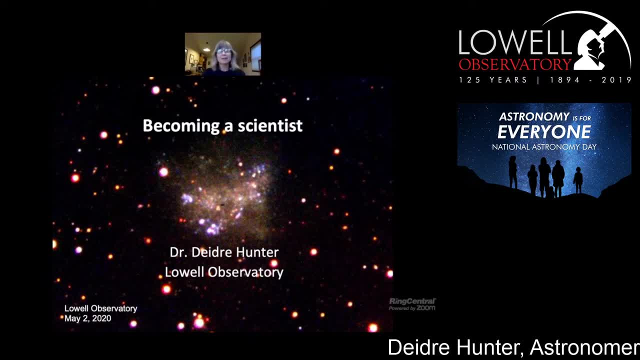 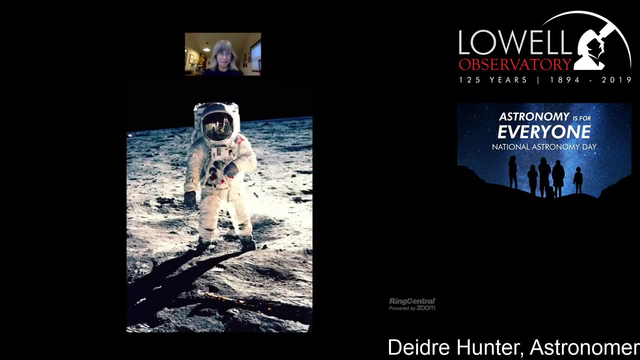 I became an astronomer and why it's fun. So I became an astronomer because of this gentleman and his colleagues. In the summer between sixth and seventh grade, a friend of mine and I decided we were going to be the first women astronauts. This was when the Apollo. 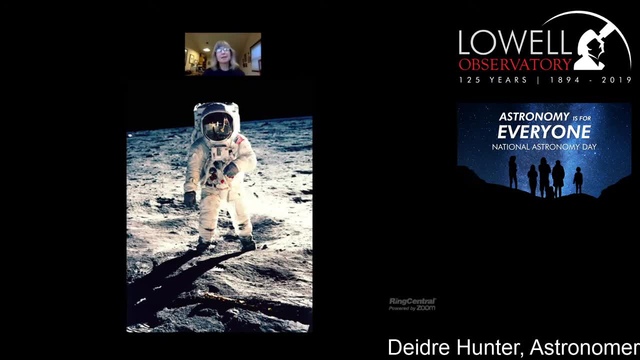 program was at its height, and it was a few years later that Neil Armstrong first stepped on the moon, And I thought that stepping on the moon or going to another planet or another place in the solar system would be so exciting. However, I found out that if you wear glasses, 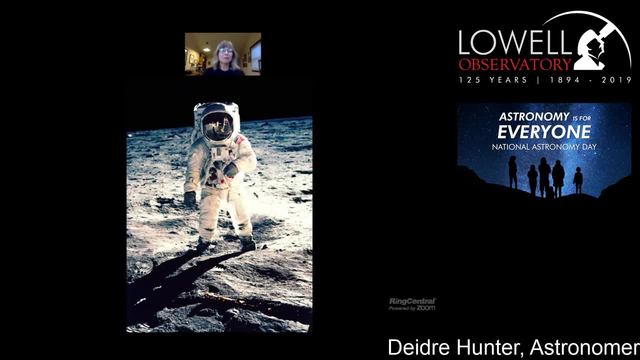 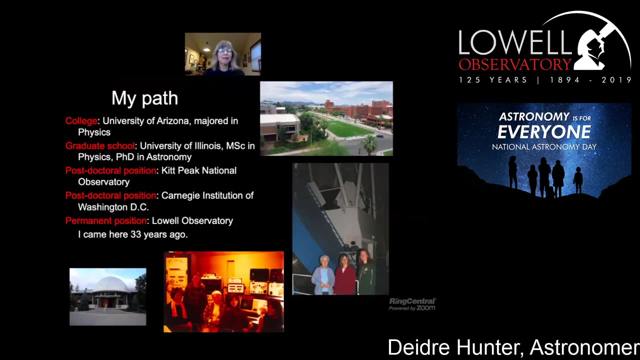 you couldn't be an astronaut, And I was wearing glasses. I didn't wear glasses even then, So I decided, if I couldn't become an astronaut, I would study what was out in space. I would become an astronomer, And so I set off on that path. 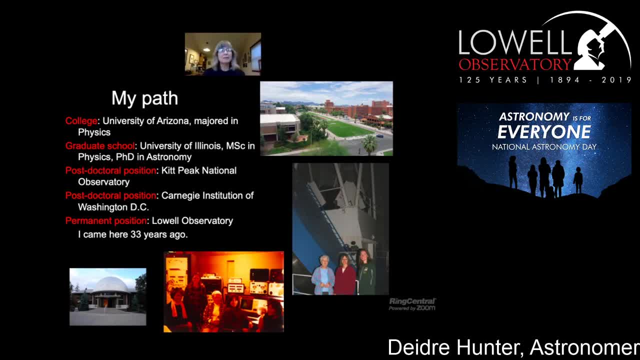 and followed a pretty traditional path. I went to college and majored in physics and I went to graduate school got a master's degree in physics and a PhD in astronomy. Then it's typical in science, in astronomy, for a recent graduate to have one or two temporary positions, called postdoctoral. 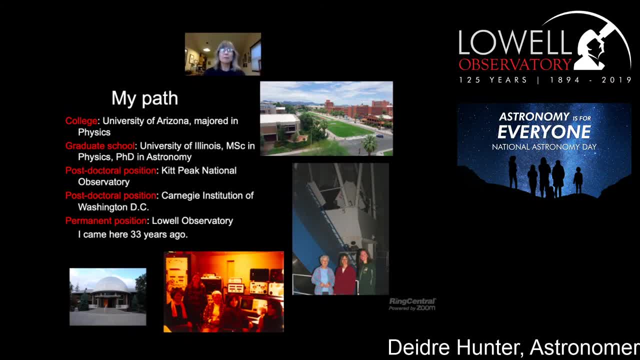 positions and it's a chance for a young astronomer to do different science with different people, learn different things and have different experiences. so i had two of those postdoc positions and then, 33 and a half years ago, i came to lowell observatory and i have been here. 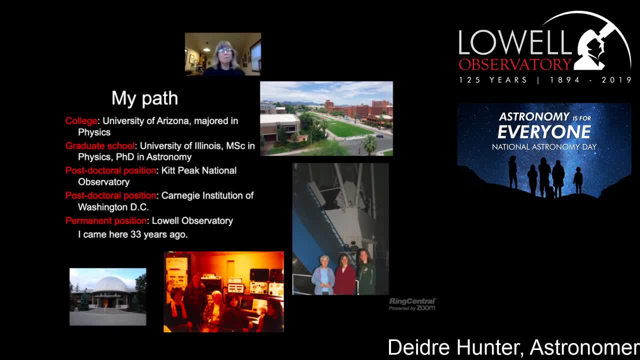 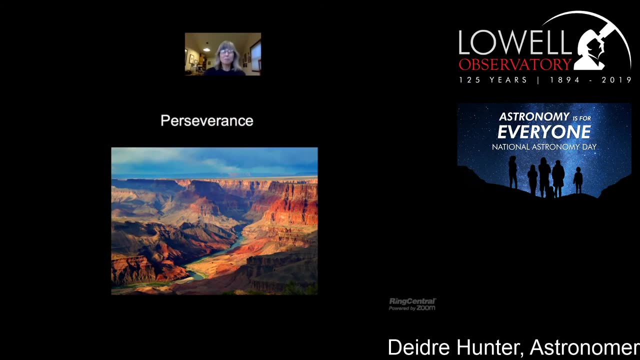 ever since. so that was my path to becoming an astronomer, and one of the things that i want to make clear to the young people- kids and young people in the audience- who haven't made career choices- is that you don't have to be super. you don't have to be super anything to be a scientist. 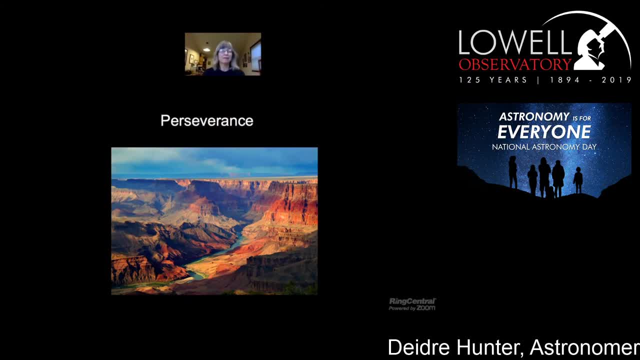 what you really need, besides curiosity, is perseverance. my husband and i have backpacked in the grand canyon- this is a picture of the grand canyon- several dozen times, and at the end of the last day of the trip we are usually down here at the bottom and we need to go up to the top. 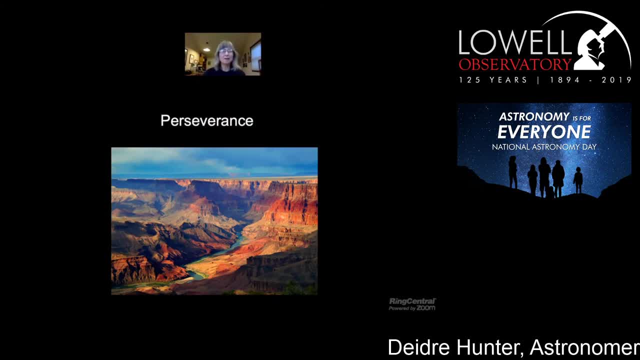 and before, as we're stepping onto the trail to start our our journey up and out, one of us says: how are we ever going to get out of here? and the other one always says: one step at a time. and so that's my advice to any buddy who's listening: that you, if you, take one step. 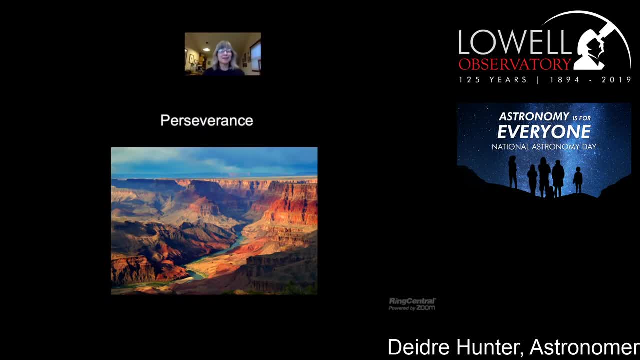 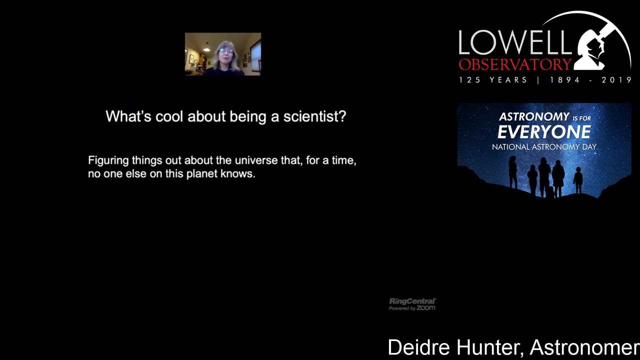 at a time, you can go anywhere and, um, you can get out of the canyon, or you can become an astronomer, scientist, or anything else you want, um. so what is it that i like about being a scientist? what i like is figuring things out about the universe that, for at least for a moment, nobody else on the planet 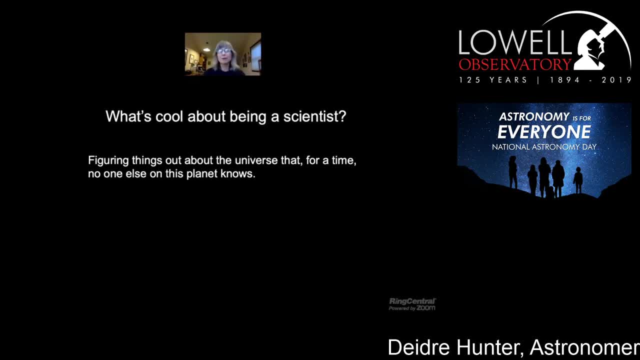 knows, and figuring out new things, things that weren't known before, and um, so when you finish a project- if i've been working on a project reducing data- and i finally come to an answer, um, sometimes it's not a clear-cut answer and then you just go huh, but sometimes the answer is. 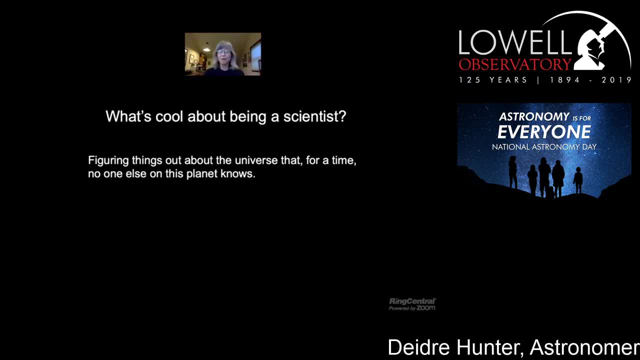 clear-cut and beautiful, and you think, wow, nobody else on the planet knows this yet. then you have to tell people, you have to tell your colleagues and collaborators, and then you have to tell those astronomers. but for a moment, you, you have figured out something new. um, and 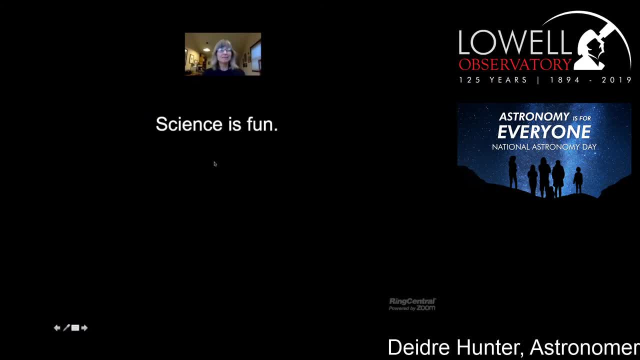 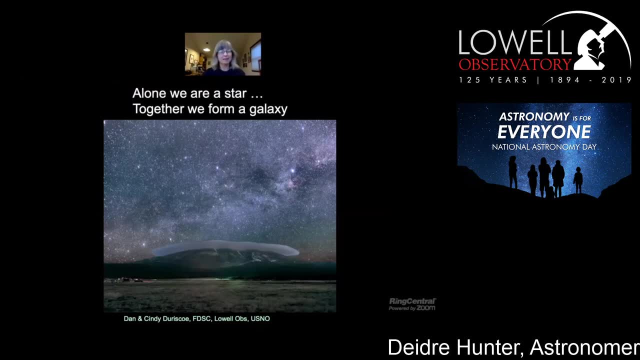 so i've once again got an answer for that. um, you take a question if you don't know the answer and you nhiều over it. uh, you know, go over it and just keep it going to the quarry and, regardless of the question, until the answer has been one thing, you just say: well, scott, what talked about? 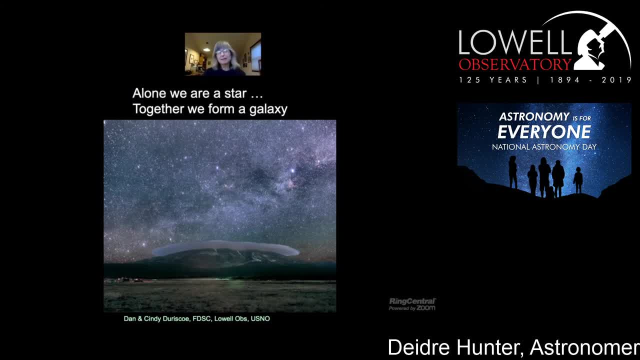 the knowledge scientists said maybe it's agreeability, it's sock practice, it's Hurrying, ive breeding and we're notepads on. is there a way to 0? say yes, it was a great question, because boob was a great question. and then all 6 here you have y gaming knowledge, Hundreds of ones. 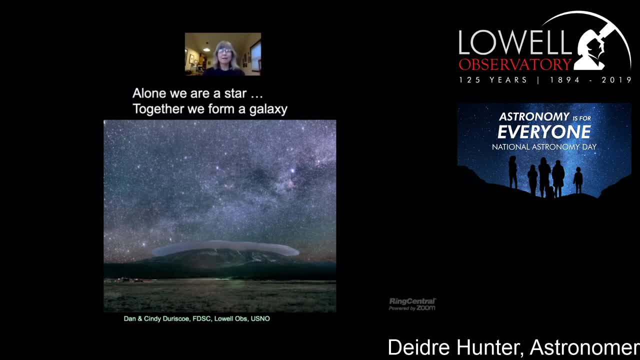 billion stars in the milky way, and they and our sun and its little collection of planets, is just one of those stars. they're all held together by gravity orbiting around the center of the, the milky way galaxy. it takes us 200 million years to go once around um and um. so the galaxies are. 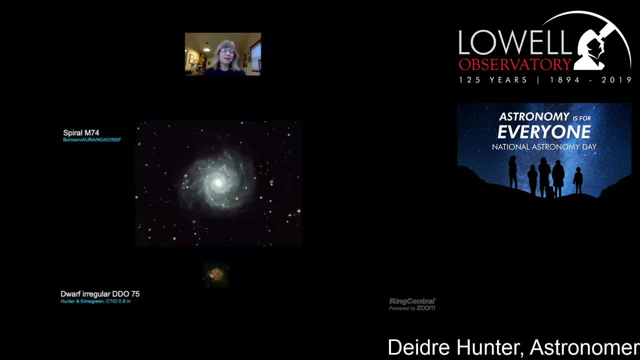 um are just beautiful. now i don't study uh galaxies like the milky way. the milky way is a spiral and this shows um a typical spiral galaxy, um here at the top, and this is a typical dwarf irregular galaxy. these little tiny dwarf irregular galaxies are the tiniest galaxies in the universe. 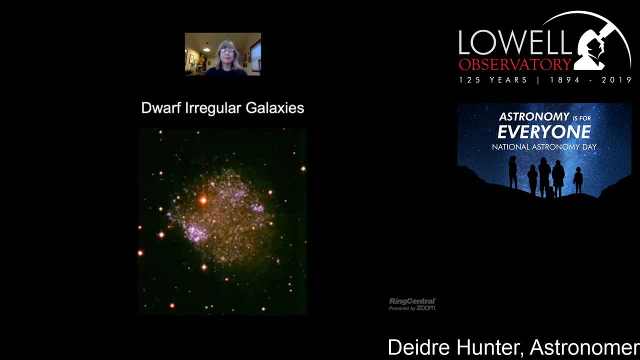 but they are the most numerous and and these are the galaxies that i study in this little um, this little dwarf galaxy, you see, all of these little stars that are. this is just the star in the milky way, that's in the way, but these other stars are. 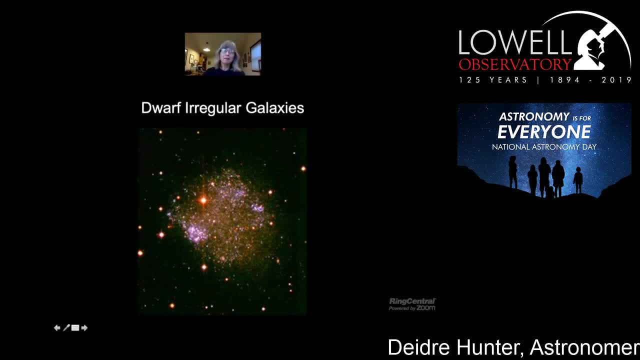 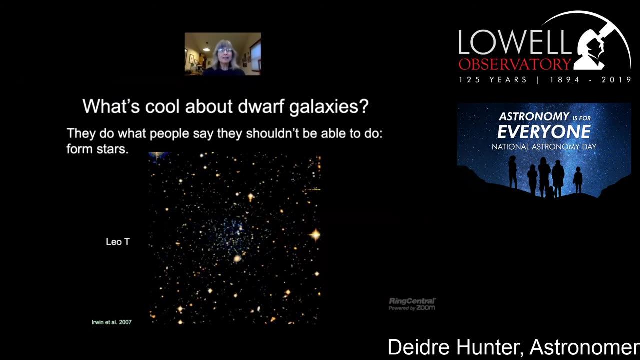 little tiny stars. those are stars in that galaxy, and these clumps of blue stars, those are young stars that have recently formed, sometime in the last um, 10 million years, um and um. what i like about the dwarf galaxies is that they do what the theorists say. they 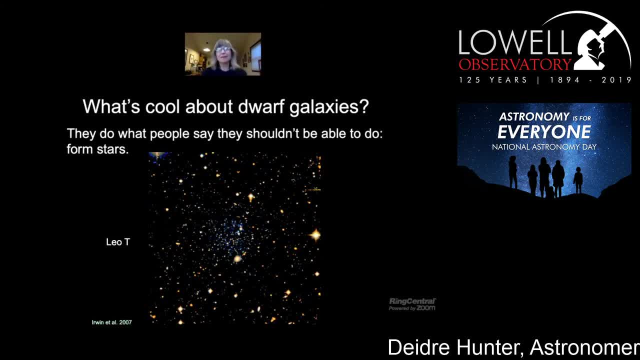 shouldn't be able to do. they make new stars. they make stars um. the people who've made models that we, that we think, help us understand how the clouds get together, that make stars and spirals, predict the dwarf galaxy, shouldn't be able to warn stars at all. 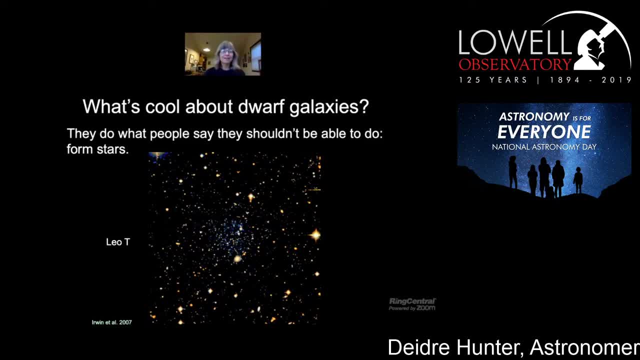 and yet they do so. i want to know how they do it. this little galaxy called leo t is one of my favorite examples of what the problem is. here is this tiny little galaxy. i'm circling the stars that are in this galaxy. it's so faint and tiny. it was a little bit of a. 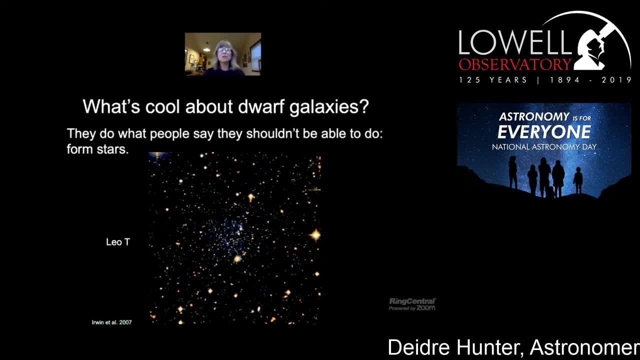 zone of discovery about a dozen years ago. it only has 300 000 stars in it. all these other stars out here, those are just stars in the milky way that are in the way um these. this, this little galaxy, only has 300 000 stars in it compared to the milky ways, 300 billion. and yet it has managed not. 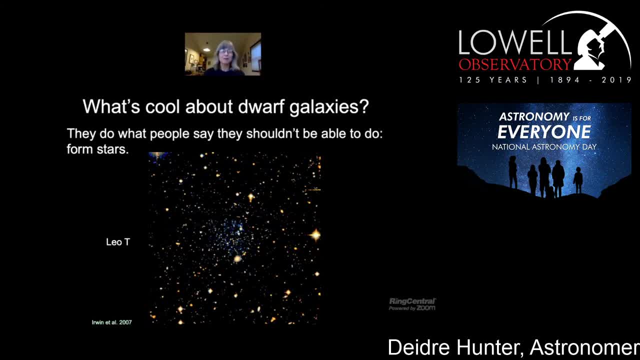 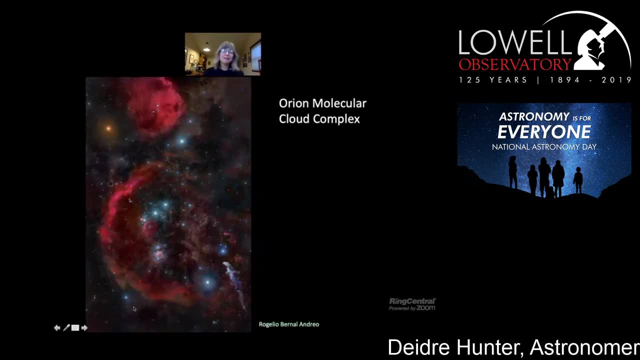 only to make those stars, but to make multiple generations of stars. there are old stars and there are young stars in that little tiny galaxy, um, and this picture i just had to show because show you, because this shows the closest place to the earth where new stars are forming in the milky way. this is not in a dwarf galaxy, this is in the 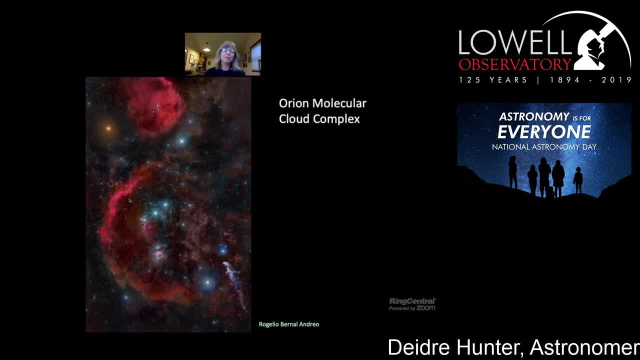 milky way, but this is called the orion molecular complex. and, um, you see, in front of the cloud there are the? um, there's the constellation of orion and here's the belt in orion and here's the sword and this huge, uh, cloud of gas. um, you know, we think of the space between the. 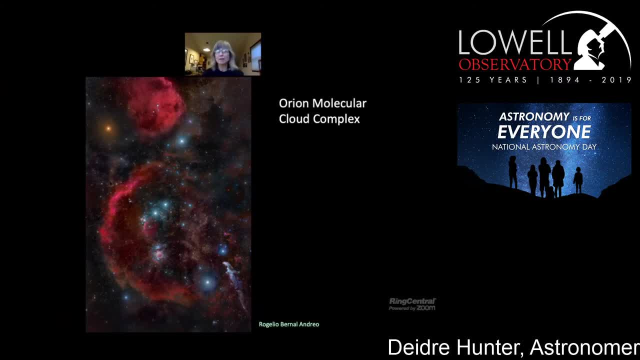 stars as empty. but it's not. it's full of the gas of hydrogen and helium atoms, and the density of that gas may be a 100 billion billion density of the air in this room. but, um, it gets together occasionally into a cloud and then gravity pulls it together and it stars out of the little clumps. 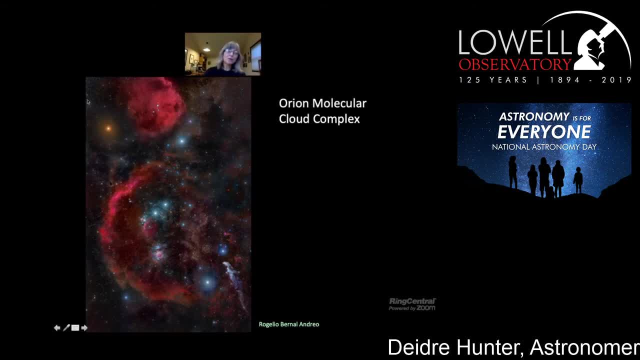 in the cloud. and that's what's going on in this huge cloud: um, it's just, it's past the constellation of orion, it's um um 1200 light years, i think, and the cloud, this cloud of gas and dust, is opaque, which, so you can't actually see the pockets in the cloud where young stars are forming. 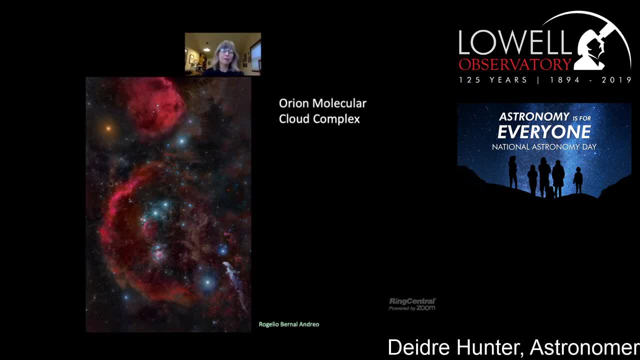 um, you have to use a far infrared or radio telescopes to see into the cloud, except down here in the middle, in the middle of the sword. here is this nebula. you can actually see it by eyes. it looks like a fuzzy bat and in that is called the orion nebula and it's a little place in this giant cloud. there's this. 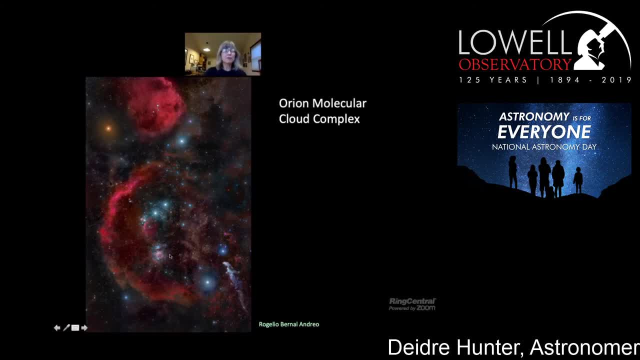 little place here where, um, a little cluster of stars are formed, including some massive stars that have, um have um ionized the gas around them because they put out a lot of ultraviolet light and produce this nebula. so this is just a little blip on this huge cloud. 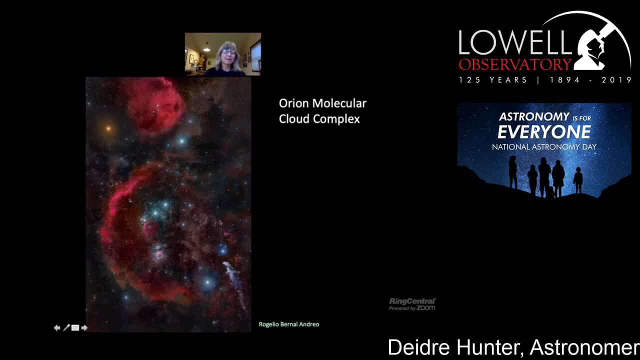 where stars are forming, um that we can see, uh, young stars starting to peak out, and so this is the process that i want. i want to understand how these clouds are made in the dwarf, irregular toxins, and that's all i have to say. um, are there any questions? i see some questions um how much was my phd? it was um seven years of. 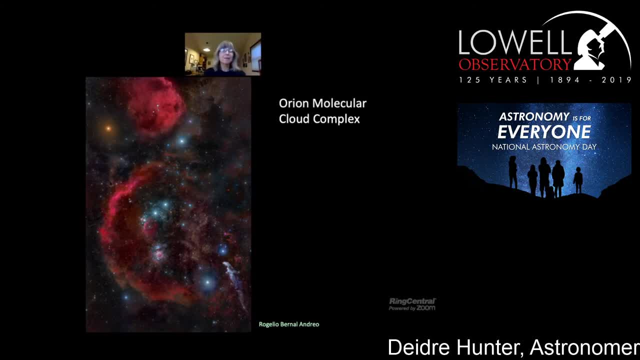 my long got a good, getting a master's degree and then doing um the phd. the phd is an internship where you work with somebody, a professor, and you work on a research project. so it was fun. once i was doing the first year and then i was doing the second year, so it was a lot of fun. 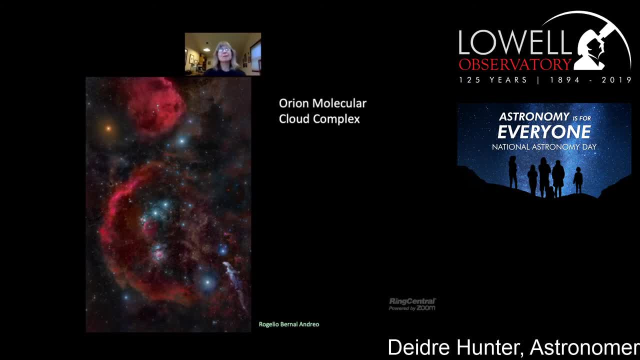 part I hated, but once I was doing my research project it was wonderful, Going to the telescope and learning all these new things about how to use telescopes and learning it was just wonderful. But they paid me to go to graduate school- Usually a graduate student when you. 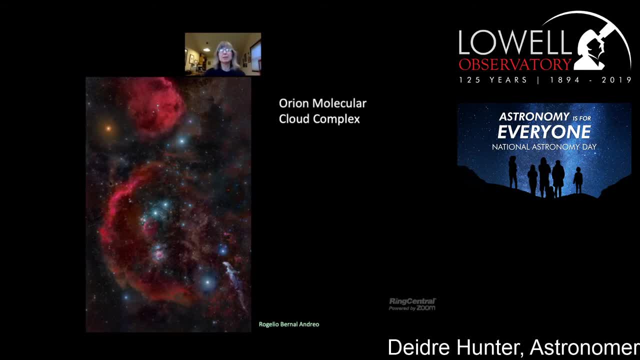 first go. you go as a teaching assistant and you're paid. as a teaching assistant You're kind of you scrape by, but it's enough to live on. And then sometimes your advisor might have money funding to pay you as a research assistant. So I basically was paid to go to. 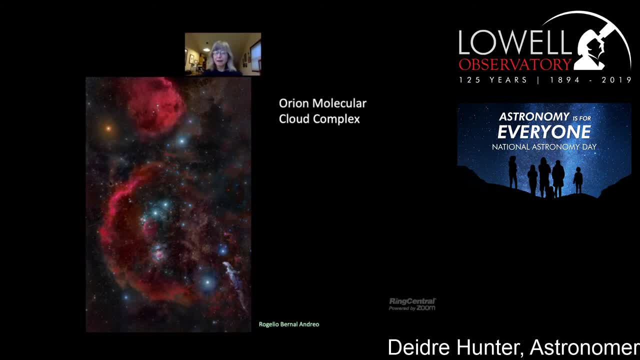 graduate school and get my PhD. How is a star formed? What is it made of? So this cloud of gas forms, That's this cloud here, the Orion molecular cloud. Gravity pulls it together And, as it pulls together, pieces of it fragment, And so, inside the cloud, you. 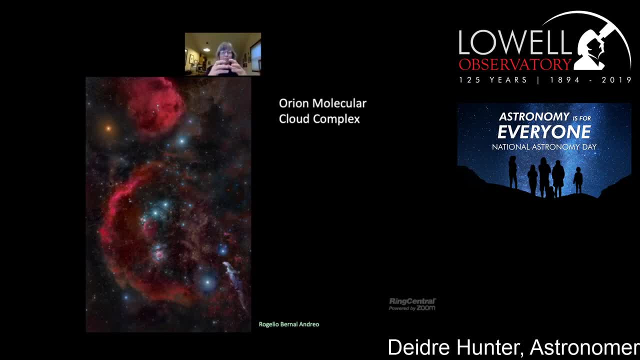 have these little pieces of gas, little balls of gas, And it's just gravity. Gravity pulls the gas together into a ball And it keeps as it gets denser and denser in the center of the ball. it gets hotter and hotter And eventually it becomes hot enough that nuclear fusion can take place. 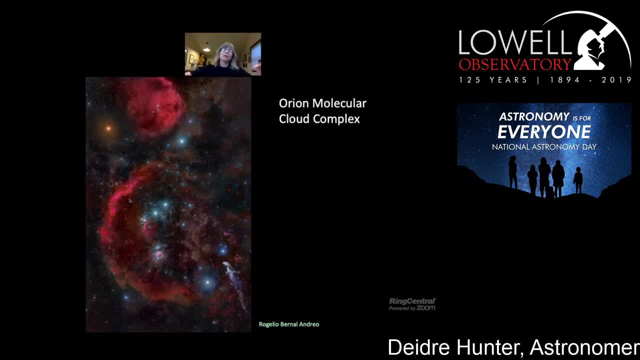 That produces energy, And the energy coming out balances the force of gravity wanting to make it contract, And so it stops contracting and it just sits there and it shines And we have a star. So the star is made out of the gas. 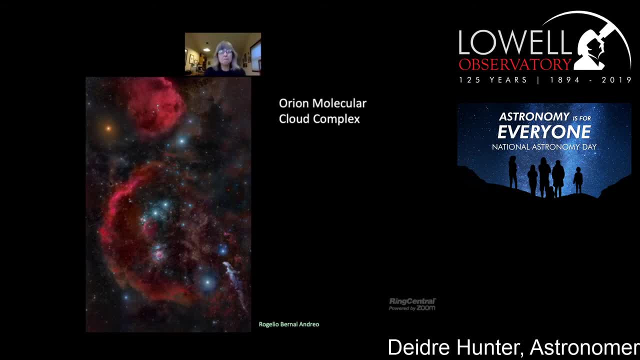 Yeah, And it's mostly hydrogen, a little bit of helium and then a tiny amount of the carbon nitrogen oxygen and all that other stuff. Those elements are made inside of other stars that were born and died before that cloud formed And they polluted the gas between. 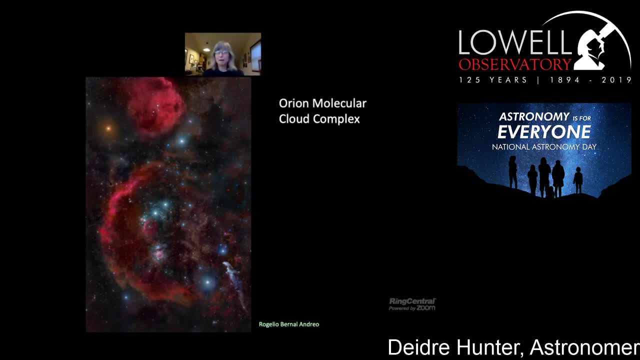 the stars, with what they're made of. What is my favorite constellation and why My favorite constellation is Orion? It's because I can recognize it easily. It has the Orion Nebula, my favorite little place showing stars, My favorite star. I never had a favorite star until recently, But now it's Betelgeuse which. 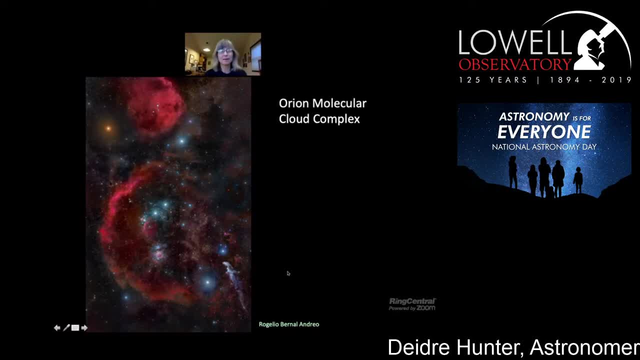 is up here in the Orion constellation. I like it because it's easier to see67. 00. it's a red supergiant and any day it could explode as a supernova, and so i'm waiting for it to explode. um, is there gas? if there is gas available, why would they believe they could not form stars? 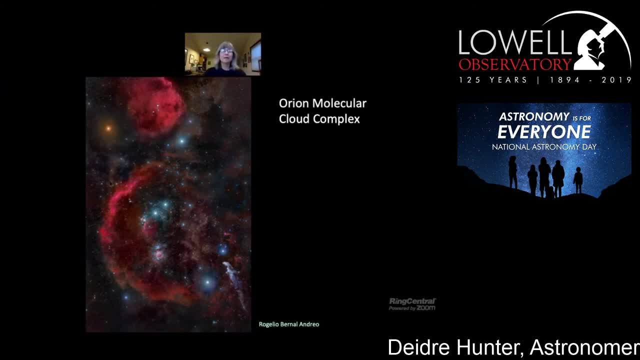 it's because the gas density isn't right, isn't high enough. the gas density is very low compared in dwarf galaxies, compared to spiral galaxies. and because the gas density is low, the gas is stable against breaking up into parts, so there has to be some process that 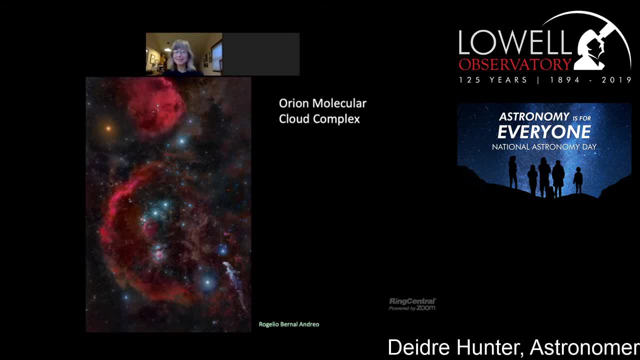 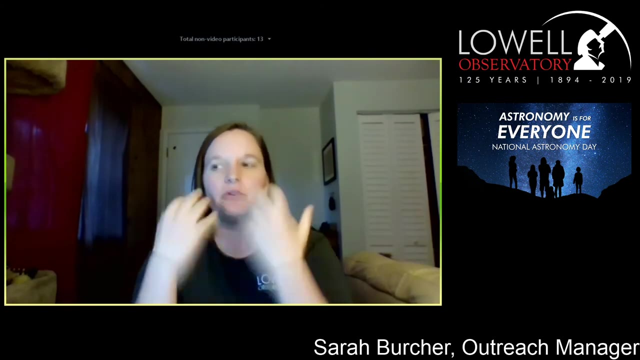 that triggers the formation of the fall. yay, okay, thank you, deidre, i appreciate that. so now we've heard from astronomer and deidre told you how a bit about how, how she got into astronomy, how she made a career out of it. i'm going to 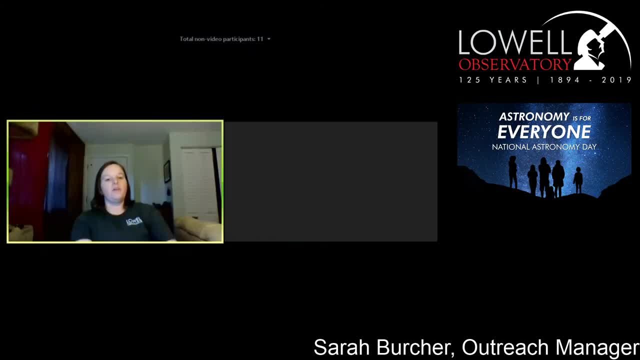 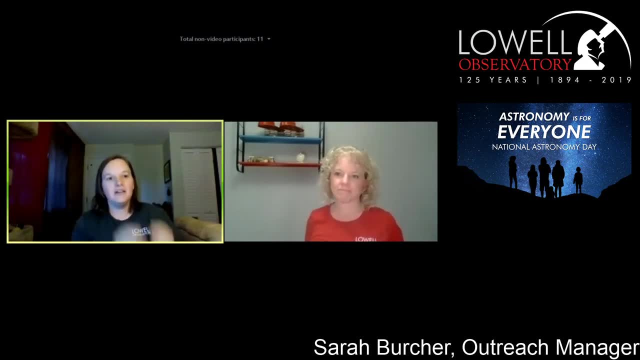 introduce one of our educators, joyce vinnie, who's going to talk to all of you about what kind of what kind of astronomer or astronomy geek are you, even if you have chosen your career already and you still want to to follow that path in some way. joyce is going to 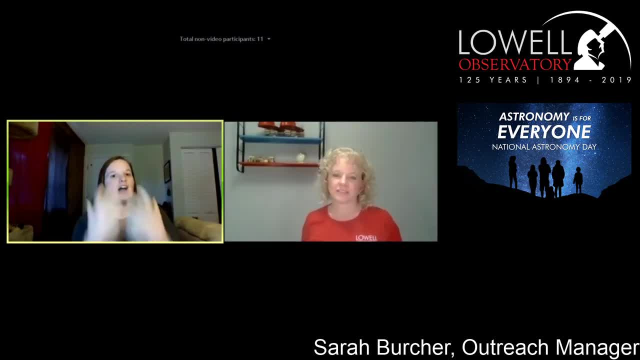 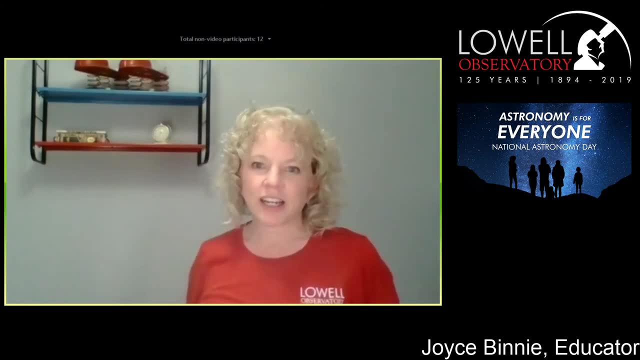 talk to you about what can what astronomy can bring to you as an individual. so, joyce, go ahead and take it away. thank you, sarah. i'm, as sarah said, my name is joyce and i am one of the public programs educators at lowell observatory. i'm also a certified interpretive guide. 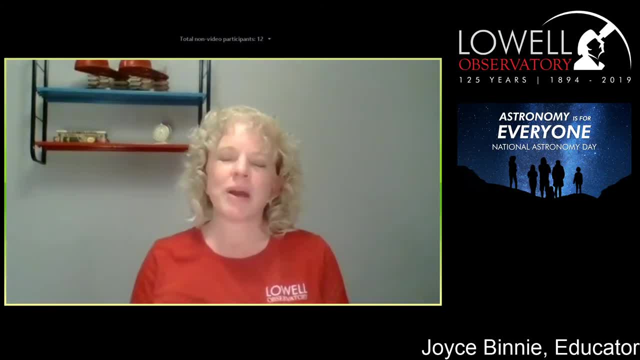 and i want to share with you today that the beauty of astronomy is that, no matter what you're interested in, you can explore, learn and enjoy at your own pace and on your own terms. so, um, we're going to talk a little bit about the types of different. 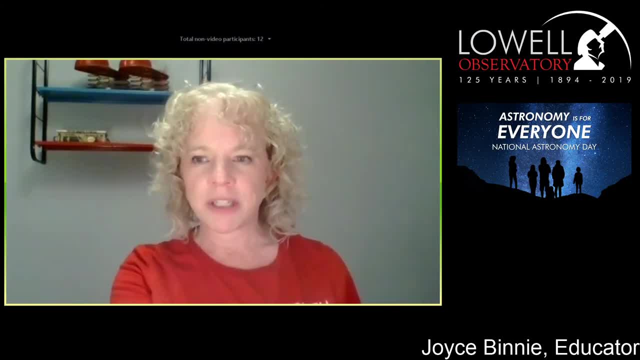 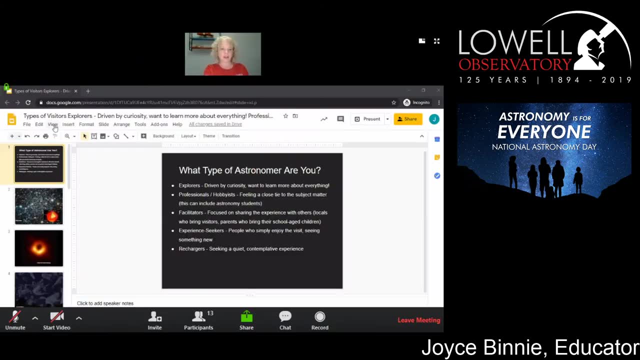 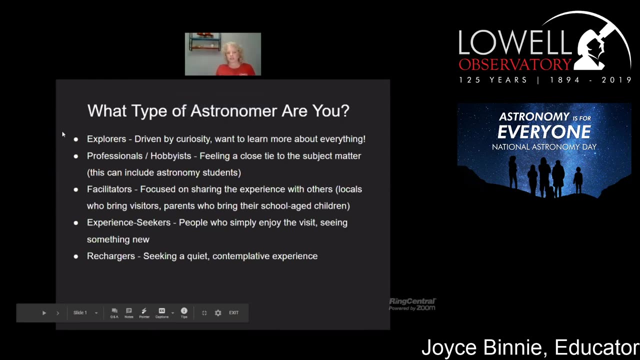 interested in astronomy and i'm going to start by sharing my screen with you now and um, let's just get this on interview, okay, so there, one of the things that i learned in my certified interpretive guide training was that there are five types of people that come to visit any location that we might be. 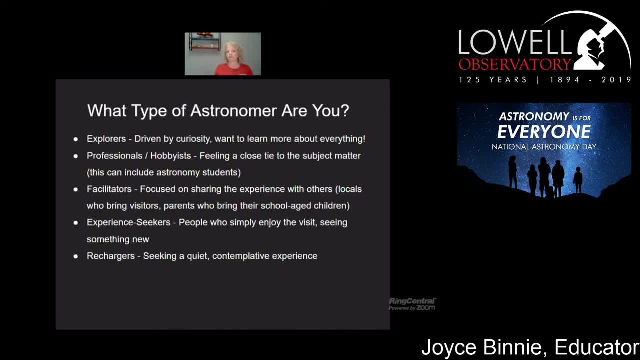 guiding at um doesn't have to just be astronomy, but we're going to. we're going to, since today's astronomy day, we're going to go ahead and just approach it from that direction. um, the first one is the explorers. they're driven by curiosity and they want to learn a little bit about. 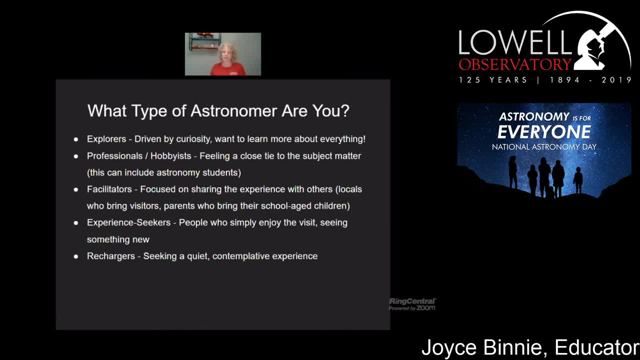 everything. the second one is the professionals or hobbyists, and we've also noticed that astronomy's students or any other kind of student in any any field, may fall into this category. you feel a close tie to that subject matter that you're going to visit this location. the third one is 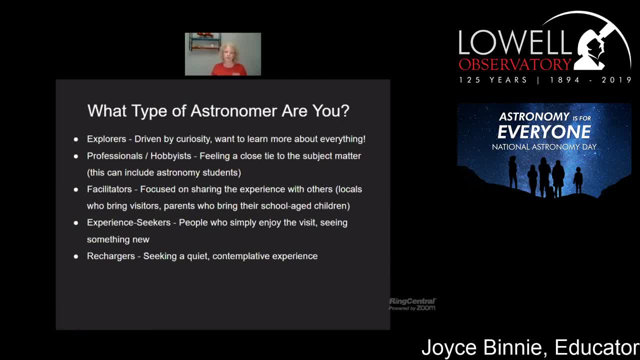 facilitators, you're focused on sharing the experience with others. right now, we know that a lot of the schools are closed, and so a lot of parents have suddenly become facilitators, trying to get their- their school-aged children motivated, since they're not actually in the classroom, maybe struggling with that a little bit, but also people like locals who bring visitors. 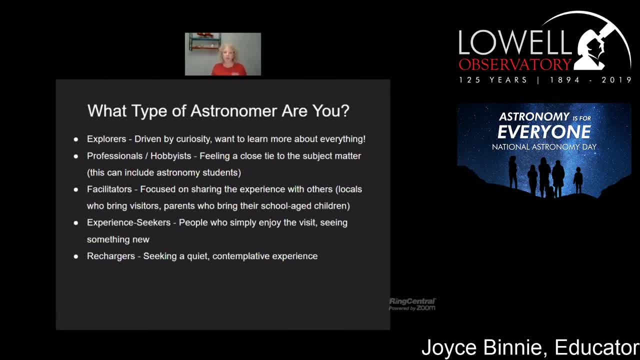 um to locations like lowell observatory. we also have the experience seekers. they're people who simply enjoy a visit, they like to see something new. and finally, the rechargers. they're seeking a quiet and contemplative experience. so myself, i identify as both an explorer and a facilitator. 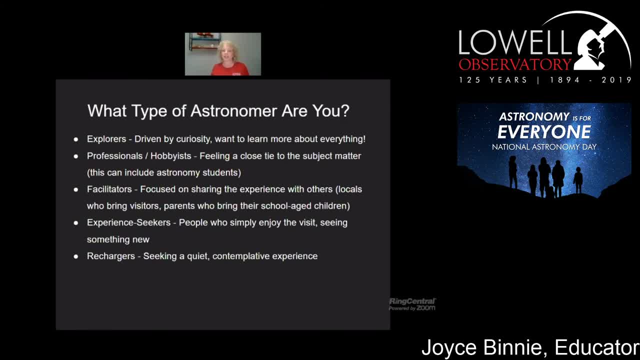 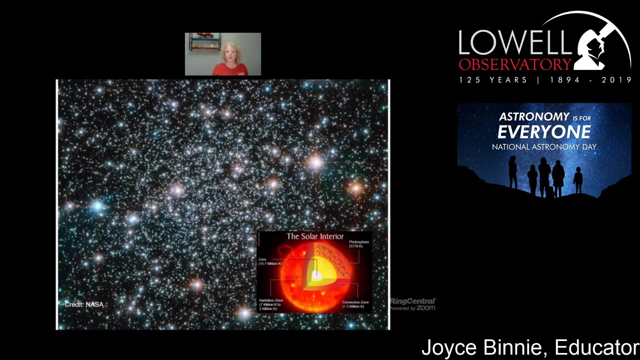 i have come to lowell observatory and have really enjoyed all of the science that i'm learning as i go along, as well as a facilitator. so the facilitator part of me loves to learn things and then share them with other people such as yourselves. now, when you look at the night sky, what is it that you see? 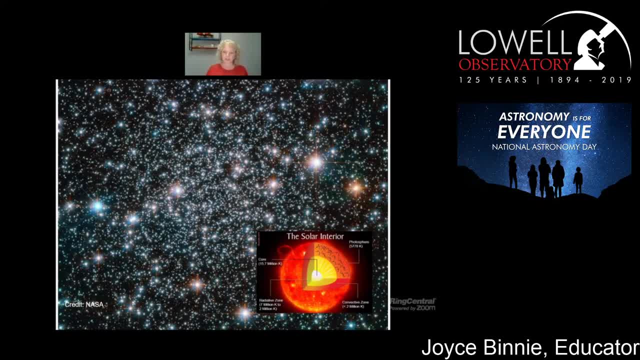 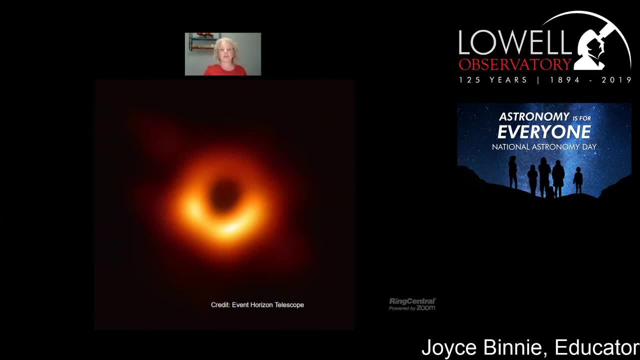 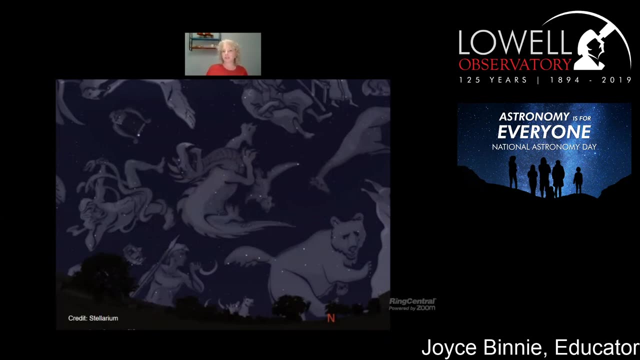 is it the twinkling stars that make you think of thermonuclear fusion, or the blackness of night that has you pondering the mysteries of a black hole? do you see pictures in the sky formed by connecting the dots of neighboring stars, and maybe that makes you think of the ancient people? 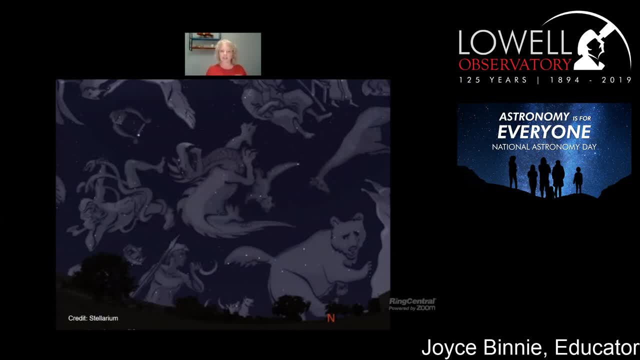 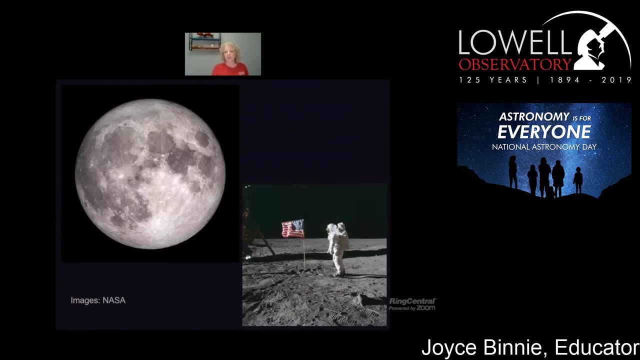 and how they would create those stories about their gods and goddesses, and also learned to know when the seasons were going to be changing. by watching that movement across the sky of their constellations that they have formed, do you appear at the moon and wonder of the ambition of the first few humans to touch its. 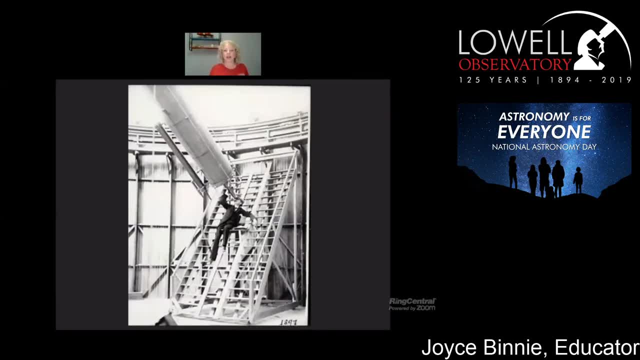 surface? or do you think of the lives of the early astronomers who must have, and how they must have, lived so dedicated to their craft that they have not been able to see them in the light of the sun, but they were willing to set aside just about everything else in life. 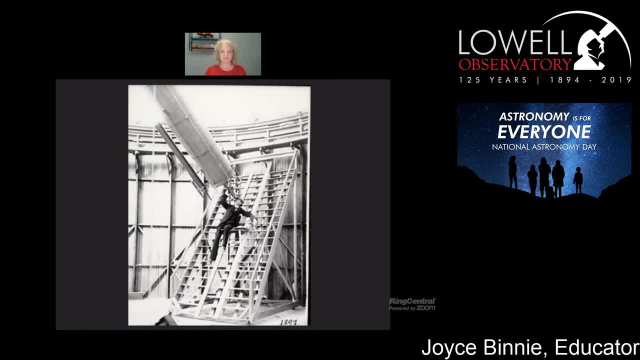 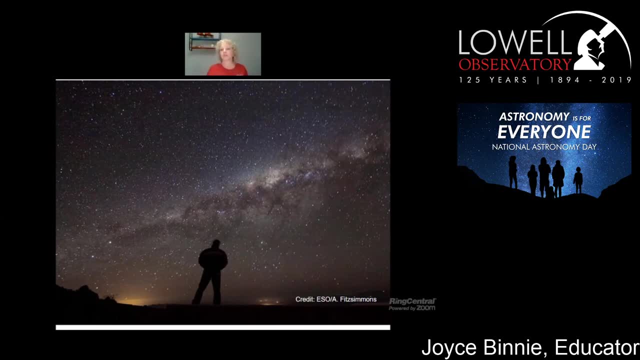 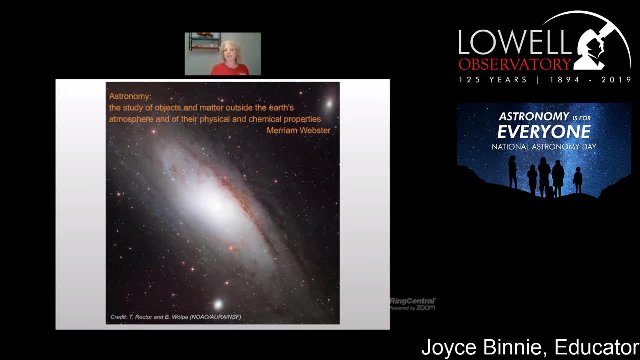 in pursuit of discovering something never before seen. maybe you just enjoy getting lost in the beauty of the universe spread out above you. so the definition of astronomy is the, according to merriam-webster, the study of objects and matter outside the earth's atmosphere and of their physical and chemical properties. but that 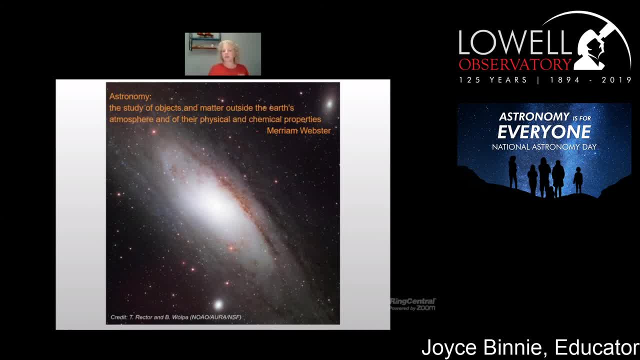 is a pretty narrow definition and we're going to talk a little bit more about that in a moment. but we know that a lot of people enjoy astronomy and don't necessarily need to engage in the science portion of it. so how do you relate to astronomy? we're going to go back to that list of different types and help you figure out. 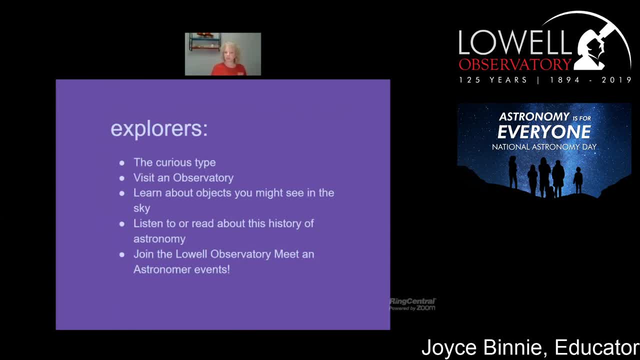 which one you are, as well as what are some things that you might enjoy if you are that type. so you have the explorers and they would identify as the curious type, and maybe you might enjoy visiting an observatory or going to a space center. like the space center, you like to learn about objects. 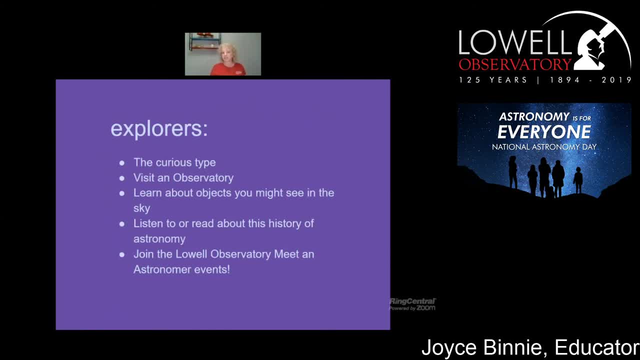 you might see in the sky. maybe you like to listen to or read about this history of astronomy or join the lowell observatory meet and astronomer events, which you typically happen on campus at lowell but are currently happening online because we are all social distancing right now. 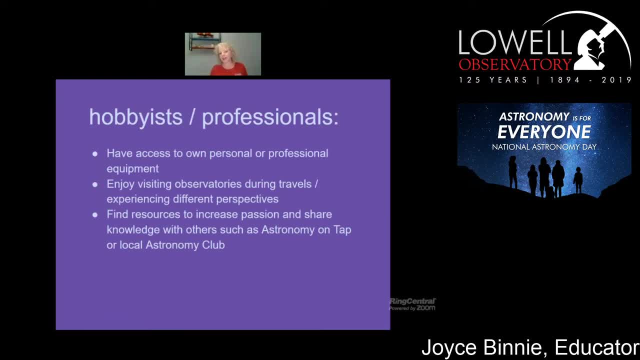 if you're a hobbyist or a professional, you probably have access to your own professional or personal equipment, but you may still enjoy visiting observatories and other space centers during your travels and experiencing different perspectives, and you may also enjoy finding resources to increase your passion and share your knowledge with others. maybe you belong to 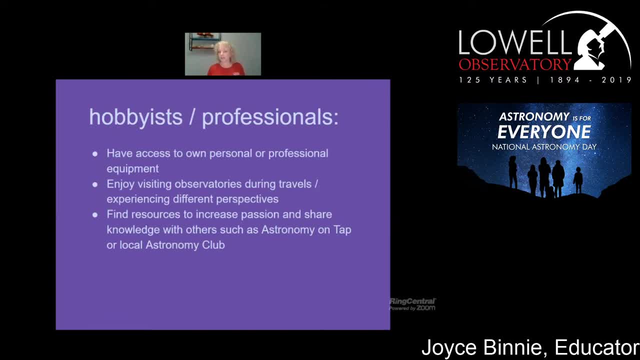 an astronomy club, or maybe you enjoy going to astronomy on tap, which is a an event that happens around to the country at different local pubs where a presenter comes in and then there is time afterwards to enjoy talking with other people who are very passionate about astronomy, and you get to have a beer at the same time. 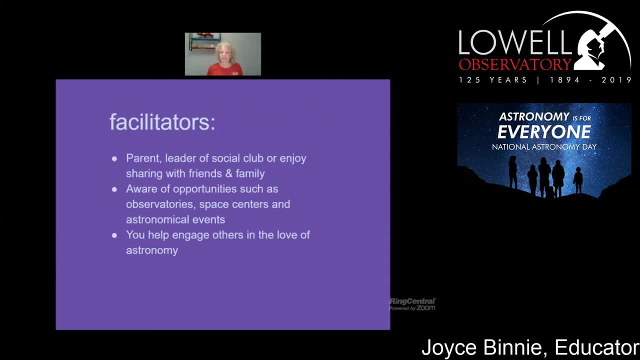 if you're a facilitator. maybe you're a parent, as i said earlier, or leader of a social club, or just enjoy sharing when friends and family come to visit where you travel together with them. you probably are aware of opportunities such as observatories, space centers and astronomical 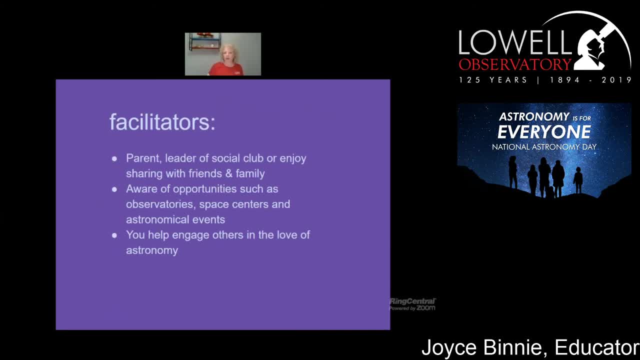 events like maybe there is a meteor shower coming up or a comet coming by, and you love you love to help engage other people and their love of astronomy. we have the experience center seekers. these are people that love being able to say: been there, done that, but in a good way. 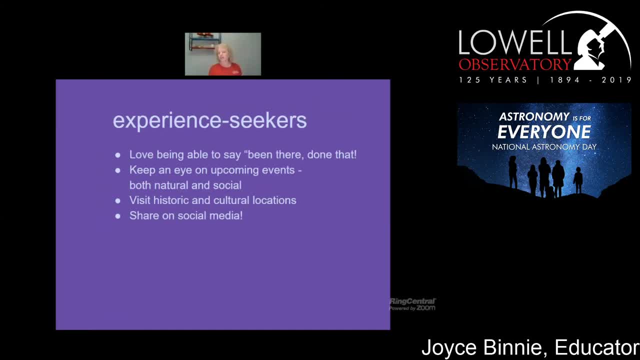 yeah, like to keep an eye on upcoming events again, both those natural- like comets coming by, meteor showers, maybe the eclipse- and social events, like maybe there's some astronomy in the park near you. you enjoy visiting historic and cultural locations and you absolutely must share it on social media. 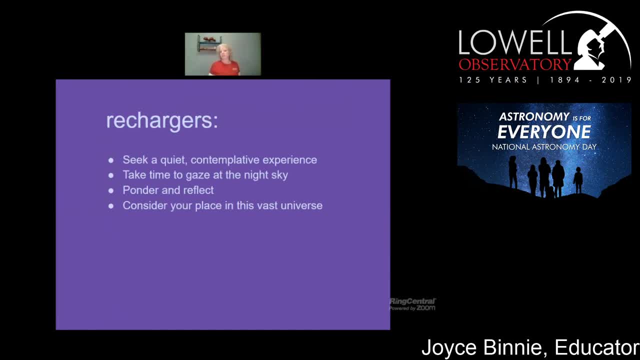 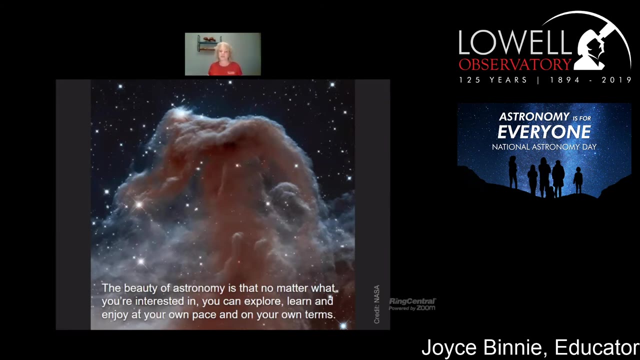 and finally, we have the rechargers. you're seeking a quiet, contemplative experience. we like to take time to gaze at the night sky, ponder and reflect and consider your place in this vast universe. there are all types of people that enjoy astronomy, so remember that the beauty of astronomy. 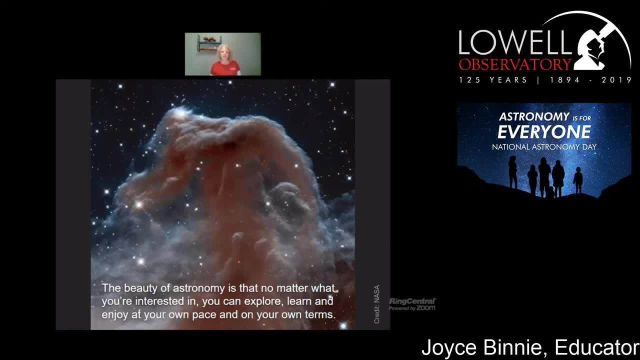 is that, no matter what you're interested in, you can explore, learn and enjoy at your own pace and on your own terms. so now i encourage you to find your identity. are you an explorer, a professional hobbyist, facilitator, an experience seeker or a recharger? drop a comment below and let us know. 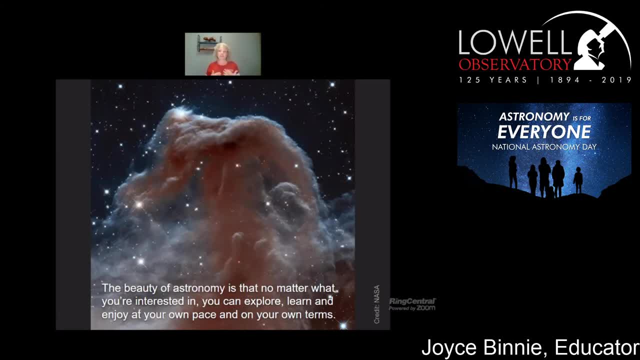 and however you identify and whatever you find your love of astronomy in, i invite you to indulge your interests, engage in nature and fill your life with the wonders of the universe. thank you, we're just waiting on some questions. if there aren't any, we will proceed. thank you, joyce, that's great. 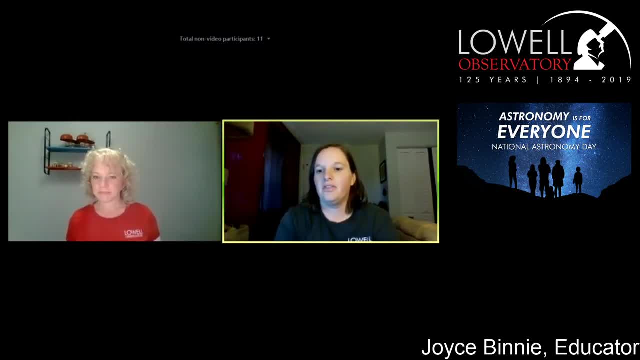 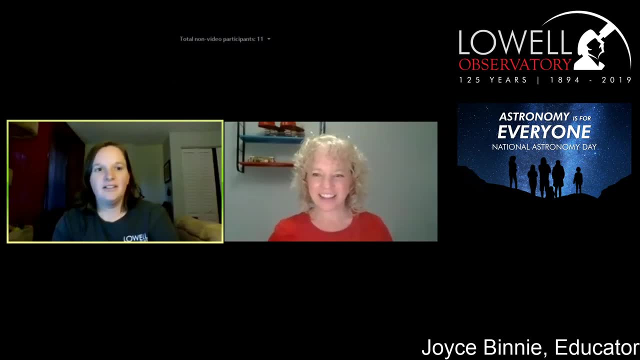 okay, is there a question? okay, i think, oh uh, all right, well, i guess she's gone or you're back. okay, uh, i think we have the question of what kind of astronomer are you, which you answer, but we can go and ask more. yeah, i consider myself both an explorer and a facilitator. 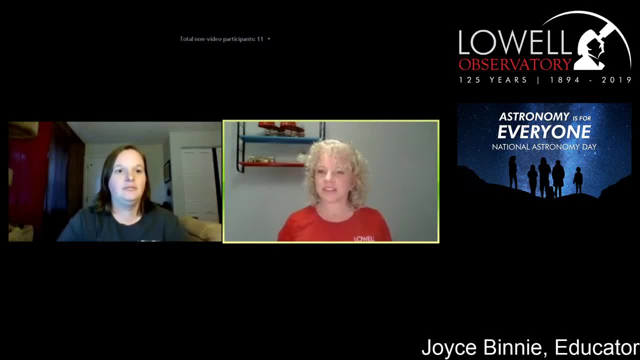 i love a little bit of everything, honestly, and so that's definitely myself and i think that anybody who's looking for what type of astronomer they are, i welcome you to consider more than one option as well. ah, okay, i see another question. um, so the uh question is: 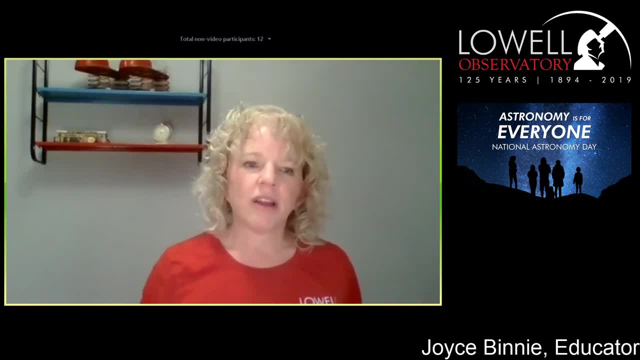 if i'm a verified interpreter. what does that mean? there is, um an organization called the national association for interpretation that does certified interpretive guide training. it is about a four-day training session and involves learning some of the very basic things about becoming a tour guide, um, and also how to put together a good presentation. 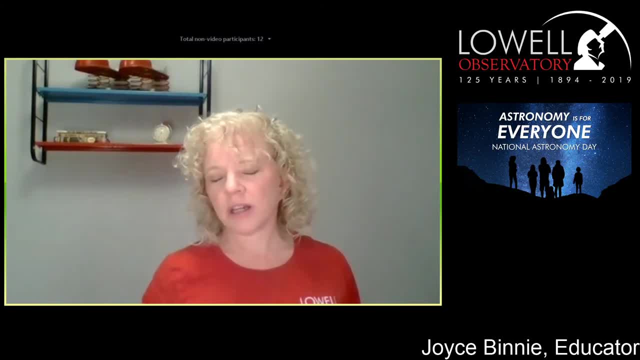 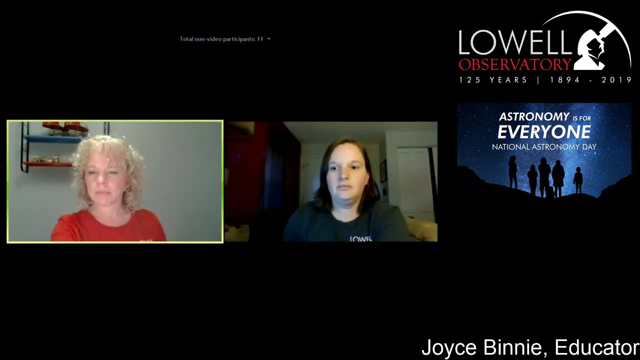 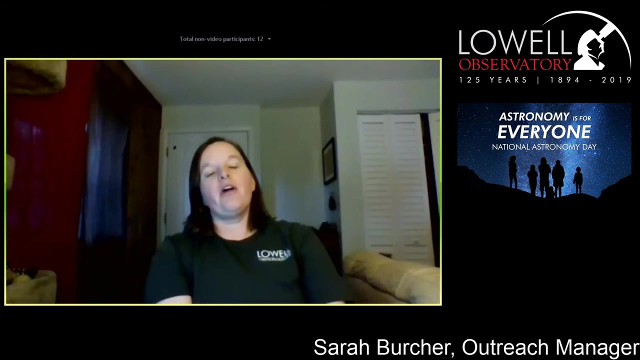 if you're interested in that, you'd want to look it up under the national association of interpretation. just um, i think it's ni naiorg, but not 100, sure? all right, well, thank you, joyce um. have a wonderful night. so now um, for those of you. 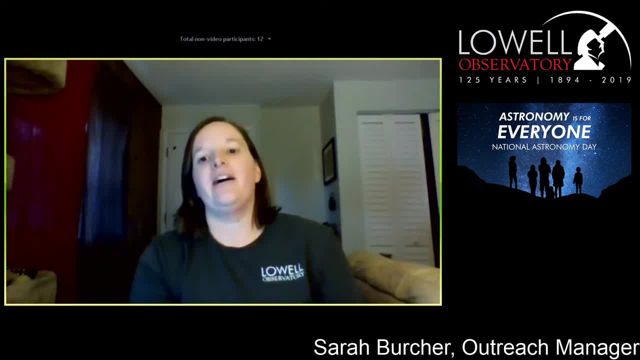 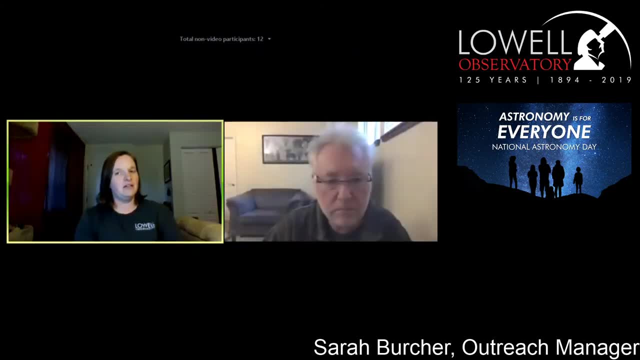 that uh identified as a professional uh in joyce's talk. i want to introduce dr michael west, who's going to talk to you about uh, how you can get paid to study astronomy and all, all encompassing things that surround it. so, um, dr west, are you ready? yes, thanks very much, sarah. 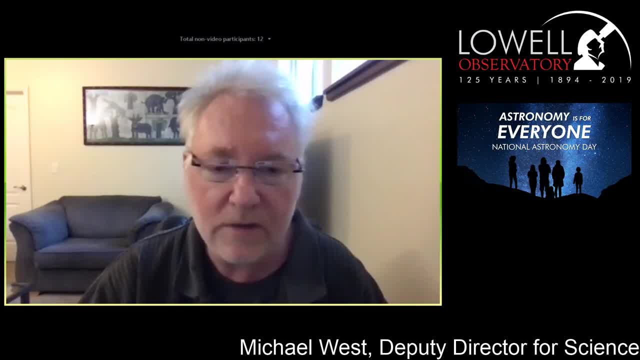 um, yeah, um, as sarah said, i'm michael. i'm one of the astronomers here at lowell observatory. what i wanted to do was just spend a few minutes telling you how you can explore the universe for fun and profit- uh, including some ways you might not have thought about before. 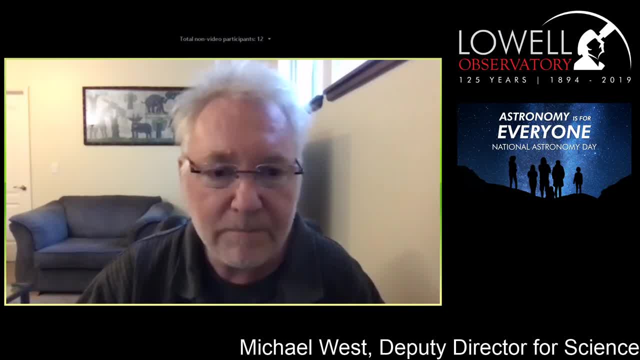 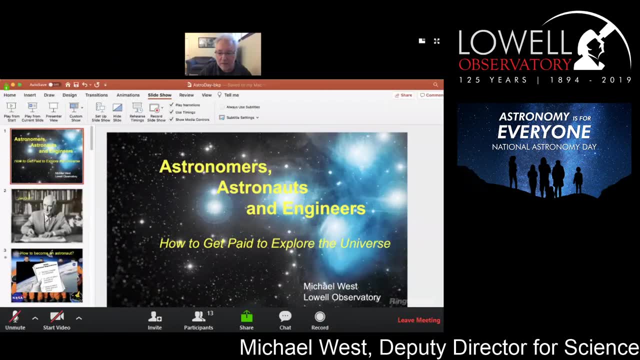 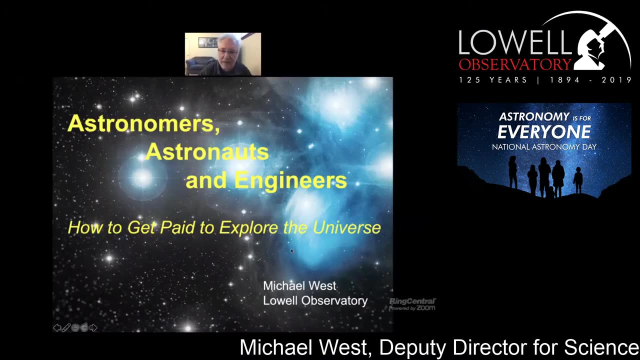 so let me just start a few slides to show you. um, hang on one second. so, uh, as sarah said, i'm a professional astronomer. i have been for uh many, many years um, but there are many ways you can actually uh earn a living uh exploring the universe, as i wanted to talk about. 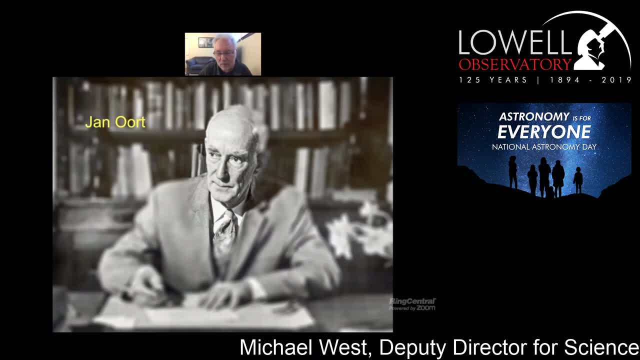 a few of those. first, i wanted to introduce you to somebody named jan wart, who you may or may not be familiar with. jan ort was one of the greatest astronomers ever, who's a dutch astronomer. he's famous for having a lot of experience with astronomy and he's known for his work in astronomy and he's 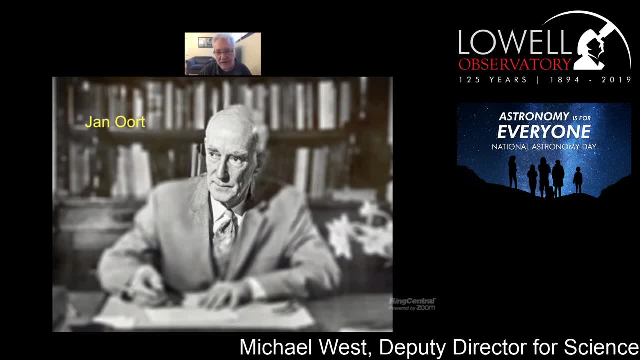 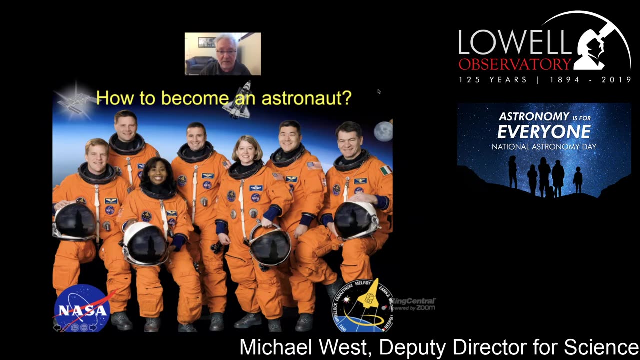 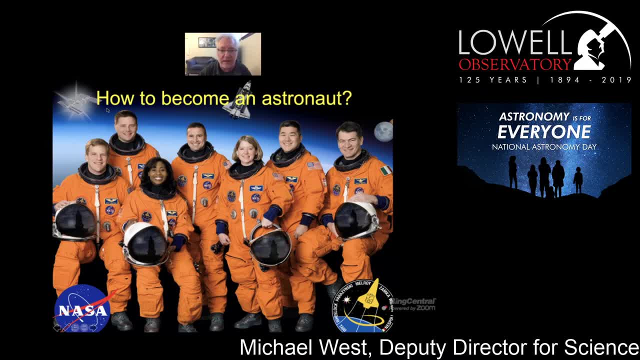 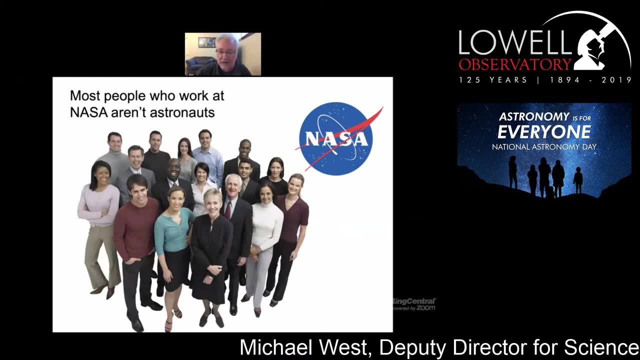 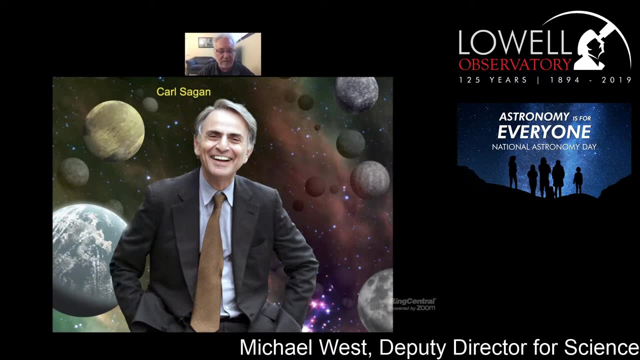 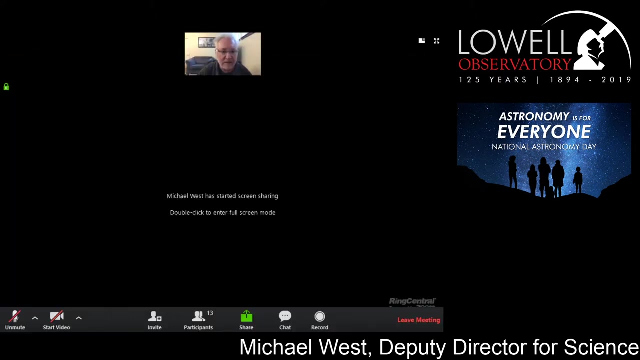 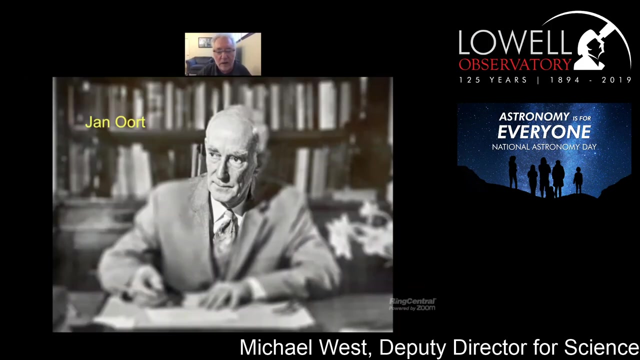 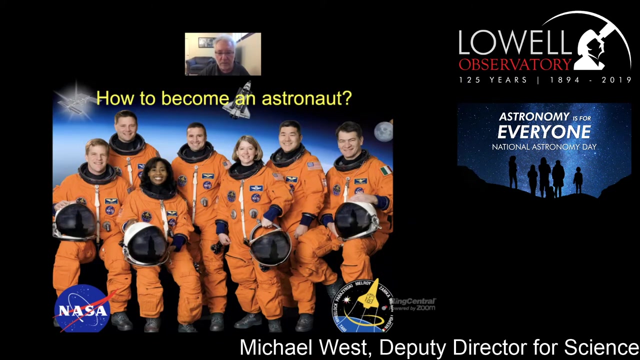 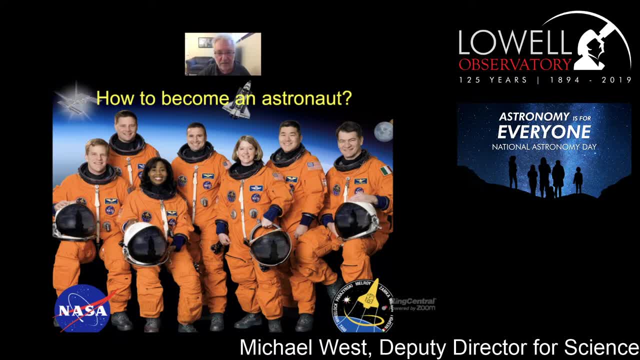 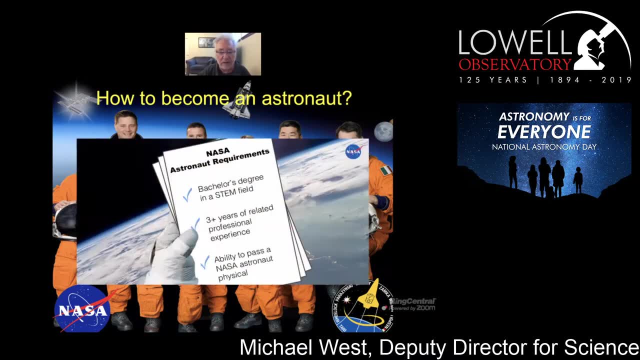 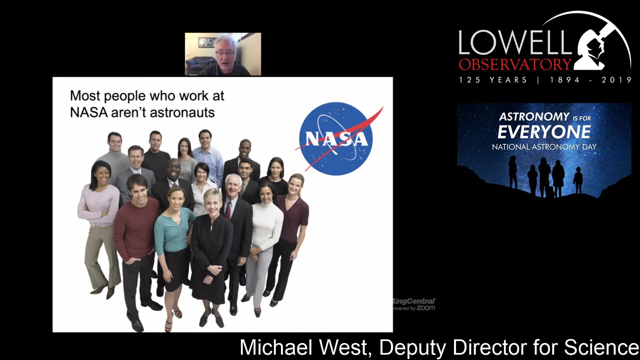 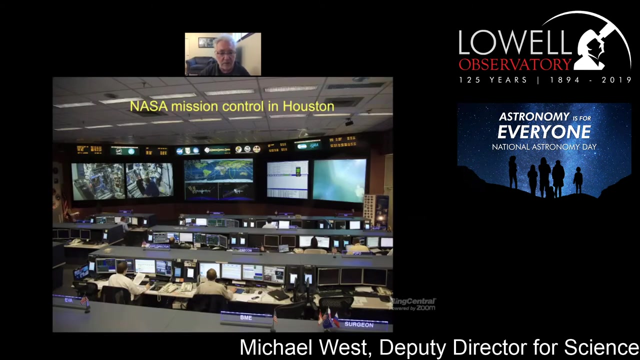 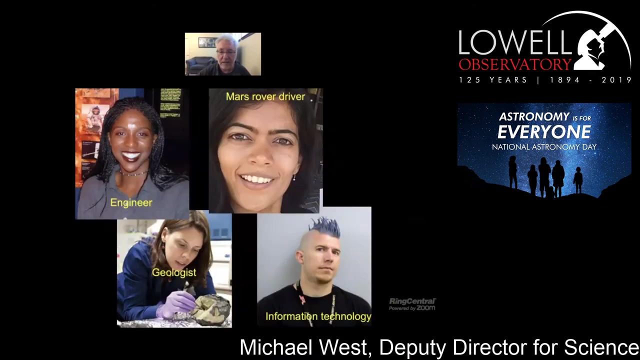 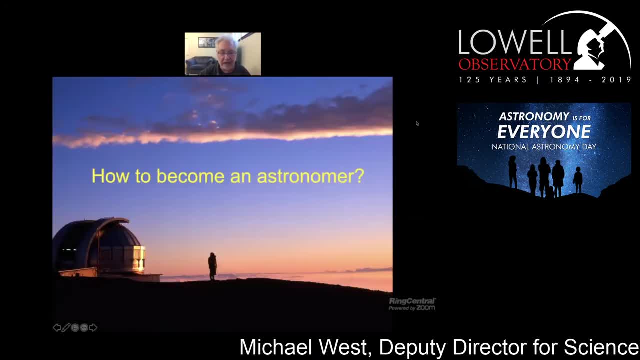 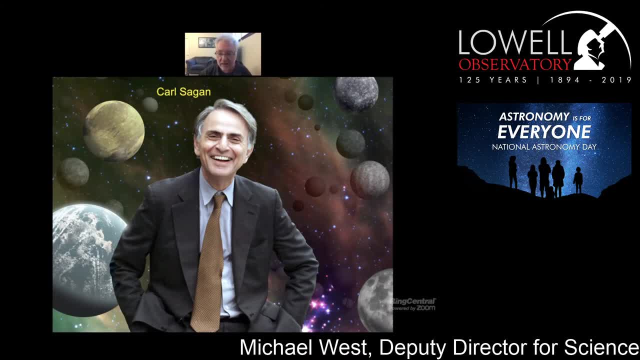 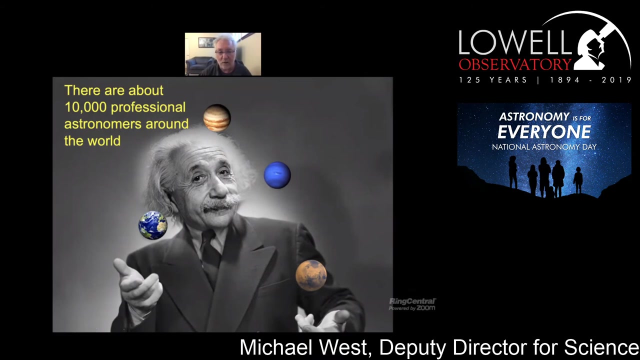 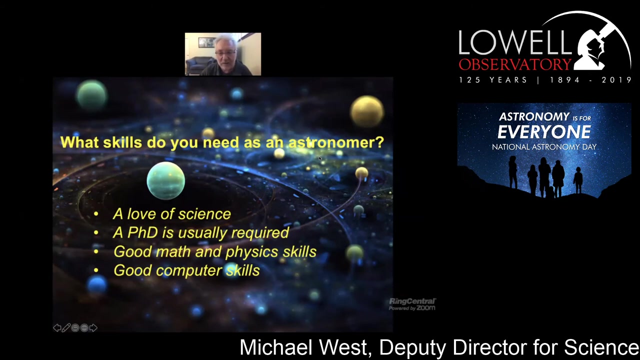 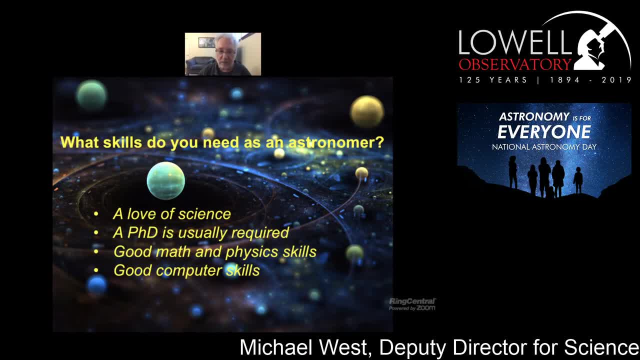 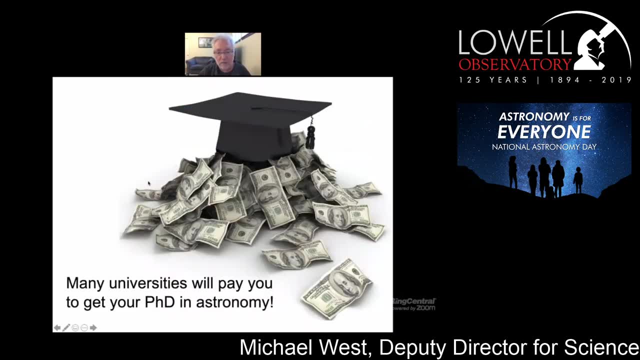 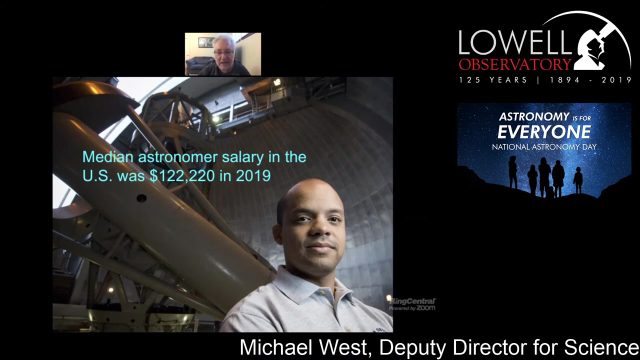 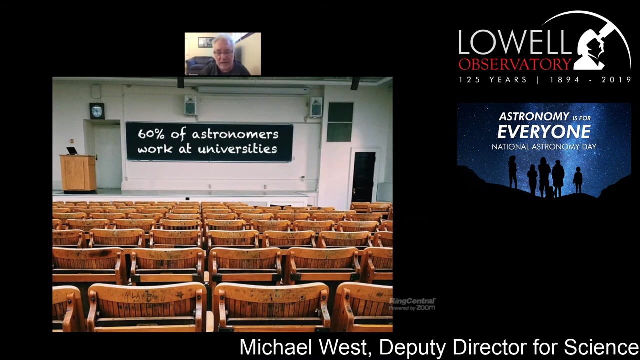 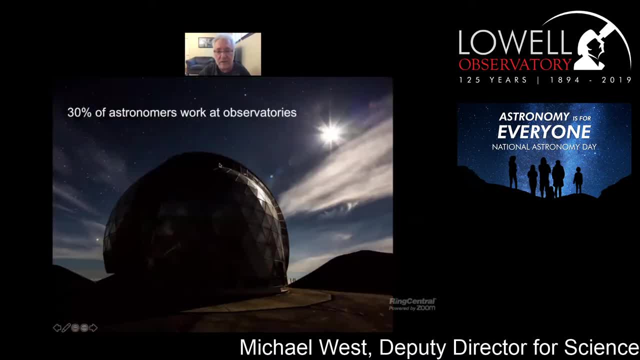 universities, where they teach classes, they do research, they supervise students, and about 30 percent work in observatories scattered all over the globe, in hawaii and china and europe, and africa and asia all over the place- australia, of course, um. so there's a lot uh of jobs there, as 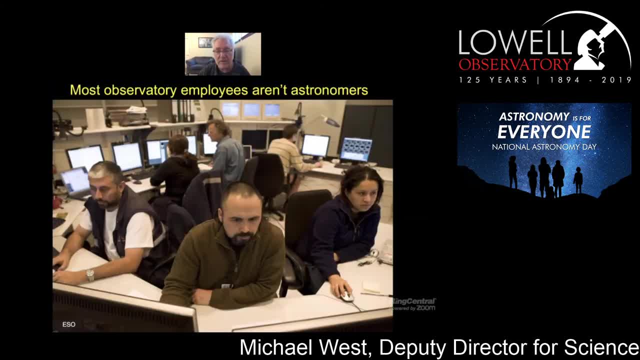 well, but most of the people that work at astronomical observatories are not astronomers again. they're engineers, they're technicians, they're the people that cook the meals for people that are working there. they're the people that buy the supplies that are needed. there's so many jobs at astronomical observatories. every one of them is essential for the success of all. 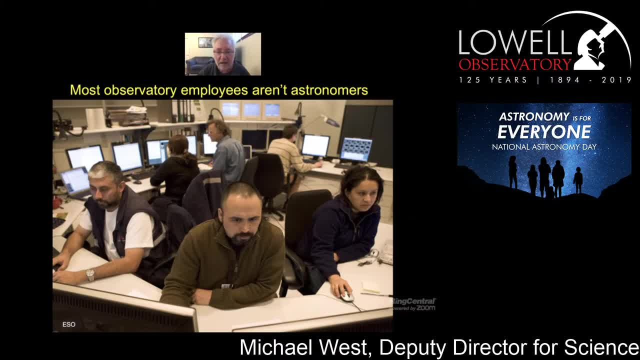 these discoveries that you read about in the papers online, we have to think of. well, astronomers made this great discovery, and it's true, but they didn't do it alone. there's an unseen army of people that support every single discovery you ever read about in astronomy. you can work for. 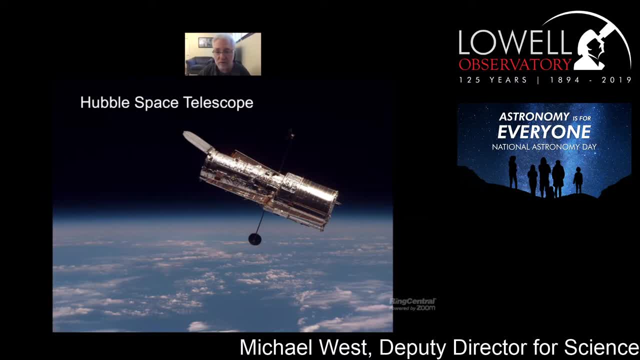 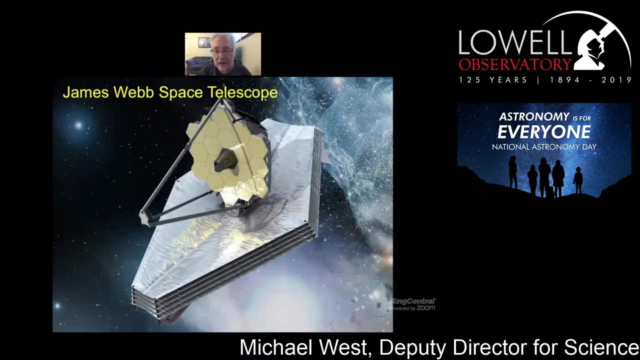 hubble space telescope. right, there's a whole need for people to work for hubble space telescope, people that can do software development, they can analyze data. that could be many different things. and of course, there's a new james webb space telescope that's coming online, supposed to launch. 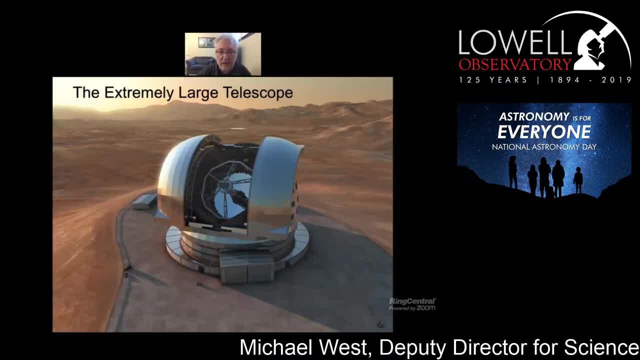 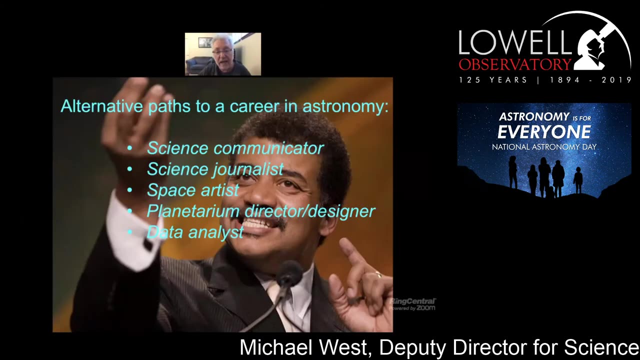 next year and there's new big telescopes being built, like the extremely large telescopes in chile. there's giant new telescopes coming online as we speak. these are opportunities to get jobs to work in facilitating the exploration of the universe and for those who don't want to, 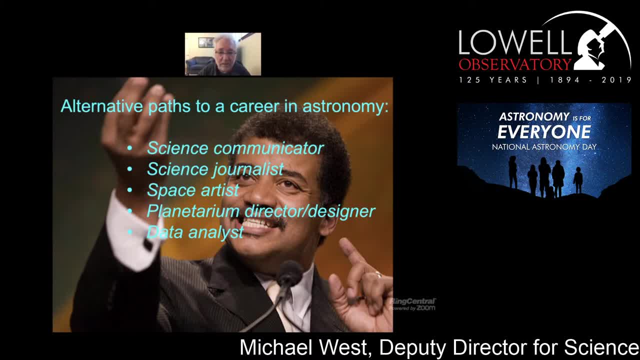 do science, don't want to do research, don't want to do mathematics. i want to emphasize that there's many other ways you can get involved in astronomy. you could be a science communicator. you could be a journalist and write about astronomy. you can be a space artist. you can work at a planetarium, you can analyze data. so, for example, 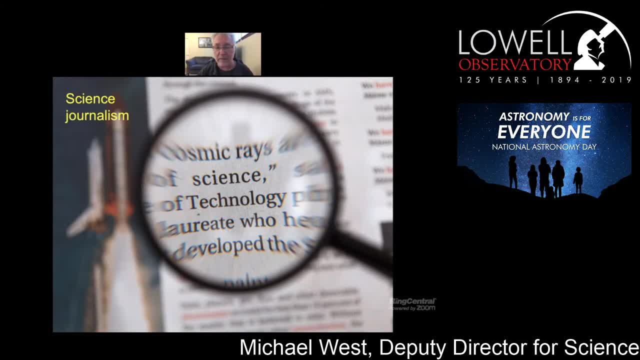 science. journalists write articles for many of the magazines that you read, or they write books about astronomy. if you're good at writing, think about this. there's a big need for people that are science communicators, that can translate astronomical discoveries into things that the public can understand. dave eicher is a good example. 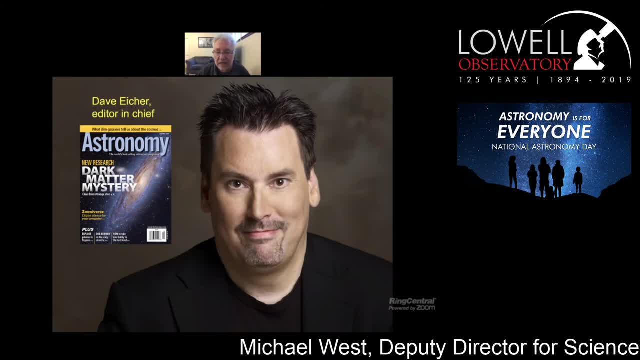 dave is the editor-in-chief of astronomy magazine. he's been passionate about astronomy since he was a little boy. as a teenager, he created his own astronomy magazine and that was a stepping stone to ever bigger things that today. he's now a well-known author and also the editor-in-chief. 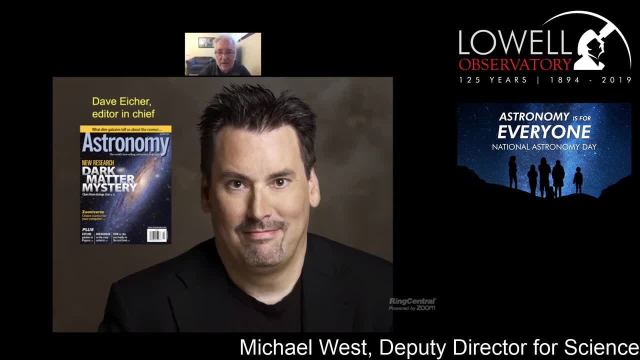 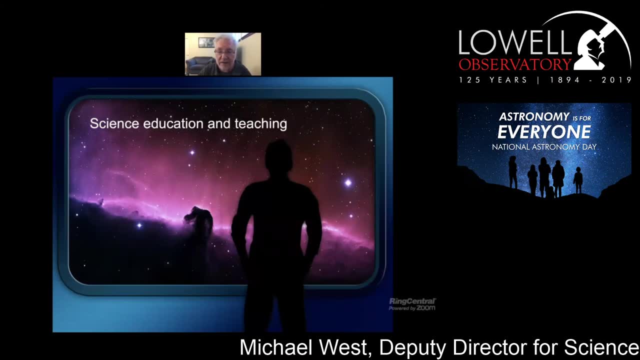 of the world's leading astronomy magazine. so good example. somebody was able to turn his passion into a living. of course, you can also be an educator and a teacher. we've heard more about this, uh, just in the last few minutes. we'll hear more about this, uh, as we continue this evening as well. but teachers are crucial. right, i was really. 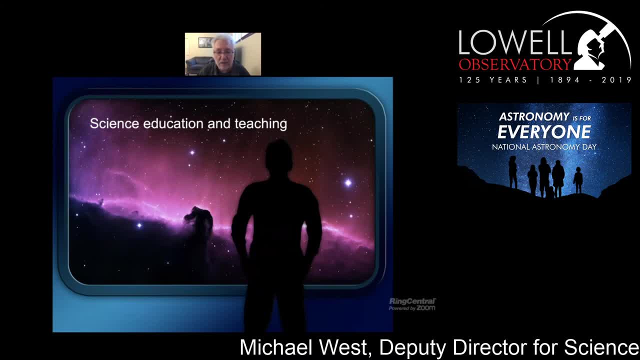 fortunate, when i went to high school, i had a high school science teacher who had a phd in astronomy, and that was a magical thing. it really impacted my life too, and any one of the teachers out there, anyone who thinks you might like to teach kids, who might like to educate people- the educators. 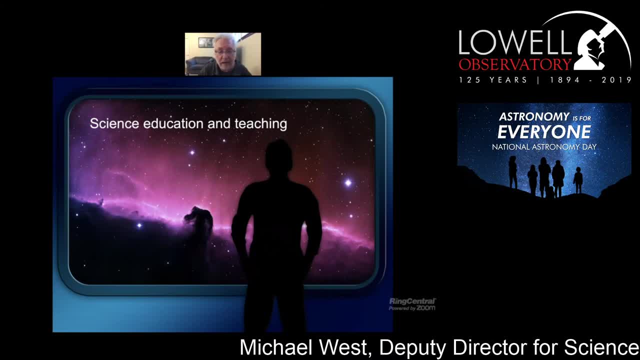 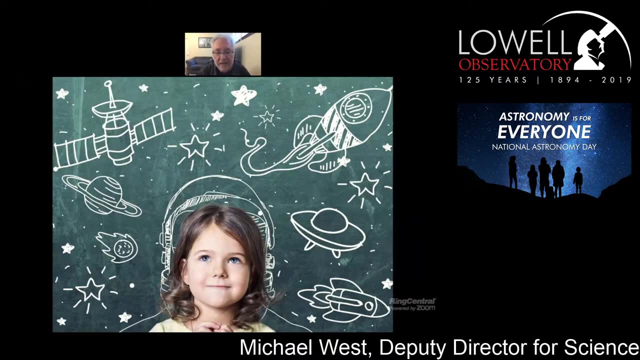 are low, are world-class at communicating uh what we understand about the universe to the hundreds of thousands of visitors we get each year, and so if you want to be a teacher, you can be the one that inspires that little girl or that little boy to become the next astronomer, to become the first 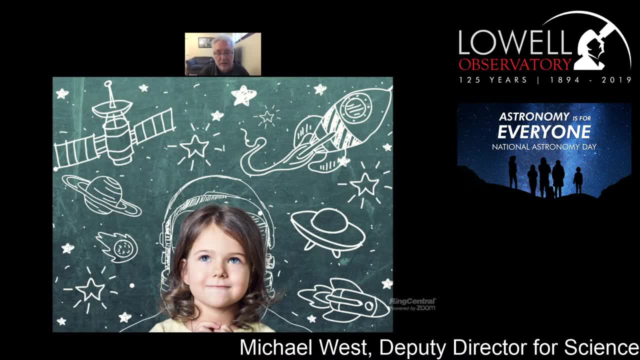 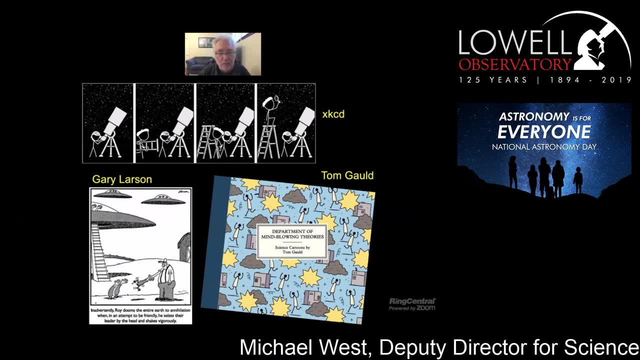 person to walk on mars. there's a huge opportunity here for you where you can help enable and facilitate the exploration of the universe. you can be the one who's going to be the first to walk on mars of the universe. and if you want to do something even more offbeat, you can be a cartoonist, for. 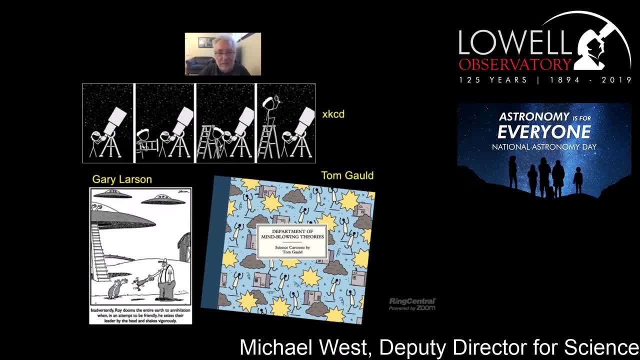 example, there's a bunch of cartoons like i show here: xkcd, if people read. or gary larson, of course is a well-known cartoonist. or tom go just has a brand new book came out, department of mind-blowing theories and it's ways of making the universe and science funny and entertaining for people. but 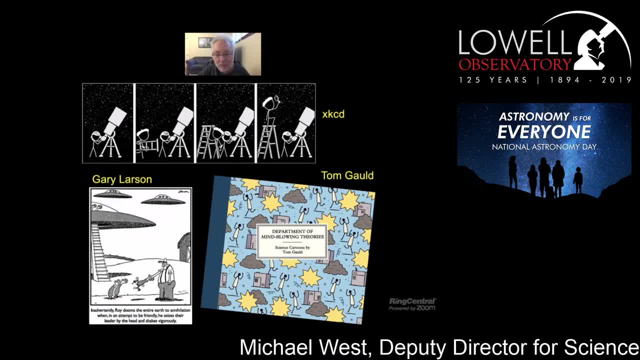 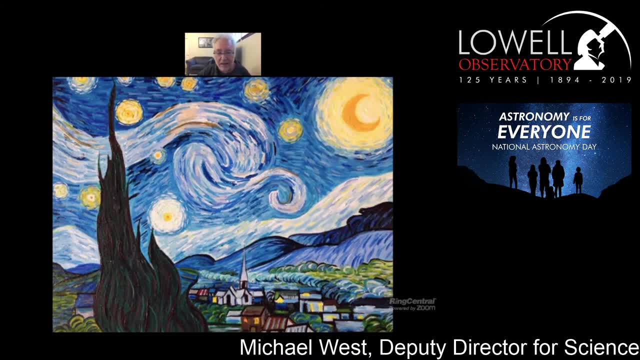 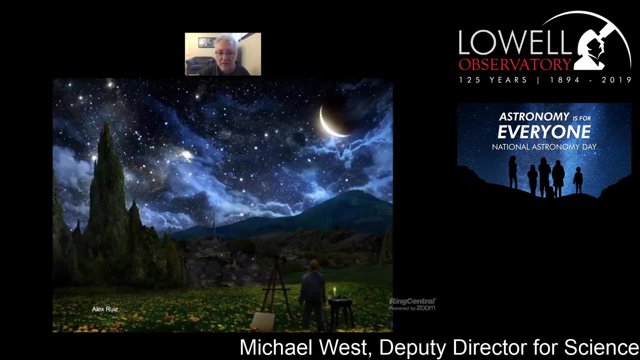 sneaking in a little message, often too right, and that's a really powerful way to communicate science. if you like art, everyone knows this well-known picture of vincent van gogh and uh, the starry night, uh. and if you like art, what a great way to bring together science and the arts to reach people. here's a really 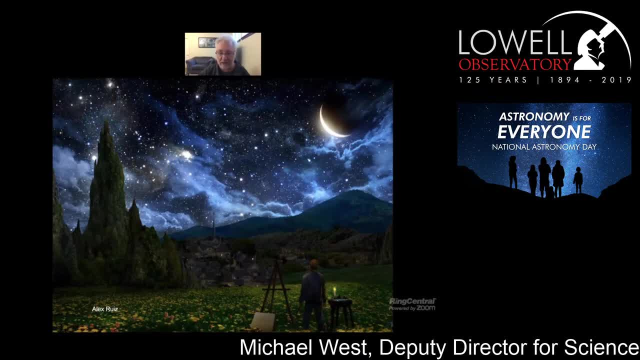 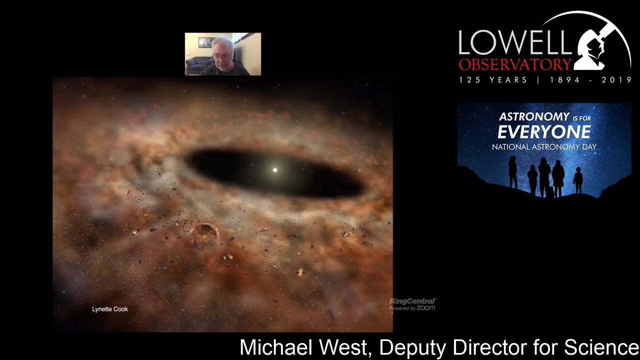 beautiful uh painting i like by uh, an artist named alex reese. he it's sort of a meta painting. he imagines van gogh getting ready to paint a starry night in the sky that you looked at um. likewise, this is a beautiful image by lynette cook. lynette is the science illustrated artist and she um. 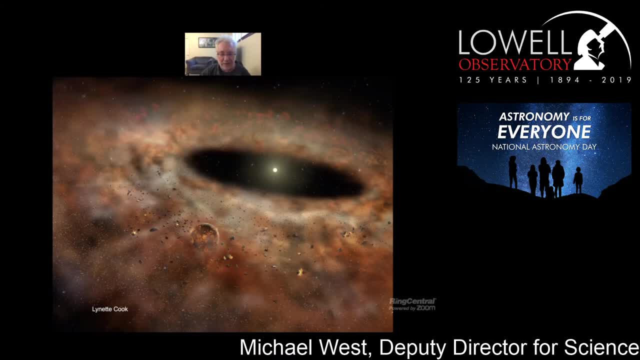 illustrates things in astronomy that we can't see with our naked eye or telescopes. so this, for example, is her illustration of the birth of a solar system and what it might look like, and it's really powerful to be able to take these sorts of abstract concepts and make them. 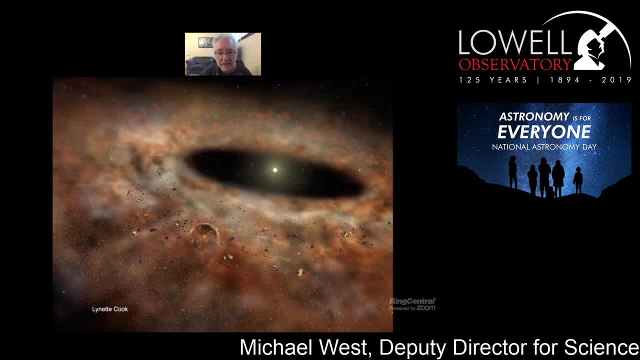 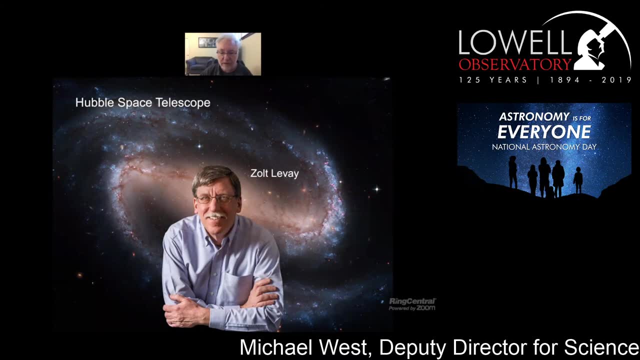 something that people can visualize. so if you've got artistic skills, think about applying them to astronomy. there's a great need for this. here's another great example: salt levee. salt worked with hubble space telescope for many, many years, and every beautiful image you've ever seen from a space telescope he had a hand in. 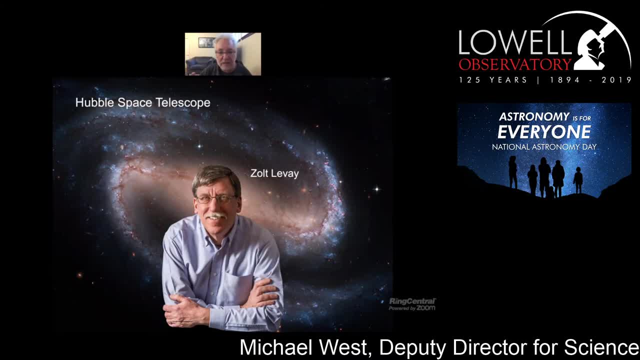 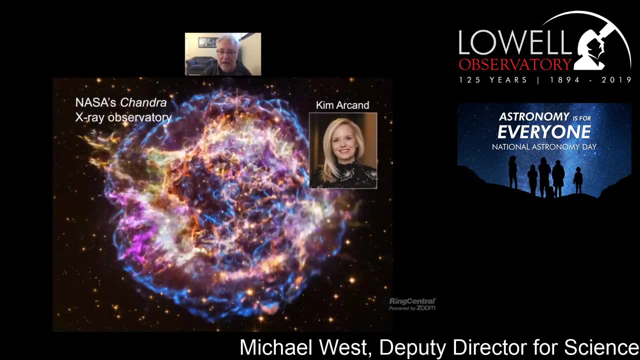 He's skilled at processing images, picking out details, pulling out the colors to convey information. Likewise, Kim Markhan is another example where she works at the Chandra X-ray Observatory. And again, X-ray light our eyes can't see. 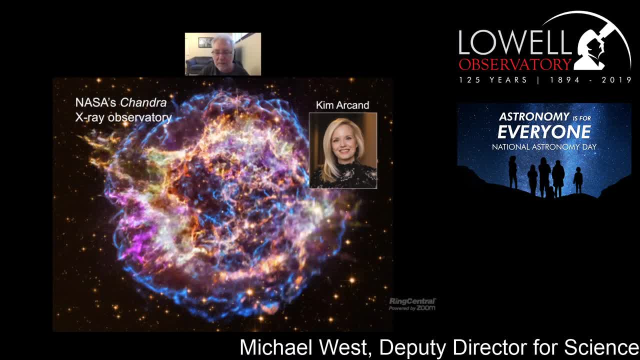 What color is X-ray light? What color does a star that's emitting X-ray light show? You need to pick these colors. You need to have some artistic skills and flair to communicate information through visual images like this. So, if you like that, if you like the arts, 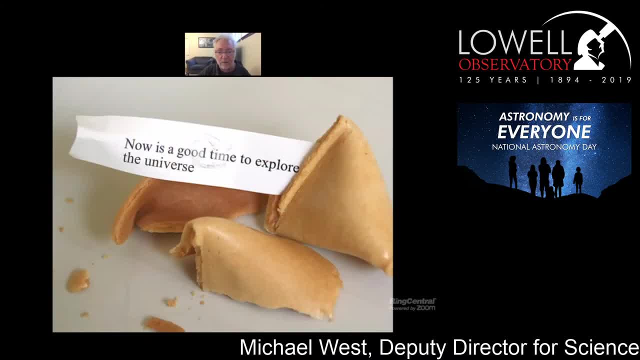 think about this as a way to get involved as a career in science going forward. So I'll just finish up by saying: you know your fortune cookie says, if you're interested in astronomy and you're interested in science, now is a great time to get involved in exploring the universe. 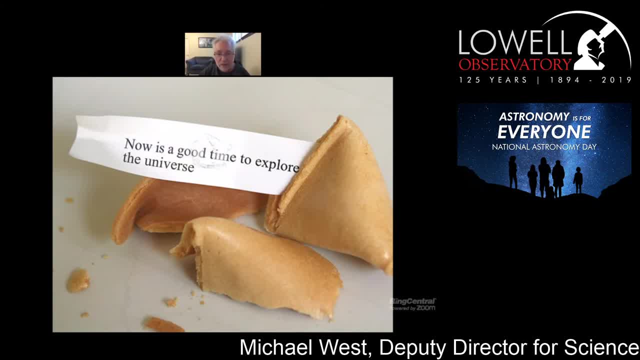 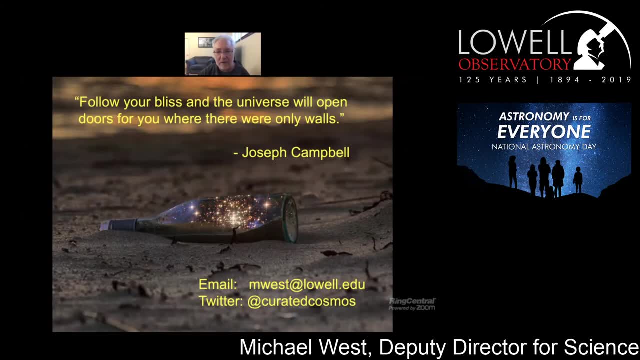 This is the golden age of astronomical exploration And, yes, you really can get involved if you're interested, in many different ways. So I'll just finish up with what I think is a nice quote from Joseph Campbell: follow your bliss, and the universe will open doors for you where there are only walls. 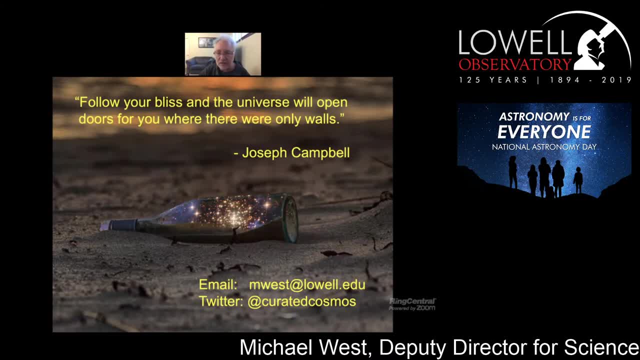 So if you have any questions about careers in astronomy, whether as an astronomer or in another field, my email address is below and my Twitter handle, So please feel free to contact me and I'll be answering any questions you might have. Thanks, Sarah. 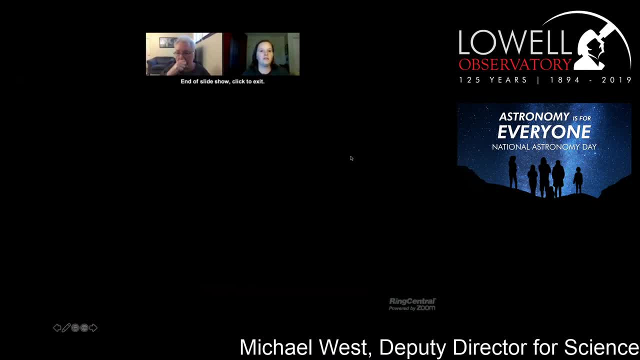 Michael, it looks like there's a couple of questions for you in the chat. if you want to take a quick look, Okay. So the first- I'll just relay them to you- is: what was your first telescope? So I well, this is embarrassing. 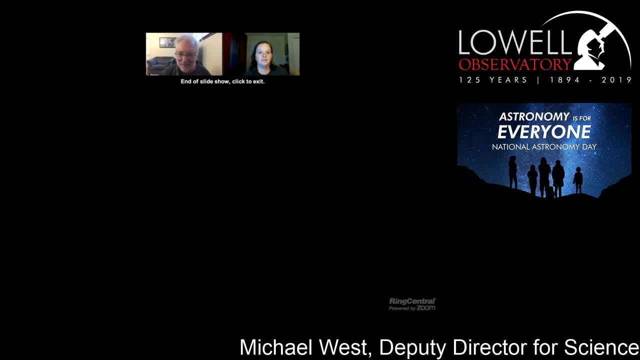 I, when I was in high school, I bought a telescope. I saved my money. I saved, I bought a. the brand was Criterion, I didn't know they even exist anymore And I'd bring it outside at night and I'd look through the telescope and it was really cold. 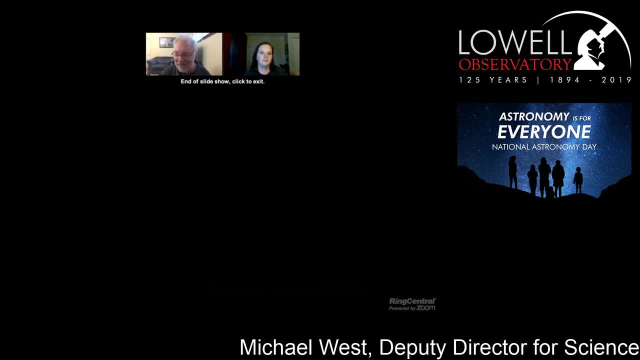 I grew up in Connecticut. It was really cold And then eventually I sold the telescope and it became. I didn't become a theoretical astronomer. I did computer simulations. That was my PhD thesis And then over the years I gradually got back into observational astronomy. 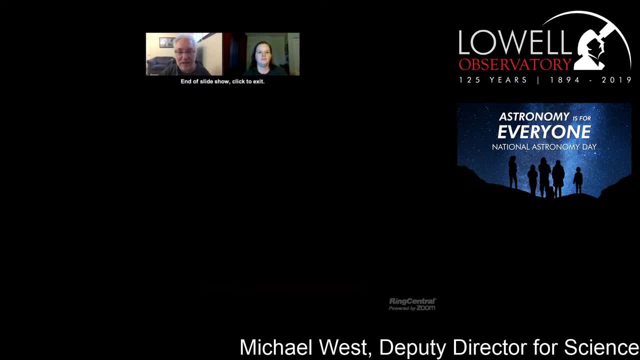 But my first telescope was a six-inch reflecting telescope that I saved long and hard to be able to buy it. Let's see. the next question I see is what's the benefit to astronomy universities to pay you to get your PhD? How does that work? 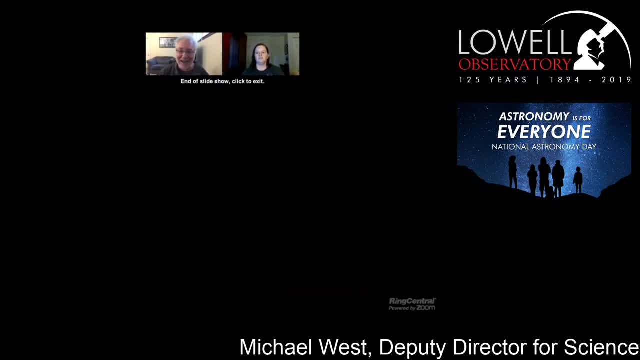 Yeah, my wife asks that question all the time. I think you know like many things you know if you go to university. right, it's not just about money, It's not just about finances, It's about an education. 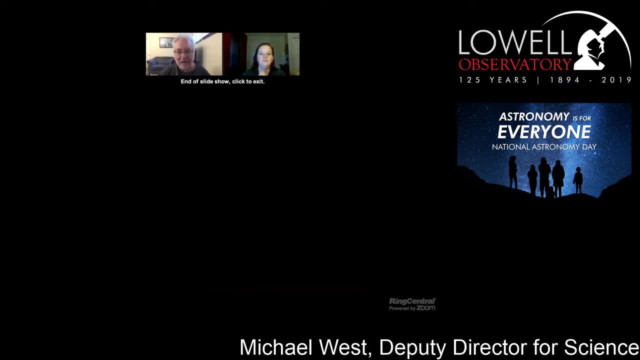 It's about exploring all the different facets of education And in astronomy in general. there's not a big market for it. There's not a lot of people going to astronomy, And so to encourage people to come, universities sometimes contribute financially. 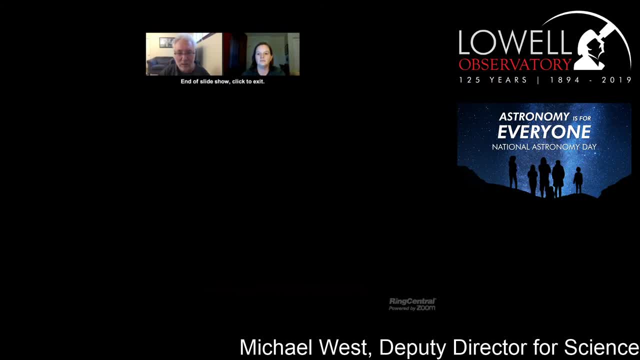 Also I should make clear that often- and I think Deidre alluded to this- is you work for a professor who helps pay your salary- part of your salary at least, which they have research grants for things like that, And then also you work as a teaching assistant. often 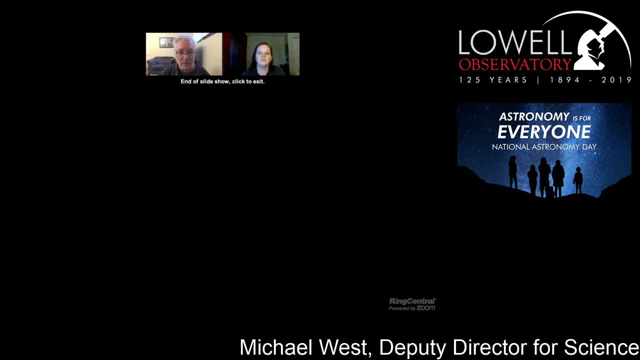 So the universities rely on you to help grade tests, for example, and to help with other. you know, when I was in graduate school, I used to do tutorial sessions. right, You help teach the stuff that they should have learned in lecture. 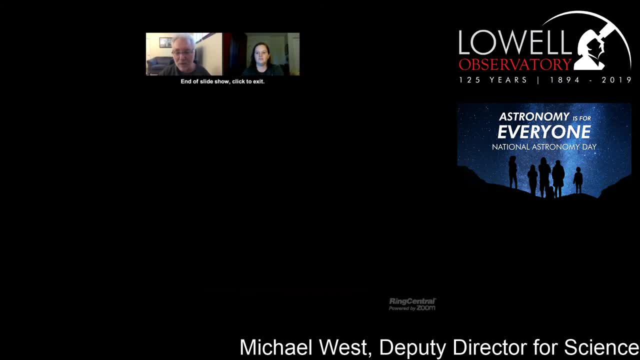 but you were there to help reinforce some of them, And I think that's one of the main ideas. So I think that's part of the reason that they do this as well. Let's see. So, let's see. Sorry, let me stop the screen share. 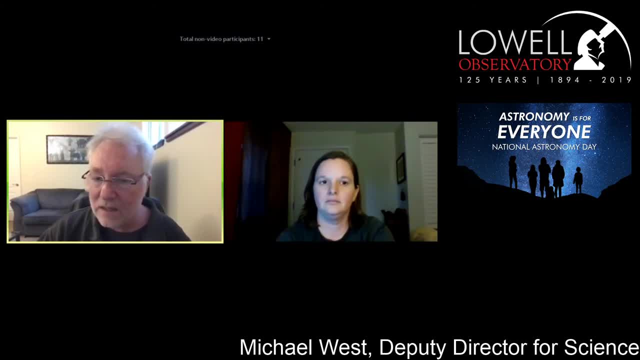 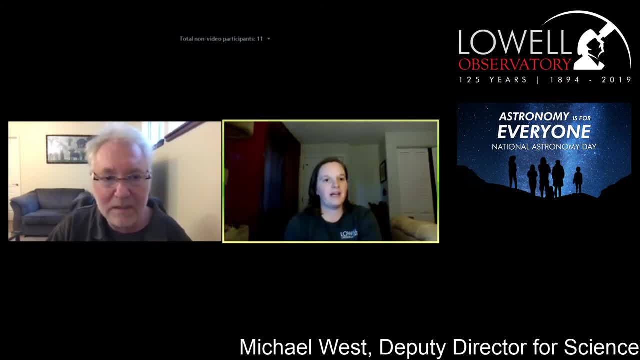 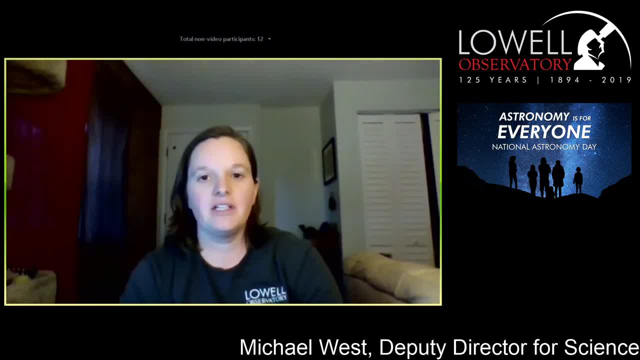 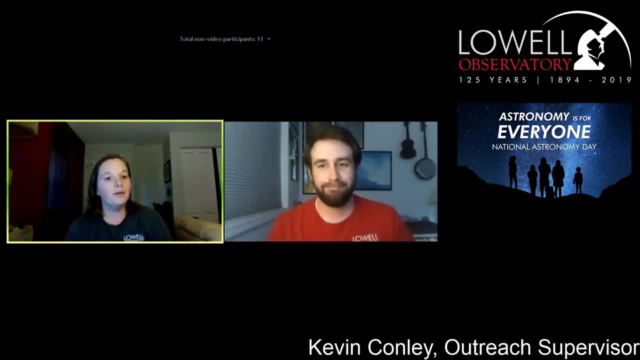 Yeah, So next up we have another one of our educators, Kevin Conley, who is going to bring us through a way to bring constellations into your own home. Spending a lot of time at home nowadays, So Kevin's going to teach you how to make it a little more exciting. 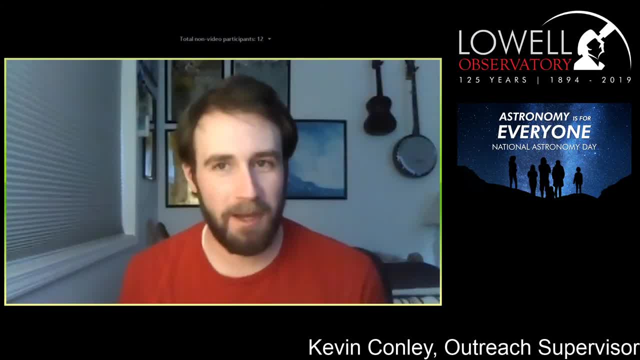 So, Kevin, take it away. Thank you, Sarah. Hello everybody, My name's Kevin. I work in the public programs here at Lowell Observatory, And while we're here, I'm going to give you a little bit of a tour of the school. 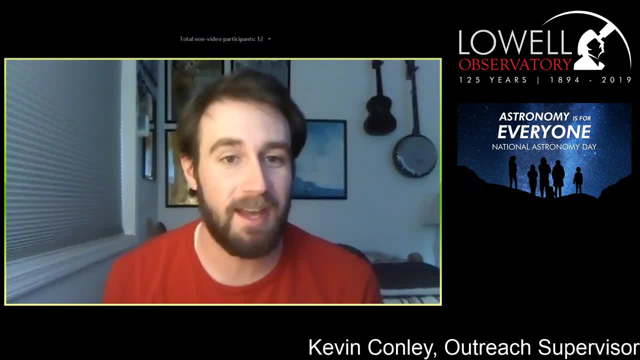 While we're all stuck at home, not all of us get to see the lovely, nice sky. The stars have been used to tell stories throughout human history. People have used them to navigate, People have used them to know when to plant and sow their crops. 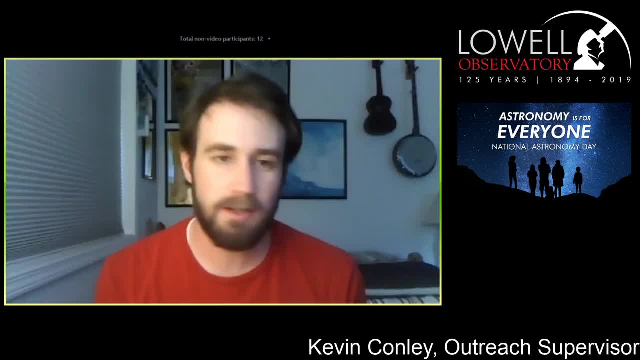 Fortunately for me, I grew up in an area where the stars are available right outside my back door, just a few steps, And I can see those constellations that everyone talks about. Some of us aren't so lucky to be able to do that. 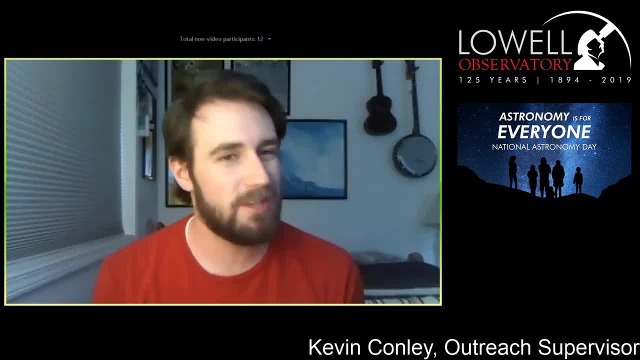 We live in a place where it's much more cloudy, Or you have some light pollution that kind of blocks out some of those stars. So for the next few minutes I'm going to go over an easy do-it-yourself at-home project. 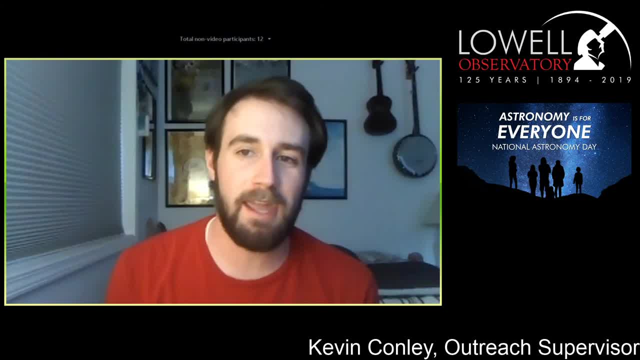 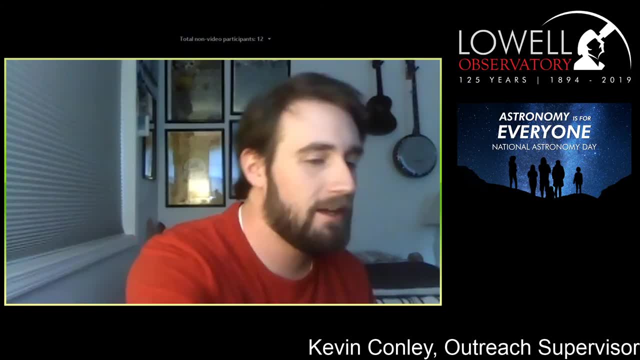 for some kiddos to develop what I like to call a flashlight manateric. for you kids, It doesn't require a whole lot of supplies. All you need is just some cups here, something to poke the holes in the cups and then a 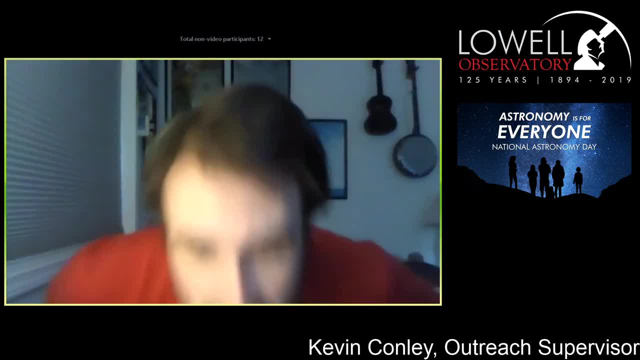 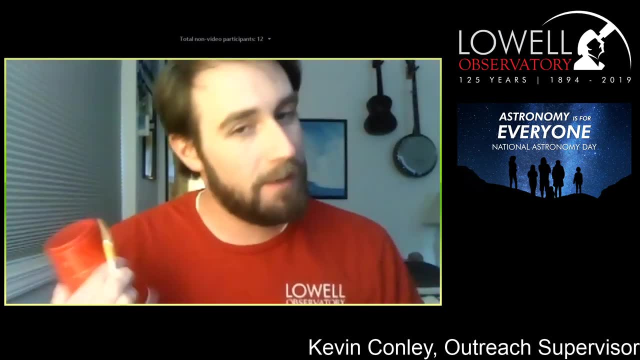 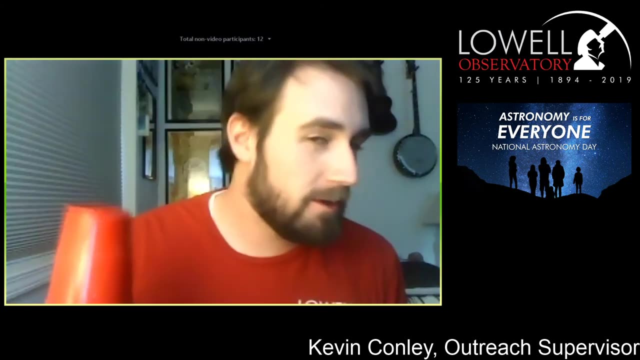 trusty flashlight here for us. So all you have to do is take one of those cups, your sharp instrument, and start poking holes into that cup to allow the light to pass through. I prefer using a plastic cup over a paper cup here, because the plastic cup will block. 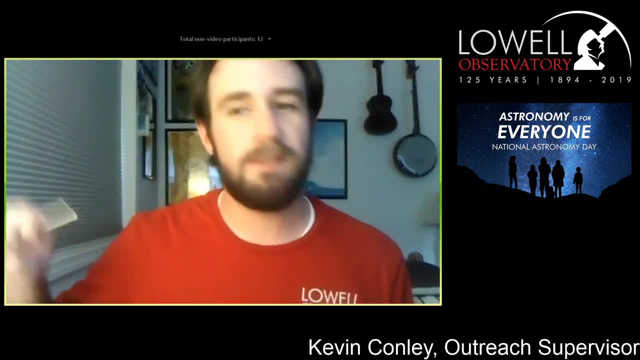 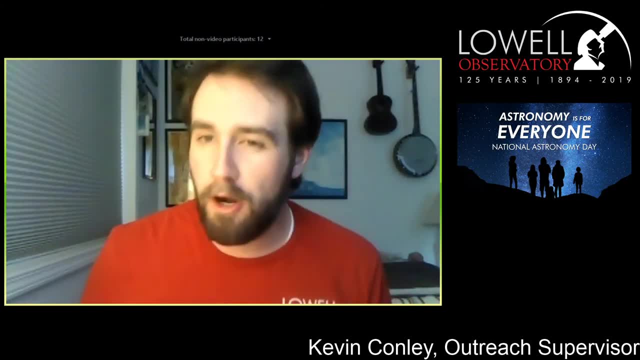 out the rest of that light from your flashlight, give you more definitive stars on the walls that you're projecting towards. So I have a few already prepared, Pre-made here. The sun's still slightly up here in Blackstaff so I can't get it quite dark enough to try. 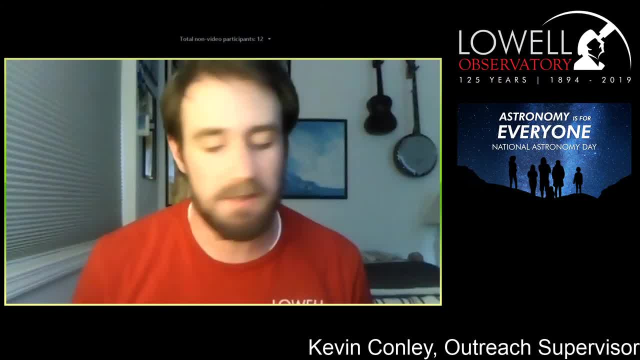 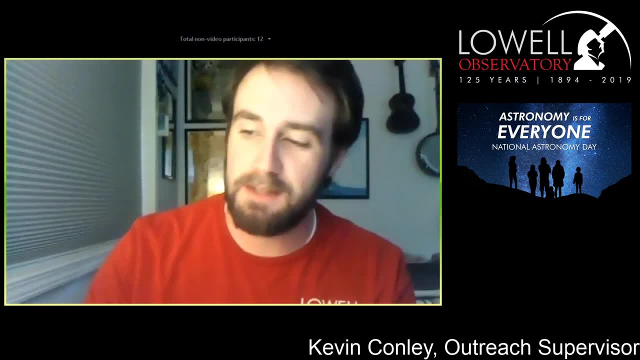 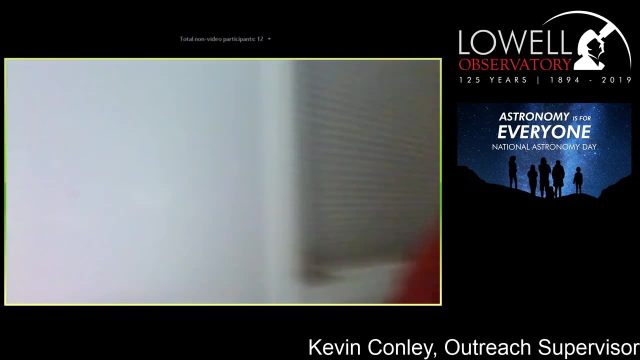 and show off all these little pinpoints of stars I was going for. But I'm going to do my best here to show the complete process after you poke those holes into the cup there for you. So I'm going to get a little bit darker here and try and point this towards the walls. 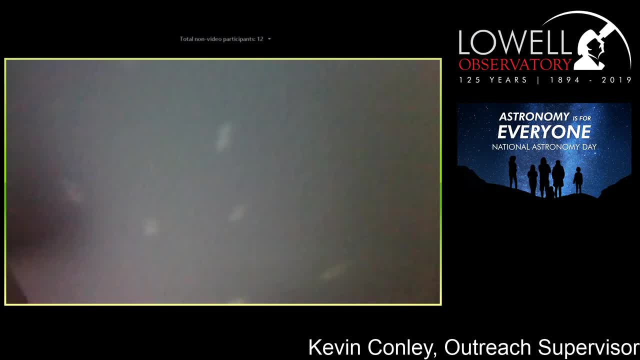 hoping it's starting to come through a little bit, But if you do it right you can start seeing those stars. You can see the stars projected onto the wall there. for you And with kids, there's a couple different ways to go with this project. 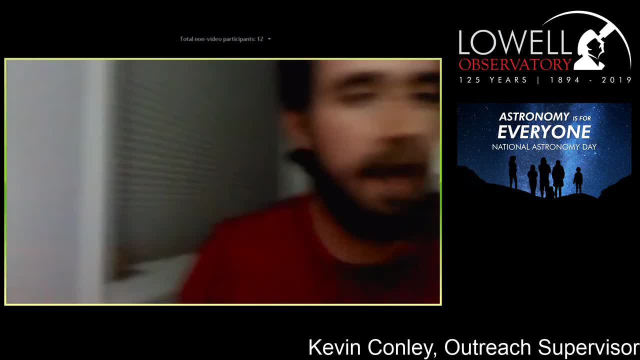 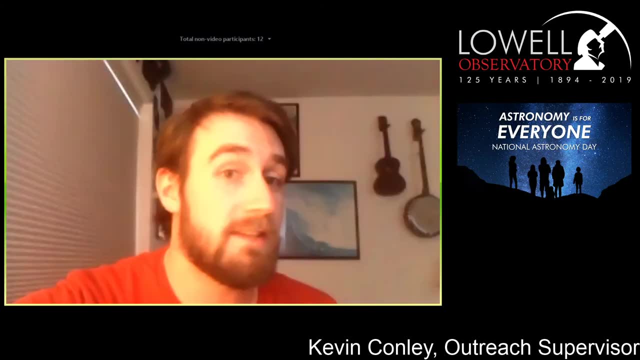 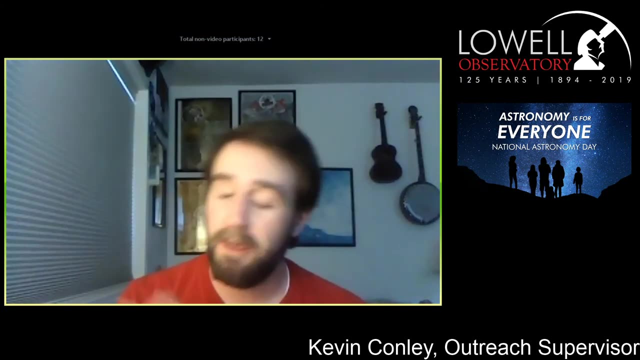 You can have them try to replicate the part of the night sky, that's of you, the constellation they like the most. or you can have them try and develop their own constellations, just like people use these stars to tell their own stories back in the day. 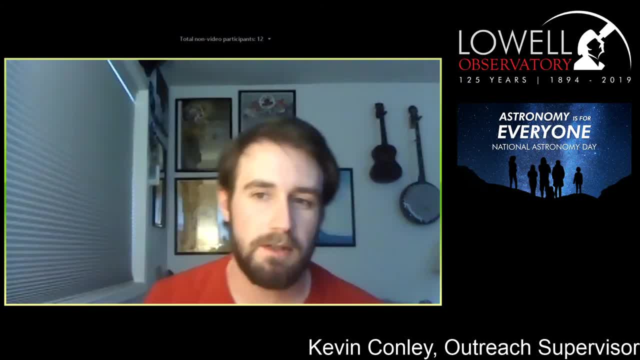 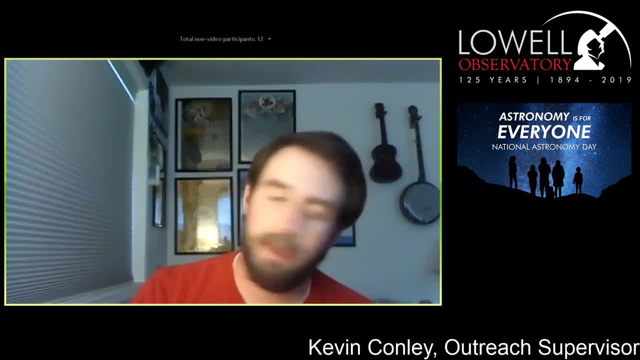 But we're not doneyet. But suddenly I'm going to show you how it looks when you put the� off of the wall. I'll bepants me back on and show you what we'll try. You'll want to pick right below the middle of that wall over here. 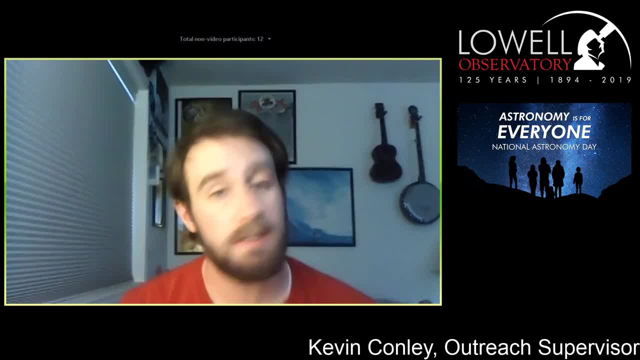 You can see the stars. These are付, which means remember these guys. they are blue, So these are the electrons. You can also see aściellulose addresses and stripes. You can see them like spots. You can also see thepper lights. 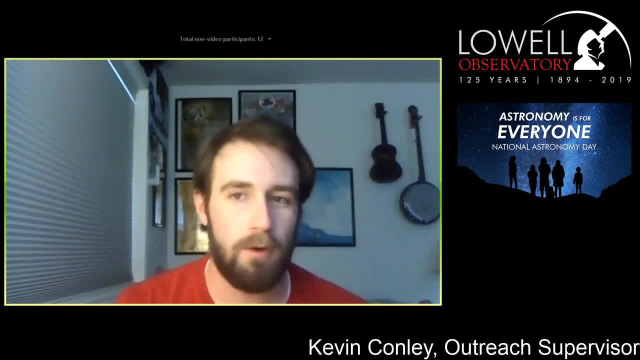 Turn thebbe ㅎㅎ, iza, especially during the quarantine here. so that's kind of brief rundown of a quick. 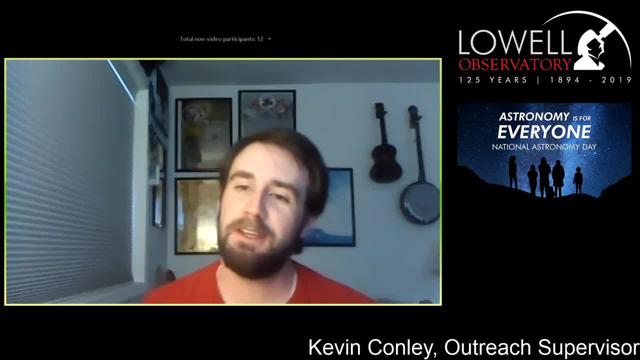 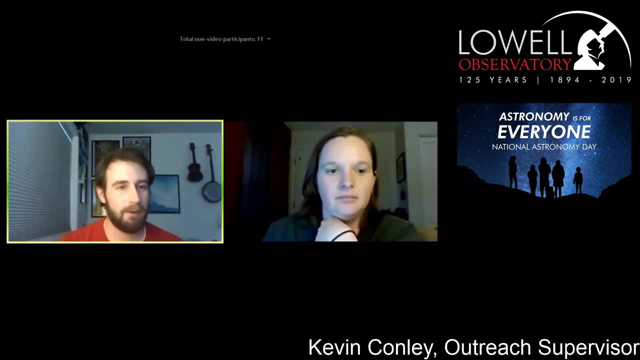 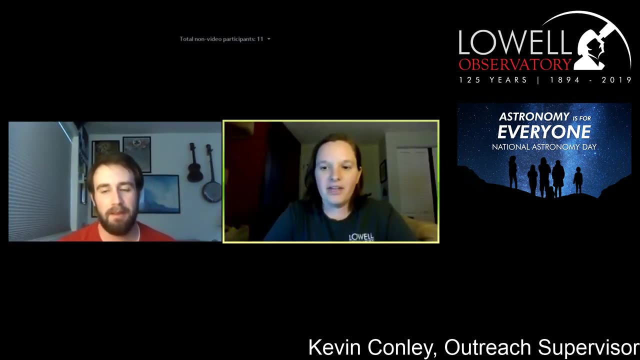 project for younger kids. there's any questions? please let me know now. any questions there? all right, all right, we'll give it another couple seconds there. Thank You, Kevin. I always think it's fun. you had to draw your own lines. you know, poke whatever holes you want and try to. 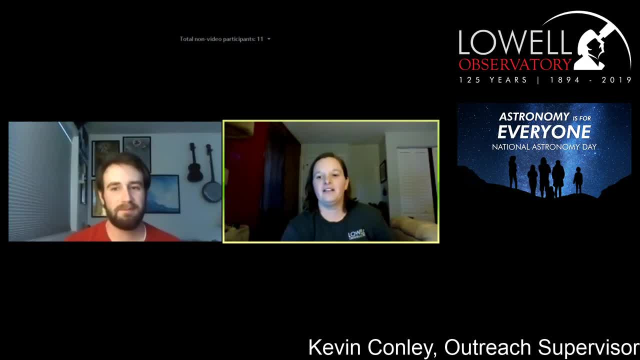 determine shapes than them. you know, I think that's that's great and that's honestly a great thing to do. even if you have nice guys- guys like in Flagstaff- if you're able to get out and enjoy the weather, you don't need to know the 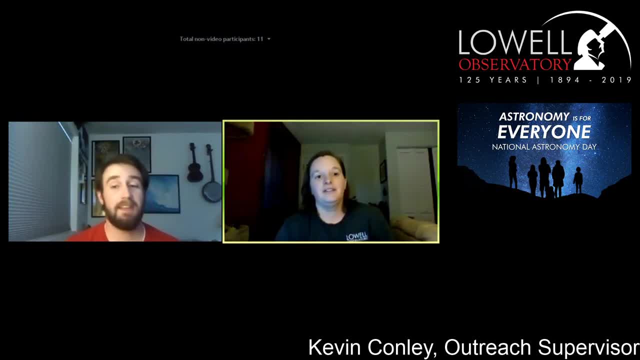 constellations to do exactly what you're talking about outside too. yeah, that's true. the question was: can he play his banjo? not sure if I'm gonna do that right now. sure, yeah, that's their time to present cool, all right. Thank You, Kevin. all right, so um on. 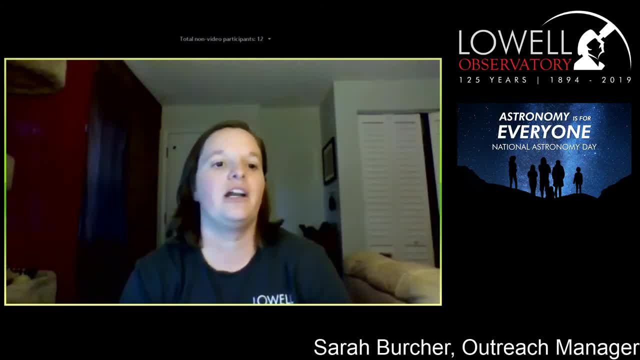 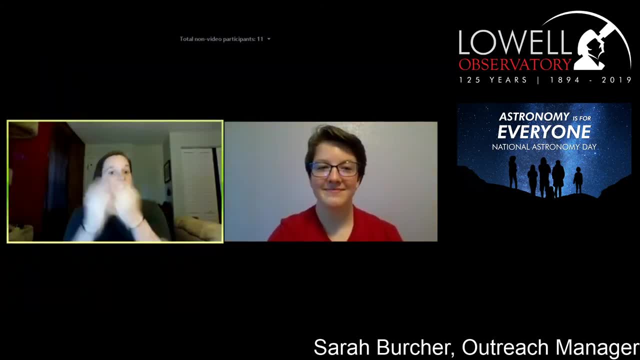 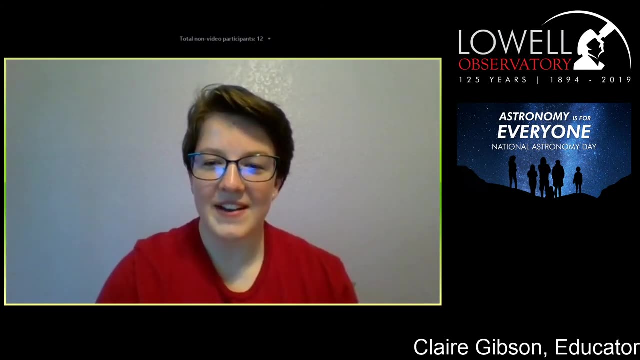 the the subject of kind of kids getting into astronomy. I want to introduce next Claire Gibson, one of our educators, and she's going to tell you about how she, as a kid, got started in astronomy. so click on how to take it away. that is well, my name is Claire Gibson and I'm just going to tell you guys. 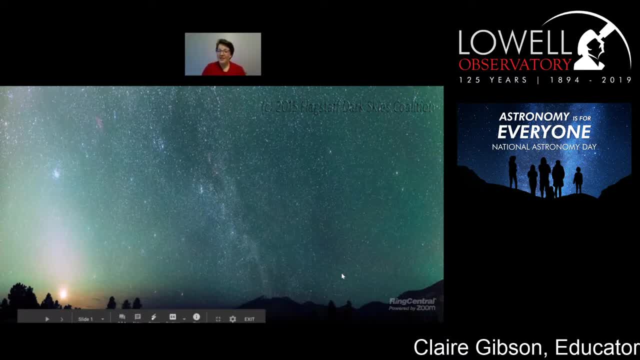 about how I came to strong. so spoiler, spoiler alert, it was a bit of an accident, but, like Kevin before me, I have grown up in Flagstaff for basically my entire life, so I've had access to beautiful night skies and the Milky Way basically all year round, but for a very long time the night sky was really 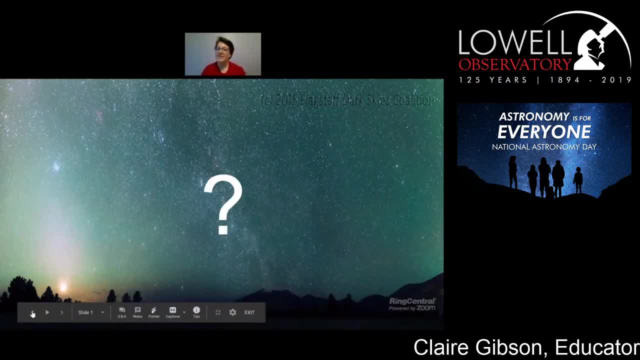 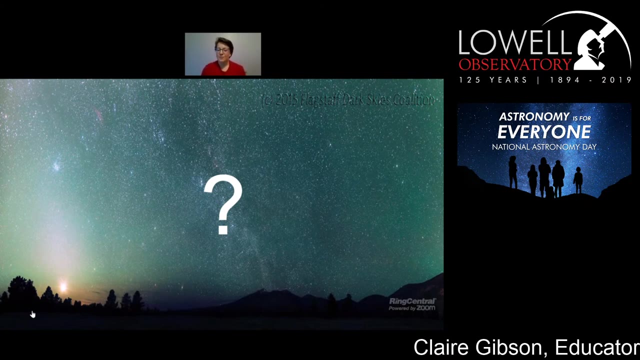 rather oops going too many, rather puzzling to me. So I didn't really know what really was, what really the universe is all about. I didn't know any constellations. I hardly knew what stars were. I definitely didn't know as much as I do now today, But my parents decided to put me into. 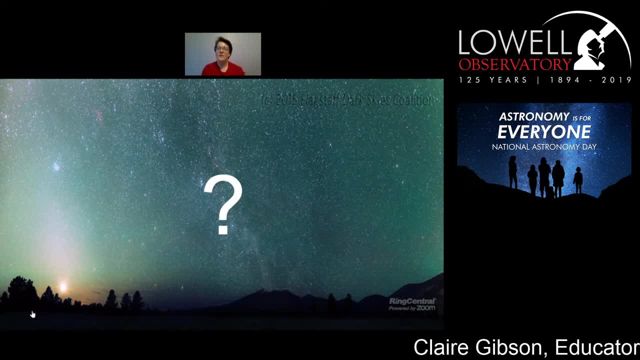 the little observatory camp for kids And that's kind of where I got my beginnings. So I went to this camp as a seventh grader And when I started this camp I was very unsure about it because I didn't want to spend my summer learning about science stuff. I just got off from school. 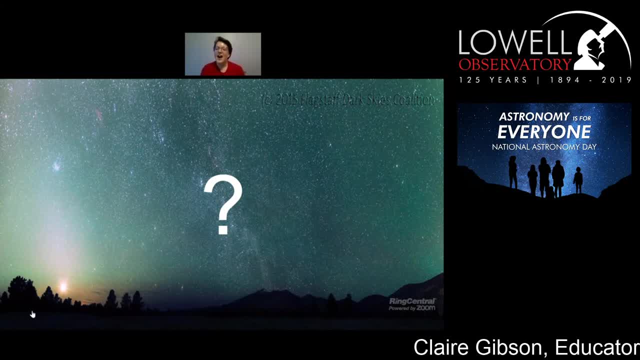 and kind of just wanted to relax like any other kid in seventh grade. But I remember the first day when I was there the camp counselors asked me to come up with a constellation name for myself to write on my little name tag. And I didn't know any constellations And so I got really nervous. 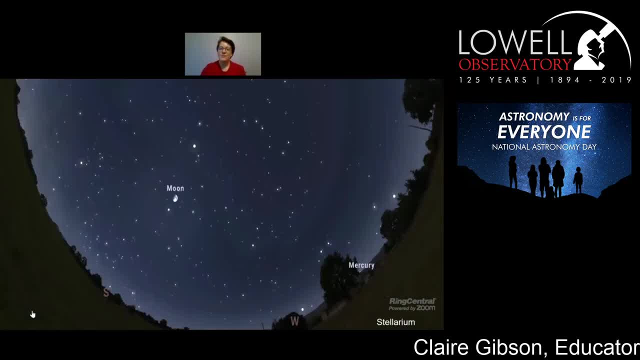 I was like, oh, what have I done gotten myself into? So on the first night I was there, this is kind of what the sky looked like to me: Nothing too interesting, certainly didn't know any constellations or anything like that It. 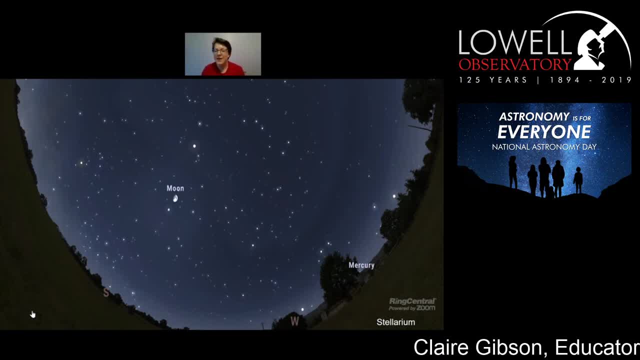 was kind of just like the regular old sky that I had known for basically my entire life. But then one of the camp counselors whipped out one of the really cool green lasers that you can point out at the night sky and my seventh grade mind was blown by that. It looked like they were touching the 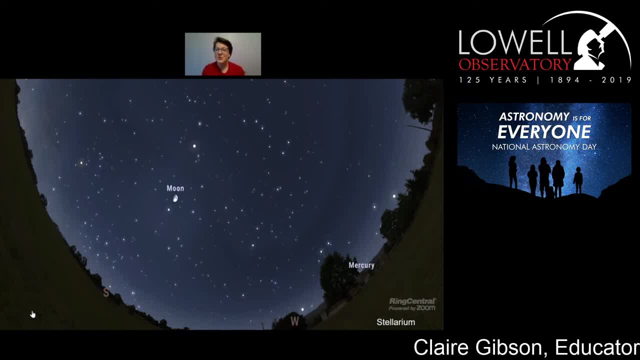 stars, and I started to pay more attention to what they were saying, to what they were saying about the night sky and all of the treasures that it holds. So I started to learn about the constellations, I learned about what planets were up. I even learned how to use a very small 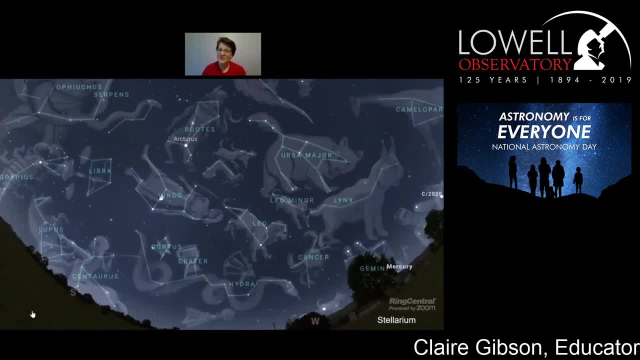 telescope while I was there And at the end of the week, this is what the sky looked like to me. The sky is full of stories, it is full of history and, most importantly, it is full of culture and many, many things to learn. 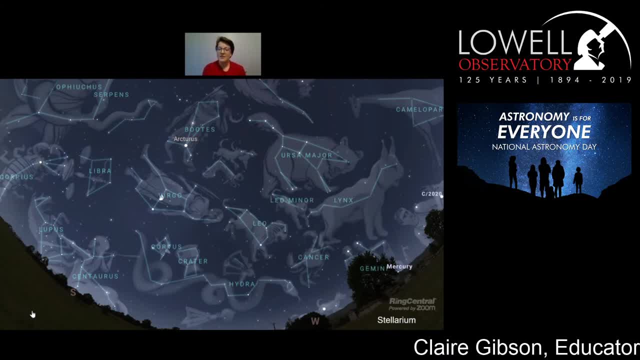 So I now had a basic knowledge of some of the stuff in the night sky. There's still certainly much more to learn. so, basically, what I needed to get me started, even after having such beautiful dark skies, my entire life was a guide. I needed someone to tell me what things were I needed. 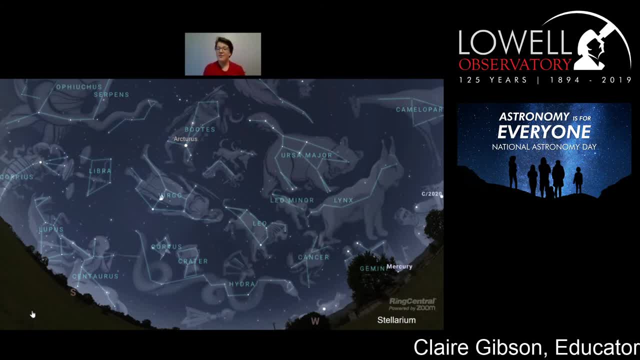 a teacher, basically. So that's what I do now. today I'm an educator at Lowell and I teach people about the night sky And a lot of times people ask me: oh, what's your favorite constellation? And I tell them: oh, that's a great story. It actually happened here at Lowell Observatory, where I found that. 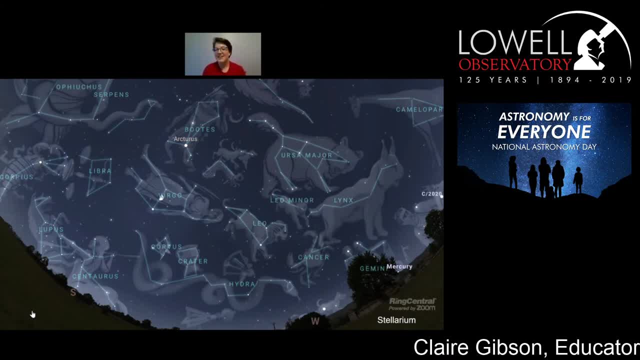 back in 6th grade. So, in case you're wondering, my favorite constellation is Corona Borealis, mainly because it is one of the only constellations that actually looks like what it's supposed to be. The Corona Borealis is actually this little constellation right here. Corona Borealis means 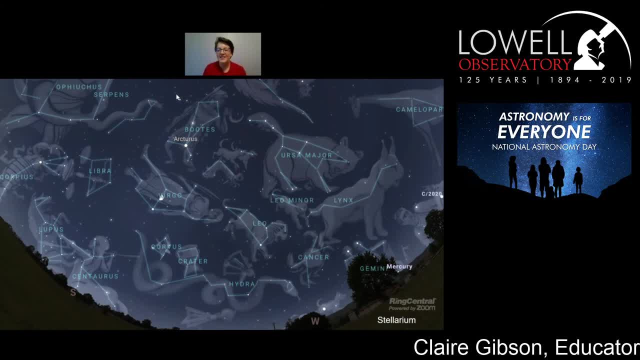 the northern crown, So it kind of looks like a little crown in the night sky and I thought it was very beautiful And that ended up being my constellation name back in 7th grade. So that's kind of a cute story. But I'd like to kind of end when people ask me: oh, what do you? 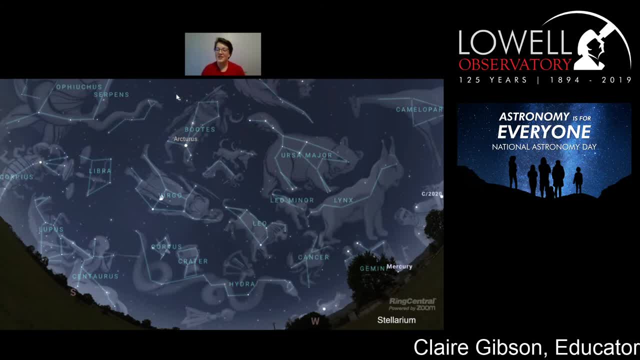 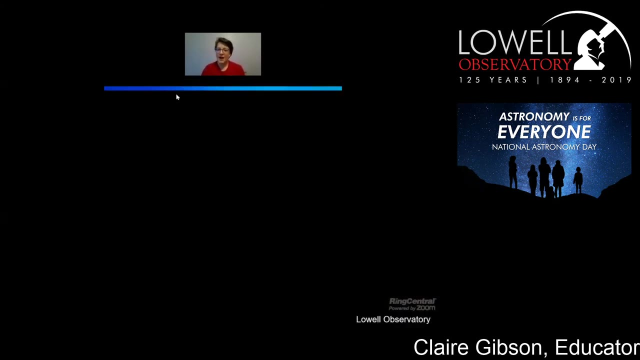 use to get into astronomy. I don't have a degree of my own right now. I'm currently in the process of starting to get one. People always ask me: oh, what do you do to learn about the universe, especially when you don't have access to it at school? And I'd like to leave you guys with a. 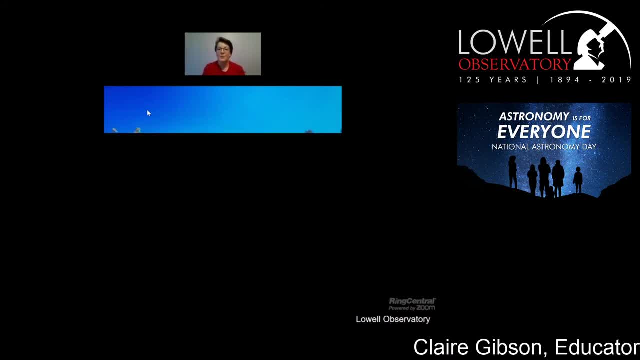 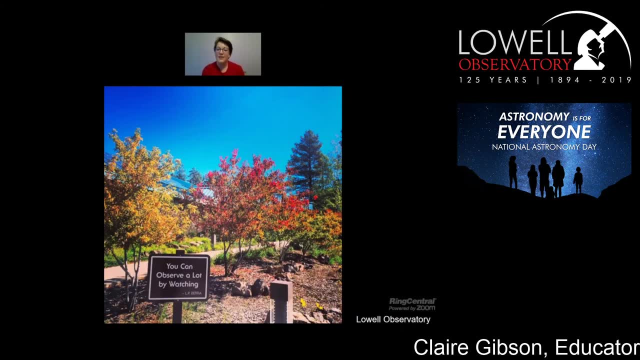 quote that I see almost every day walking up to work. This picture will load, hopefully, But there's a little sign as you walk up to the Visitor Center of Wolves Laboratory that says you can observe a lot by watching. And I tell people you don't need a fancy telescope. 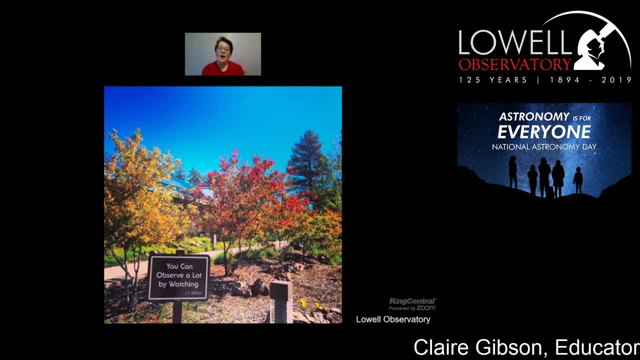 You don't need a great high school teacher even And really all you need are your own eyes or really anything. You can observe a lot by watching, So I tell people you can learn so much just by watching the night sky, as the ancient people did many thousands of years ago. 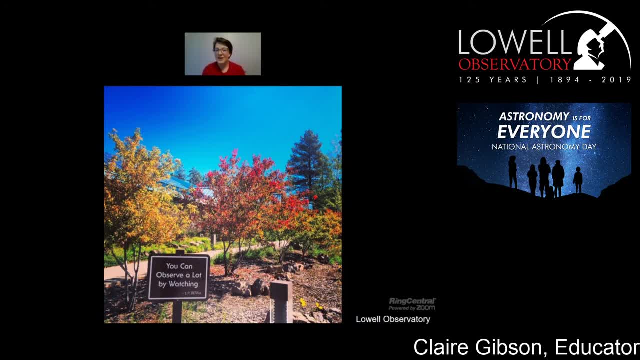 So that's kind of how I got into astronomy. I'd be happy to share my story with you guys. I'd be happy to answer any questions and give you guys some pointers if you have any of those questions for me. But for now I'll leave it to Sarah. 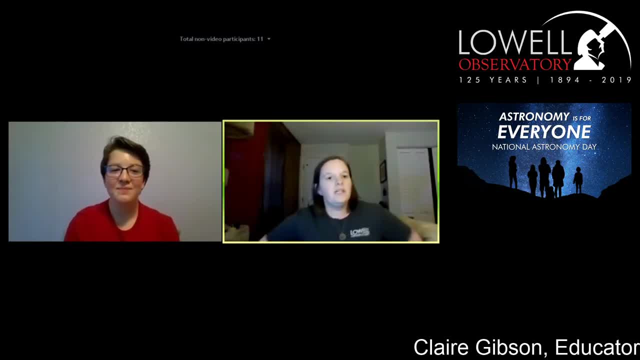 All right. Thank you, Cliff. How many years were you in LOCKSS? I was only in LOCKSS for one year. I only went for those five days. So I learned about all of the constellations And let me tell you, after that I begged my parents to let me go to the. 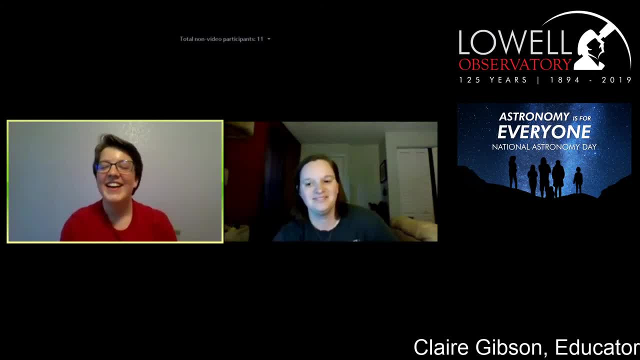 university And I was like, okay, I'm going to go to the university. And I was like, oh, we got to go back. And somebody asked me: how did I get this job? So this is a great question. I got this job really because I started as a volunteer here. So when you're the legal working, 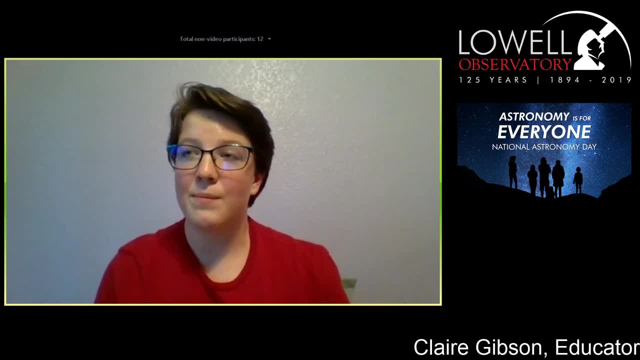 page, which is 16 for us, you can apply to have a volunteer position. So it's not paid, obviously, but you can still do some pretty amazing things, And my job basically every night was to tell people about the constellations. So that's how I started And eventually once an educator. 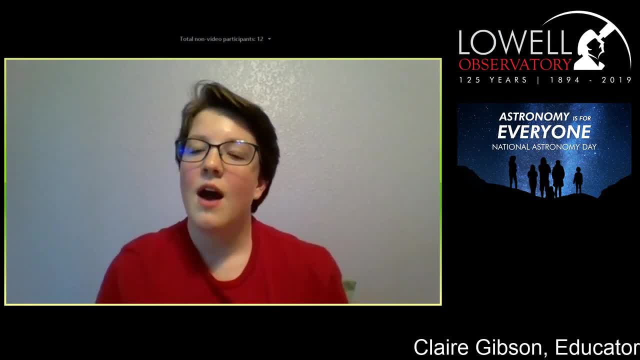 position opened up. they usually do seasonal hiring. I applied for that position and did the whole process. I had to go through an interview still, but that's how I retired here. Got another question from Laura Nealon: Do you have a favorite memory or event from Roll Observatory? 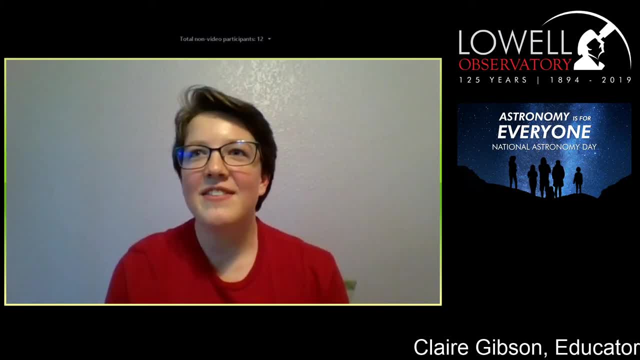 Yes, there are many. One of my favorite events was probably the 50th anniversary of the Apollo 11 moon landing. that happened just this past summer And let me tell you, Roll Observatory was so incredibly busy, but the energy there was just amazing to be around. 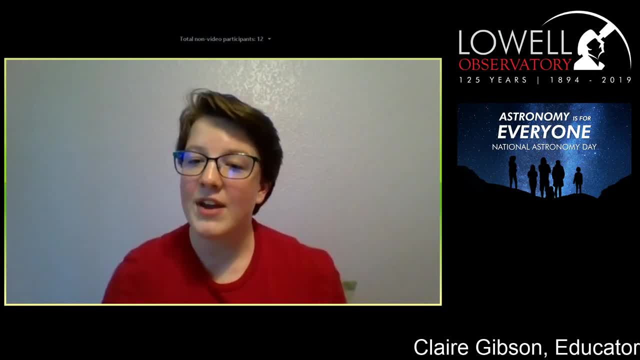 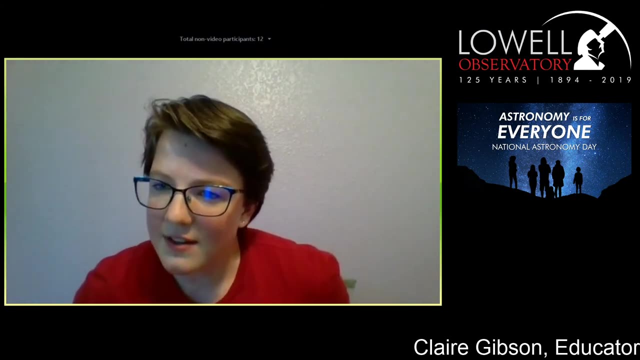 Everyone was so excited about sharing and remembering such a great feat in history and for science overall And just being around that energy being able to facilitate and give people more information about that is so amazing. It looks like I skipped one of the questions. Summer Brown, My daughter, is 12, finishing seventh grade and getting into astronomy. 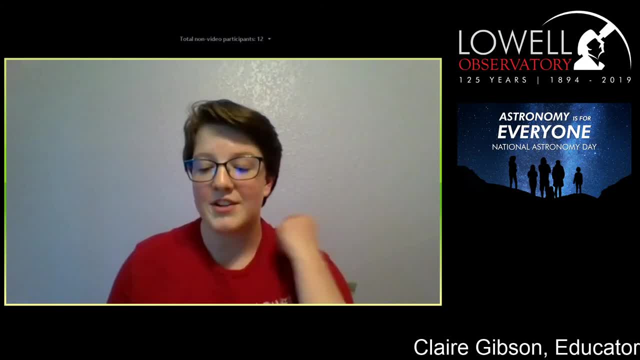 What is your biggest word of advice to her? That's a great question. So one of my main things for her is to try, just try to get involved as much as you can with whatever you have available with you. So a lot of the things that I did was that I read a lot of books. I subscribed to some. 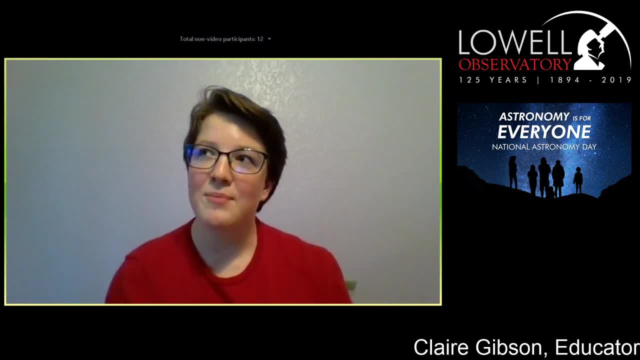 astronomy magazines, and I tried to just take up as much information as I could on my own, So I didn't have to go anywhere. I didn't have to go to a fancy to do this. I did it at my own pace in my own house, which is a good way to do it. 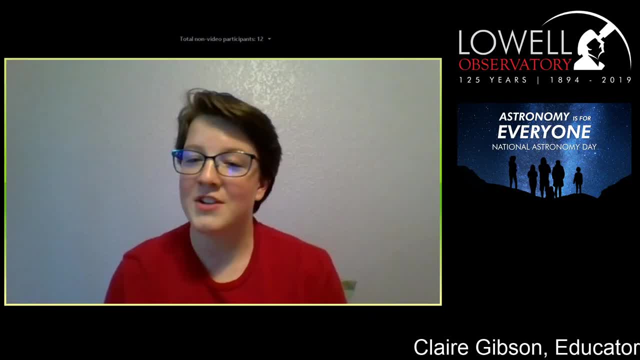 You don't want to rush so much all at once, because there's so much to learn about the universe And if you take your time, that's the best way to do it. So there's so many great things out there. Got another question. 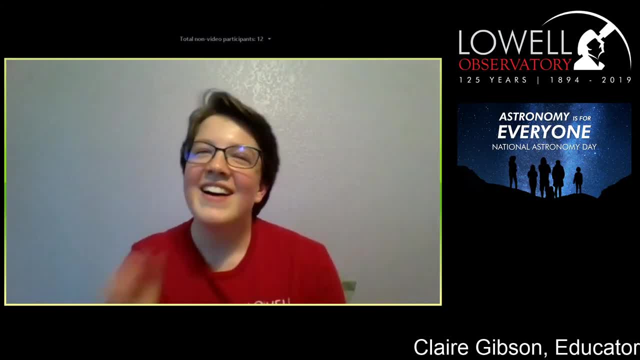 What is the strangest thing you have seen in the sky? Good question, I haven't really had too many strange things that I've seen in the sky. I can tell you one of my favorite things. I guess one of the one of the strangest funny things is the first time I looked at Jupiter, over a couple successive. 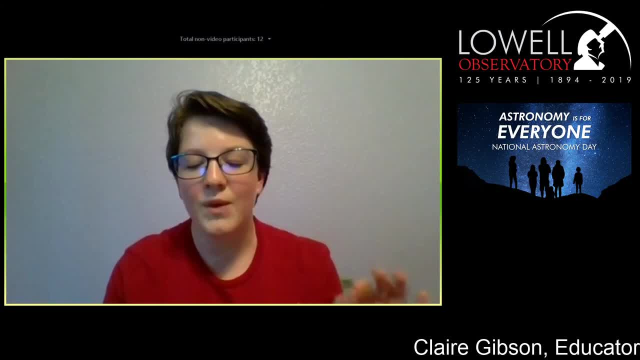 nights I could see the four Galilean moons and they're just kind of what looks like four little stars line around Jupiter. And when I looked at it the next night the Moon's had moved and that was like weird to me for some reason. I don't know why that was weird to me, But it makes a lot of sense now because that's how moons work around the. 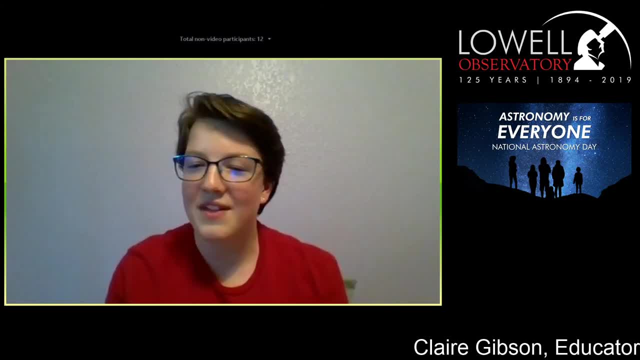 planet, But to my little seventh grader mind it was not a very good start. rather weird to me. so I guess that's one of them. Another question is: where do you look at the stars? So since I live here in Flagstaff, I've had the great opportunity to just have some beautiful. 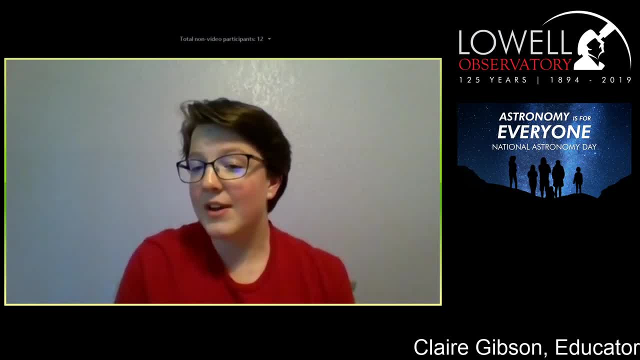 night sky. to be able to do that, A lot of my job involves looking at the night sky as well, but there's some great resources online as well, such as delirium, where you can have the night sky on your computer so you can actually plug in the time and your location. you can have the stars. 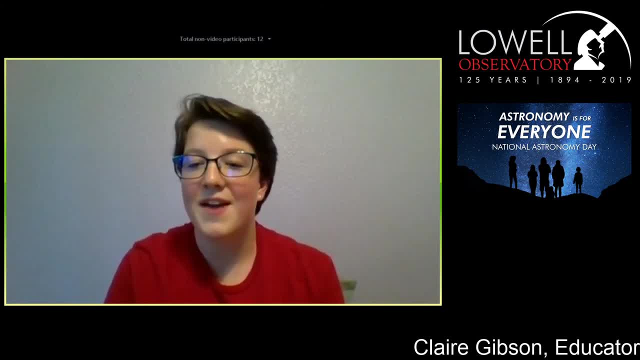 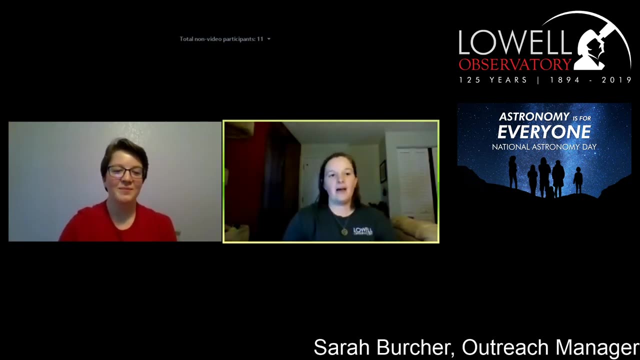 right there in front of you if it's a cloudy day or anything like that. but if there's any other questions, I'd be happy to answer. All right, thank you very much, Claire, appreciate it. Okay, so next up we have one of our astronomers, Dr Gerard Van Bell. You've heard from Michael. 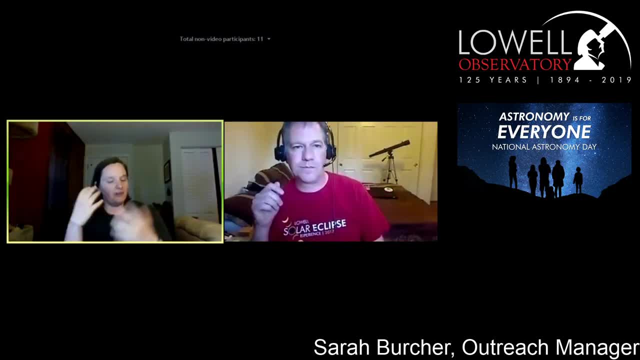 you've heard from Deidre about how to become an astronomer and some other options there. Gerard's going to tell you, once you get there, what happens. What does a day in the life of an astronomer look like? So, Gerard, take it away. Thanks, Sarah, and 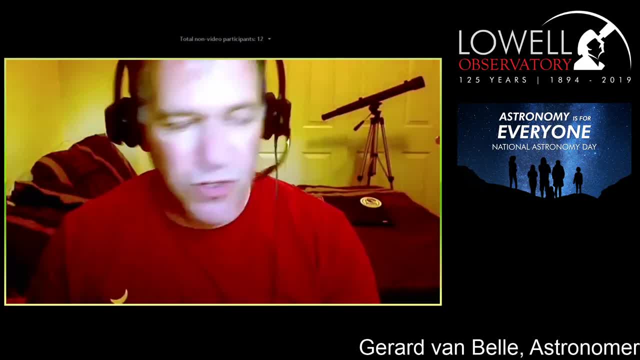 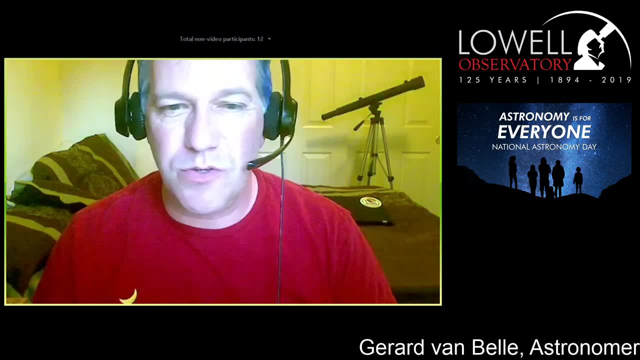 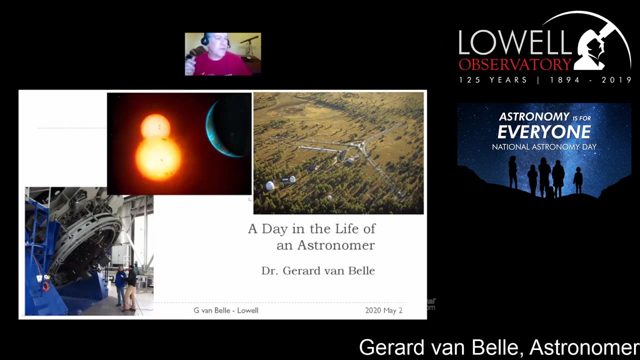 I have to tell you, you know, working as an astronomer, I get this question from time to time and it is really truly one of the hardest questions to answer. It is so incredibly hard to try and answer what the heck I do every day, and part of it is because it's a lot of fun to 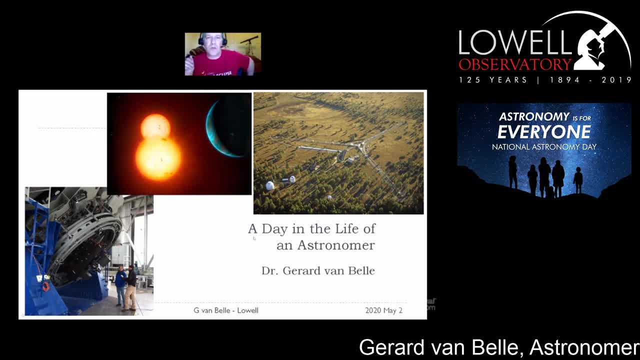 to do all the things that I do. One of the things that I really value about being an astronomer is that I'm doing something that I really enjoy. It's a lot of fun and, at the same time, I'm also doing something that gives me a lot. 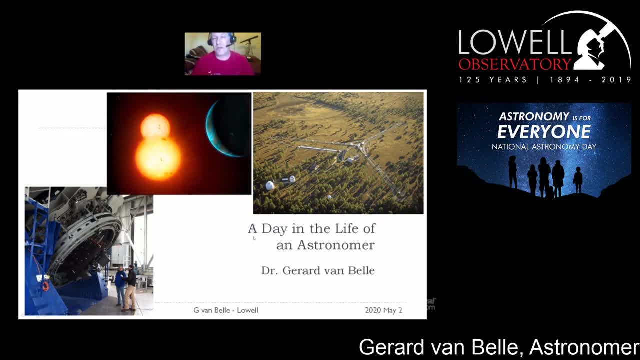 of autonomy. I can do a lot of things that I'm doing because I'm just interested by them and I'm motivated by them. There's very. there are certainly a number of things that I have over the course of every single day where you know you kind of have to do them. you know you have to fill out certain. 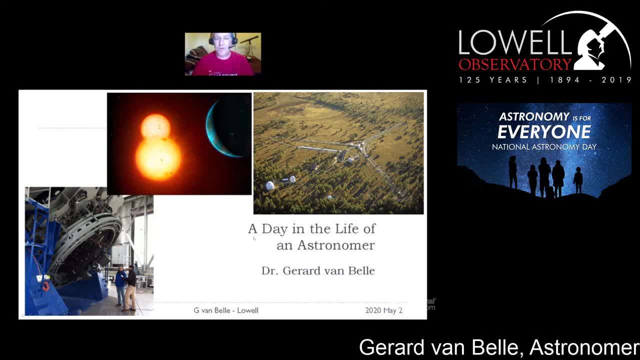 paperwork and that kind of thing. like any job With a degree in astronomy and working in astronomy, you get a lot of freedom to pursue the sort of things that interest you. so one of the things that I've worked on for a long time is kind of specialized relative to what a lot of astronomers do, which is I do work on instrumentation. 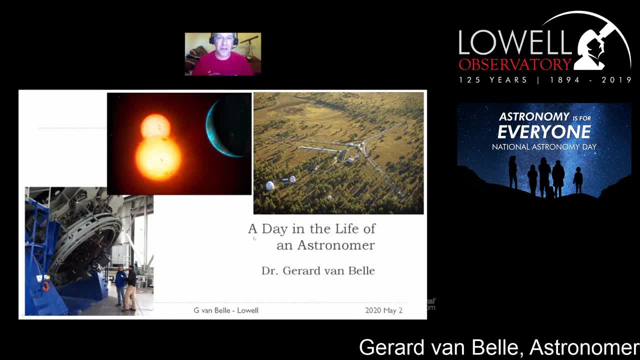 so I'm kind of a a rogue engineer, actually, of sorts, where I do a lot of work on the tools that we use in astronomy, so let me show you some of these things. So I'm going to show you one of these things that I do get to work on on a day-by-day basis. 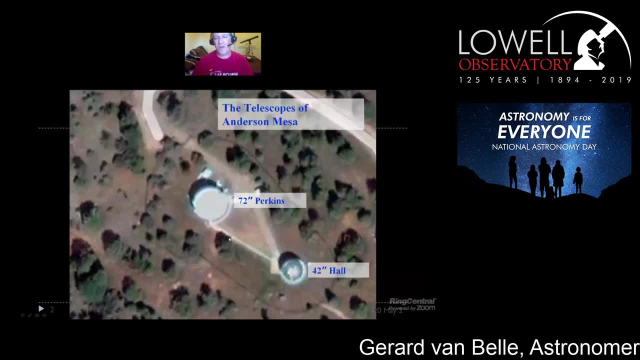 With the observatory. we work with telescopes, and the Lowell observatory actually has a large number of telescopes we have at our disposal to work on. In fact, we have one that was built a very long time ago, the 72-inch Perkins telescope I'm showing right here. 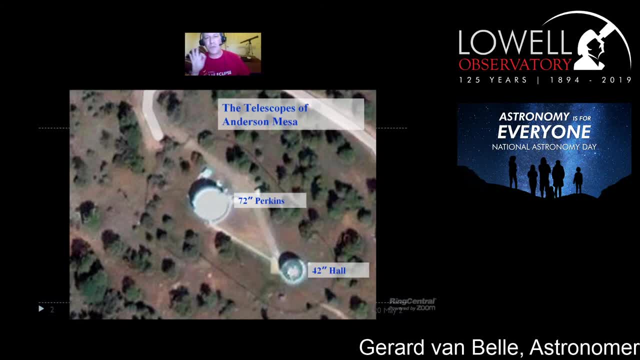 This telescope, when it was first built in the 20s, was the third largest telescope in the entire world, was actually not at Lowell at the time. It was out in Delaware, Ohio, and it spent its first 40 years of life there before somebody looked out the window and realized the weather's not very good. 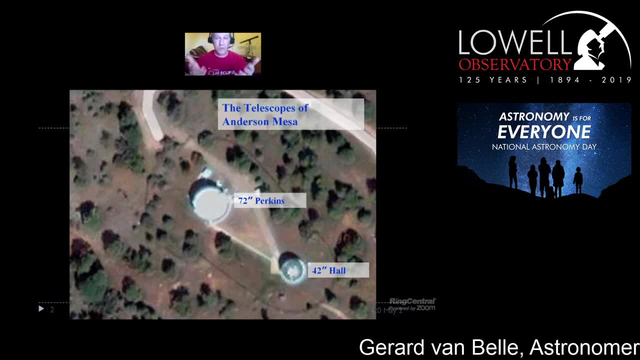 in Delaware, Ohio, And so it got moved to Anderson Mesa, a place that's just outside of town here, And we've had it as part of the Lowell Observatory ever since the early 60s, We also have the 42-inch Hall Telescope, And one of the things that's important about a telescope- 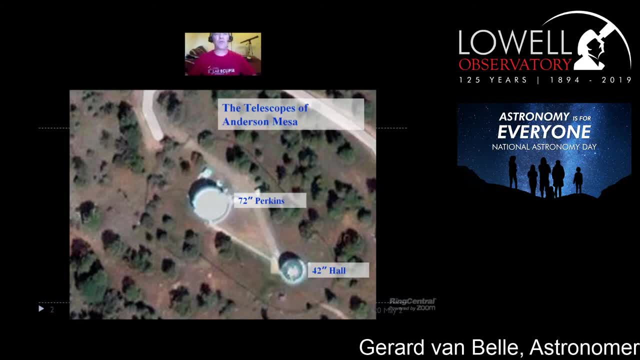 is that when a telescope gets physically larger, you get a better and better ability to pick out fine detail in the sky, And so the 72-inch was quite valuable at its time, And they were able to do a lot of research with that as being a large telescope being able to pick out detail. 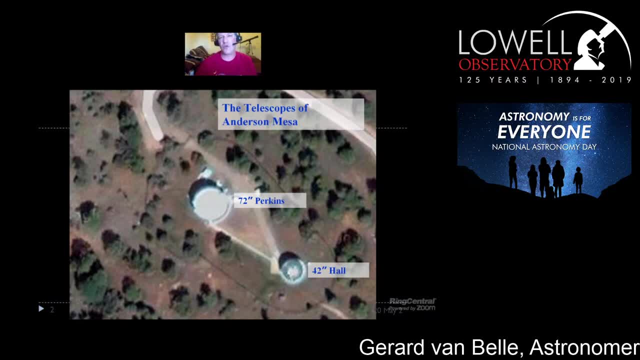 And nowadays the 72-inch has gone from Lowell to Boston University and they are continuing in their partnership with us in using that telescope. So the 72-inch Perkins is continuing its life up on Anderson Mesa. But next to the 72-inch Perkins and the 42-inch Hall is something called the Navy Precision Optical. 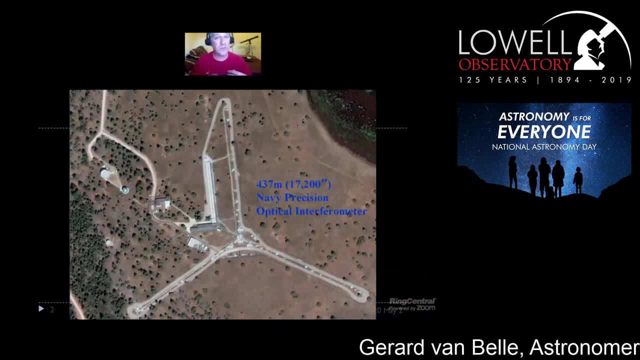 Interferometer. This is a facility that Lowell is one of the partners in developing and running and using scientifically, And it is about the size of four football fields from tip to tip. You can actually see this Y-shaped sort of array here And it is actually so large it's easily seen in these Google Earth photos And it is able to take. 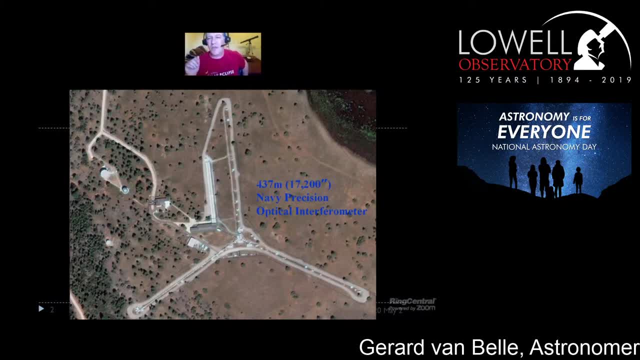 pictures of exquisite detail because of the fact that it's physically so large. As I believe Kevin mentioned a couple of segments ago, stars can be used for navigation. That's one of the reasons why the Navy is interested in having observatories and runs the US Naval Observatory and the Naval 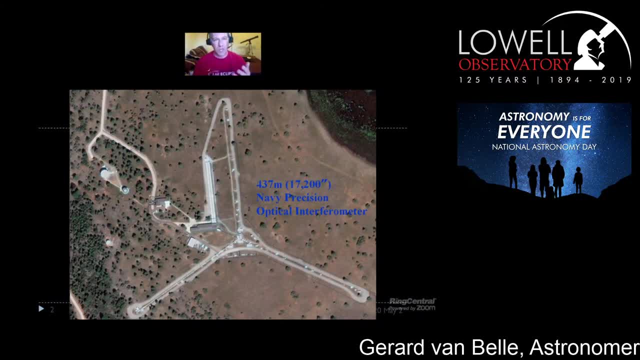 Research Lab. There are two partners. There's a running Envoy. The Lowell Observatory, though, uses Envoy because we want to look at stars and be able to image actually the surfaces of stars and see spots on those surfaces and do that kind of. 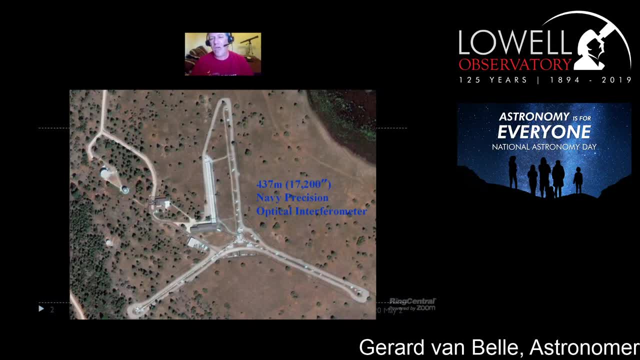 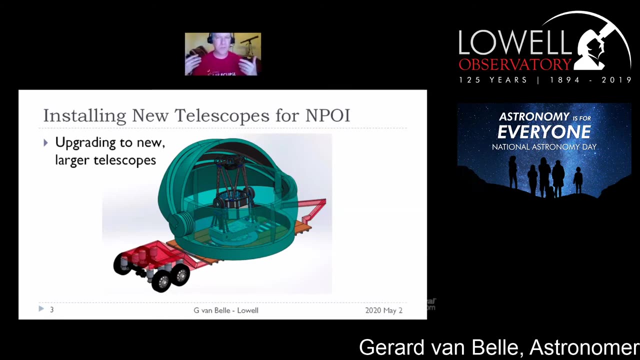 thing And we have the facility operational, but we're in the process of trying to get it more operational and trying to get it operational with upgrades. So that's one of the things that I'm involved in, which is looking at how to get big telescopes put out and feeding the array. So this is a 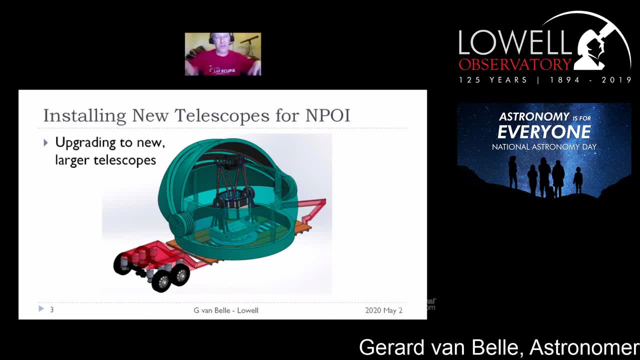 very special facility. It's a very special kind of telescope. It is made up of individual telescopes that are linked together, And by so doing you actually synthesize this very, very much larger telescope, And so we've gone from designing these telescopes. 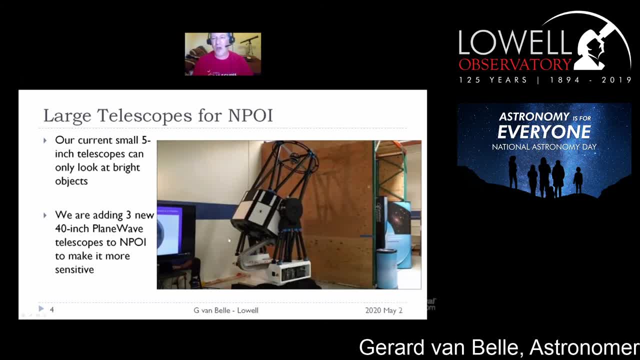 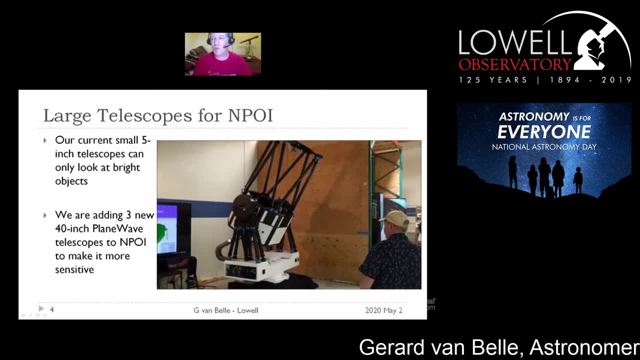 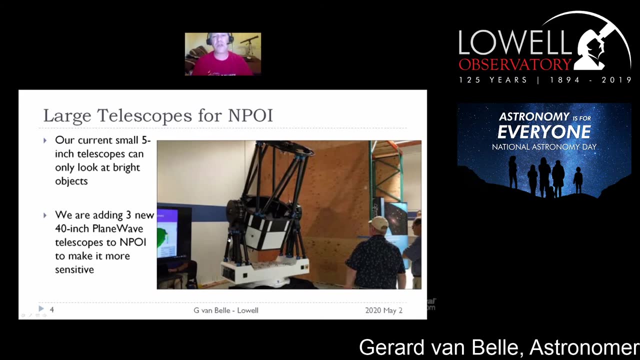 something that I've been involved in- to actually now taking receipt of some of these telescopes. Here is an illustration of one of the telescopes that has come out to the site. These are 1-meter 40-inch plane wave telescopes, and we're in the process of integrating them into the system, so it's very exciting to see an idea like this start. 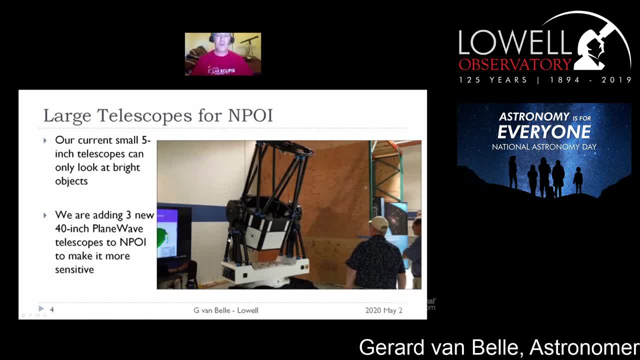 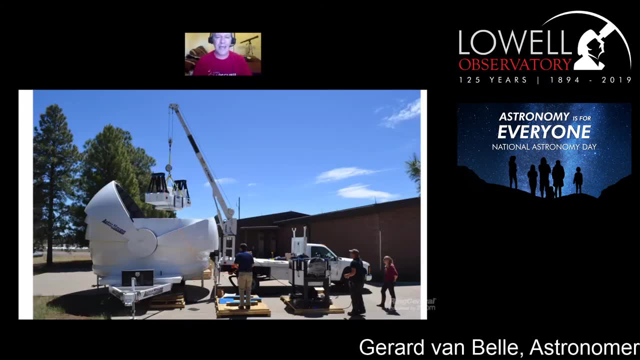 from a spark in your head to actual designs and specifications and purchase orders and delivery out to the site, And so a day in the life of an astronomer like myself can actually span a very interesting and very wide range of going from things like design work all the way to. 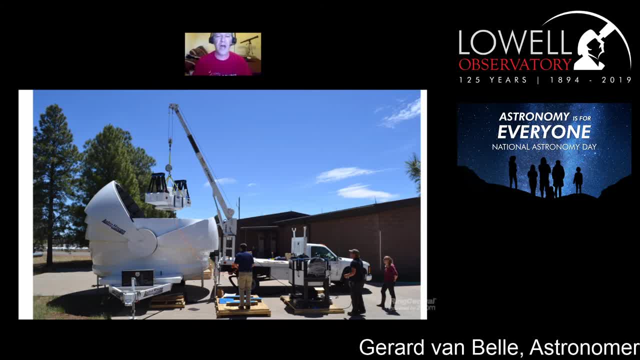 driving a forklift or, you know, flying large telescope parts in through a dome on a crane. it's, you know, part scientists, but also part mechanical engineer and part civil engineer and part longshoremen. you know it's a very exciting work from time to time. so this was one of our one meter telescopes. 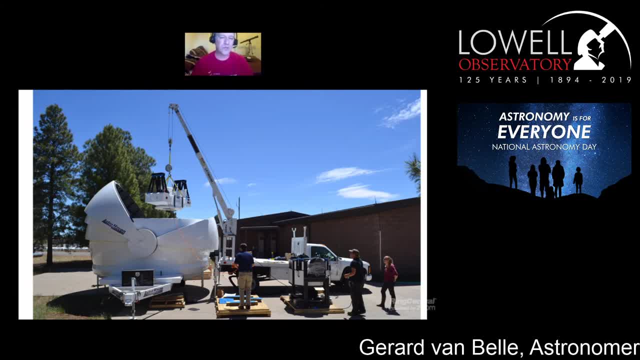 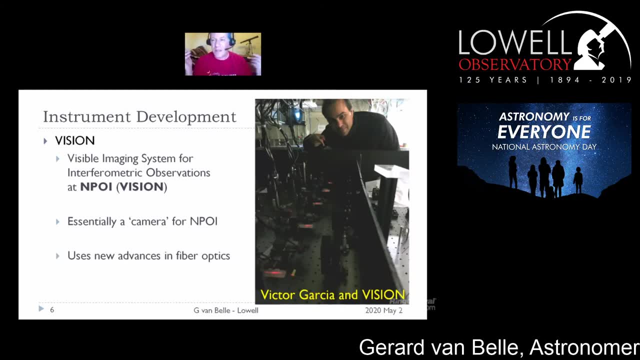 being delivered a couple years ago out of the site as we put them into the telescope dome you can see here and getting integrated into the array inside the buildings that are at the center of the site. we also have the various cameras that are being put together that take pictures. these are very, very. 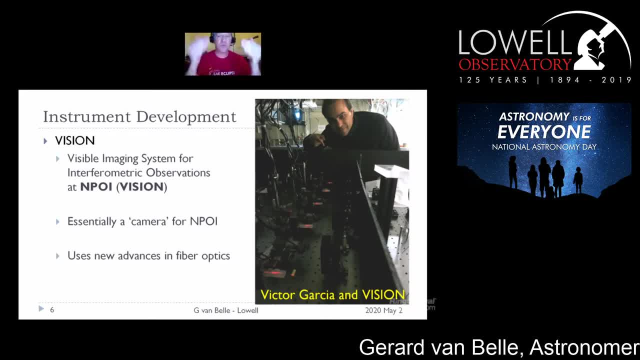 specialized, because they're taking feeds from multiple telescopes at once and then synthesizing everything together to make an image. everything has to be aligned to on the order of about 20 nanometers- that's maybe two to five hundred times the size of the telescope dome- and then we're going to be able to. 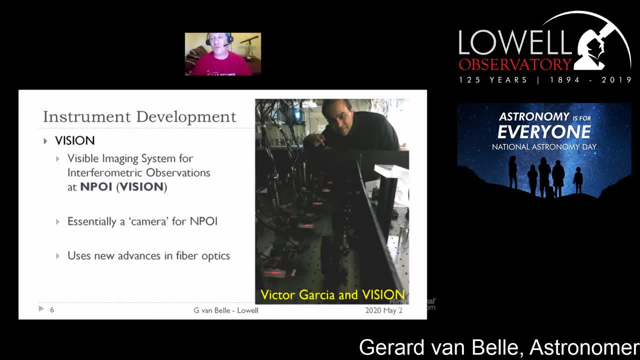 take a picture of the diameter of an atom, so we do a very good job of lining things up. my colleague, Victor Garcia, is shown in this picture here, and you can see the red laser light of the various feeds that are being fed into this camera. we call vision. there's a lot of terrible acronyms in astronomy, and so 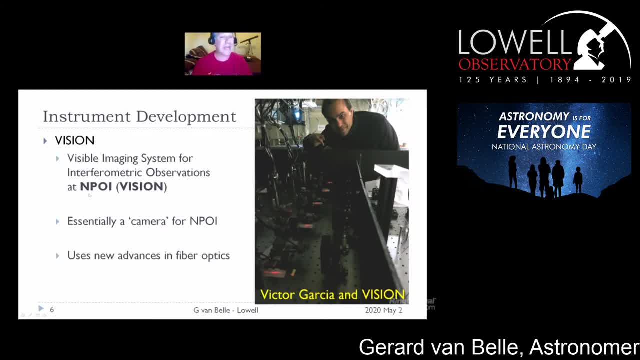 this is one of them: the visible imaging system for interferometric observations at endpoint, and so, yeah, we basically take advantage of new technology that's coming out and we're going to be able to take advantage of that technology and try and get to better and better instrumentation by adopting that. 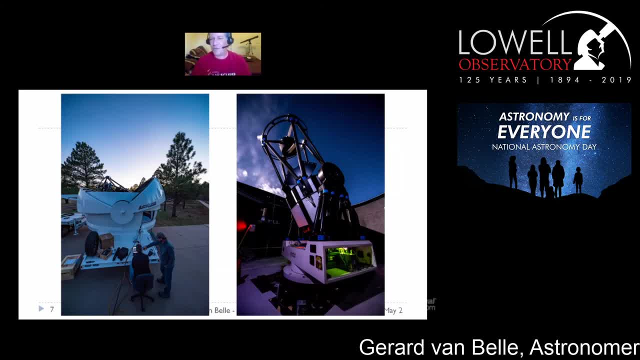 technology. so here's actually a nice view of these telescopes getting put into action on the sky. so in addition to design work and the the implementation and crane work and that kind of thing, you also get to stay up at night and run these incredible machines to try and catch new glimpses of things in the sky. 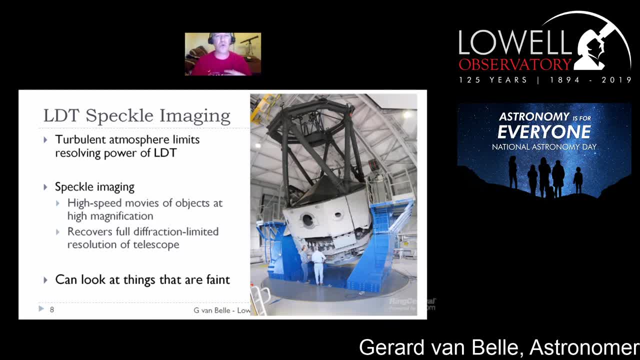 one of the big things that is happening here is that there's a huge amount of space in the sky and there's a large amount of energy that's being spent on telescopes. that is more of. a conventional telescope that we have at the Lowell Observatory is the Lowell Discovery Telescope, the LDT, And we use that telescope to do science as well. This 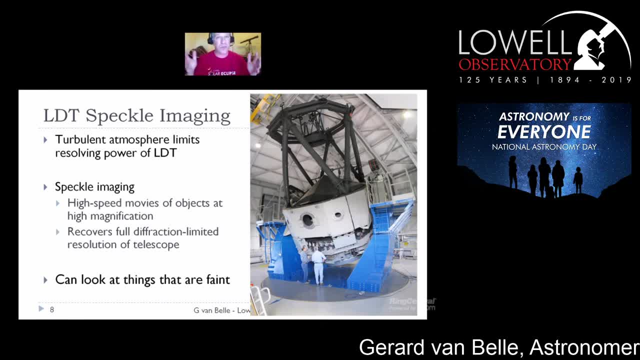 is a telescope that has a primary mirror. That's what really defines the performance of an optical system. That is 4.3 meters in size, That's about 180 inches across. You can see my colleagues standing right here taking a look at this, And the mirror is hidden inside of this cover right now. 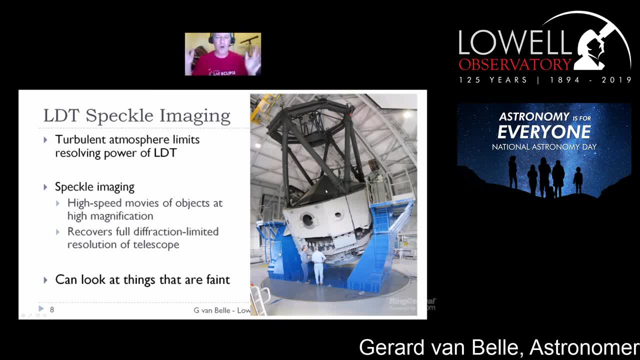 because it's the middle of the daytime in this photograph And these covers flop open and you're able to look onto the sky and see things in very, very high detail, And so one of the things that I like to think about in my job as an astronomer that builds a lot of instrumentation, I think. 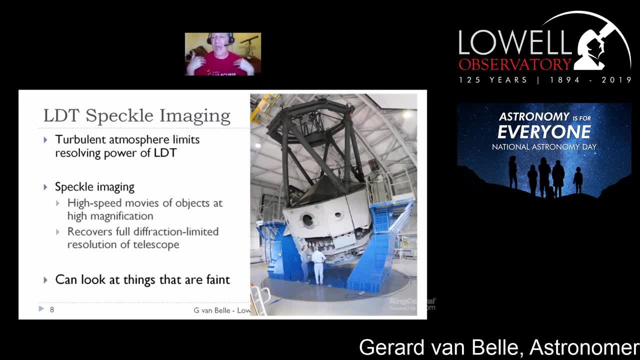 about this a lot on a day-to-day basis is: how do we actually get the full amount of resolution of detail on the sky from the sort of telescopes that we have And how do we maximize that? So one of the problems that we have is when you look at something at very high magnification through the 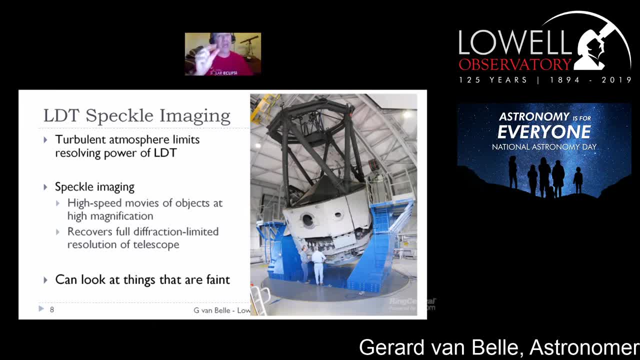 atmosphere. it's a lot like looking at a coin that's at the bottom of a swimming pool And you can see that coin kind of dancing around and smearing out, especially if somebody's just jumped in the water and the water is very turbulent. The air that we stare throughout into the sky is a lot. 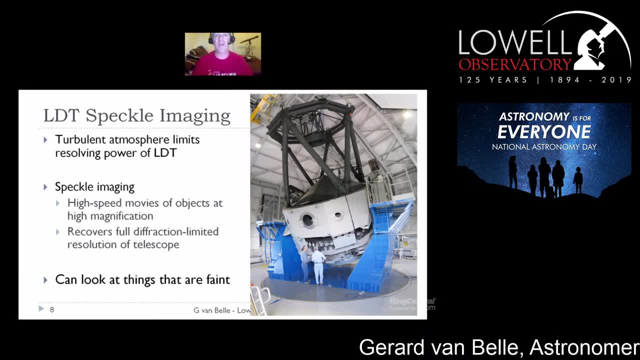 like that- And that's why stars twinkle- is that the air is this boiling turbulent medium that's kind of always shifting and moving around it at pretty fast speeds, you know, 10 to 100 times a second. the atmosphere is kind of blobbing around, And so there are tricks that we can do to try and get. 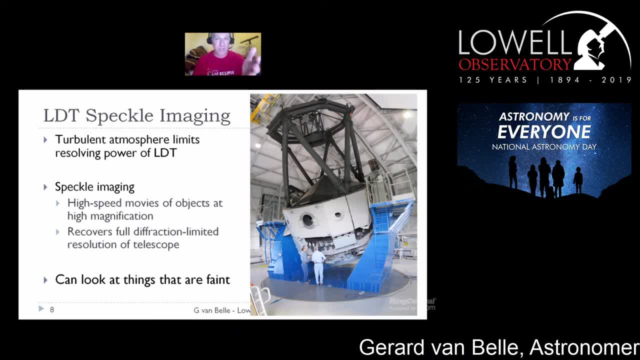 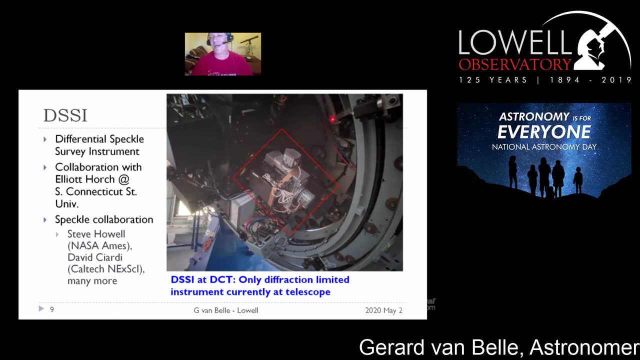 around that. So this is something that I've been doing at this telescope, at the Lowell Discovery Telescope is trying to figure out how to get all of that resolution, even though the atmosphere is trying to smear it out. So I'm working on something called a speckle camera When light comes. 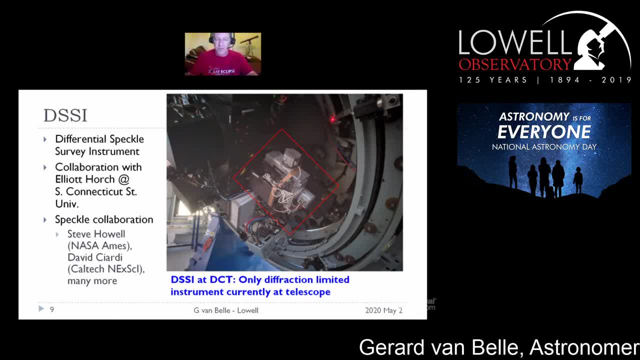 through the atmosphere and it gets smeared out. it forms these bits in your picture that are little blobs of light. We call those speckles, And so this is a camera that we use on the back of the Lowell Discovery Telescope. here in red, There are multiple cameras on the back end, So this is one of five. 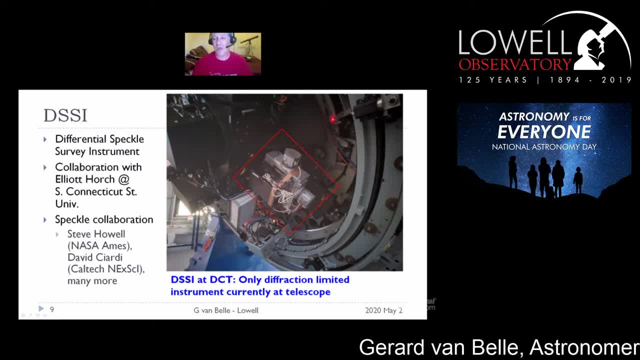 that we have simultaneously attached to the telescope, And it's a pretty interesting thing. It basically is able to look at very high speed. Let me show that again. At very high speed it makes a very quick movie, And so it doesn't make that smearing effect. 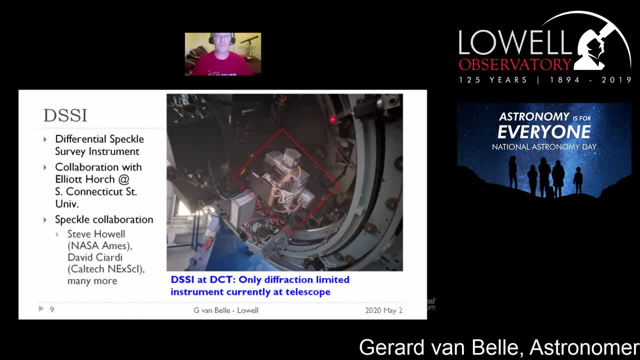 of the atmosphere go away, but it does freeze it out. And so again, if we think about the quarter at the bottom of the pool, if you were to take a very quick snapshot of that, you could at least freeze out the effect of the turbulent water. 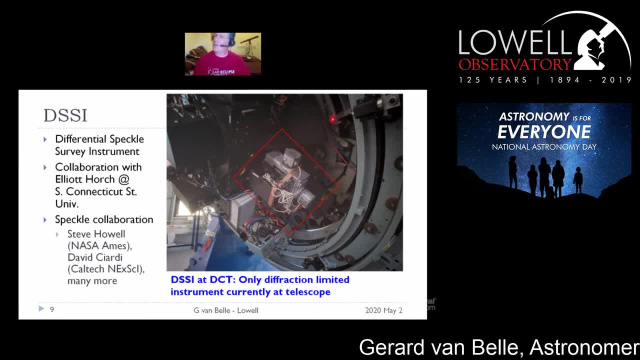 And if you did that many, many times, you could maybe tease out what exactly it is that you're looking at. If you're looking at a quarter, or is it a nickel, maybe you could tell the two apart. And so I've been in the 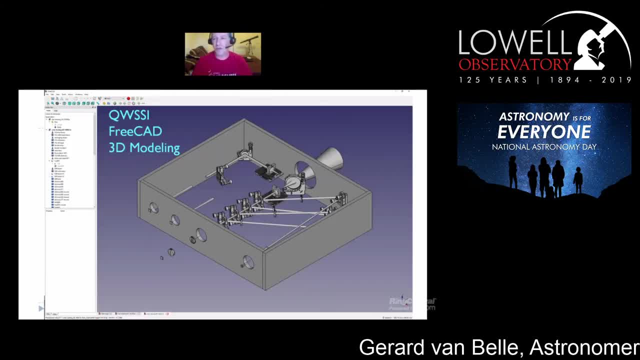 process of trying to build the next generation of this kind of instrument. We've gone from something called Dizzy to something called Quizzy, And again you start from. you know coming up with an idea in your head on literally the back of a napkin. 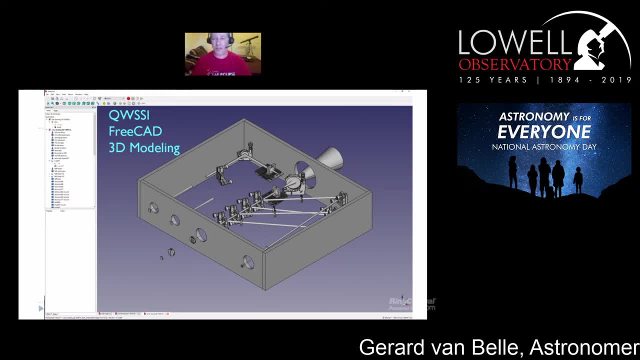 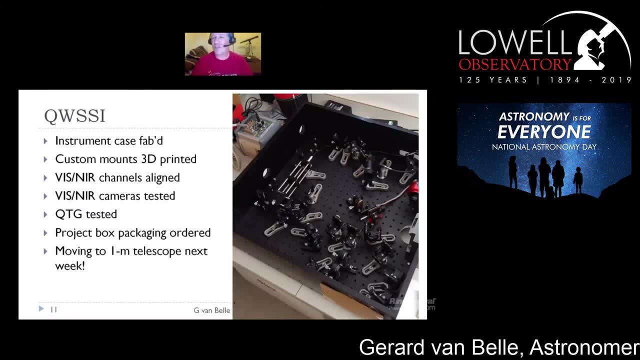 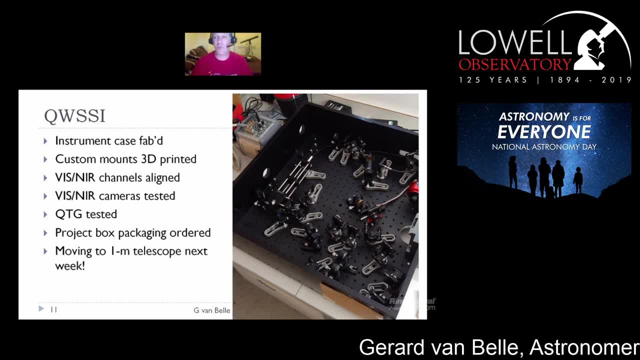 So we have a machine shop of a null that will build some of these parts, Like the box that this instrument went into. but a lot of what we have is bought Commercially off the shelf. So these cameras right here, These detectors that are on the backend or purchased, 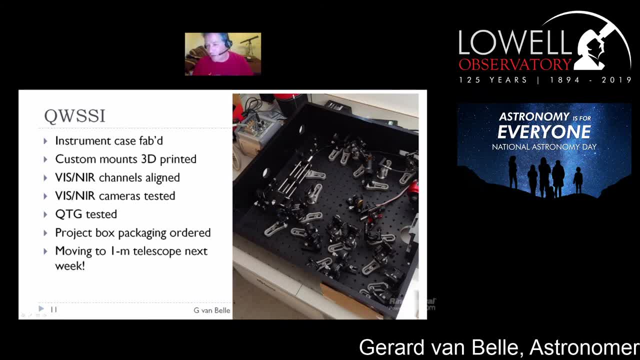 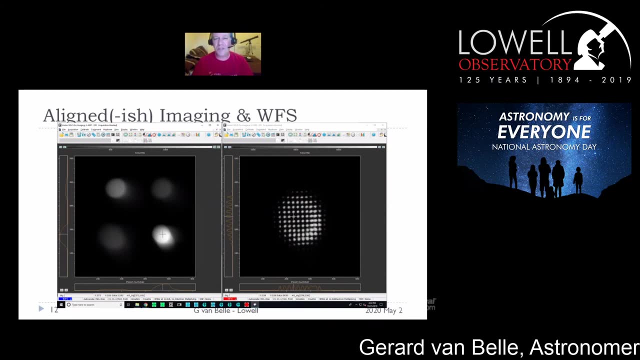 from companies that make them: the individual optics and components of these mounts and these little clamps that are silver here. these are all simply purchased from online vendors and we we're trying to get this next generation instrument moved out to the telescope. we have tested it in the lab and so you can actually see what the cameras see in the 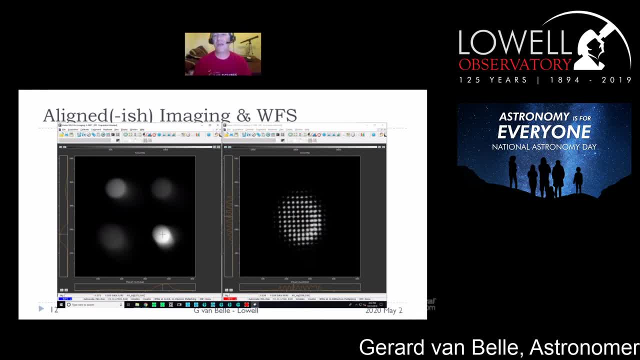 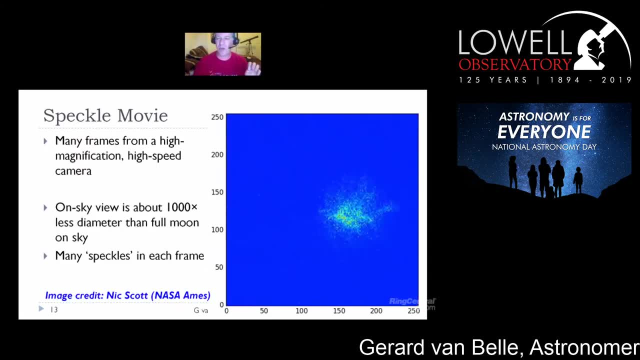 laboratory with an artificial source, but we're hoping to make it out to the telescope and see what it looks like. with the telescope it should look a bit like this. here are some of these speckles. i was telling you about where we have a very, very high speed camera. this has been slowed. 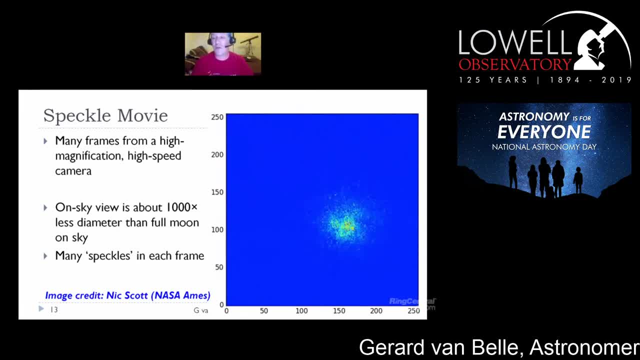 down a lot, but this is on the order of about 30 frames a second, and so, uh, this is at a much, much slower speed, but you can see what the atmosphere is doing if you're looking at a star at very, very high magnification and the uh, the magic that goes on here is we're able then to design software. 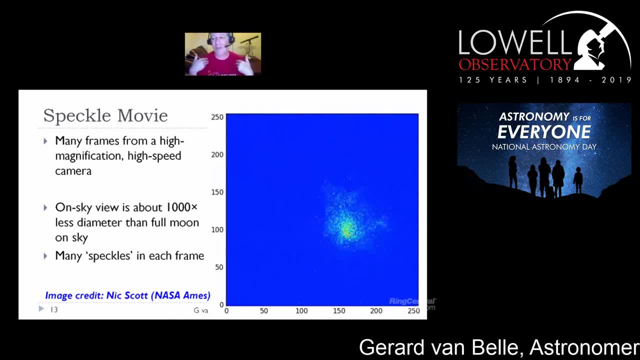 that can mathematically analyze this and it can make the atmosphere- not totally, but it can make it mostly- go away, can make it seem like you're staring through a clear atmosphere, just as if the telescope were in outer space, and you get something that looks like this: 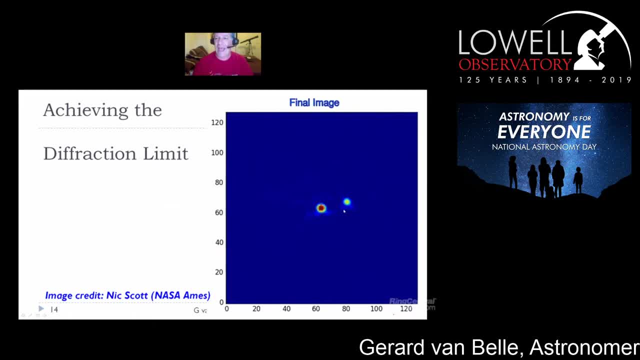 where you can stare at a star at much higher resolution and it'll actually let you explore and try and find, in this case, a faint star next to its host. you actually have two stars that are next to each other that you would never have seen beforehand, but you get to tease that out because 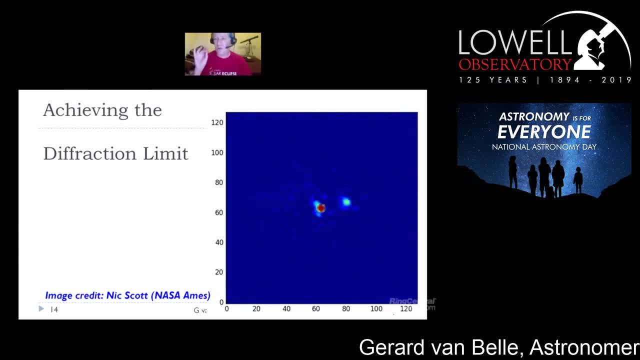 of the fact that we have now specially designed this instrument to try and explore this kind of phenomenon, and so i'm a little bit of a fish out of water with doing engineering, having been trained as an astronomer like michael west and deidre hunter and some of 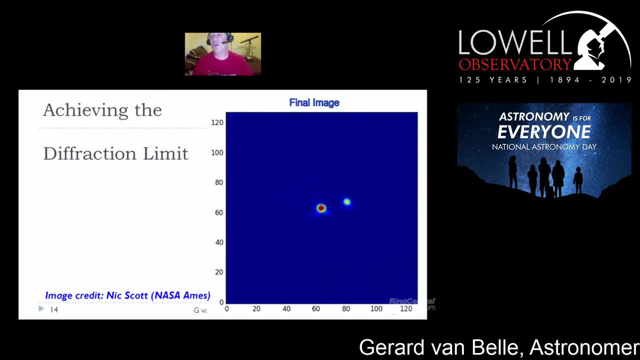 the other astronomers on the show tonight. we go to school and we take a lot of classes in physics, but not so many of us, myself included, take a lot of engineering classes. a lot of the engineering i'm doing is kind of self-taught, but a very useful thing of having me in this position is that 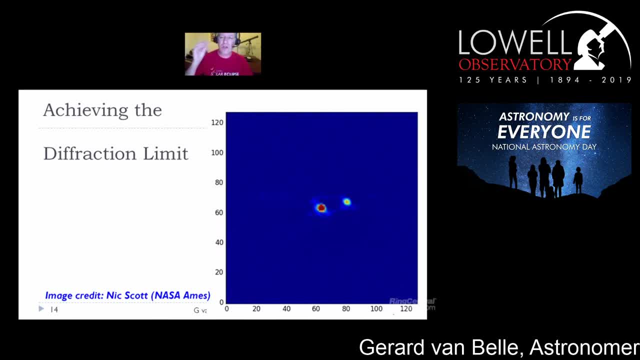 even if i'm not the best engineer in the world, i have a very clear idea of what i want the telescope to do, of how i want it to be able to give me this science. so that helps me in designing the instrument to do what i want it to do, because i'm the end user, i'm the person that's actually able. 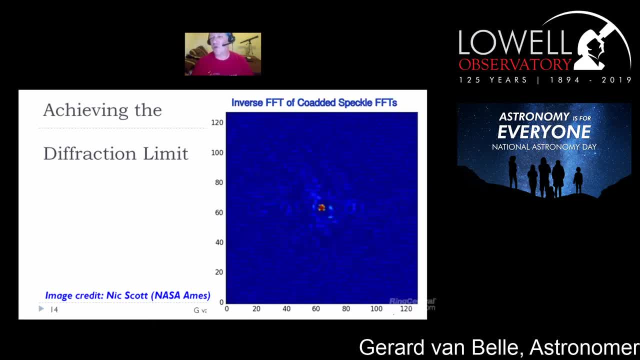 to uh, uh, be the consumer of the data products that come out of that. so in this particular case, uh, we have a big survey going on where we're looking at all these, very at all of the stars, to our own star, the sun, and we're trying to see if they have little faint companions like this one. 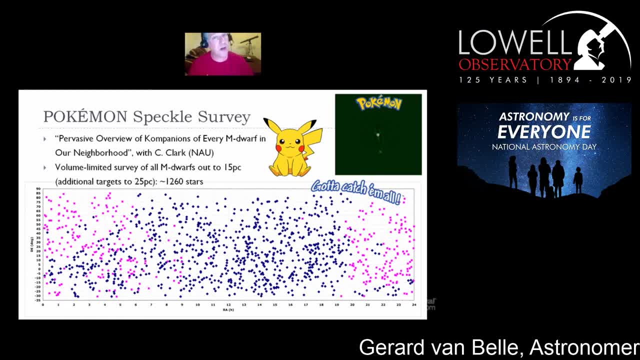 uh, we uh cleverly came up with the name of the pokemon speckle survey, the pervasive overview of companions of every young dwarf in our neighborhood. i'm doing this uh work with uh catherine clark, grad student at the northern arizona university, and so this shows a map of all. 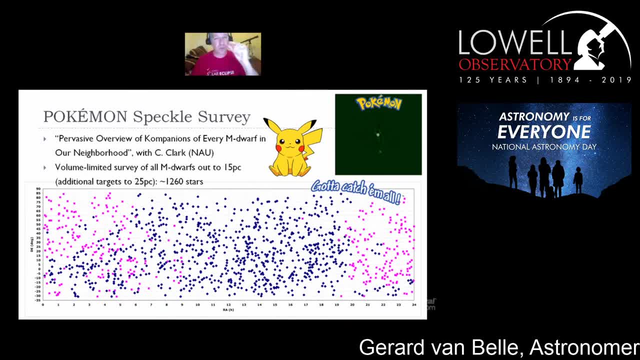 the stars in the sky that fit that description as far as being very small stars and being very near. trying to take a snapshot of every single one of those stars- about 1260 stars- and trying to see if they maybe have a little companion. so in this case we're finding about 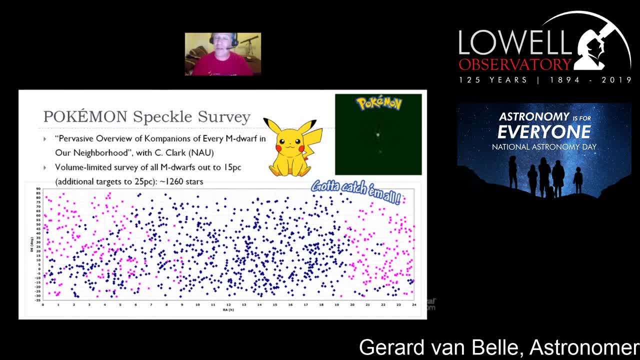 one-third of these stars have a secondary star next to us. so, just as we have in our own solar system, the- uh, the sun has a pretty big companion in terms of the planet jupiter nearby it. uh, these are stars that have even bigger companions that are, in fact, not just big planets but even bigger. 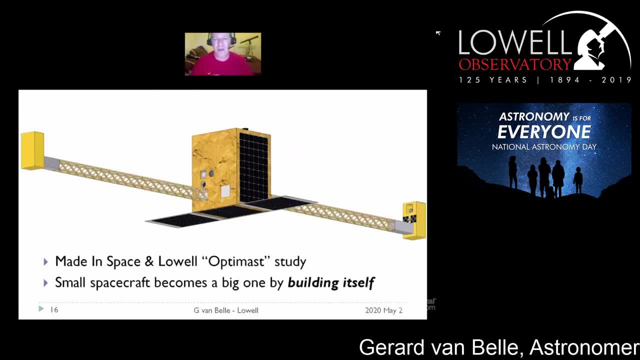 then that they're small stars themselves. um, finally, the last thing i'm working on, and this is one of the things that's been kind of fun to deal with in, you know, these interesting times where people are stuck at home and i'm stuck at home and i'm not able to go to my lab. 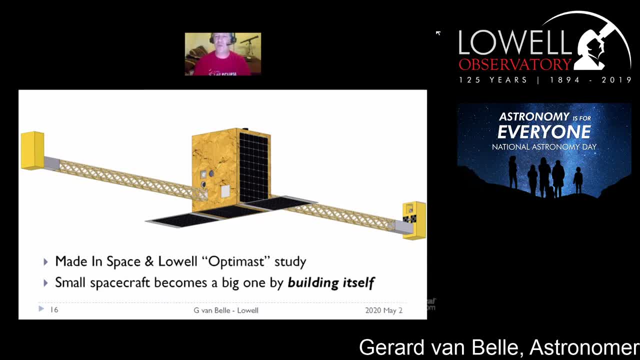 is. i'm working with a company called maiden space. we're trying to come up with a clever idea on how to design a spacecraft that we can send up into space. that will be small and fit inside of a, a small payload trout on a rocket, then become a very big telescope once we get up there. So this is a concept that 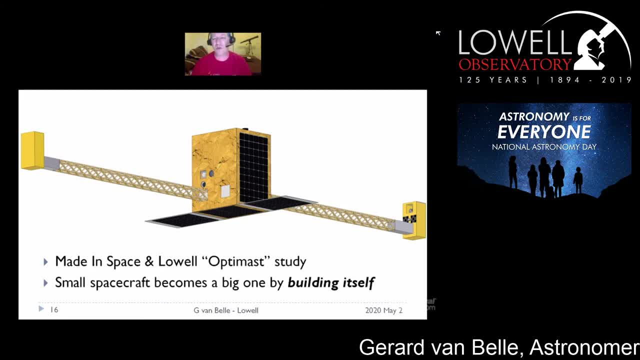 made in space and we at Lowell have come up with called Optimast, where you basically send up a very, very small package and then, once you get into space, the telescope manufactures itself. In this particular case, we will have small mirrors on these at the ends of these booms, but these booms don't exist when. 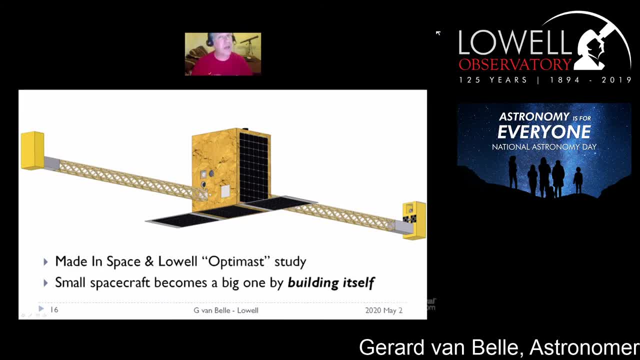 the telescope is launched, The booms are printed by a 3d printer in space, and so this sounds a little science fiction, but it's actually really kind of interestingly possible and tantalizing right now. Made in space has a number of manufacturing facilities right now on board the space station, and so they 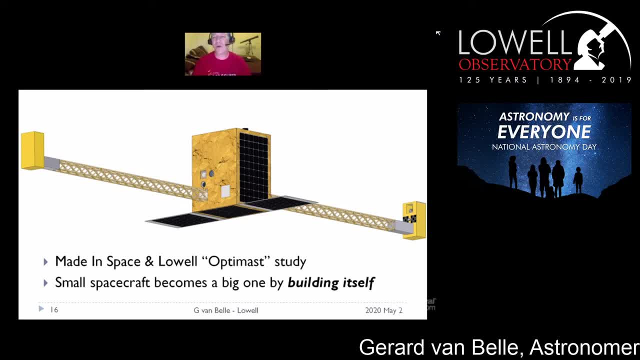 actually are great colleagues to work with because they are actually doing some really amazing things for real that seemed to be pulled out of Star Trek and this is stuff that's happening today up in orbit, So it's a lot of fun I'm working with them. They. 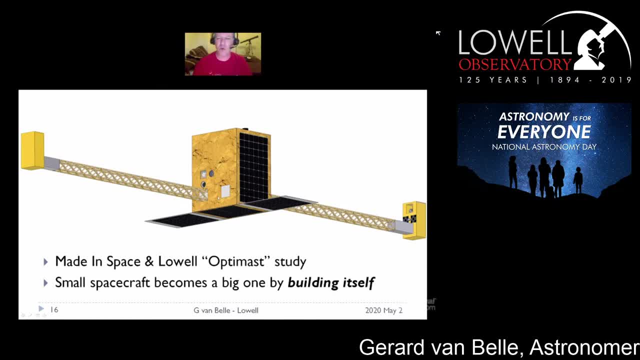 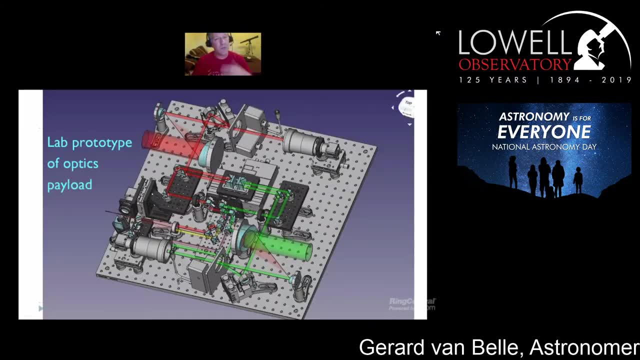 are providing the infrastructure for these boom printing. In the middle of the spacecraft there is a slice that is an optics payload that looks like paper, a little bit like this. This is my contribution is I've been coming up with this design that then works with these printed booms and the mirrors on the 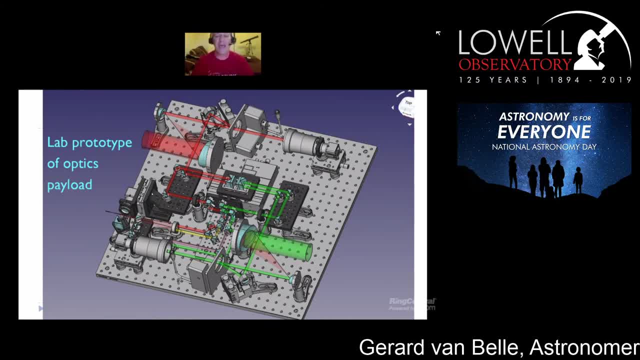 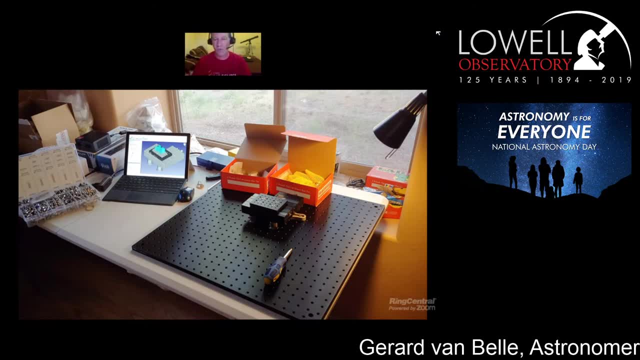 outside of it. so this is another thing that I'm doing during the day, and a fun thing that I'm able to do at home is taking this idea and I've been working me on actually turning it into reality, because, again, you can order the parts and bolt it together, and so I have just started on this, with getting some of 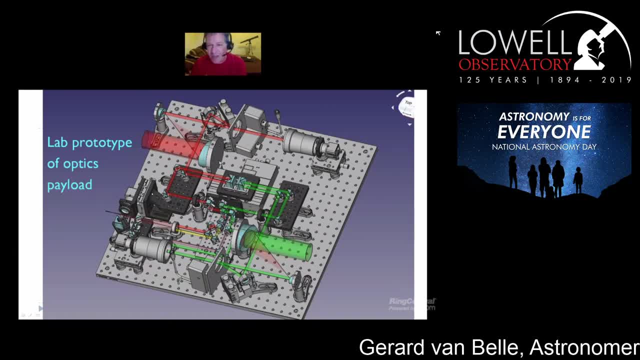 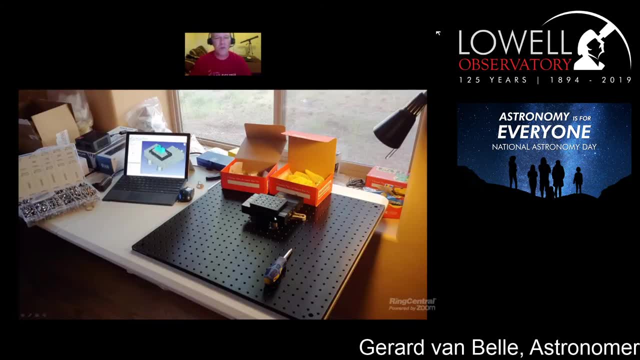 these parts. if you look back here on the plan, you can see this motorized stage right here in the middle. that's the first thing I bolted on to the breadboard, and so actually getting this all put together so that we can then test it in. 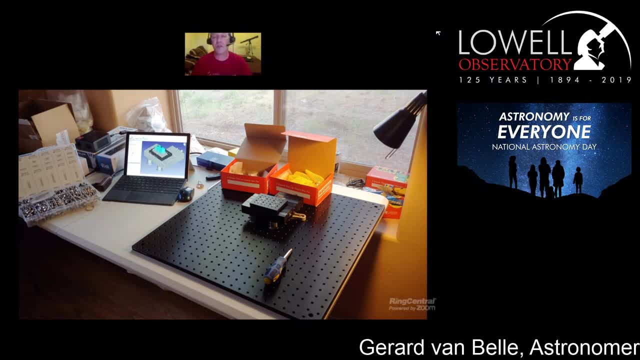 the lab, which then maybe will get us to the point of building something that's more representative of the actual spacecraft to the camera in the future. but this is going to be the initial lab test article and so we can actually do that at home. I've kind of stolen a bit of area from my kids playroom and it is. 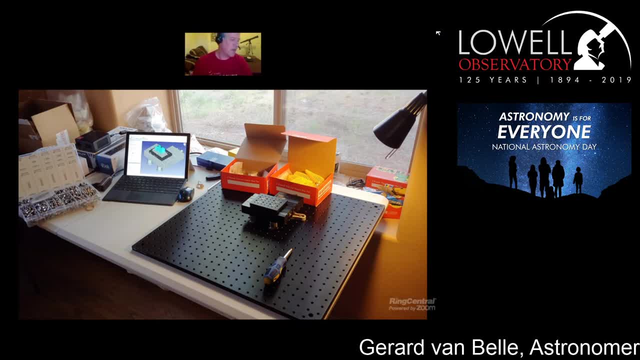 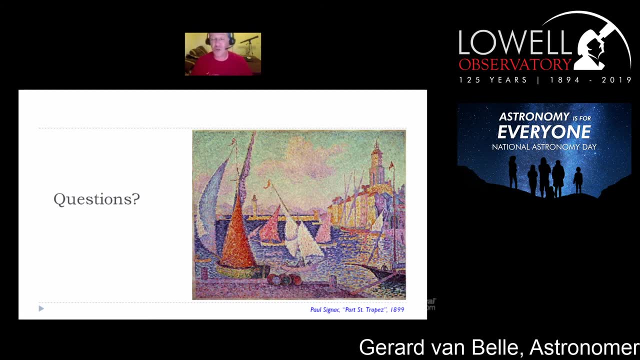 now a small workspace for me, and so with that I'm going to turn it over to any of the questions that might be there, and it's always a lot of fun to try and wade through this morass of you know, all the little things I'm coming up with. the 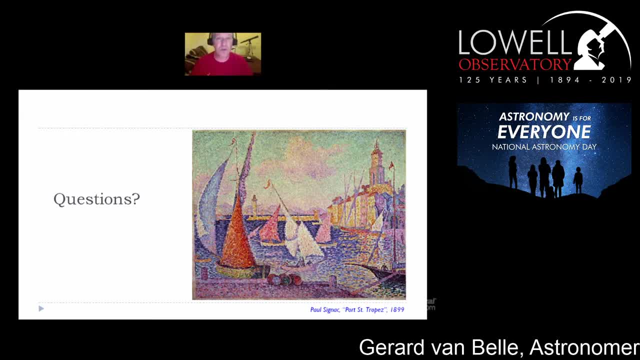 day with you. know what does an astronomer do on a day-by-day basis. it is a interesting challenge to try and organize it all, but it's always very exciting and very fun. I see a first question from Terry Pantano. have you noticed less turbulence during this stay-at-home period? it would seem that. 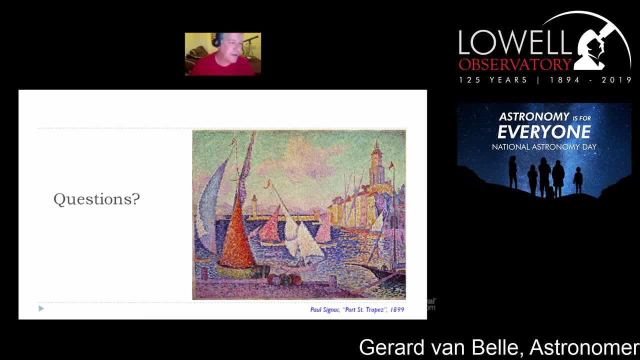 besides the fact that there's a lot of activity going on in the lab and the science, less pollution. there are less domestic and military flights stirring things up. so unfortunately I haven't had a chance to do a lot of work on sky, and the reason for that is, at the moment our little Discovery telescope has been 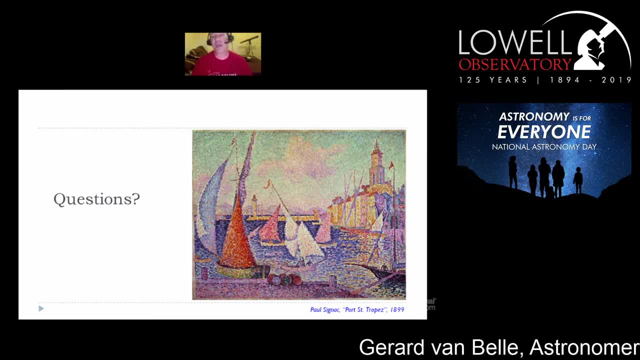 actually in hibernation. we actually have a pretty good-sized crew that runs it and we're still trying to fish through all the appropriate protocols to, you know, be able to keep things running but keeping people socially distant. a on paper, a single person could run the LDT at night, but in 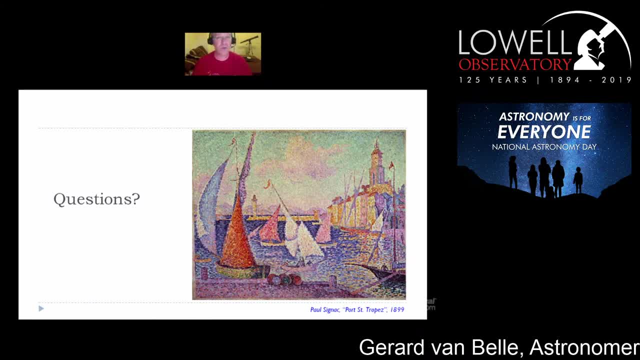 practice, for the purpose, for the purposes of safety, we have always two people out of the site. it's a fairly remote site, about an hour outside of town. even if we were to sort out that- and I think we'll come up with some way to do that- we, you know if anything needs maintenance on the telescope, that often. 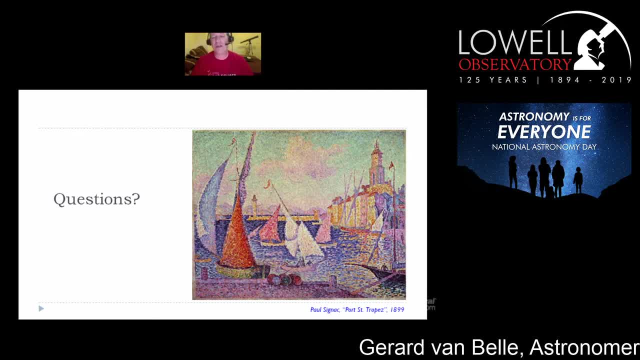 requires two or three people, and so we need to make sure that we can approach this safely and be happy with that. so I'm really eager to see how that is with less flights. but by and large, the principal driver of turbulence of the atmosphere is the solar heating. solar energy is a much bigger driver of the 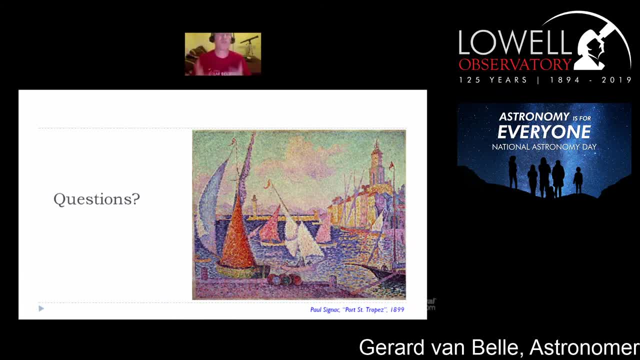 energy that makes the atmosphere of this boiling turbulent medium, and so I think this the my expectation would be that the turbulence is going to be about the same. I have another question here from summer Brown: what is your absolute favorite part of being an astronomer? what do you find is your biggest challenge? so my favorite part is doing all sorts of 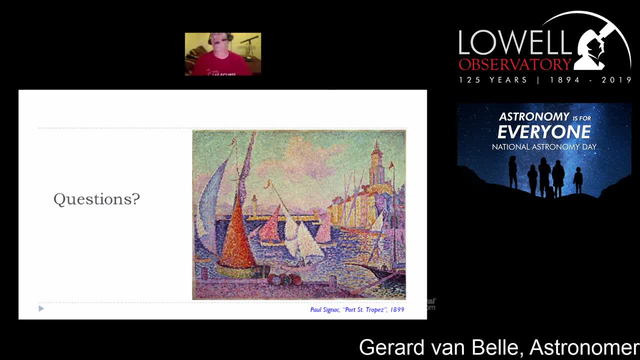 interesting things and having a lot of autonomy to do it. I like the aspect of the fact that I get to do things that and see things that people have never seen before. sometimes we get to see things that people have never seen before. sometimes we get to see things that people have never seen before. sometimes we get to see 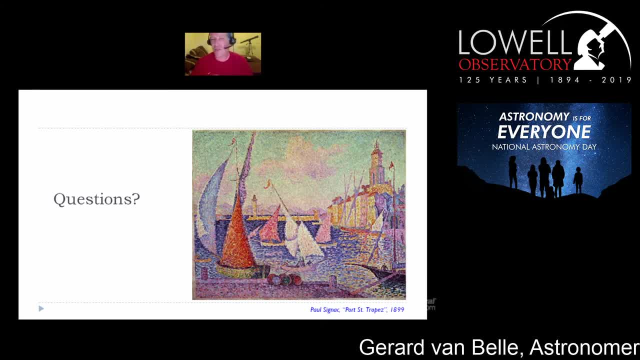 things through telescopes that nobody has has had a chance to do before and in and in my specific role as astronomer, that does this rotation. that's actually especially true because I build cameras and telescopes and instruments that nobody has built before and that have capabilities that nobody has had before. 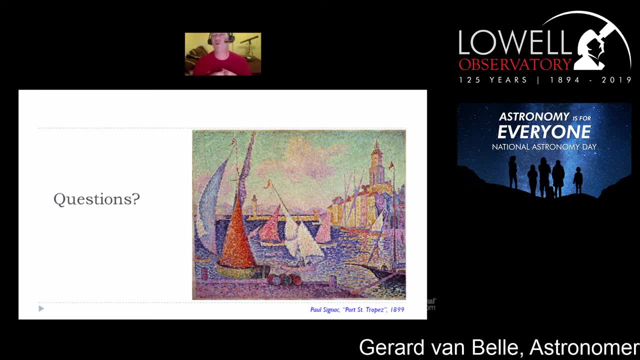 and I'm the first person that gets to use them, and so you get to do some of the fun stuff of, you know, skimming the cream and doing this sort of discovery and observations that nobody else has been able to do before. so that's been a 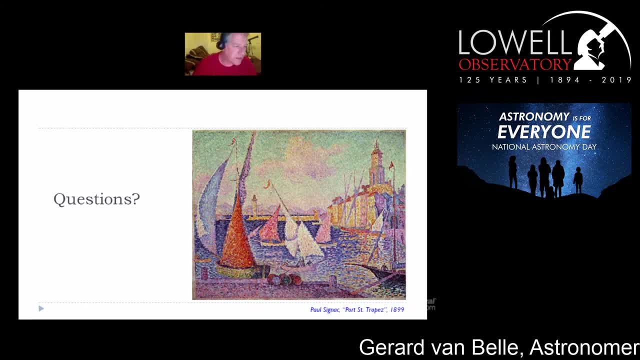 lot of fun. another question for Terry Pantano: what plastics do you plan on using an optimized radiation with detrimental effect? so the materials that go into building this sort of thing have all been space qualified. we certainly- and this is more in the wheelhouse of my colleagues- over made in space, but 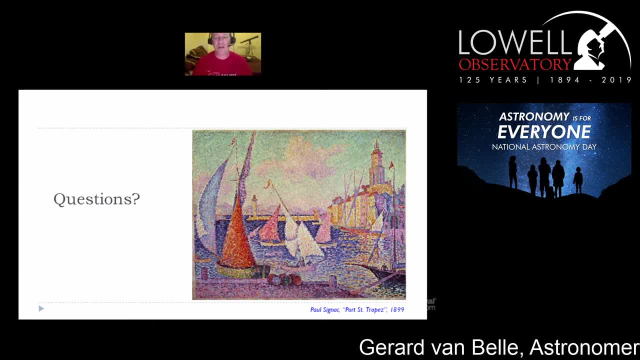 certainly all these things have been vetted so that they are expected to meet the mission lifetime expectation and that's inclusive of the entire range of phenomenon you expect to encounter in the space-based environment. so that includes ultraviolet aging of things due to the radiation of the Sun, that includes any kind of flexing, that. 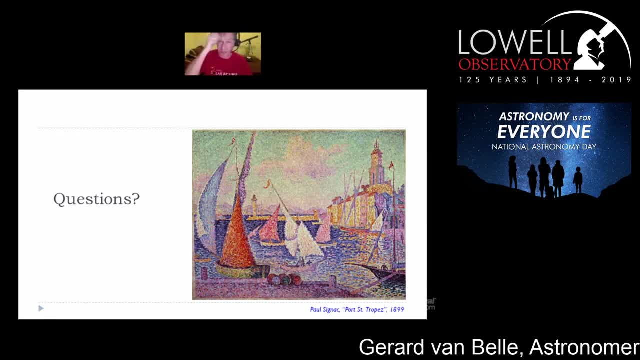 may come from the motion of the spacecraft and a number of things like that. so we try to make sure that we have our handle on those things. a question from my lovely wife, Stephanie VanVil. did I major in astronomy or physics? so when I went to college I went to Whitman. 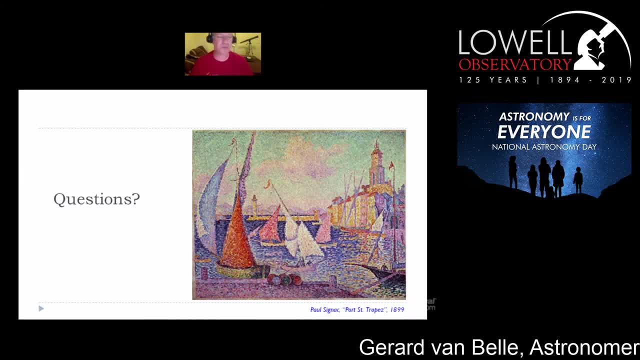 college in Walla Walla Washington place- so nice they named it twice and they they had a program there where you can do three years or within and then two years at a engineering school of your choice- Caltech or Duke or Columbia, I think was on the. 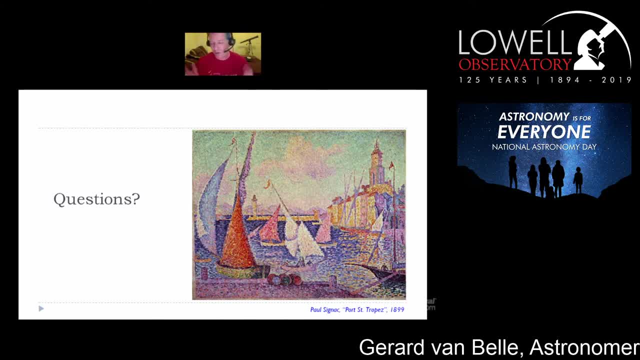 roster at the time and I went to Whitman thinking that well, nobody actually gets a drop test in astronomy and so I would go there and I would then transfer away from Whitman and do, probably, mechanical engineering. But while I was at Whitman I got very 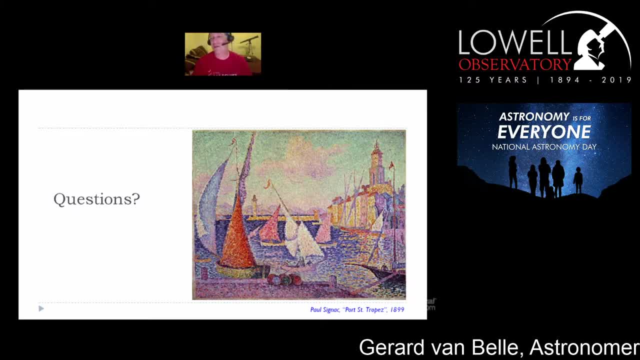 interested in astronomy and ended up to just stay at Whitman. I really loved my time at Whitman College and so I decided to remain there and not go to Caltech was my choice for graduate for the second part of this combined degree. So while I was at Whitman I did a combined degree in physics and astronomy. 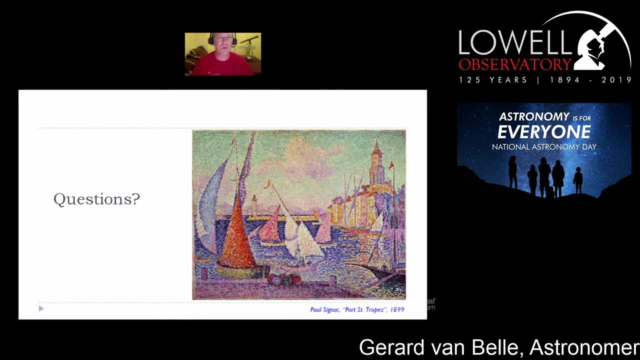 and then I went to Johns Hopkins for a master's degree, also in physics, and then also went to the University of Wyoming for a PhD, which on paper also says physics. Both the Johns Hopkins and Wyoming time was physics but it was a lot of the strong. 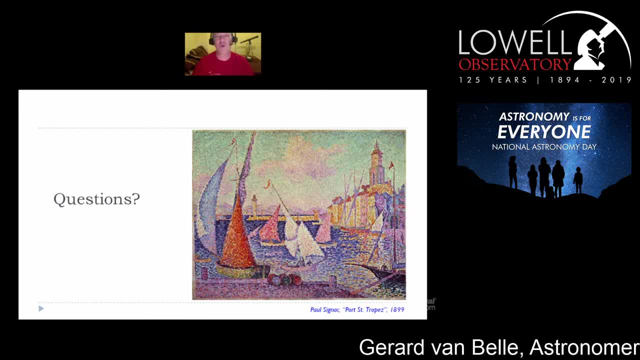 astronomy. You can do a lot of astronomy, lot of hands-on working astronomy. so my the, the words on paper say physics, but technically is a lot of astronomy. and just like with deep Deidre hunter- dr hunter and dr Michael West talked earlier, they once you get to graduate. 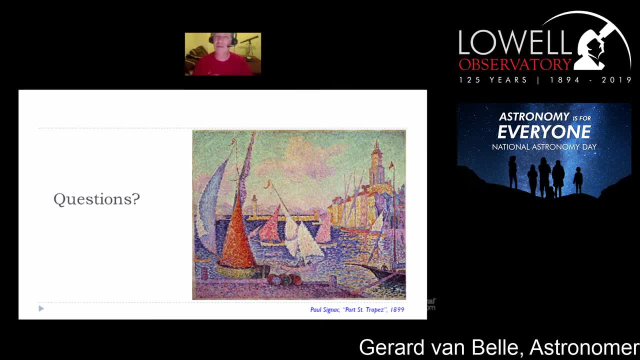 school. they pay you to go to school a lot, but enough to get by on it, so that's quite nice. a question here from Lewis Van Bell, my younger brother: why make booms on the satellites? why not use a swarm of nanosatellites? ah, so this is. 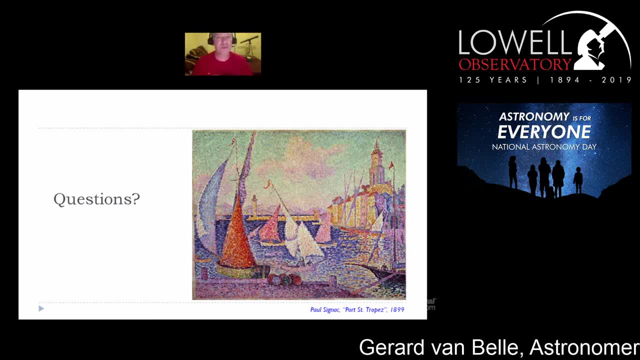 actually a very interesting question that we get a lot. formation flying is the term of the art that go into this place. so, information flying, you have small spacecraft that would fly around a central spacecraft that has the cameras and in that case you have six degrees of freedom to worry about each one of these. 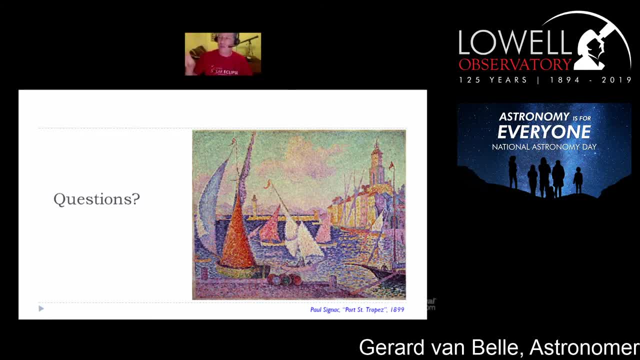 you know, companion satellites could move around in X, Y & Z and to tilt and roll. so I have to control all of that with consumables. you need little rocket motors on board this thing, and so if you have instead your outboard optics on the end of a boom, the boom fixes things in place. they're not going to float away. 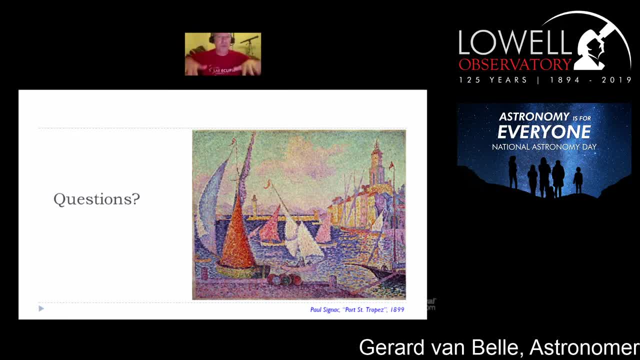 and the boom may twist and bend a little bit, but more or less you have a straight line that joins the central spacecraft to the outboard spacecraft, which can flex a bit. but you now have really kind of turned this into a two-degree freedom of problem is basically constraining these nanosats to. 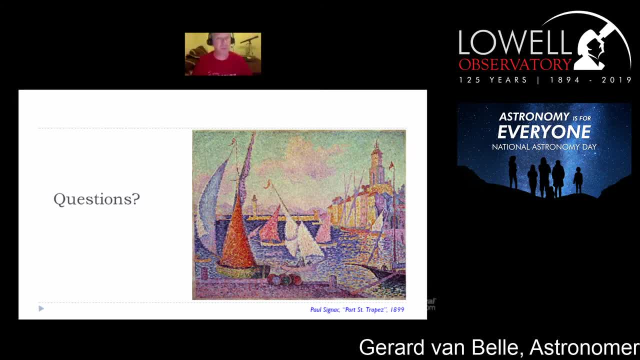 be on the inside of a sphere, and so it's a much simpler problem. that's probably a good stepping stone to doing this case of formation flying further in the future, but it it is actually a lot simpler to do this case where you have it attached. and now I'm getting a question from Christine Van Bell. my younger sister wants to know who is the best. 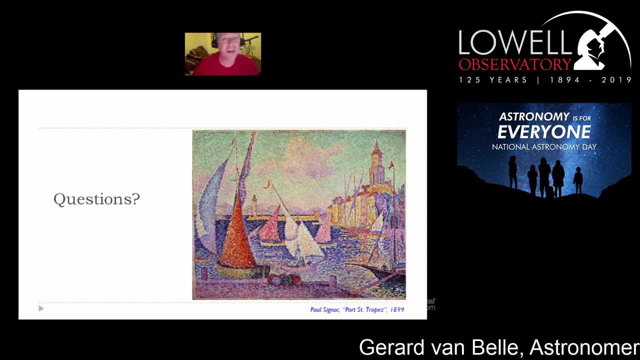 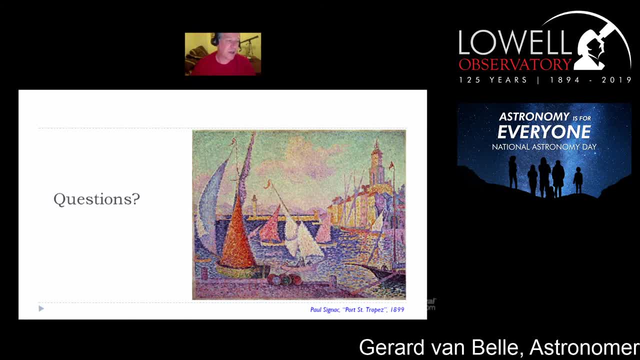 sister, so no comment. who is my favorite sister? and that's a tough sister, so no comment question. as she correctly notes, it was my, my mother sister who knocked my tooth out with a book, oh, sorry, with a shoe, because I was reading her Harlequin romance out loud as a young child. then she apparently ‑‑ at this, so skip that and go. 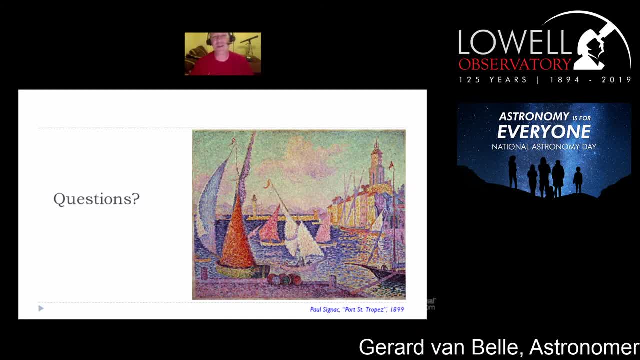 school, uh and uh, that is nowadays called shoreline christian school, uh, and so that was a a small, private christian school that i went to. that gave me a very good preparation to go on to whitman college and the rest of my education. another question here: do you think there's life? on other planets? will humans get to mars in our lifetime? it's actually two very interesting and separate questions, um, so i do think that there is almost certainly life somewhere out there. we have a good example of life here, um, and the universe is such a big, large place that it's. almost inconceivable that there would not be life elsewhere. if you look at the geologic record on earth, you know some four billion years ago, as soon as the conditions here on earth were favorable, life sprang into existence, and so i expect that to be the case elsewhere. 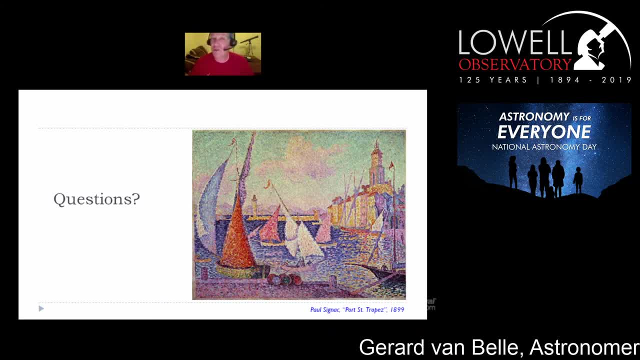 but, as i said earlier, the universe is a big, huge, large place, and so our ability to encounter that other life is going to be limited because, uh, the distances between the stars are so great that, uh, you know, even the fastest spacecraft we could have today if we were to go towards the 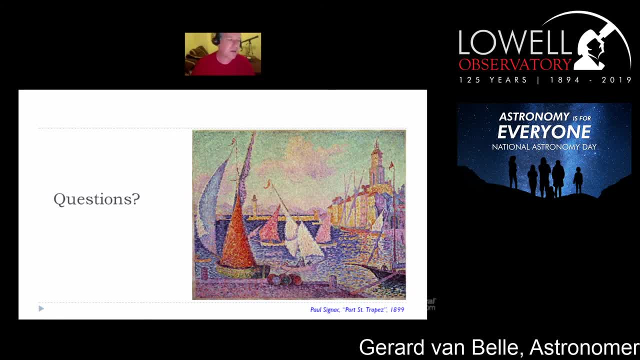 nearest star, we could have the fastest spacecraft we could have today. if we were to go towards the nearest star to us, it would take a hundred thousand years to get there, and so, uh, i think that that is a tall order. we're getting very, very good at remote sensing, and so telescopes like the 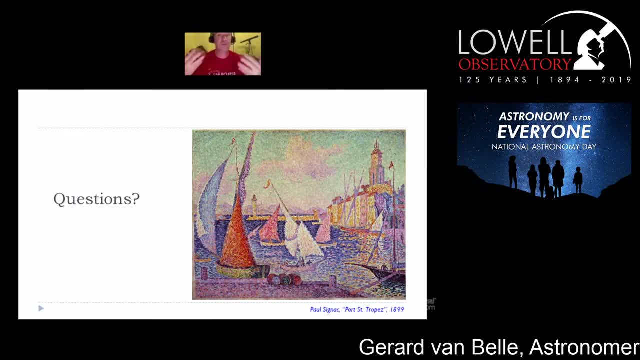 lowell discovery telescope and employ and these new bits of instrumentation that we're building today. um, i believe that within the next 10 or 20 years, we will use the most advanced telescopes to detect life around planets being hosted by nearby stars, even if we can't get there. 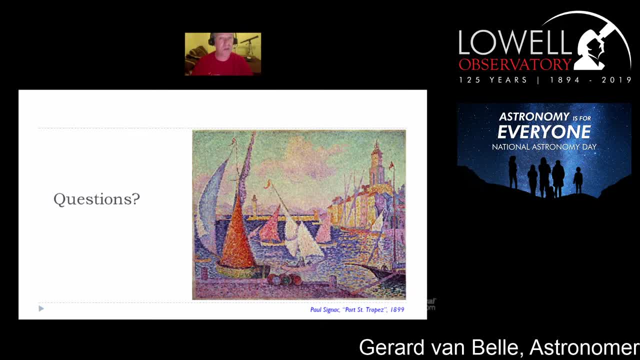 i think we'll probably uh, come up with good evidence that there is life there. uh, what do i find my biggest challenge from summer? brown, um, trying to figure out what i'm going to do. every day i wake up in the morning and i'm like: what do i have to do today? so i i tend to be a 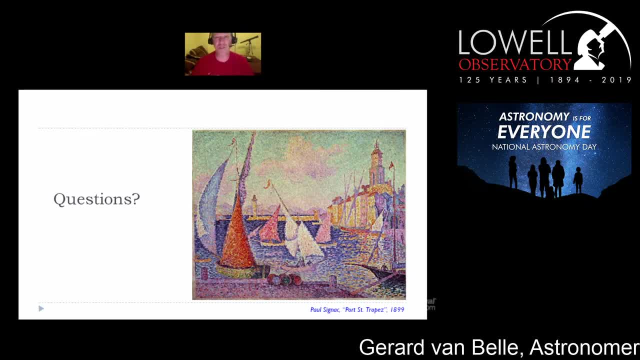 little over enthusiastic in in uh coming up with projects i should join and work on, and so i have a lot of irons in the fire and that can be very difficult to uh juggle everything. but, uh, it's a new challenge. that's, uh, uh, always very exciting, so i love that very much. um, i am going to turn it. 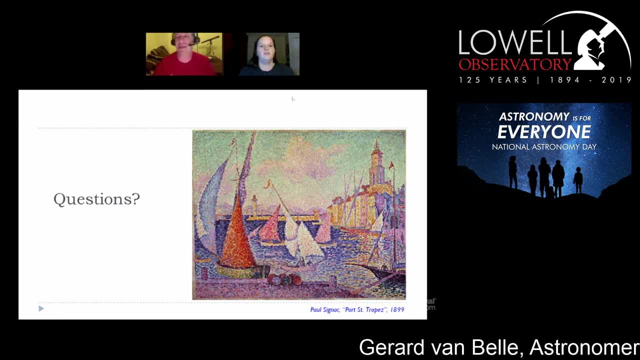 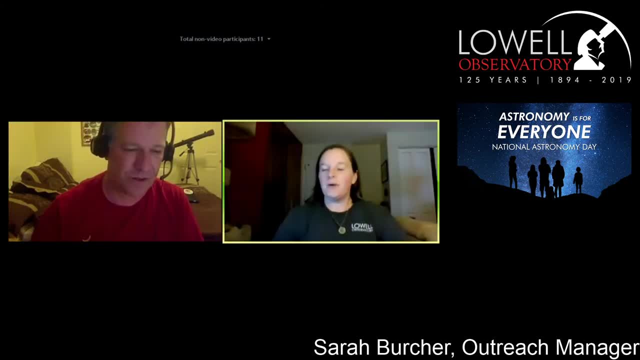 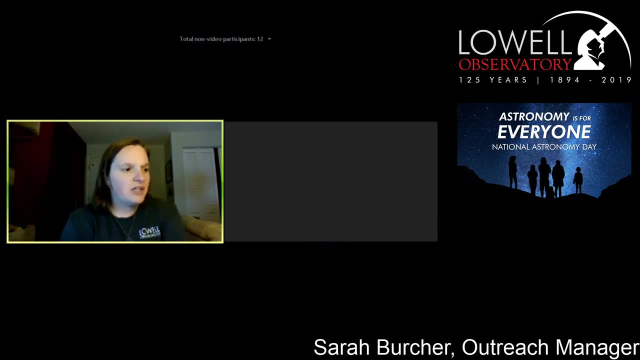 back over to sarah at this point and, uh, let's stop my share, sarah, thank you so much for bearing with me. all right, thank you, gerard. so, uh, we are going to shift our gears a bit once again, um, and i'm going to introduce one of our educators, melissa panter, who is going to talk, um, about how more 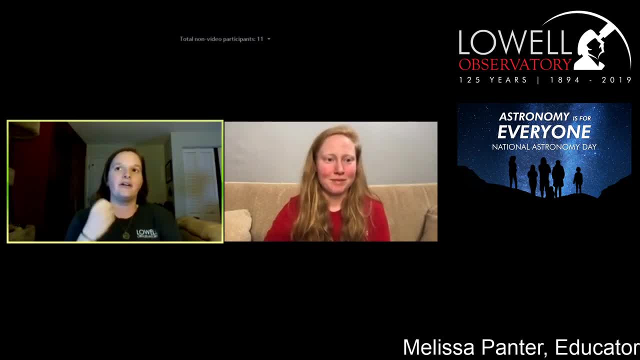 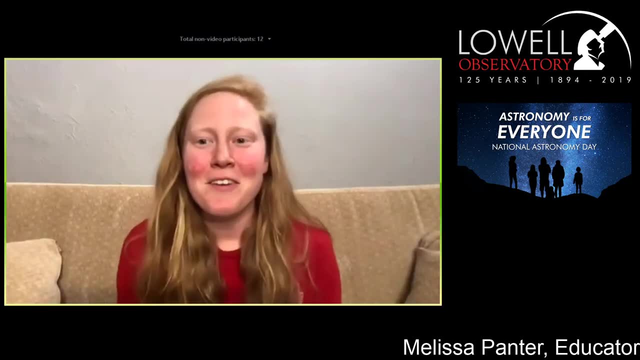 about how the world around us can influence us and how we can influence the world around us, influence our, our experience with the sky. so, melissa, take it away. thanks, sarah. hello everyone, my name is melissa panter. i am an educator at low observatory um, and we're going to talk about 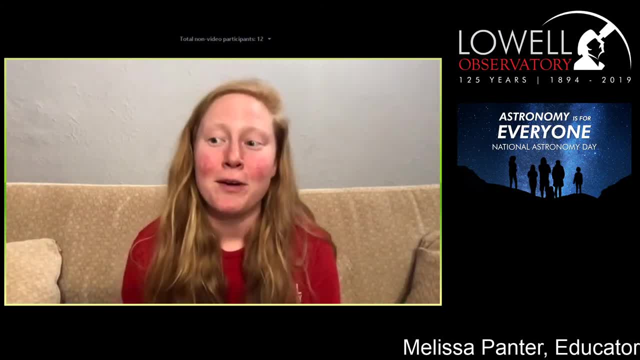 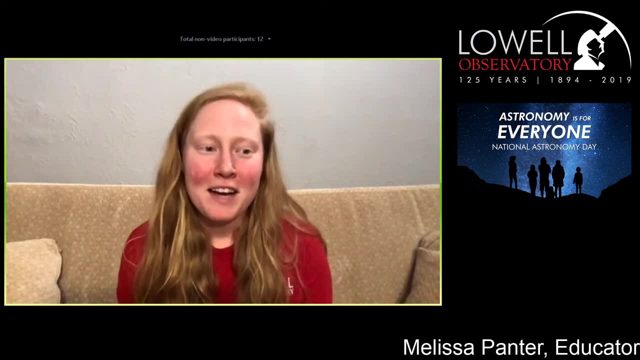 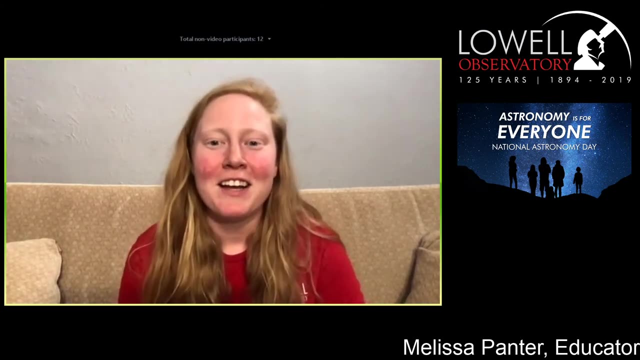 basically what brought me to astronomy and, unlike with john or claire that we heard, um, and they started like young in their childhood looking up at the sky. um, it kind of took me a little bit longer to get there in my, uh, in my lifetime. um, it's kind of like a winding path, i would say so. growing up, i grew up on the 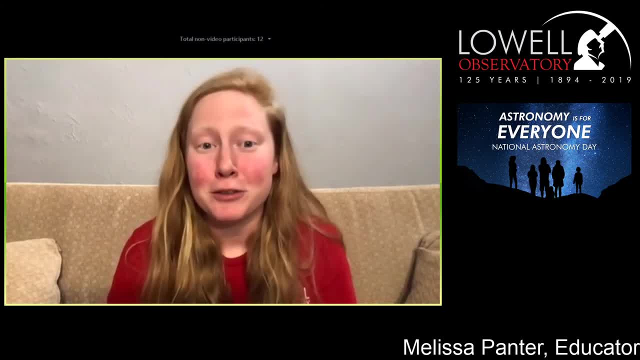 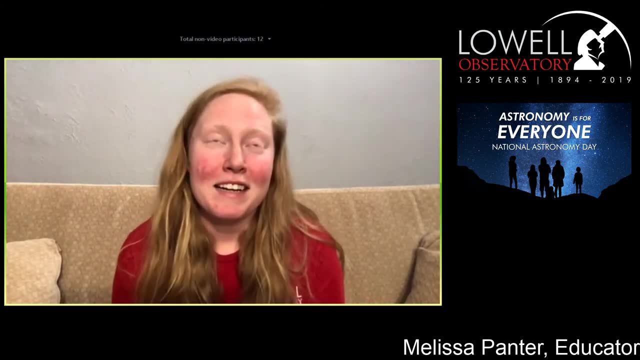 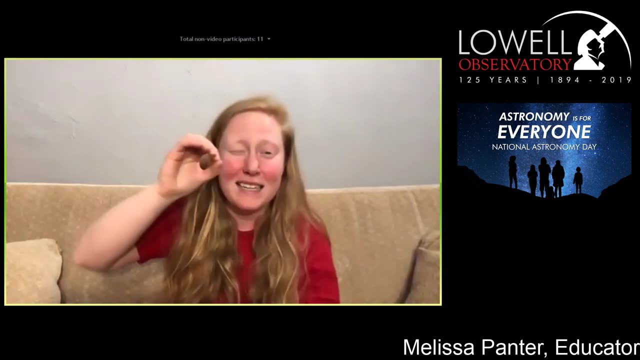 east coast where, um, i was surrounded by trees and not a lot of stars, so it didn't really spark my interest in astronomy. um, you can kind of- if you're from the east coast, you probably know this- you go outside and you look up and you just see trees and just like a little tiny hole in the sky and 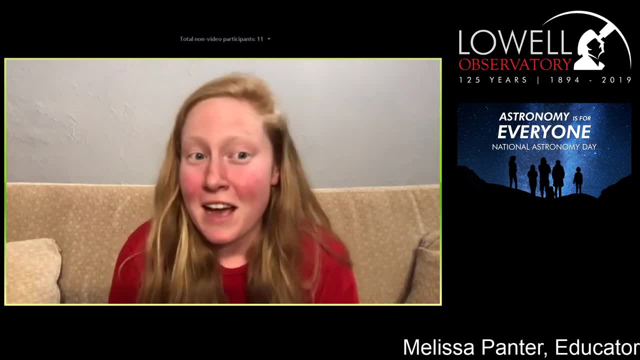 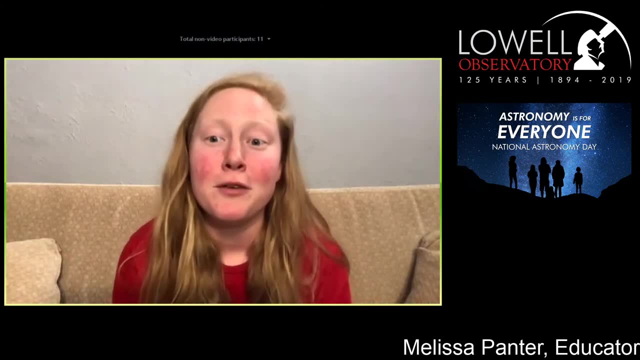 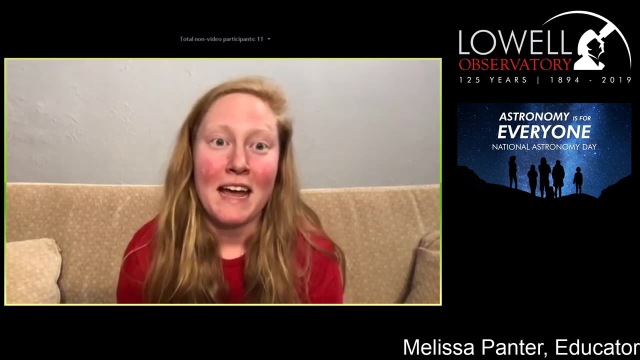 that's what you can see up above you. um, it wasn't until after college for me. i started going out west, closer towards arizona. um, i went to cuba, new mexico, with americorps, which is the domestic peace corps, and myself and my team ended up living out. 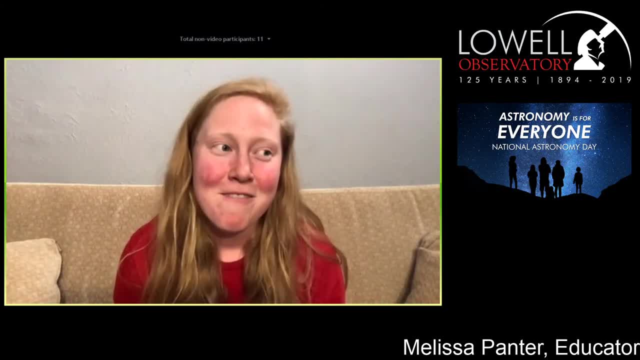 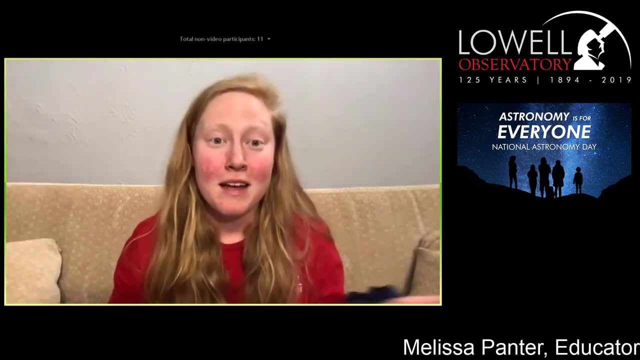 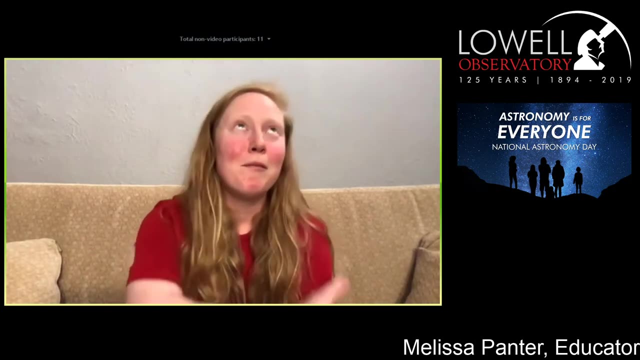 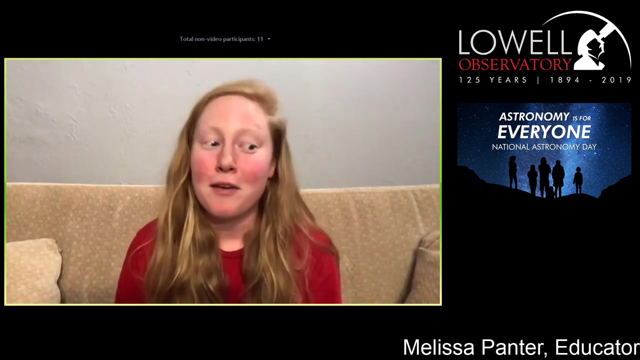 on the navajo reservation and i remember vividly the first night we were out there. that land was so wide and so open compared to what i was experiencing back home, that when i looked up at it it was more stars than i've ever seen in my whole entire life and it blew my mind. i was like 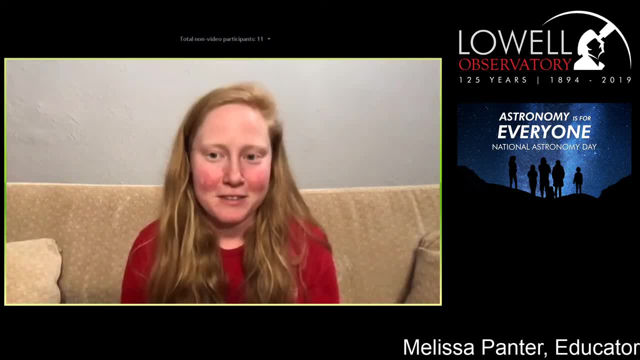 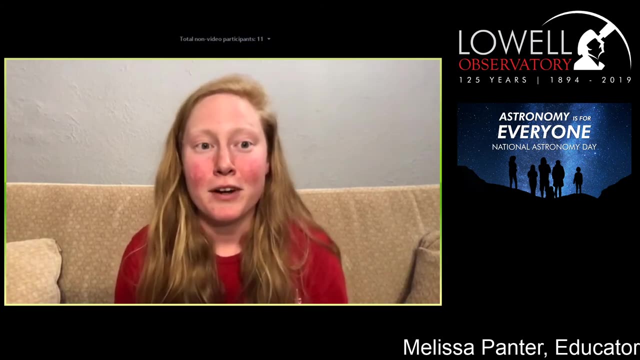 what is life? who am i? i'm just a speck in this universe and i really didn't start really diving deeper into these ideas of what the sky, what the universe was giving me, until i started working in public lands. um, i used to mentor youth in a youth conservation corps in yellowstone national. 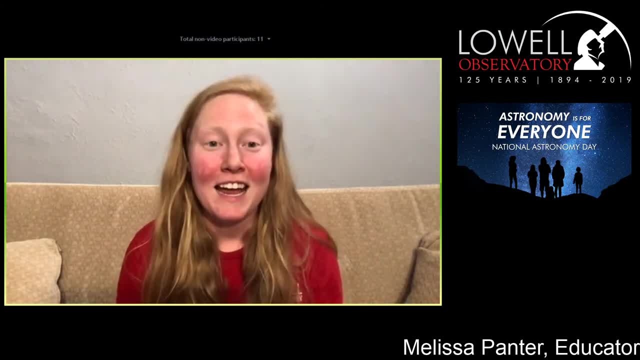 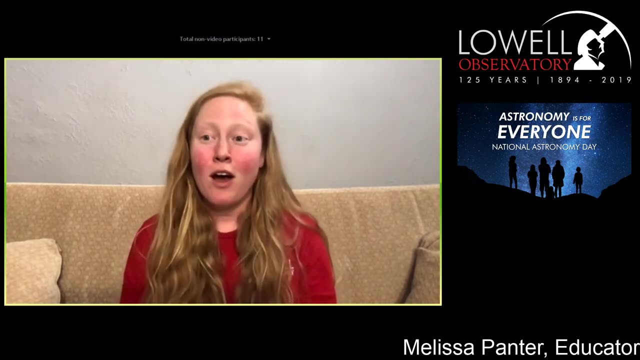 park, where we would go into the back country and we would start asking these questions together with these youth from across the country experiencing, sometimes for the first time, just like i did- the night sky, seeing all of the milky way, seeing all of these crazy planets. you. 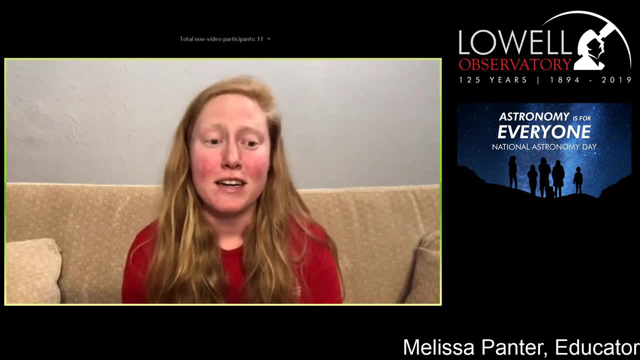 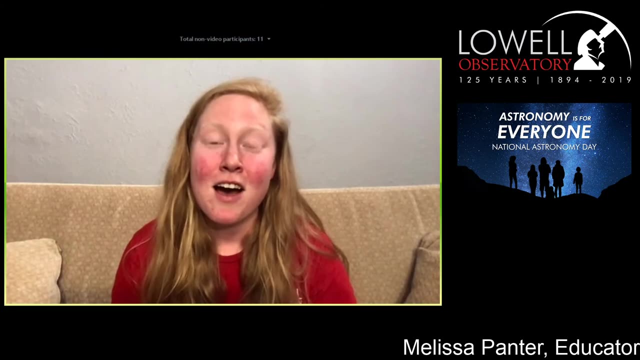 normally couldn't see um, and really started diving into astronomy. it wasn't until i actually, this past summer, met lowell observatory's historian kevin schindler, who you're going to talk to later today. um, i met him at grand canyon national park. inside the canyon i was working at the bottom of the. 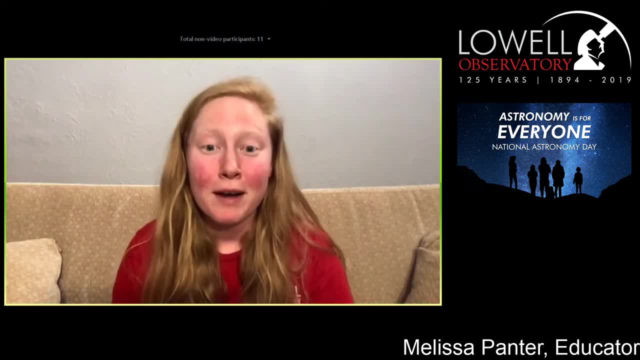 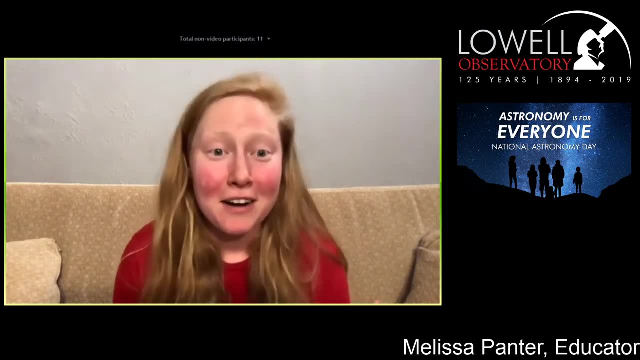 at the grand canyon and he hiked down to give a program about lunar legacy, about the apollo astronauts actually training in grand canyon, and my nerd radar went off the charts and i was soaking in everything he was telling me to the point where i was like, oh my god, i'm going to go to. 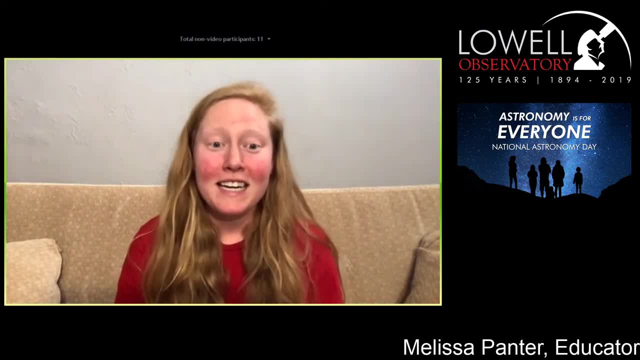 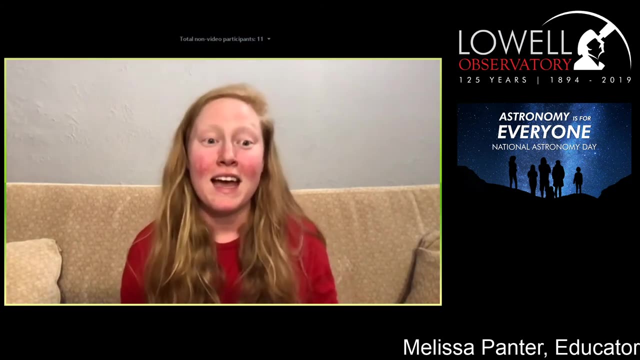 the point where myself and one of my co-workers actually ended up creating um, an apollo program for visitors who came down to the bottom of the grand canyon, and that experience just really got my astronomy sensors going. i started researching more than i ever had and really 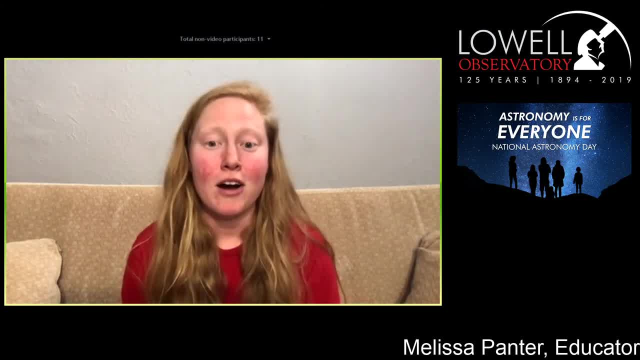 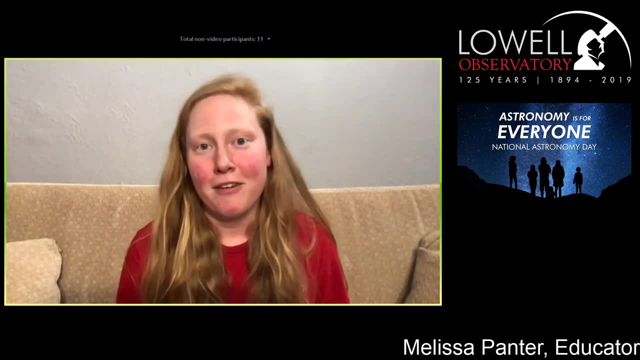 started connecting with other humans about our past, our history, exploring the night sky, in land and sea, and i was like, oh my god, i'm going to go to the bottom of the grand canyon. we were sitting at the bottom of the grand canyon looking up and discussing how we, 50 years ago, 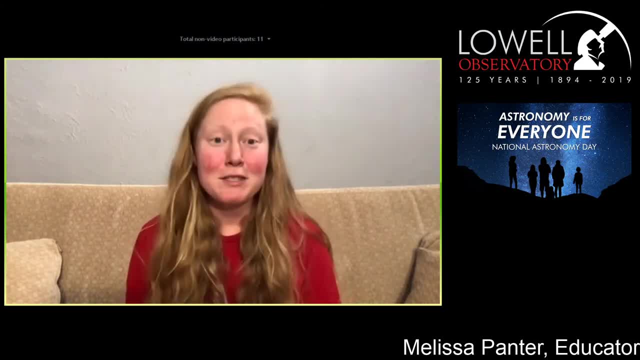 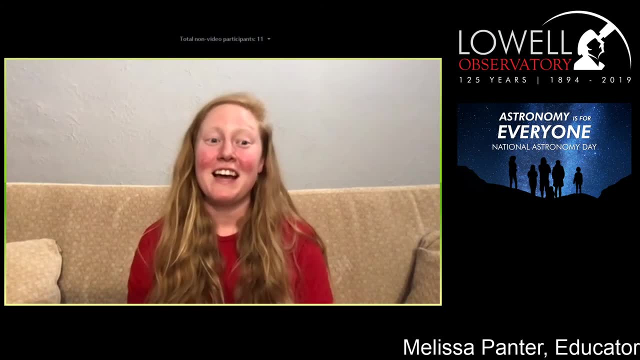 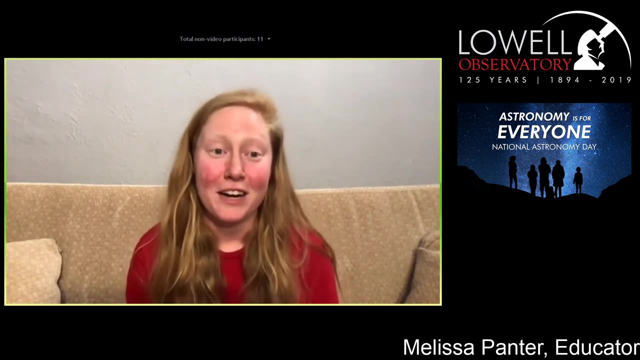 landed humans on the moon. it was mind-boggling, and so i started going to lowell observatory on my off time and eventually was able to apply to work here as an educator, doing something i love, which is talking to the public and sharing, sharing experiences and the night sky and our knowledge. 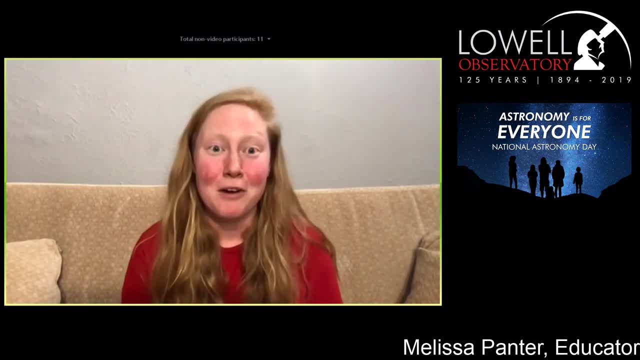 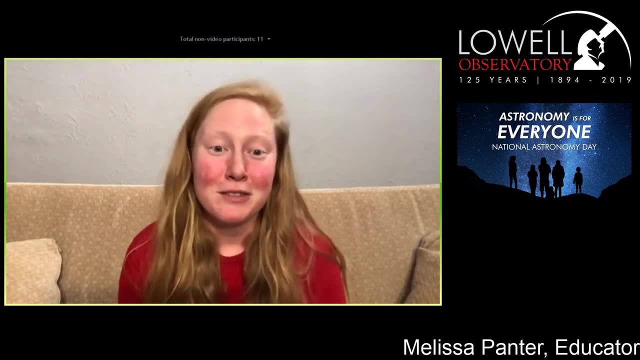 um, which has drastically changed what i know and what's out there in the universe. i'm starting to learn about galaxies, stars. you got a couple of those snippets from our astronomers earlier. it's been really exciting, um, becoming an astronomer, uh, at lowell observatory and kind of. 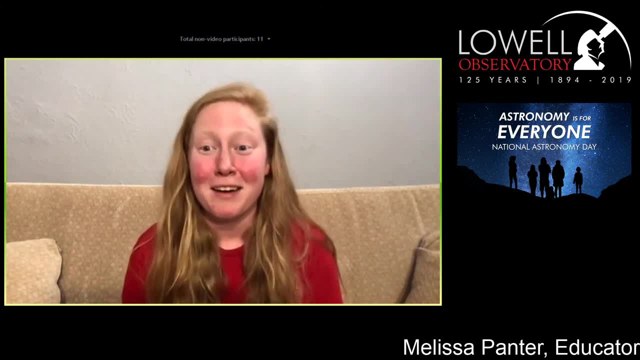 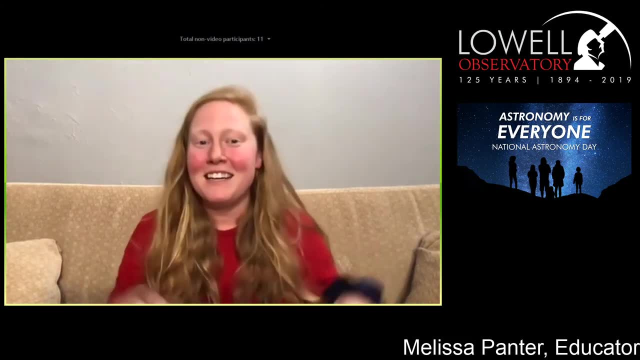 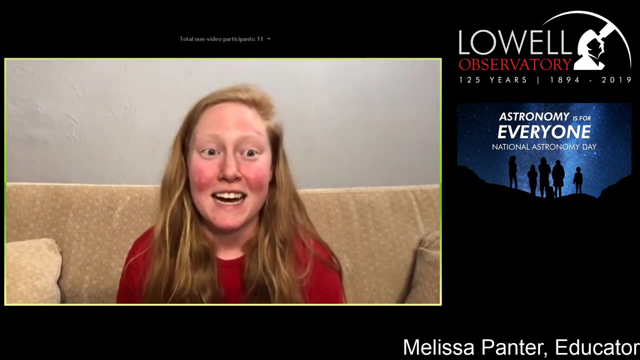 being a late bloomer in some terms. so i know we had a lot of people asking: oh my seventh grader is interested in this. well, you could be the seventh grade. 26, 30, 50, 100, and it's never too late to start learning about the night sky. 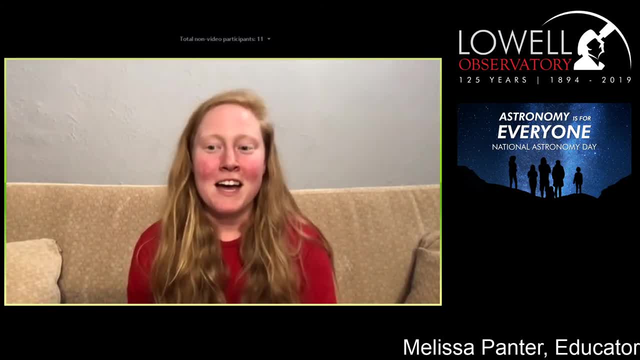 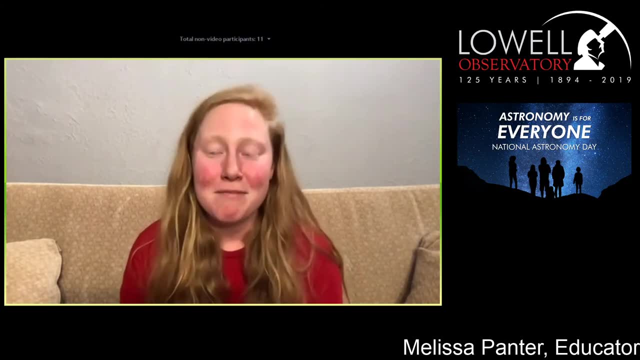 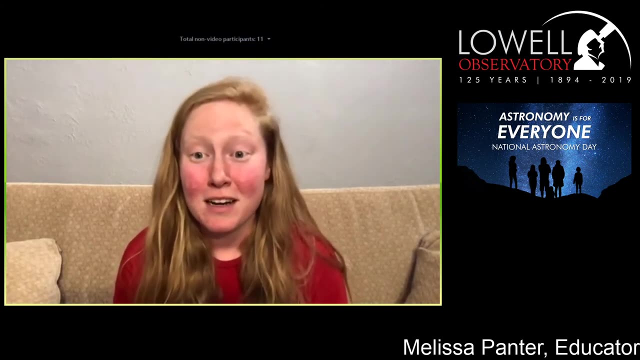 and letting your curiosity take the wheel. um, hopefully you all are excited about what you've been learning. this has been awesome. i really have been kind of basking in all this knowledge that we've gotten over the past hour and a half. um, definitely, joyce talked about what kind of 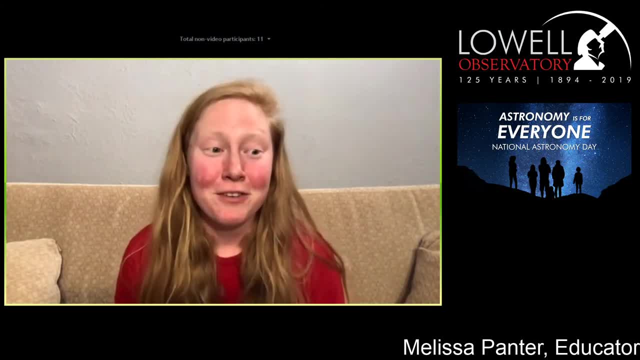 astronomer we are, um, i would say over the past few years we've been learning a lot about the universe. i've been a facilitator, an explorer, an experience seeker and a recharger just at different times, and so just it's just fun to get out there and start looking and start exploring and seeing. 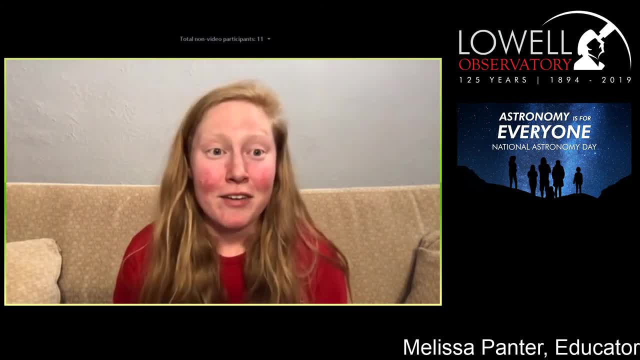 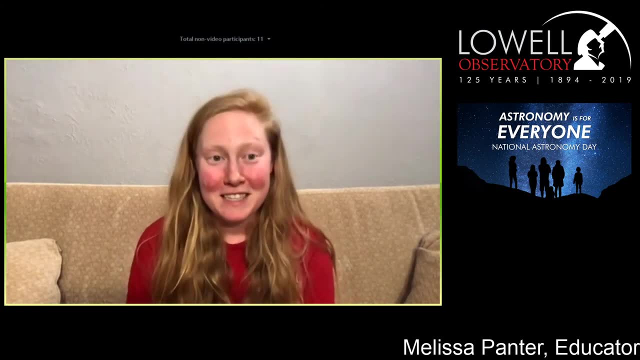 where you can go with, um, just your eyes, you or, uh, binoculars or the telescopes at lowell observatory when we open back up. it's just a really great time. so hopefully you get something out of my story of how astronomy has changed over the years, and i hope you all have a great day and i'll see you next time. 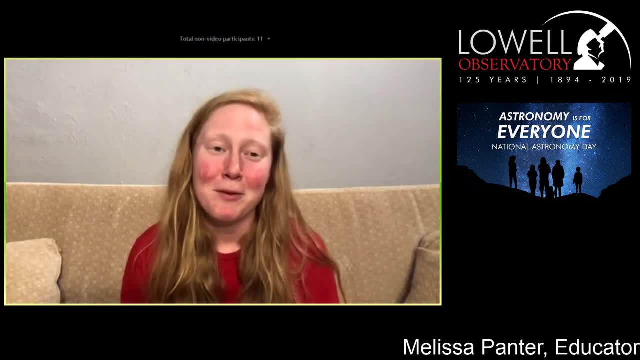 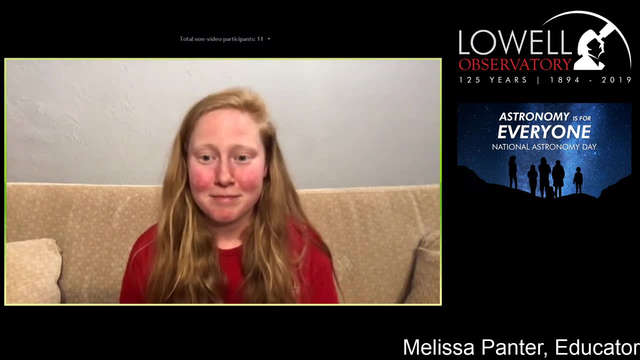 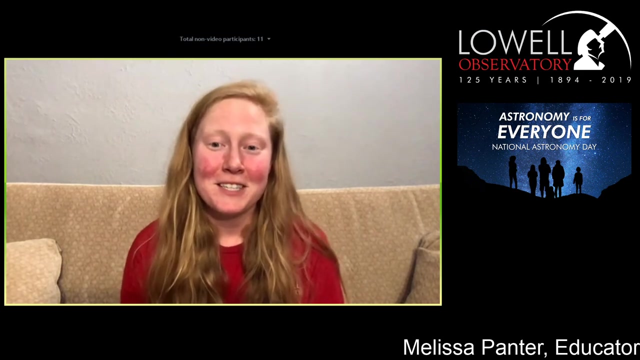 astronomy came to me. um, this has been awesome. i hope you all are having a happy astronomy day, um, and we'll see if we have any questions. yeah, so we're asking seeing if there's any questions going on. um, hopefully everyone is getting their fill of astronomy. 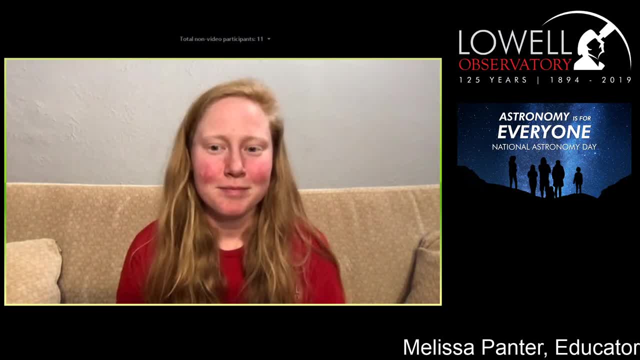 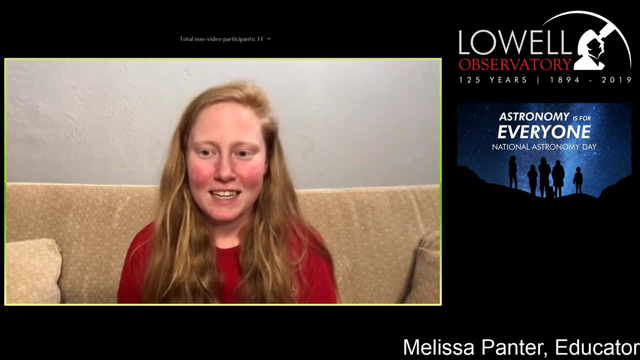 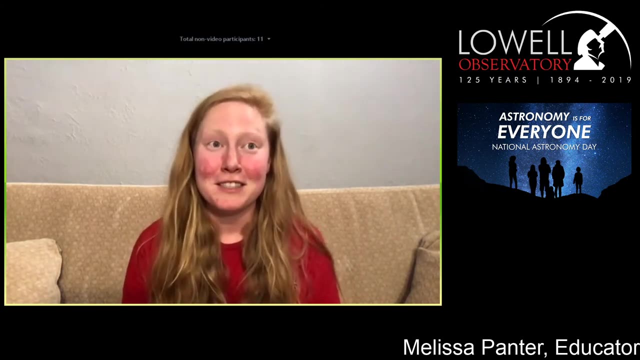 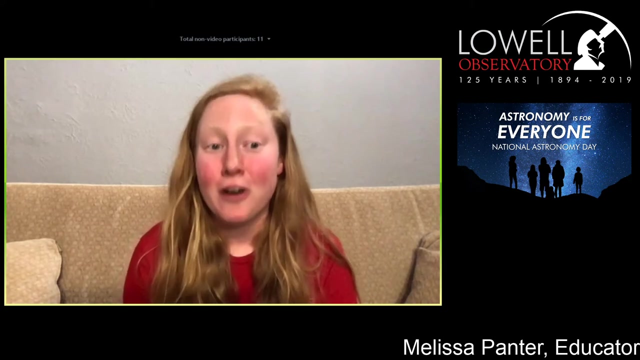 about 30 seconds seems really long. okay, it looks like we have one question: what gets me most excited about the universe? wow, summer, that's a good question. i think the thing that gets me most excited about the universe is talking, talking, not just talking with water. about the universe talking about. well, what are we seeing? um, i love exploring, just different. 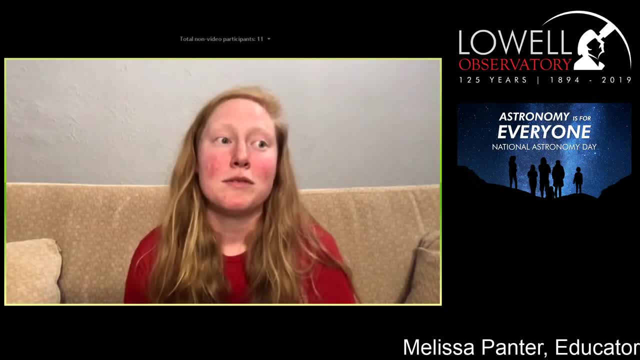 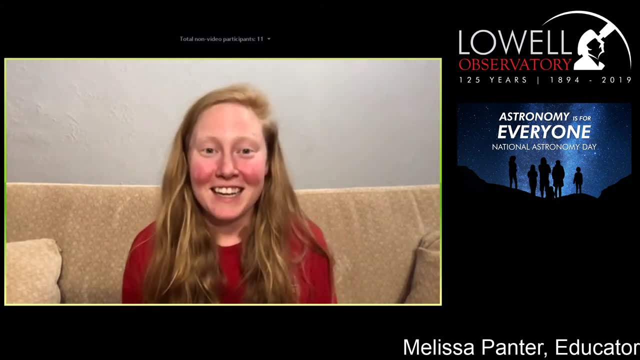 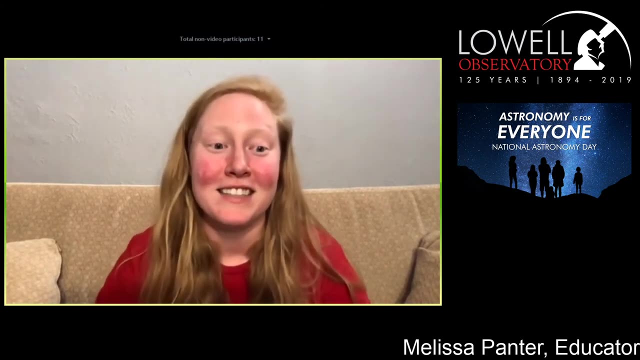 hypotheses. i love exploring, just by talking to each other, what could be out there. is there life out there, who knows? like that's just stuff that gets me really going. just it's this huge unknown that we're trying to understand as humans and exploring one step at a time, whether it's through. 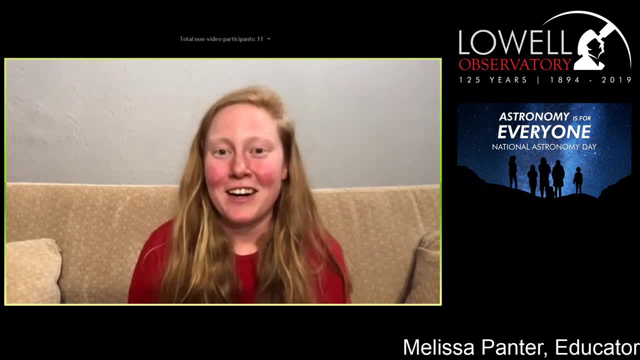 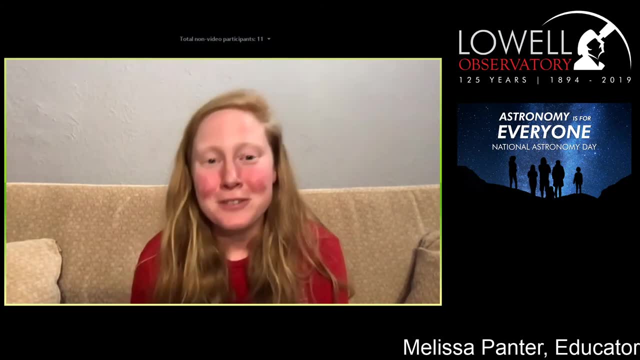 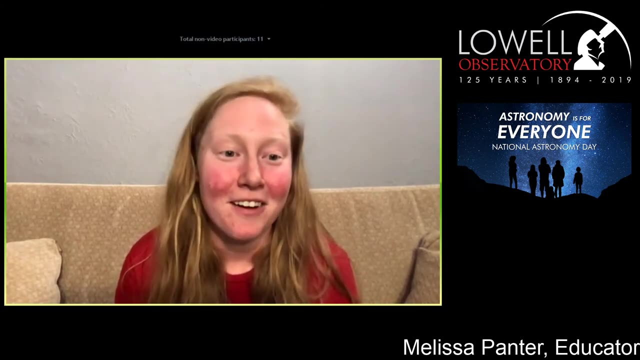 getting better telescopes and working on our turbulence in the night sky to make a clearer picture, or if we're looking at the gases that are creating new stars and dwarf galaxies. it's just really you can't go wrong, or how excited i'm gonna get with all of that. 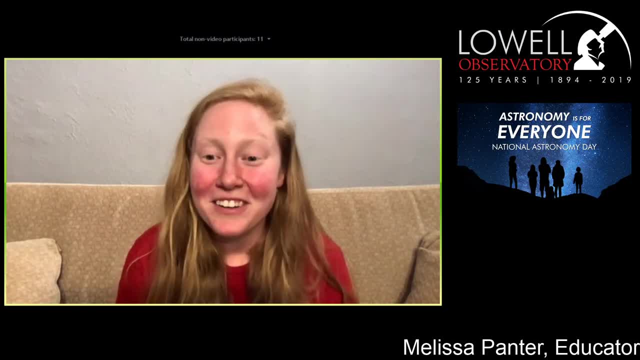 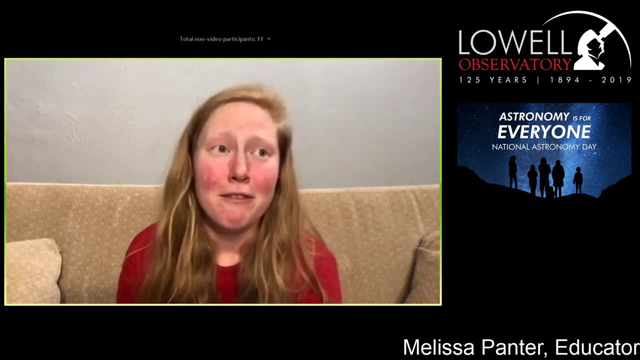 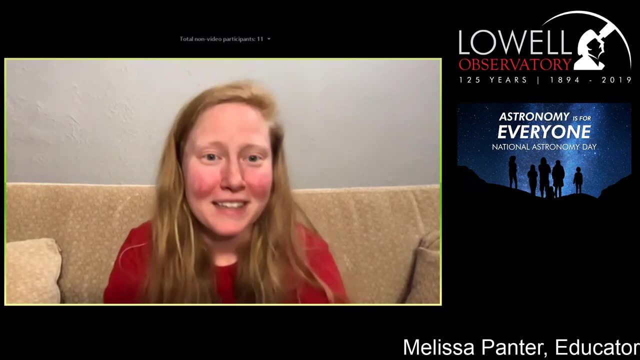 and then i have another question. was seeing the milky way for the first time, like seeing god, seeing the milky way for the first time? um, i didn't know what it was. i was like that's a weird cloud that's kind of just going across the. 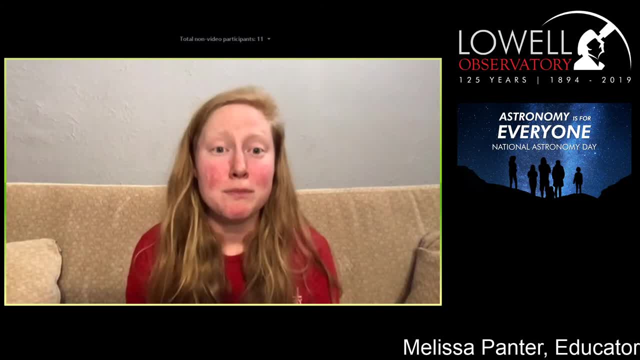 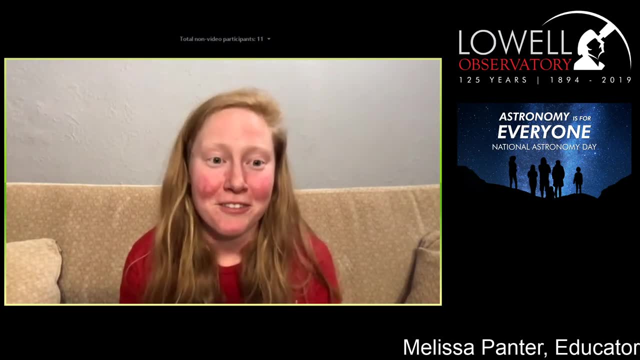 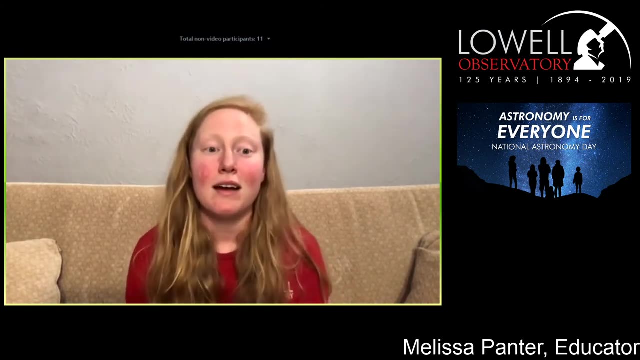 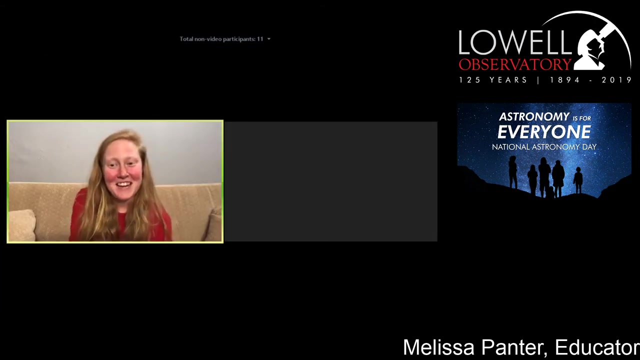 sky. um, it definitely spoke to my soul. um, it was a really amazing and humbling experience seeing that for the first time, kind of putting into perspective how many stars, how many galaxies, how many different things are out there. um, good question, jacob. thank you. that's all the questions i have. so, sarah, take it back. thank you, melissa. so, melissa, uh, just talked. 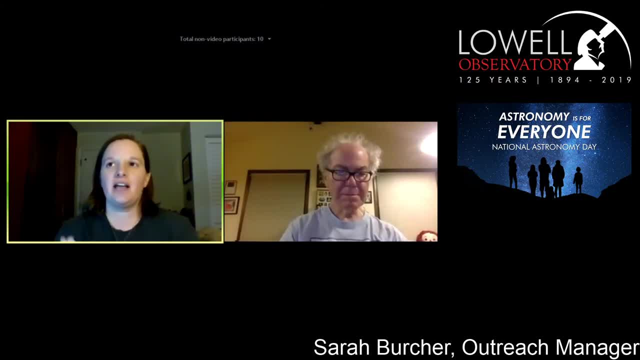 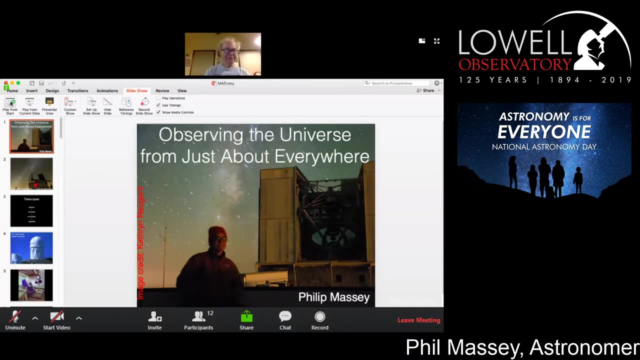 to us about how her perspective of the night sky, her perspective of astronomy, changed by seeing it from all over the us. i'm now going to introduce you to someone who's observed the night sky from all over the world. uh, and we'll see how that works for dr phil massey. take it away, hi, let me just get. 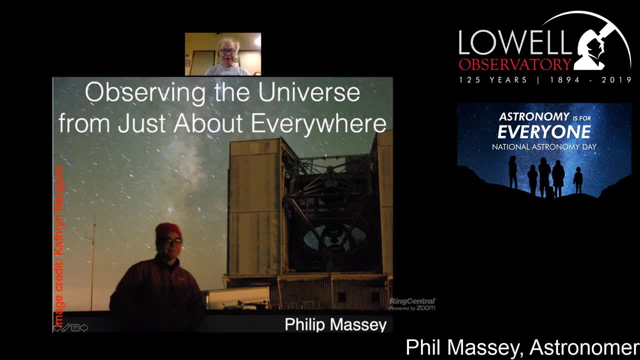 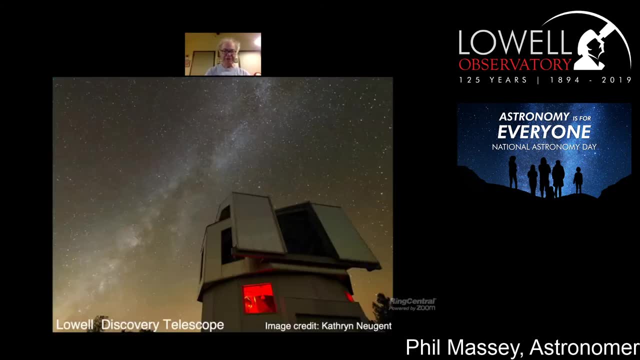 um. i'm phil massey. i'm an astronomer here at lowell and um. i am fortunate enough to be able to use this wonderful telescope, the lowell discovery telescope, and um. it has it's 4.3 meter telescope, it's very big and it's um has great instruments on it, and so why is it that i go anywhere else to? 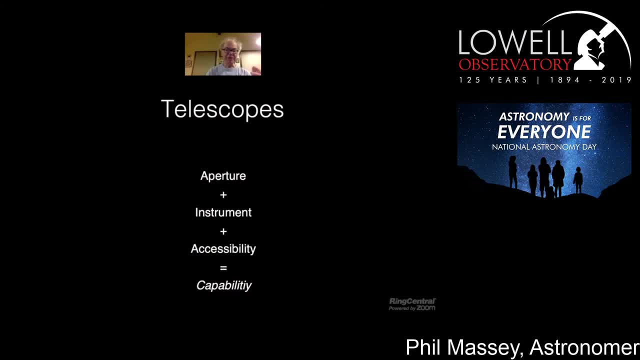 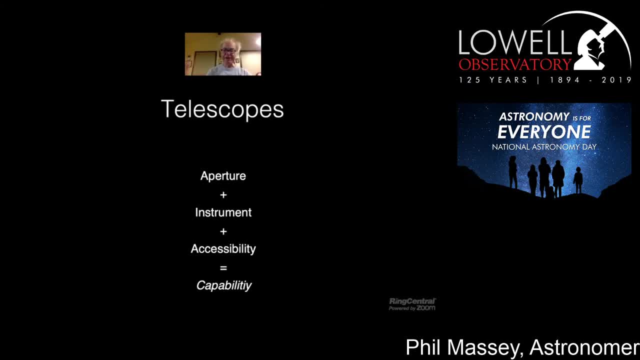 characteristics. one of them is how big the telescope is, and that's sometimes all astronomers talk about. when we talk about um a telescope, we often refer to it by its um- how large the mirror is- we'll say the 4.3 meter discovery channel telescope- and, just like a big rain barrel, collects. 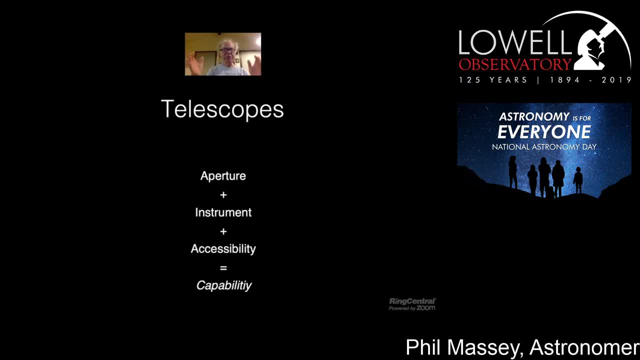 more water than a little rain barrel. a big telescope mirror will collect more light than a little telescope mirror or the opening in your eye, but, um, there's more to a telescope than just how big it is. there's also what instrument is on it, um, and there's an issue of accessibility. 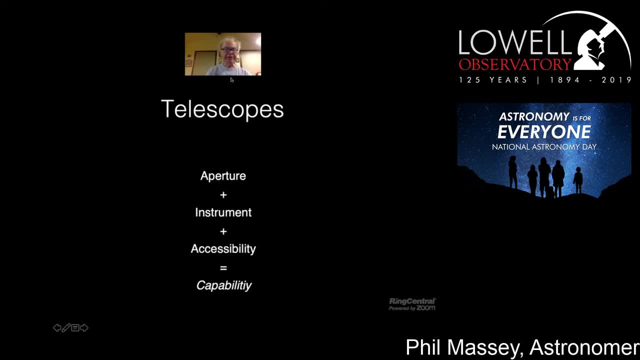 it may be that what you need to observe, you can only see from the southern hemisphere, um, and you need to use the telescope down south, um, maybe, um, you need to do a time series of something and you really just need half an hour every night, um, and that requires them to be. 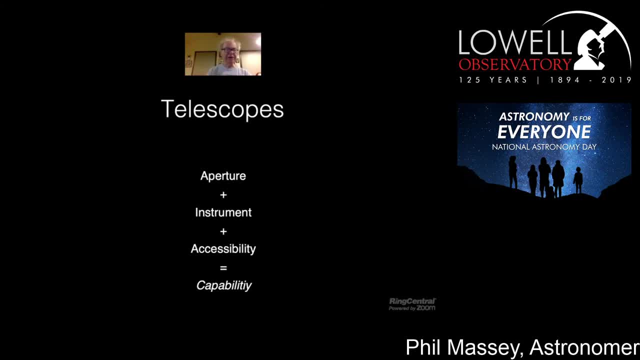 scheduled in a different mode than is usually done in telescopes, what's called q mode um. and so the combination of these three things- aperture and instrument and accessibility- is what i like to think of as capability. and so when my group um comes up with a project and we 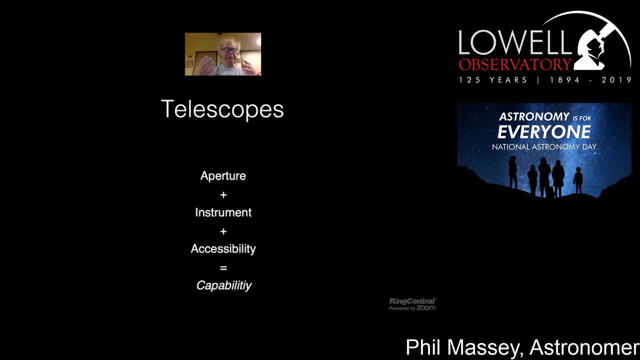 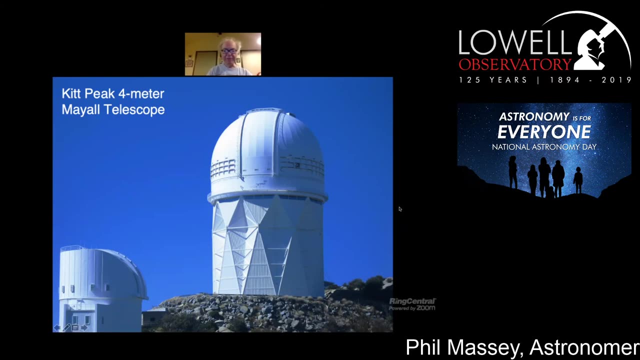 want to answer a question. we figure out: what capability do we need in order to carry out the project, and how do we carry this out? um, i'm going to start off by talking about a project i did 20 years ago, um, actually, and that's using the male forming your telescope to survey nearby galaxies- galaxies, they're still forming. 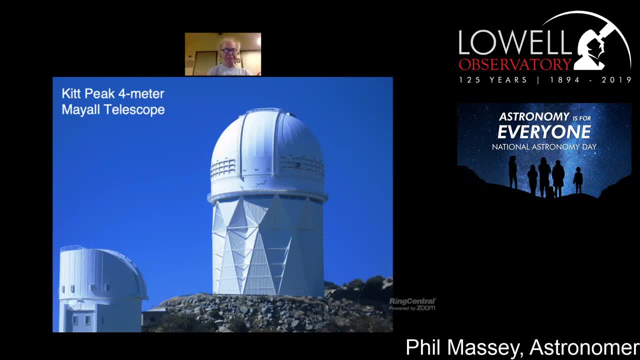 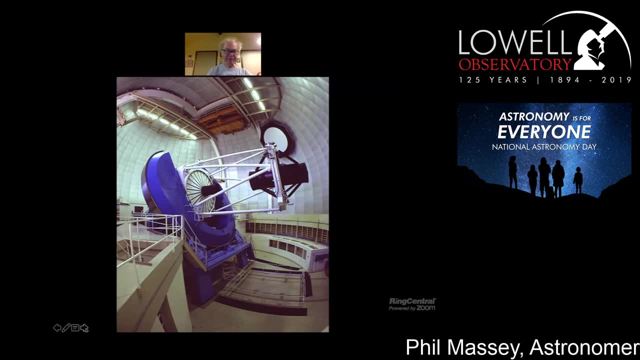 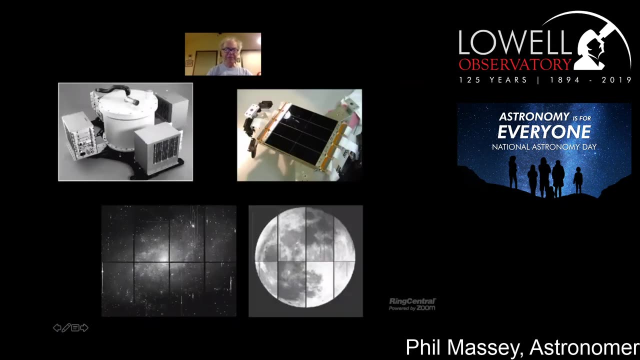 stars, galaxies like the andromeda galaxy and um other nearby local group um galaxies is fine telescope but for 17 years i helped look after, as a kid, peak um four meter telescope scientist um, and we use this remarkably remarkable camera, this mosaic camera that has um eight ccds on it and um when you took 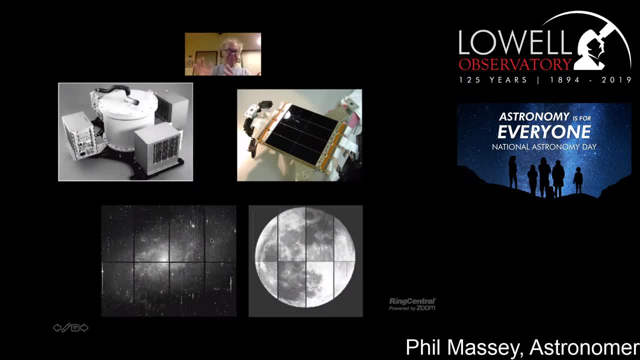 an image. you would, the image would. you would have these gaps between them, but that wasn't the bad thing about it. the bad thing about it was you basically had eight different detectors, eight different charge couple, devices that responded differently to light, and so the weight that, um, i calibrated this. it was about the time. 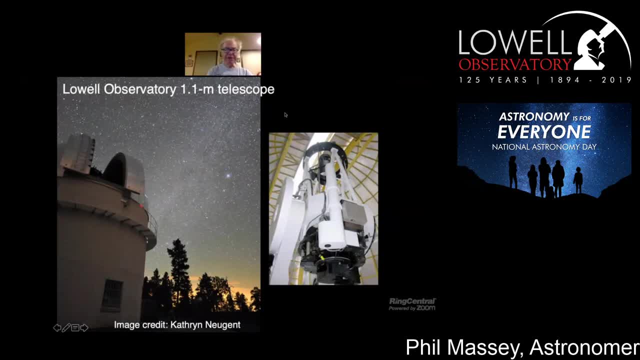 that i was coming to low observatory as an astronomer and i used this wonderful telescope here, the 1.1 meter out of an anderson mason, and i was able to get 30 or 40 nights on it and this allowed me to then compliment the data we had gotten on the roger telescope- the two of them. 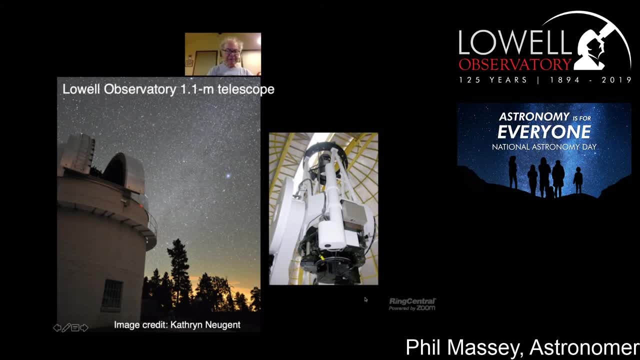 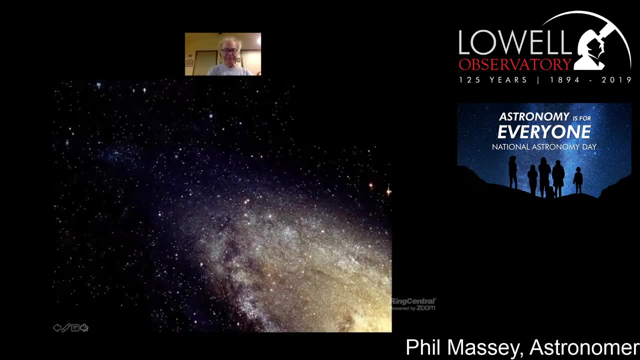 together were essential for doing um the. the two of them together were essential for doing um the science. a more recent example, and here are some of the great pictures we got as part of the survey. a more recent example: some of you may have seen the video I 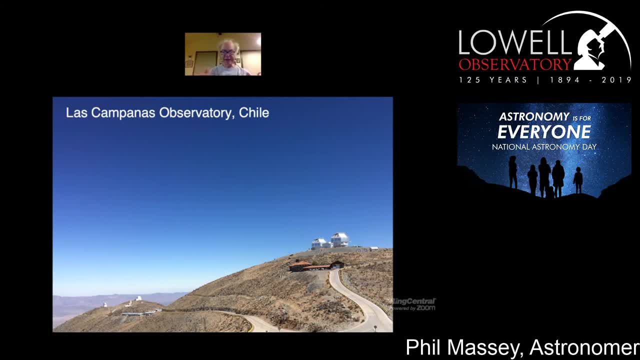 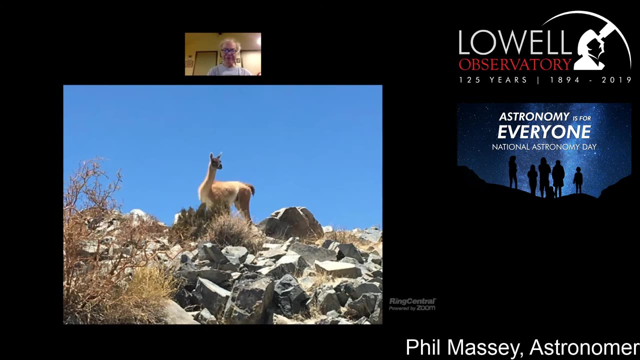 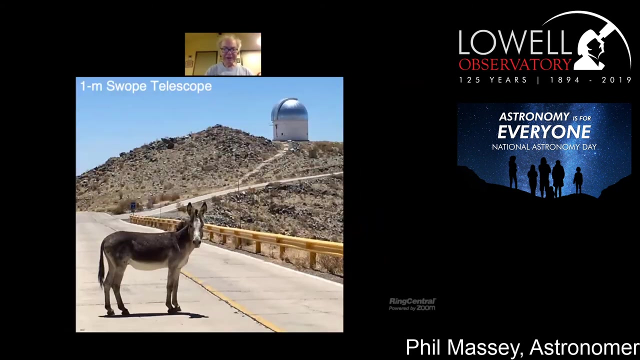 did a couple weeks ago on observing from Chile, and I just came back. we just finished a project, actually last week, from some data that we got in December and January. Chile is a wonderful place to observe. this is one of the inhabitants. it's a ganako. I have another ganako on my shirt and this is 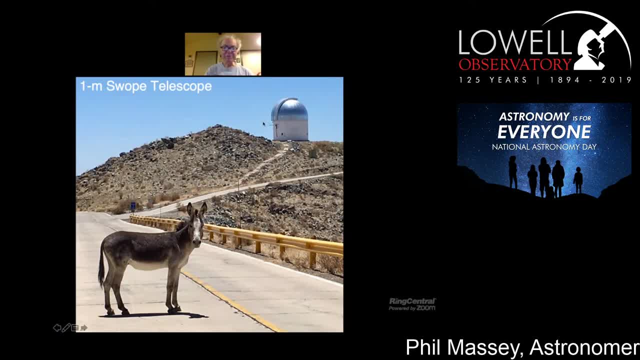 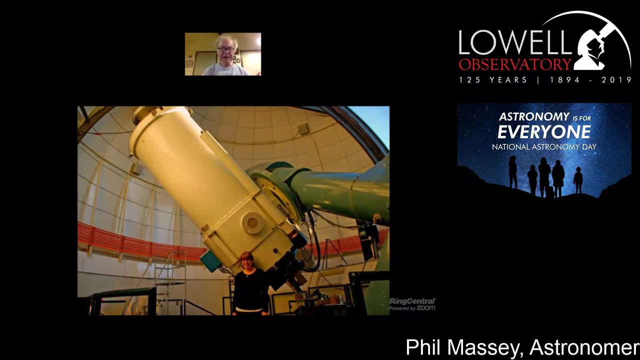 a burl and this is a telescope. we use the one-meter Swope telescope. we were looking for a particular type of admission line star and we use. here's a picture of my good friend and colleague, Katherine Nugent, for scale again. this is a picture of my good friend and colleague, Katherine Nugent, for scale again. 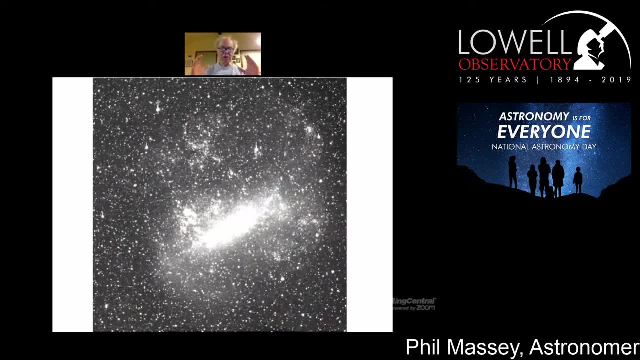 this is a picture of my good friend and colleague, Katherine Nugent. for scale again, this is a one-meter Swope and we wanted to survey all the. this is a one-meter Swope and we wanted to survey all the large Magellanic Cloud and the thing about the. 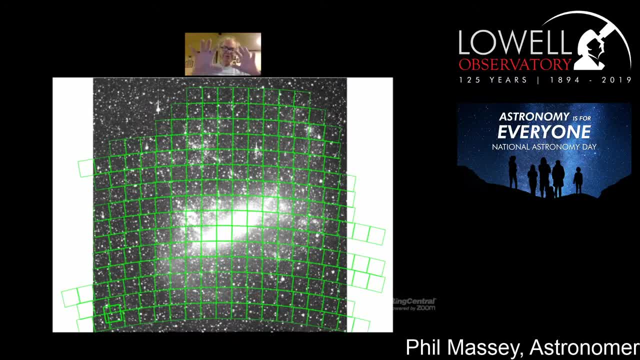 large Magellanic Cloud is. it's large, and so we wanted to look at lots of different very large area, and usually a smaller telescope has a larger field of view than the big telescope, and so we use the one meter telescope- not a gigantic telescope by modern standards- to do the survey. 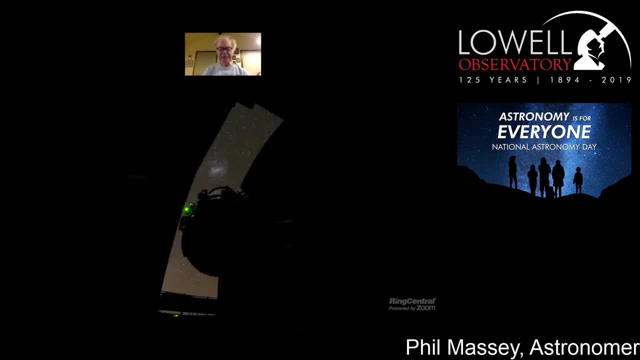 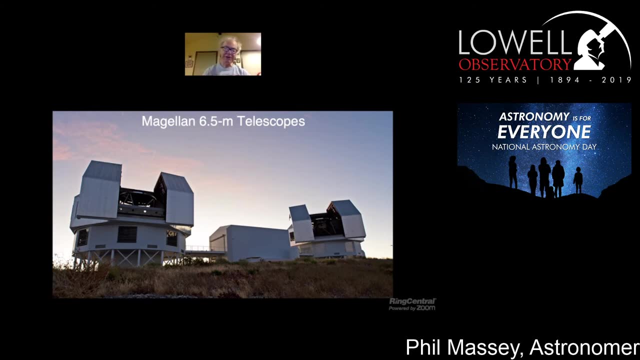 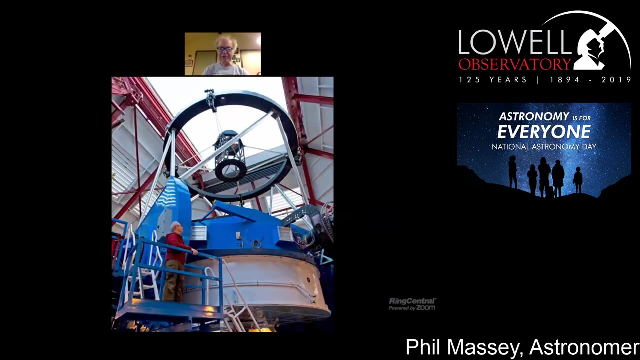 and then with the, and here we are observing the large Magellanic Cloud with it. and when we came up with our list of the mission line stars, we then came to this telescope, the Magellan six and a half meter, the particular one on the left, to take spectra of them, to see which of them were actually what we 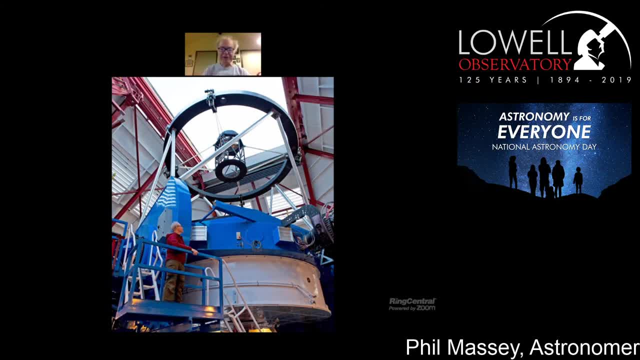 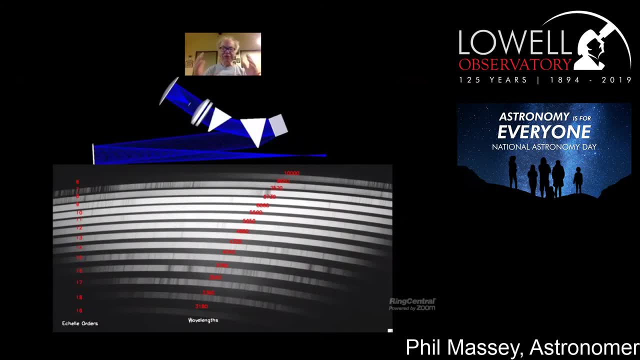 thought they were. it's a very large telescope, but the thing that really drew us here- and you can see how beautiful the sky is in Chile- what drew us here- was this remarkable instant mage, which takes light, breaks it up into the spectrum and allows us to get very high resolution data. all the 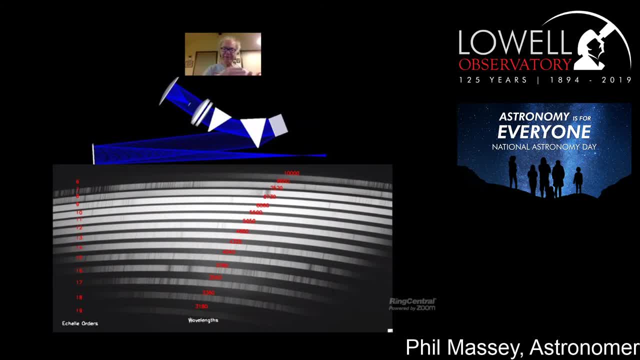 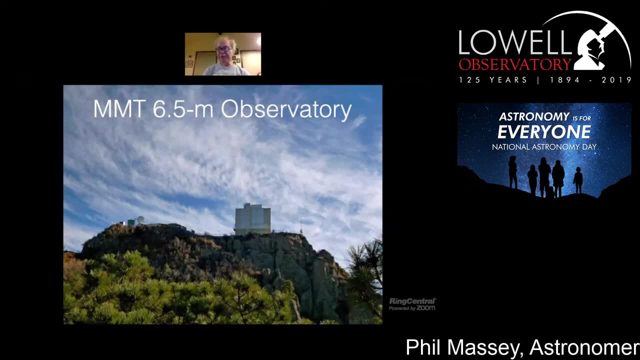 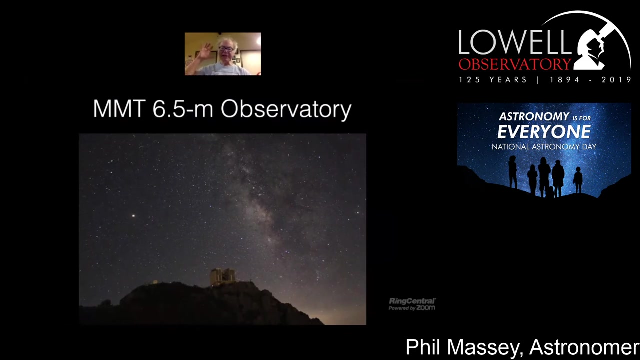 way from the ultraviolet- what just barely passes through the earth atmosphere- to the near infrared. another telescope that we've used to great advantage is the six and a half meter MMT down in southern Arizona. it's located on Mount Hopkins. here's a little video that shows the entire. 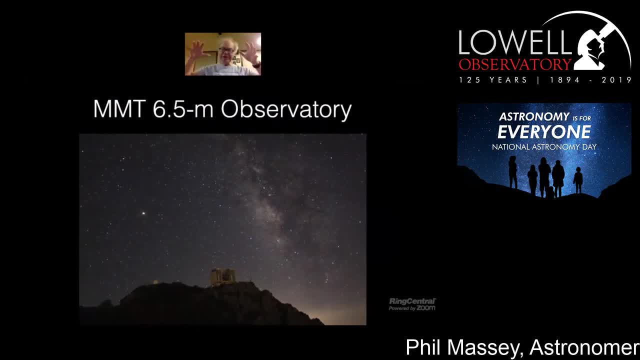 building turns. as you're tracking, the building is turning very slowly. as you move objects, which we're going to do in just a minute, you can see the whole building turn. it's located very near to Tucson but you can see that even though there's some light pollution there, the Milky Way is still spectacular- it has. 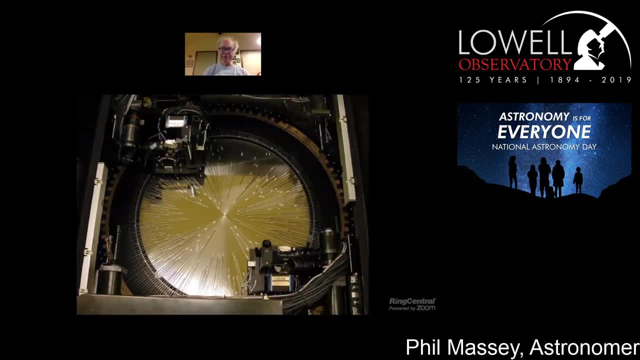 this very large six and a half meter mirror. but the most remarkable thing is this instrument. that's why we went to the MMT. it's the only telescope that we could do our projects with, because we wanted us to take spectra of stars across the face of M 31, the Andromeda Galaxy. it's a gigantic Galaxy, this. 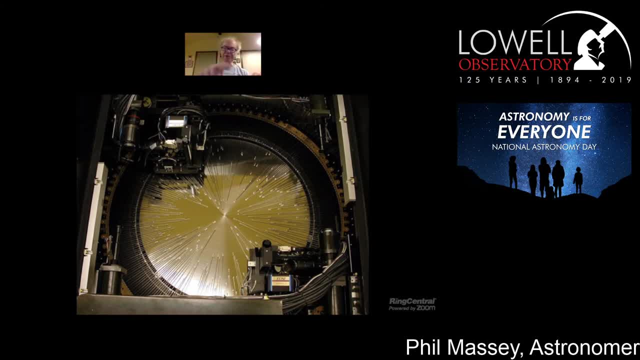 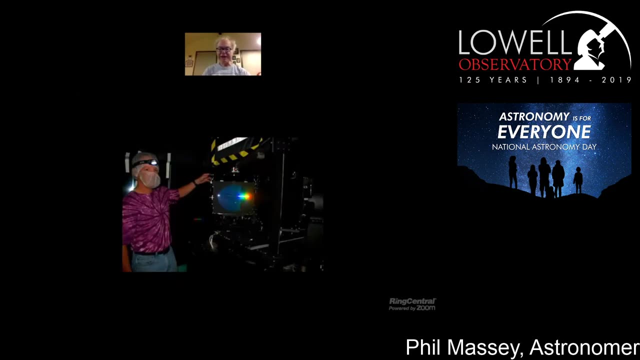 instrument consists of 300 fibers, with two little robots named Fred and ginger, and they dance around, moving fibers in just about 10 minutes to the positions where your objects are, And the field of view of this is a degree, And then these fibers carry the light down into a spectrogram. 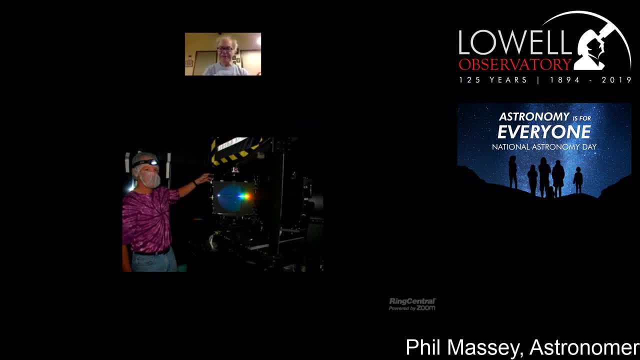 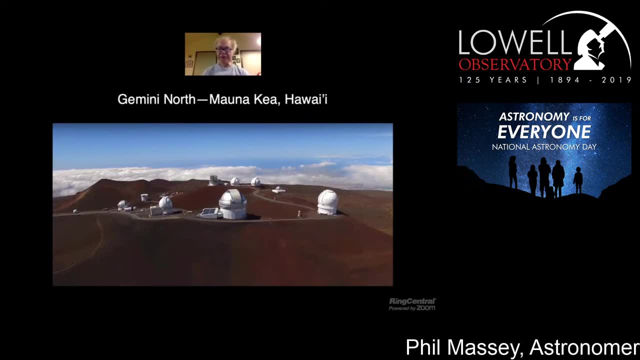 that's located a couple floors below the telescope. Another telescope that we've used recently is the 8-meter Gemini North Telescope, located on Mauna Kea. Now this telescope is usually scheduled in Q-mode, so that astronomers put in a proposal, they get, say, a night. 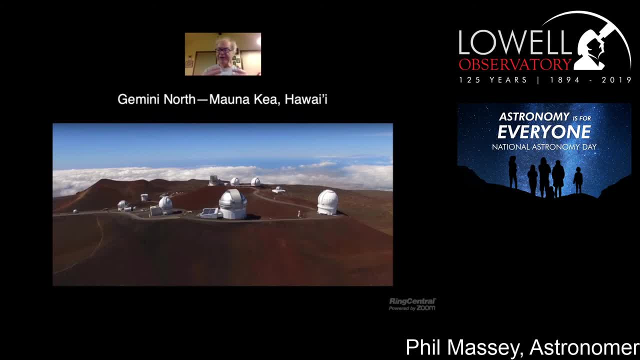 and they don't actually go and take the observations themselves. Instead, technicians and staff astronomers take the data for them, But we always like to take our own data. We think we're pretty good at it and it's a lot of fun. 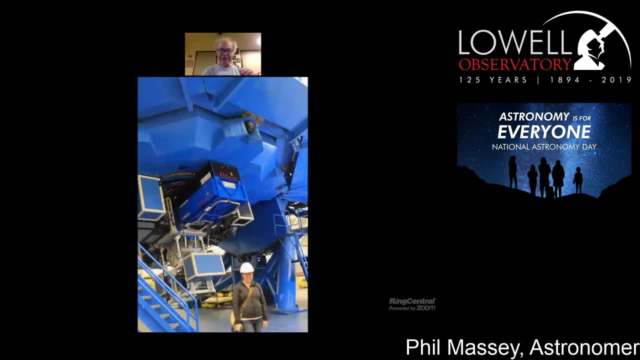 And so we actually got to visit the mountaintop. This is now Catherine Nugent, next to the instrument cube at the bottom, They have four instruments mounted. They can be always used. We used them the same night, just changing a mirror that diverts the light. 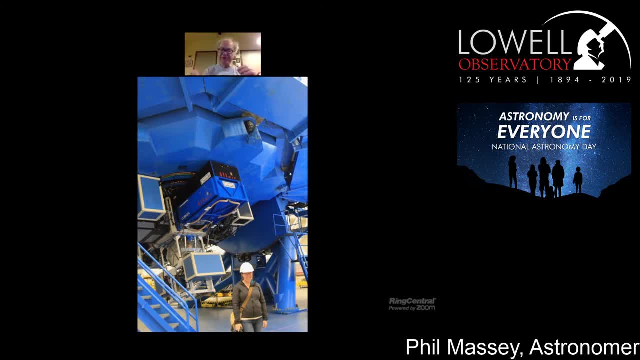 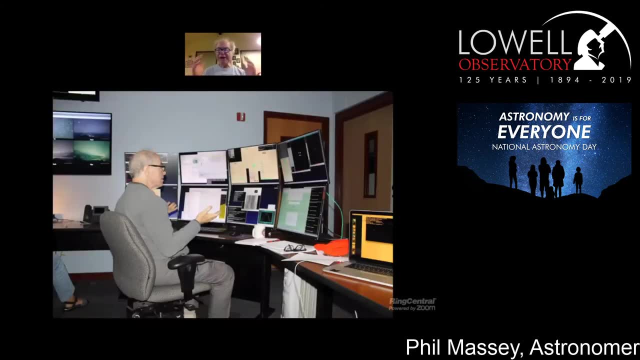 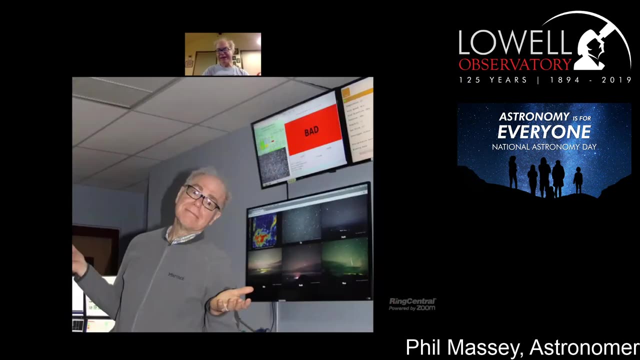 from one direction to one instrument or another instrument, So that's very suitable for then sandwiching in a whole bunch of programs. And during this time we got to be the cue observers And it's a pretty complicated system. You're running four different instruments and some of us were not that good at it. 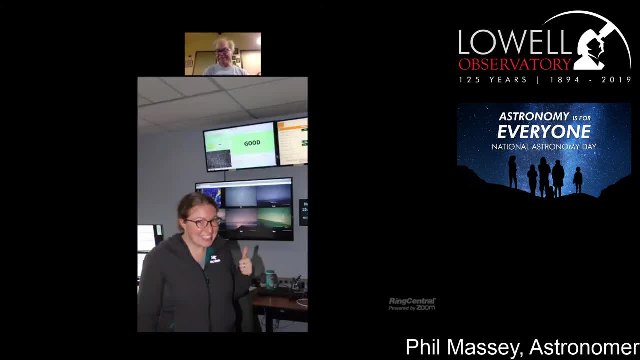 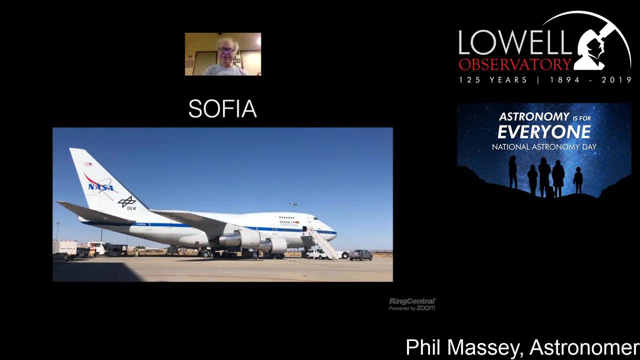 while others of us were actually quite good at it. Another telescope that we got to use recently is again often scheduled in cue mode, and that's SOFIA. It's a 2.7-meter telescope located in a 747.. 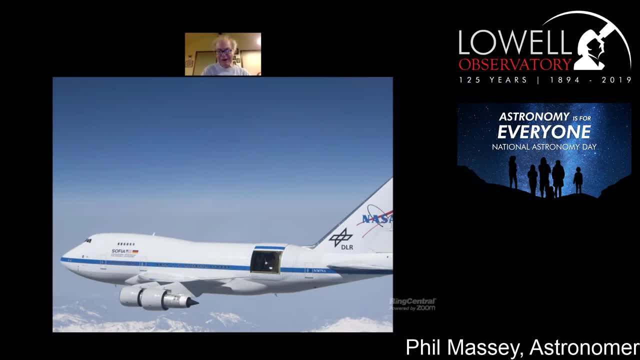 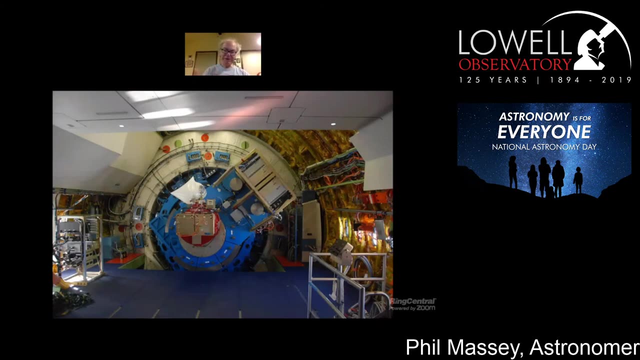 Here's a picture- This was not taken by us- of what it looks like with the chamber open. The telescope is in the rear of the aircraft and separated by an airtight seal. Here we see the back of the aircraft. This is where the astronomers actually are and the technicians. 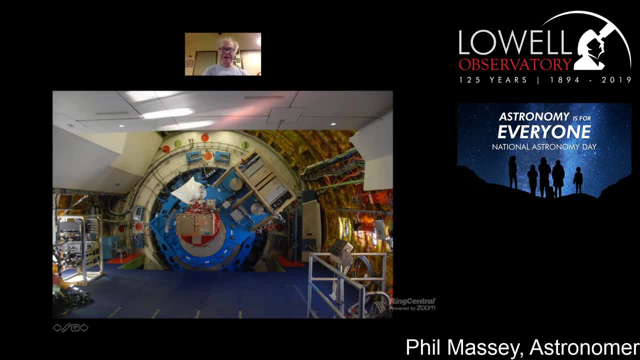 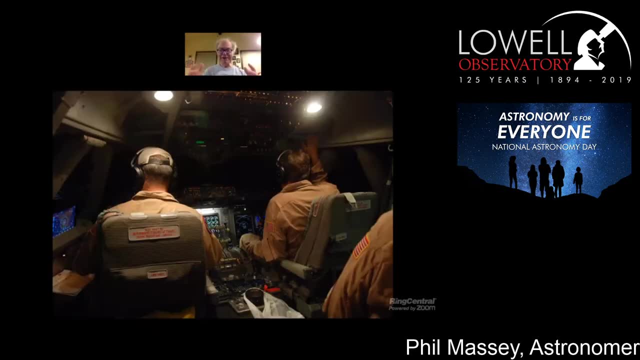 And we can see the instrument here mounted on the telescope. It's quite exciting. We got to go up and visit the pilot and co-pilot navigator while we're doing this. One of the amazing things about SOFIA is the telescope can move up and down. 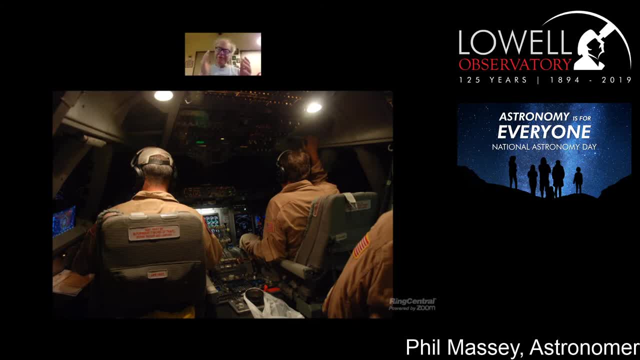 but it can't move left and right, And so in order to observe a particular object, the flight path has to be exactly in the right direction, and then you just change the elevation of the telescope, And then, as you observe another object, then the plane has to change and go in a different direction. 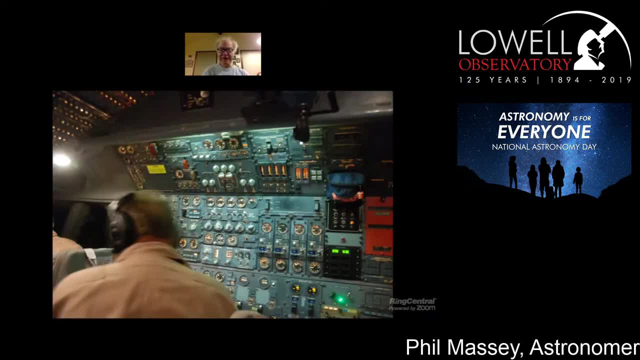 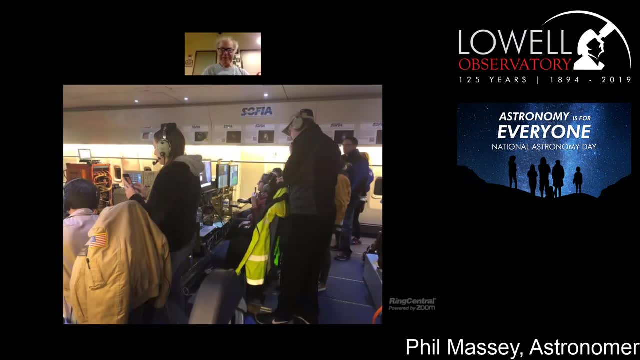 And, of course, all this is set up in advance. It's quite complicated. We were down with the – they often fly school teachers, Some of these are teachers and other public communities. Some of these are communicators, Some of these are technicians. 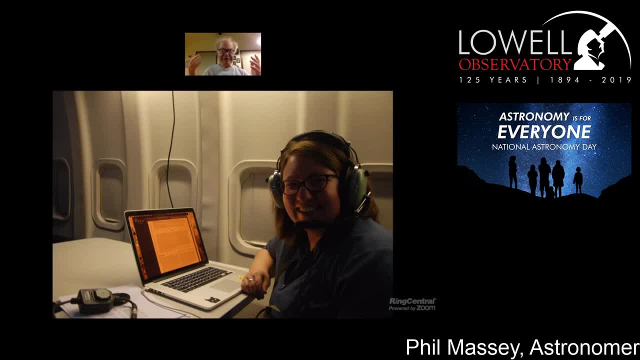 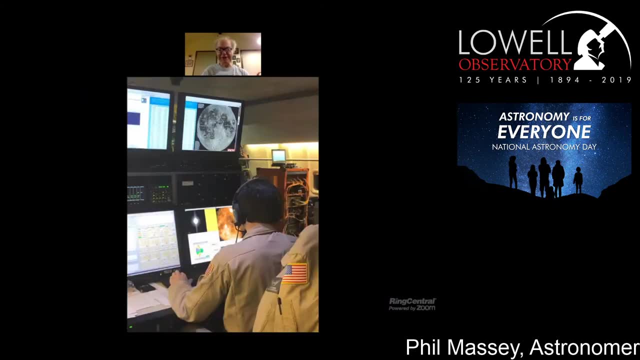 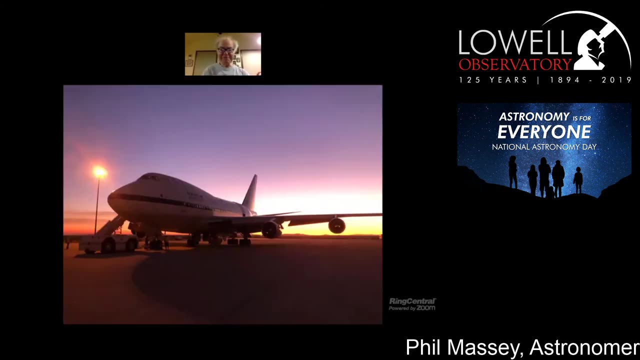 Some of these are astronomers. Here's Catherine, all set up for doing observations. We didn't actually get to observe any of our objects that night because of a last-minute schedule change, But we had a lot of fun anyway And we got to observe – we got to see them observe the moon. 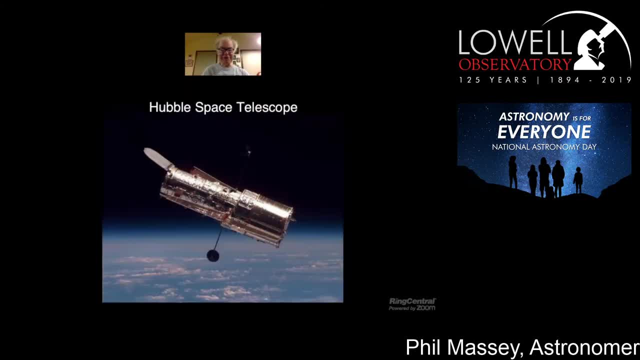 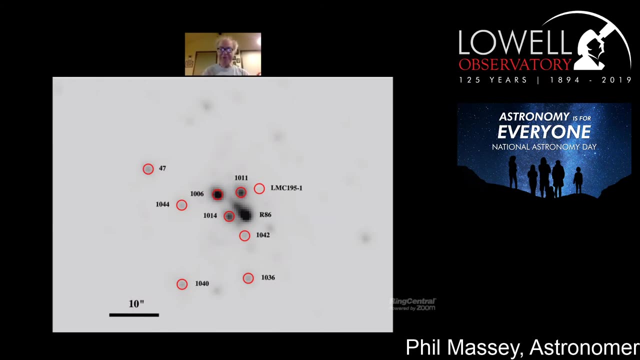 This is the plane as we were leaving in the morning. Here's the telescope that's always scheduled in Q mode. It's a 2.3-meter telescope, but it's location, location, location And one of the reasons astronomers like to need to use the Hubble telescope. 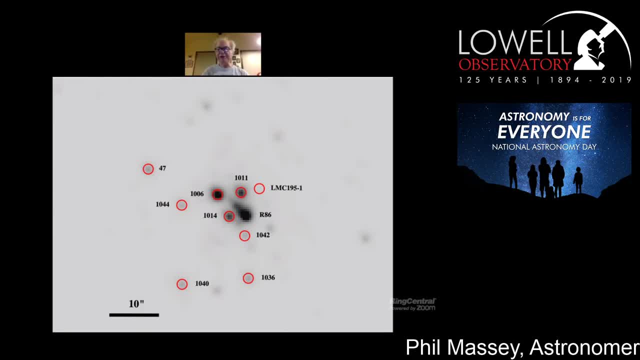 why we needed to use the Hubble – this is a crowded region in the Large Magellanic Cloud known as Luki Hodge 41,, which my summer student, Victoria Lager, has been working on. This is a ground-based image from the slope. 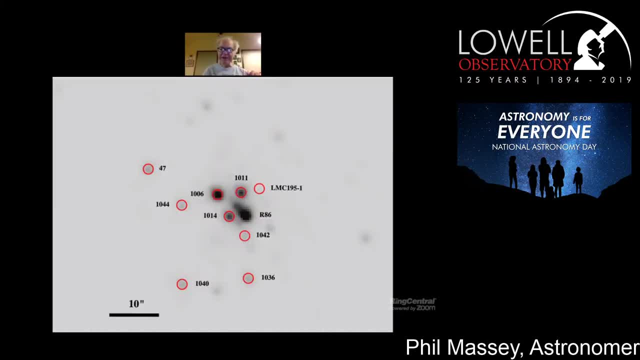 This is what it looks like. same field, exactly from Hubble, And you can see what appears to be just one or two stars here breaks into an entire little cluster of stars. It also allows us to do something you can't do at all from the ground. 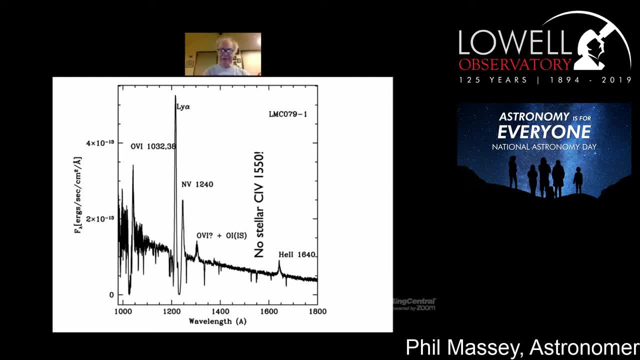 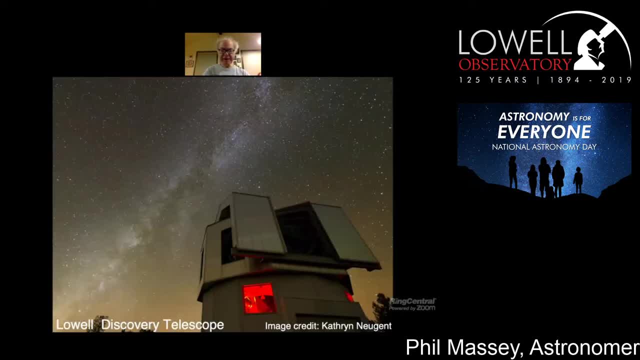 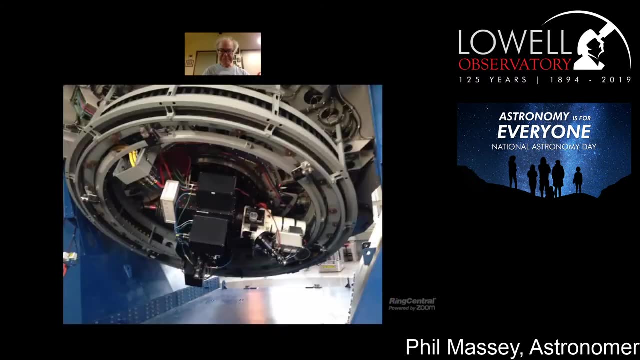 which is to take spectra in the ultraviolet. This is now far in the ultraviolet light that would never get through the Earth's atmosphere or try us. This now brings us finally back home to the Lowell Discovery Telescope. It has an instrument cube on it, just as Gemini does. 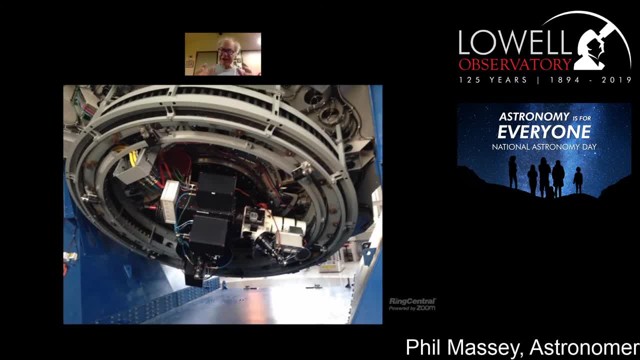 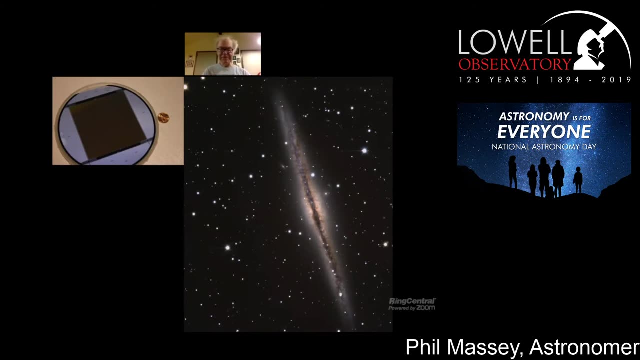 We can have any of five instruments active during the same night and just change from one instrument to another by changing the location of the little pick-off mirror. It has, in my opinion, the best CCD camera in the world on it. I am a little prejudiced in that I was PI for the instrument. 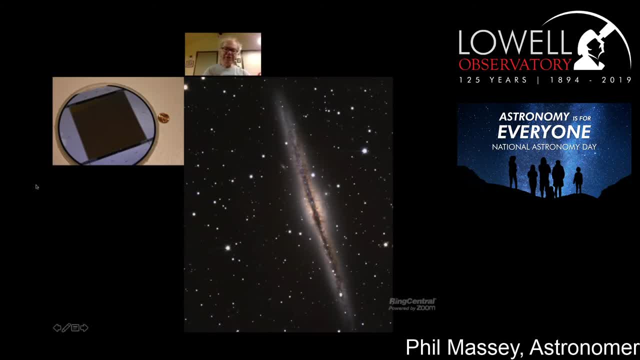 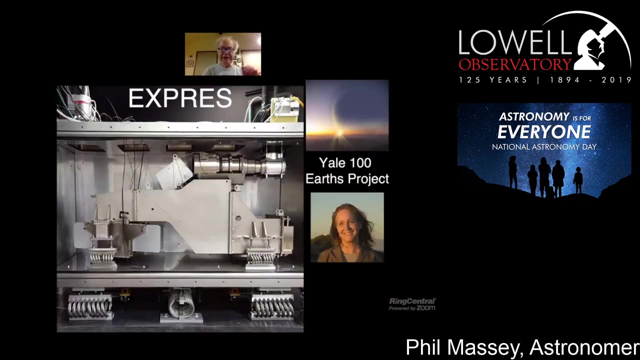 This is a large monolithic imager and you can see how large the CCD is. Compare it to a penny. Most large CCD cameras are mosaics. as I showed you earlier, This covers the same area as that mosaic CCD. But the instrument I'm really looking forward to using is this spectrograph. 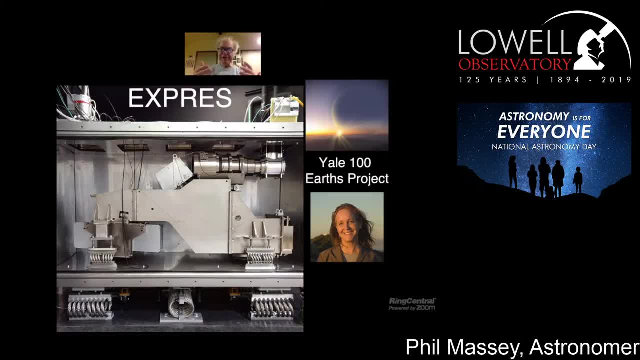 This is called Express and it's part of the Yale 100 Earths project that Deborah Fisher- Dr Fisher at Yale- is leading, And what Katherine Nugent and I are hoping to do next semester is look for red supergiants that have gobbled up a companion star. 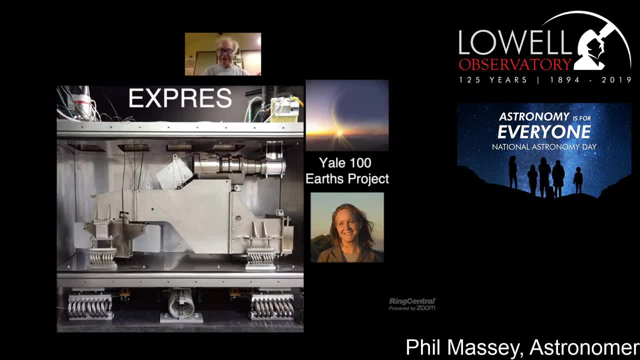 If they do that, they should be spinning faster than normal red supergiants. So that's what we're planning to do with the instrument. So that's why I observe not only at Lowell but at other places in the world. Thanks, 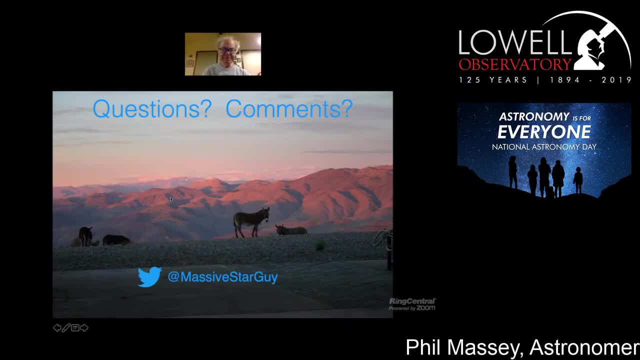 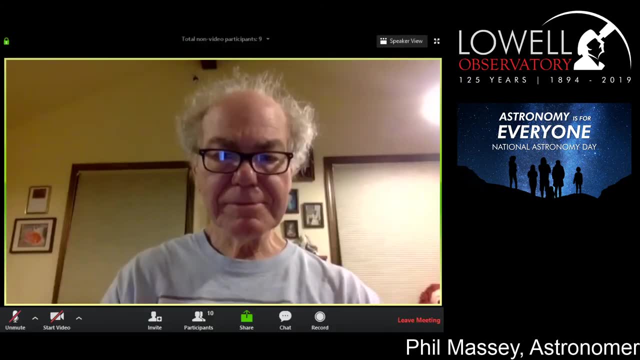 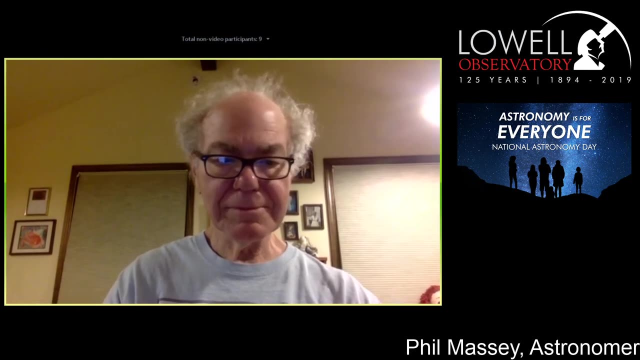 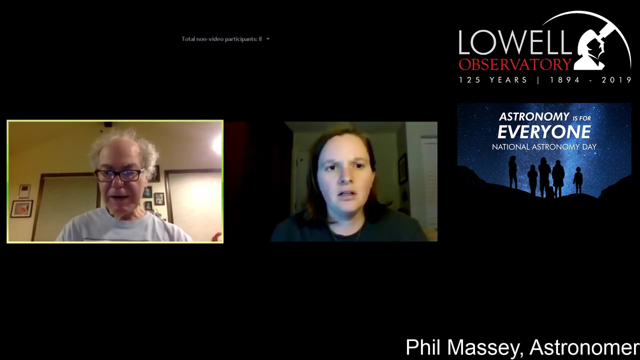 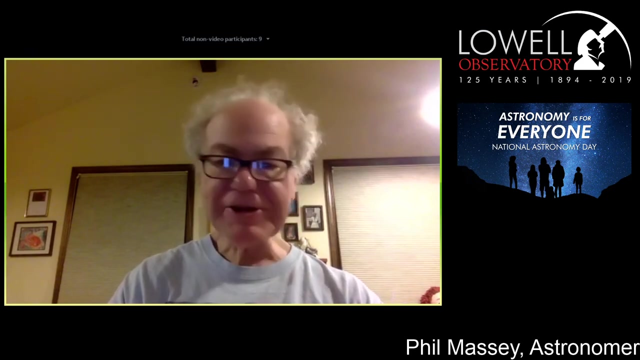 Let's see if there are any questions. Bill, are you able to see the questions coming up for you? I can see – there we go. What's my favorite telescope? I'm so glad you asked that There's a Zen koan about a –. 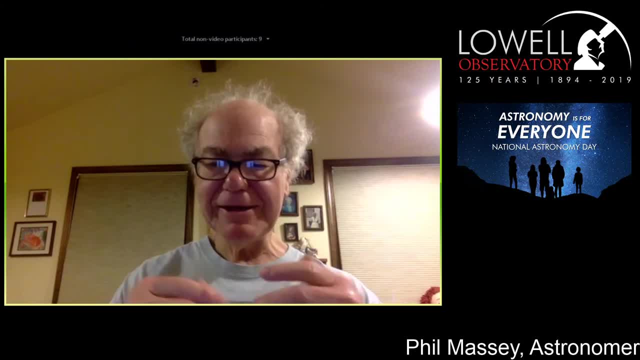 a Zen student that walks into a bakery and says give me your best loaf of bread, And the baker is very offended. He says: they're all my best. I love observing in Chile. I love using the Swope 1 meter. 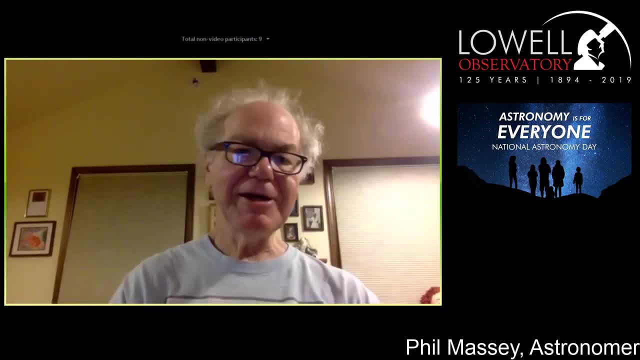 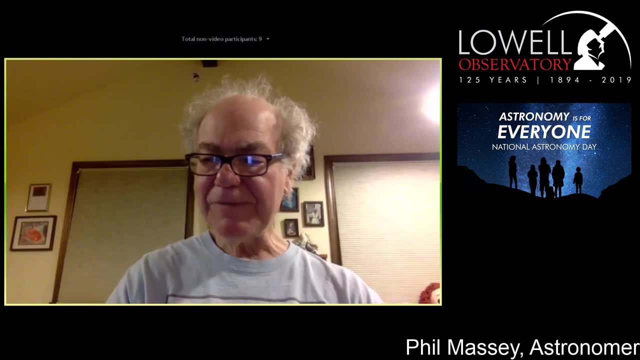 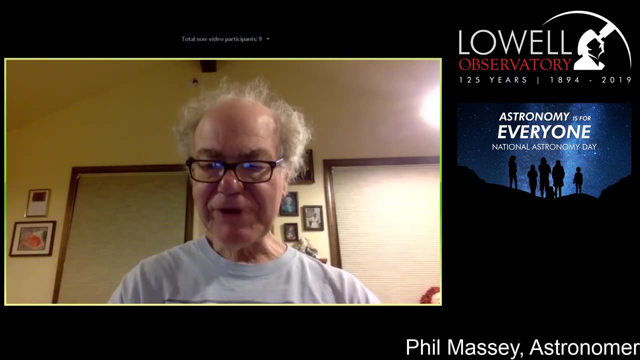 I love using the Magellan 6.5 meter. It's so great to be able to just drive an hour and use the Lowell Discovery Telescope. Sophia was an amazing experience. I'm not sure I would really want to do that again. Gum and I, that's so-so. 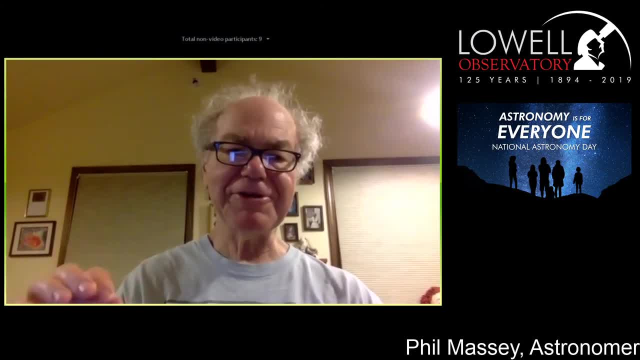 I can tell you, my least favorite telescope is probably the Hubble Telescope, simply because it's so difficult to get observing time on it that I find that for me I have to write the same proposal and rewrite it for usually three to four years in a row. 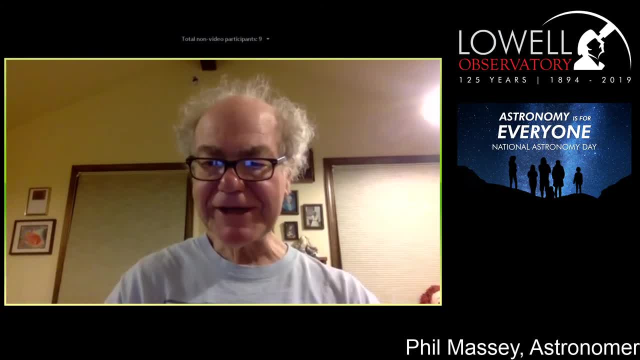 before we actually get the observing time, So that's a little tedious. How badly does Starlink – interfere with your telescope's long exposure imaging? Well, that's a good question. I was kind of oblivious to the whole Starlink thing until I was observing in Chile in December. 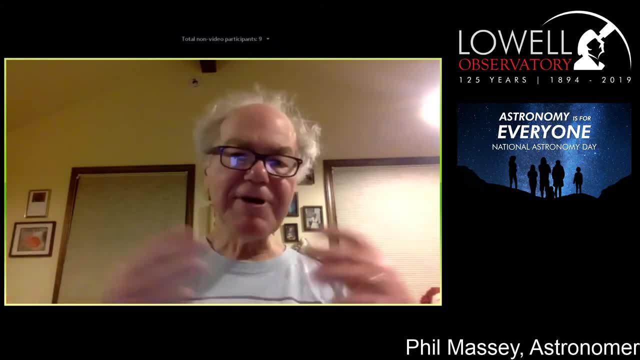 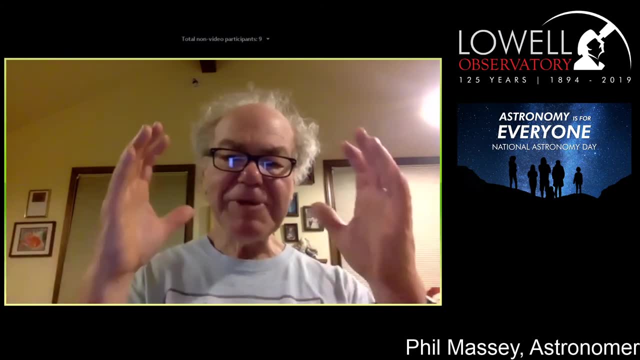 And I'm looking at the Magellanic Lens, which is as far away from the ecliptic and the equator that you get. You just don't have satellites passing through there. And then the five-minute exposure. I had three of these darn things go through the exposure. 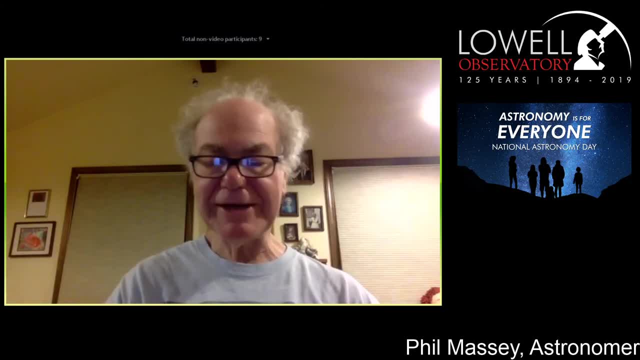 I had to throw out the image and – and take another. I think all astronomers are concerned about this, And it's one thing now when there are only a few hundred of them. it's going to be even worse when there are thousands. 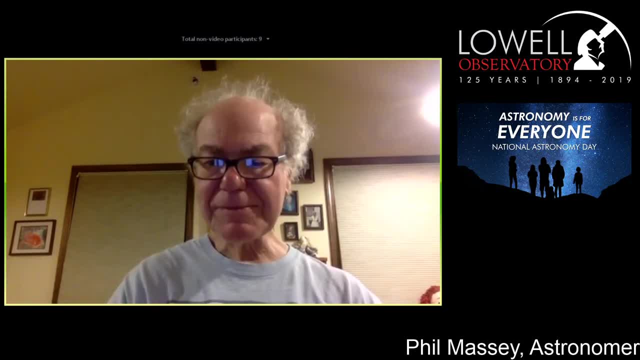 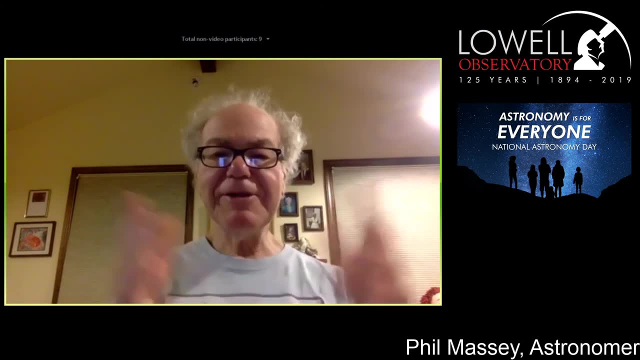 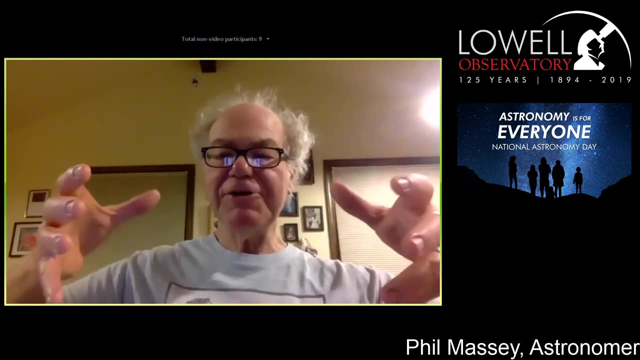 And so that's an issue, Sophia. So Jacob writes: why can't the telescope move left and right? Well, you can imagine that there are pretty tight constraints. right In a normal observatory you have a telescope that can move all the way to the zenith and back. 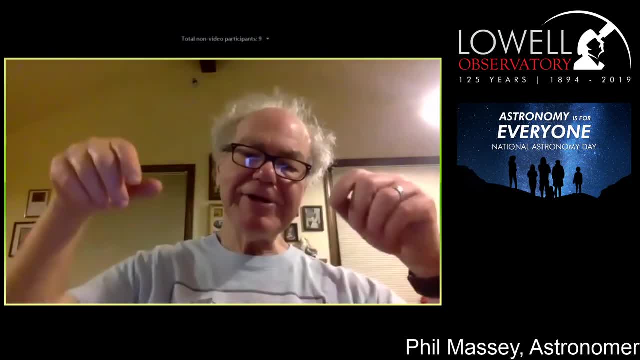 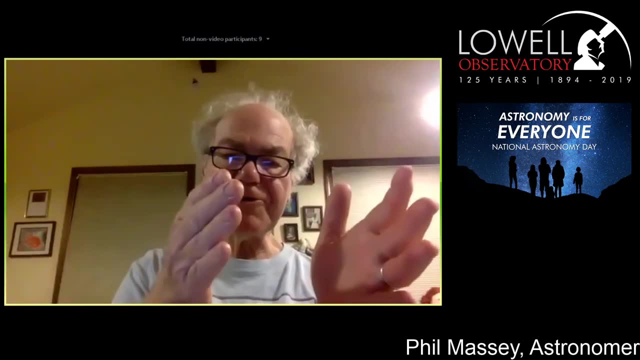 and all the way around in a circle. But you can't go all the way around in a circle. You don't have the ability to look all the way. If you turn very far to the left or to the right, you would be looking at the tail of the plane. 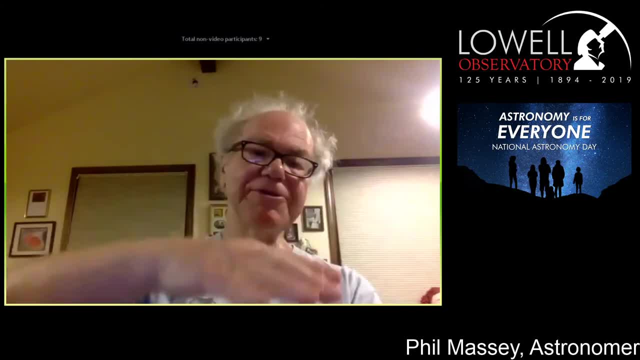 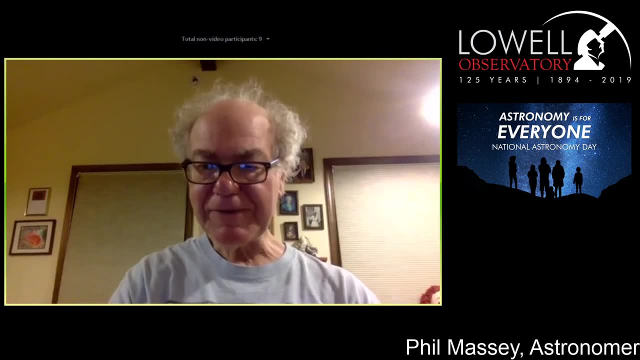 or the front of the plane, And so, because you're restricted to this one opening in the side, that's why they have to alter the flight path or the tubes or something. What telescope location was your favorite and why? I think we've touched on that. 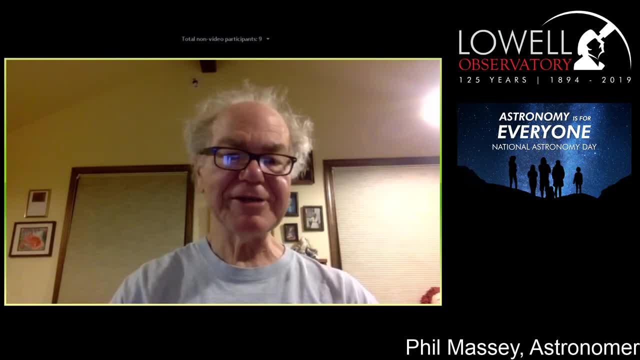 I do love going down and observing at Las Campanas in Chile. The people there are wonderful people. Our good friend and collaborator, Nydia Moral, is there. It's always fun to talk with her. And how does the moon look like? using Sophia? 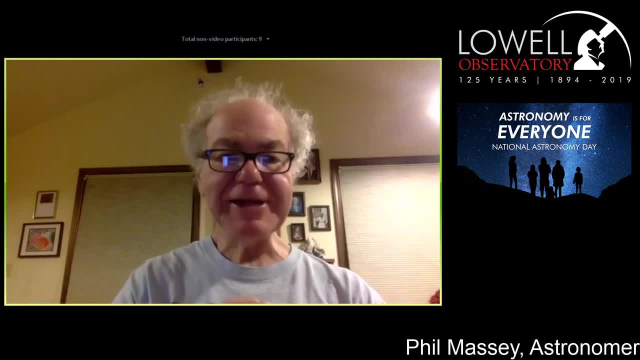 Well, it's observing. They were taking spectra in the infrared for reasons that I remember, but I'm probably not allowed to talk about because I don't know if this is actually published yet or not, And so we were simply seeing a visual image on the guider. 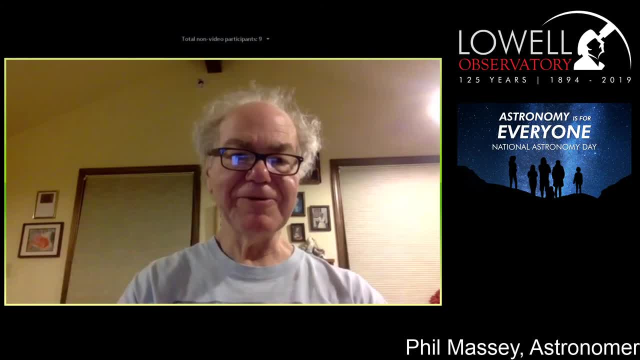 and then they were taking infrared spectra And so we saw infrared spectra and their wiggly lines. So maybe let's see three or four waiting period for Hubble. Why so long? It's because the oversubscription with Hubble is 10 to 1.. 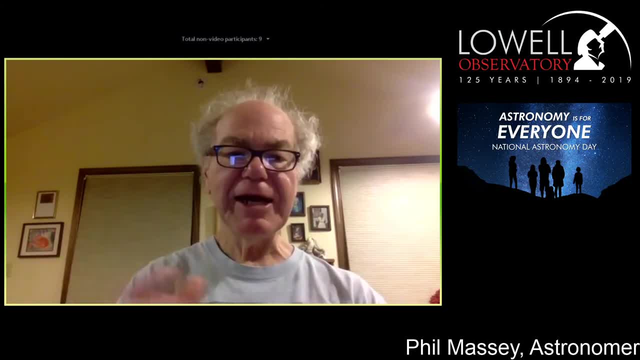 There's no other telescope that can do what Hubble can do, And so there are a lot more people with really great projects and great ideas than there is available time. Do astronomers get individual use time or as a group, from your location? No? 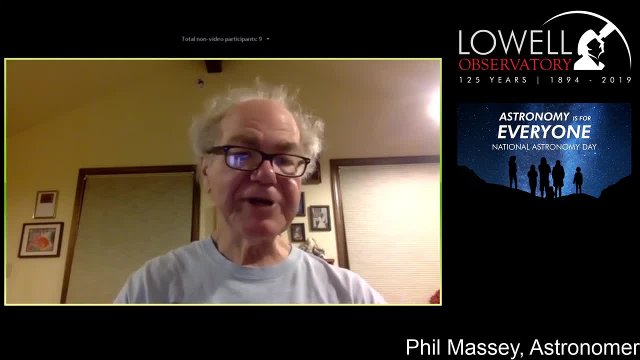 Say, for instance, at Lowell Observatory, there are about 15 astronomers, and most of us do not overlap very much in what we work on, And so I have a team, but that team is distributed throughout the world, And so our group will apply for time. 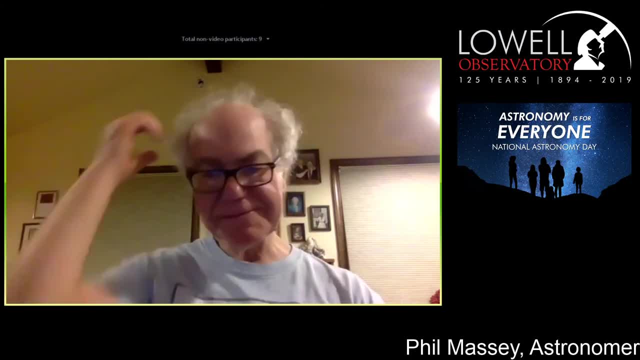 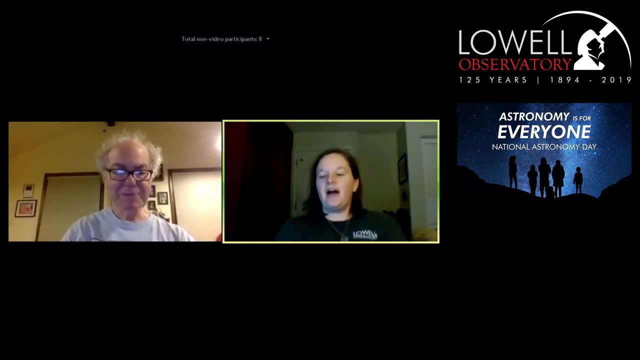 But it's not local to Lowell. I think those are all the questions and I'm going to turn it back to you, Sarah. All right, Thank you, Phil. So we are going to switch gears once again. We've talked a bit about professional astronomers. 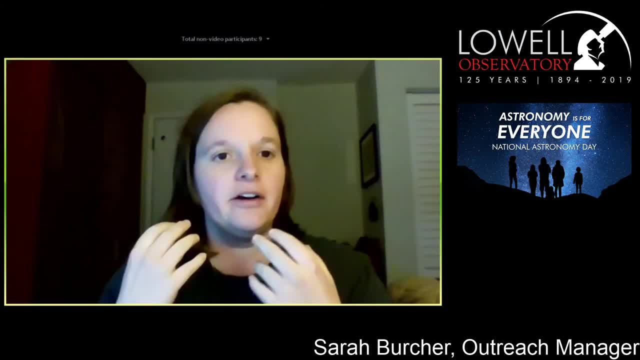 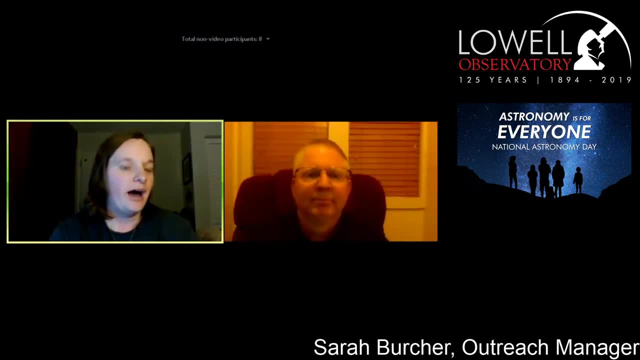 We've talked about those of us who educate in astronomy and our Lowell Observatory historian, Kevin Schindler. He is going to come and talk to you about Robert Burnham, Kevin. I'll let you talk about why he was such an interesting person. 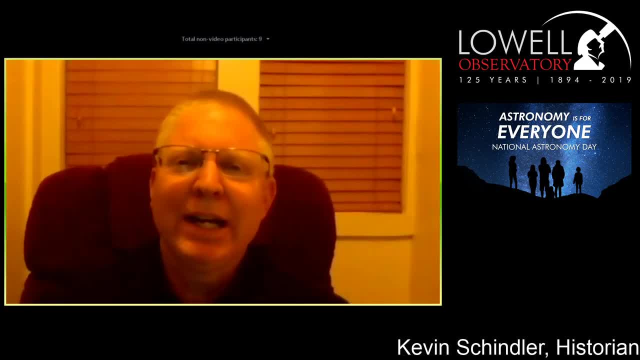 Sure, Thanks, Sarah, And it's really great to talk to everybody tonight, And I'm struck by listening to everybody's talks. There are really a couple common themes that go through everything we've been talking about tonight, And one of them. 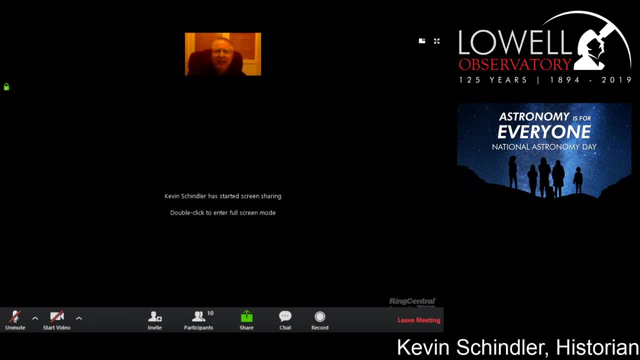 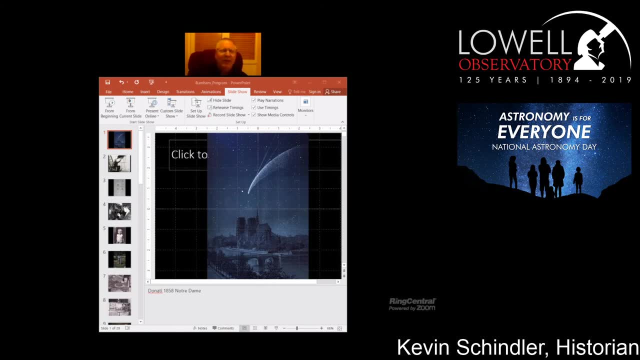 I'm going to start my program here. One of them is passion. I think we're all so passionate about astronomy And I'm just checking Sarah to make sure that's coming up. I think it is, Yeah, coming up. 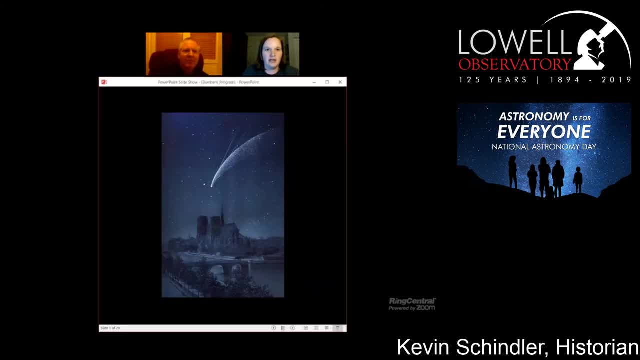 go ahead and hit your presenting thing, the from beginning guy, And then you should be good. How's that Looks good? So you know, I found out, Percival Lowell started his passion for the observatory back when he was three years old. 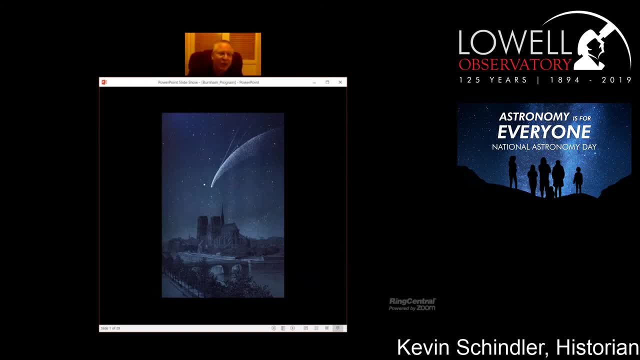 A comet named Donatje's Comet was up in the sky- And this is actually a picture of it- over Notre Dame in Paris, And Percival Lowell saw this And later in life he remembered this is how he got interested in astronomy. 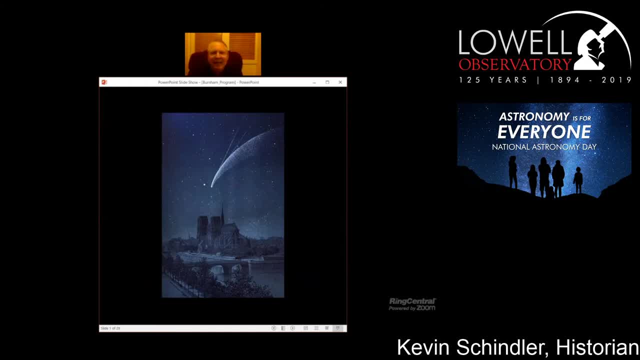 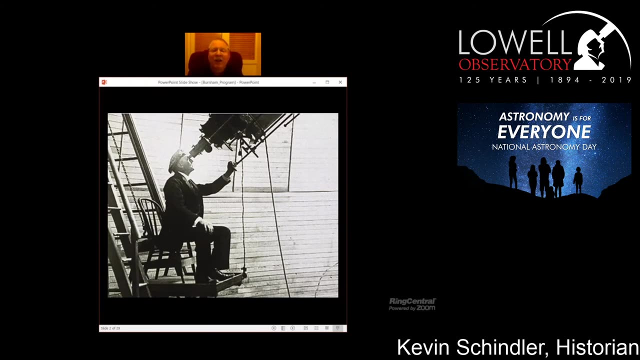 He said. I still remember the small boy inside of me in the staircase, gazing with all his soul where the stranger stood. That inspired him to go into astronomy, And he did this with gusto. He bought a telescope for $20,000,. 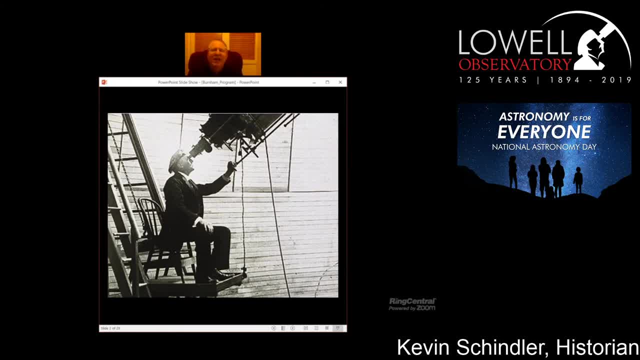 established his observatory up here in Flagstaff And that passion he started really has continued with, of course, not just astronomers and educators and others of all but people around the world, That whole thing about history repeating itself. You know, Percival Lowell came here. 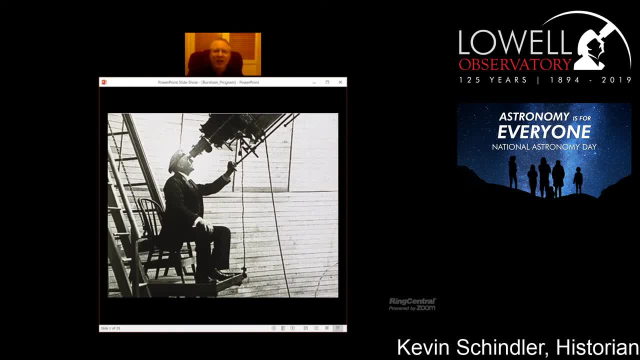 built one of the best telescopes in the world and did astronomical research. Well, 50 years after that, you know, telescopes are getting bigger. This telescope he's with here was, by modern standards then, getting kind of small, And so the observatory. 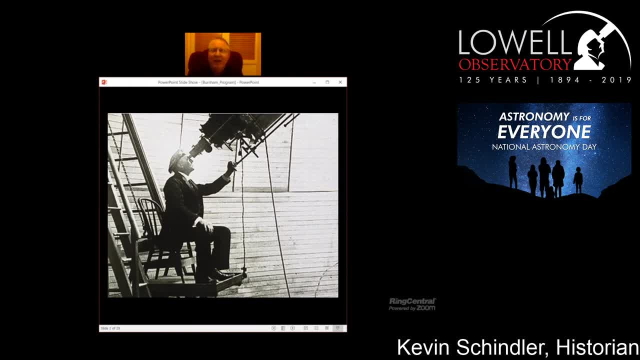 acquired the Perkins telescope that Gerard talked about earlier and made just really great discoveries. The technology is improving. It's time to get another telescope, And the leadership of Lowell built what we know today as the Lowell Discovered Telescope, And I should point out that 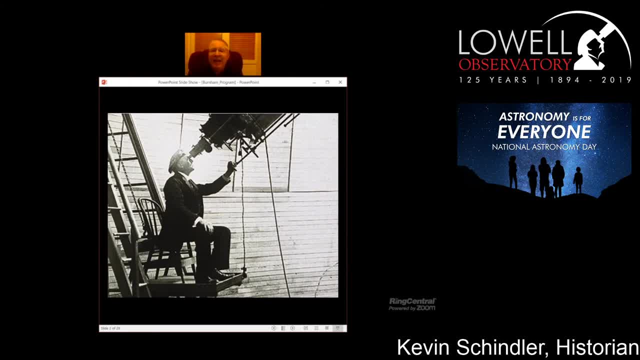 the Perkins telescope is now operated by Boston University. It's still on site at Anderson Mesa with some other research telescopes, But its lifetime is continuing. So while we don't own that telescope anymore, we have the Lowell Discovered Telescope as our workhorse. we just keep. 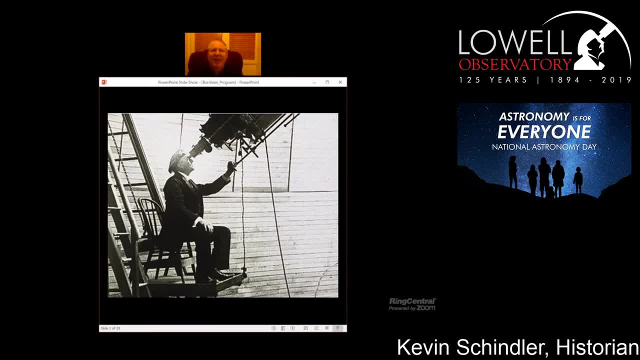 using good telescopes. The passion of doing astronomy we see repeated, And I think a theme that's kind of interesting for me is we're getting to Robert Burnham, because Percival Lowell was a self-taught astronomer. He went to college to study mathematics. 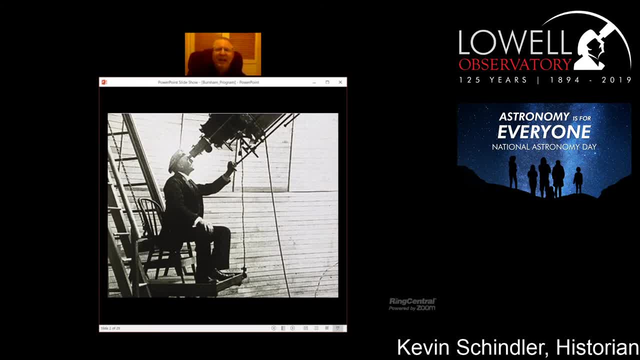 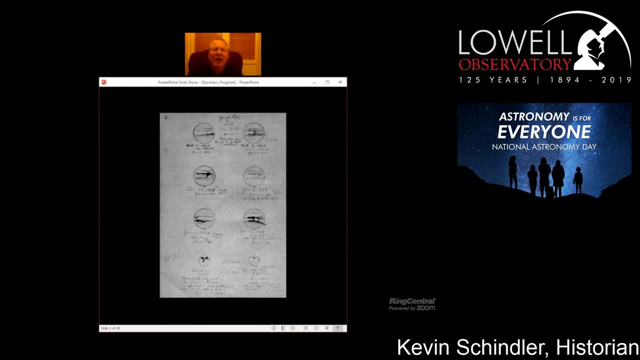 but he was self-taught in astronomy But he was so passionate about it and he started his observatory Well gosh around 1915 or so, right around when Percival Lowell died. there was a fellow who lived in Illinois. 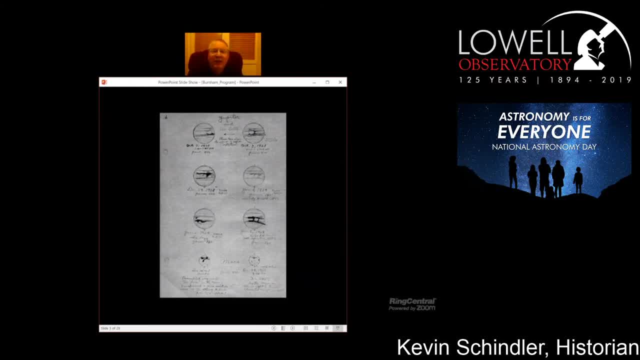 then in Kansas lived on a farm And what he started to do on the farm he built his own telescopes and he made drawings And he was really familiar with Percival Lowell and Percival Lowell, he later said, was one of the people that inspired him. 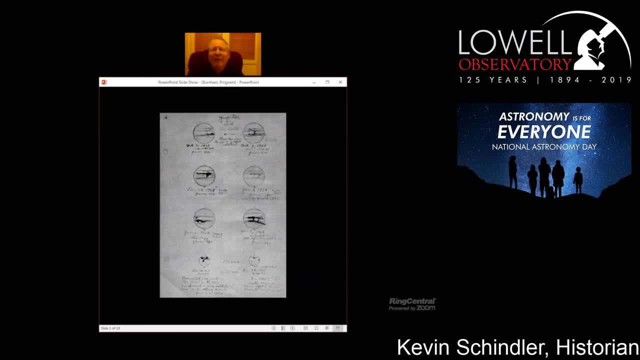 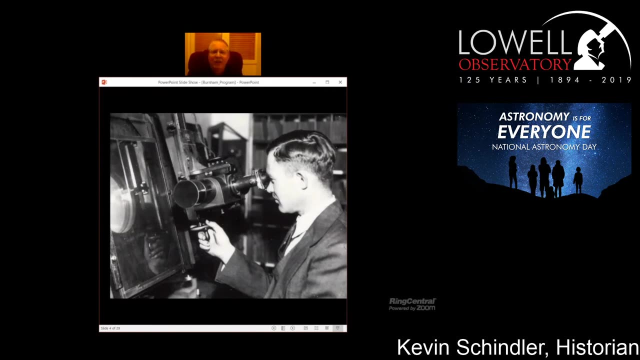 And so he sent some of his drawings to the Lowell Observatory. a decade after Percival Lowell passed away, He sent these drawings in and he said: what do you think about these drawings? And the leadership said, hey, we love this. why don't you come and work for us? 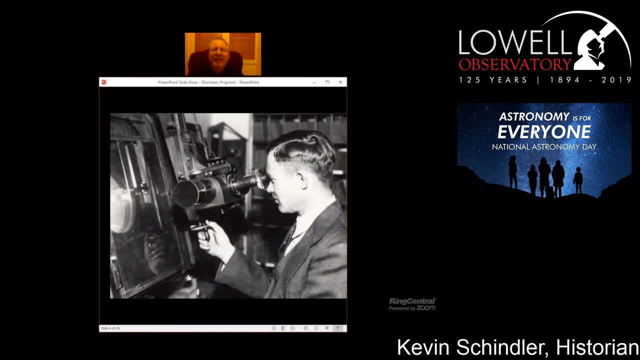 That fellow's name was Clyde Tombaugh, another self-taught astronomer who, by the time he was 24 years old, he discovered Pluto, And so what a great passion he had for astronomy. Well, while Clyde Tombaugh 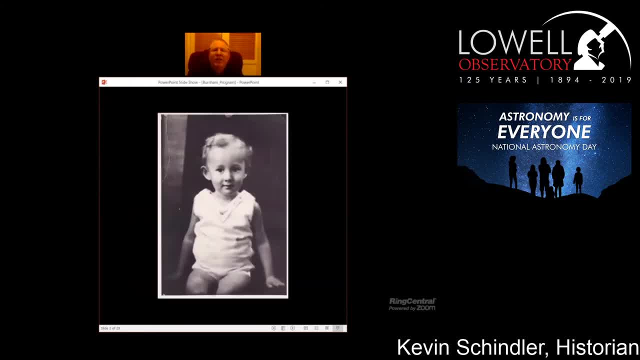 discovered. Pluto, worked there for another 14 years and then left and went to New Mexico. He moved into the 1950s just as Clyde Tombaugh was getting settled working in New Mexico, There's this young guy. He was born in the early 30s. 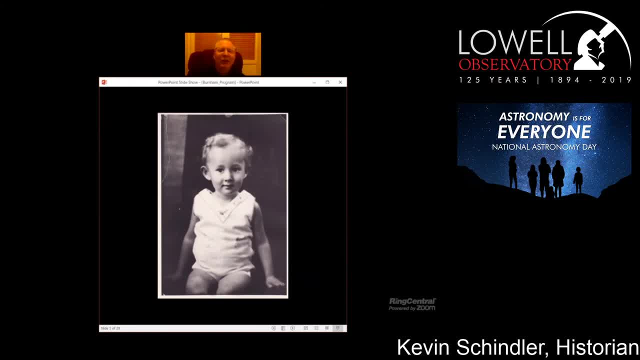 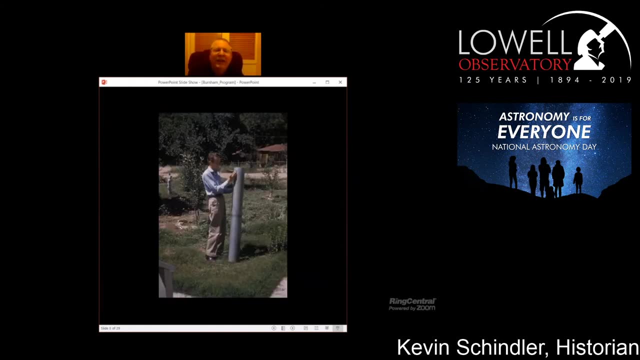 1940s, just as Clyde Tombaugh was leaving Lowell, this kid, his name was Robert Burnham. He was born in Chicago, His family moved to Prescott And he got really interested in astronomy as a kid And he grew up in high school. 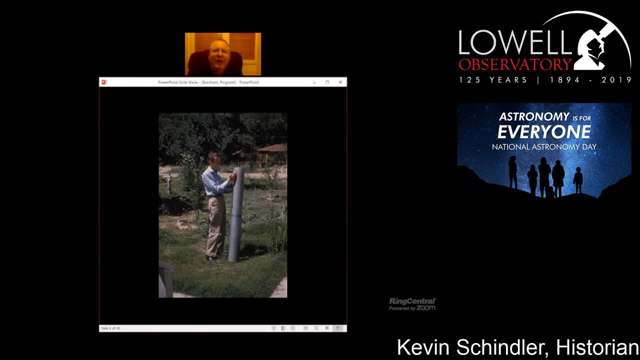 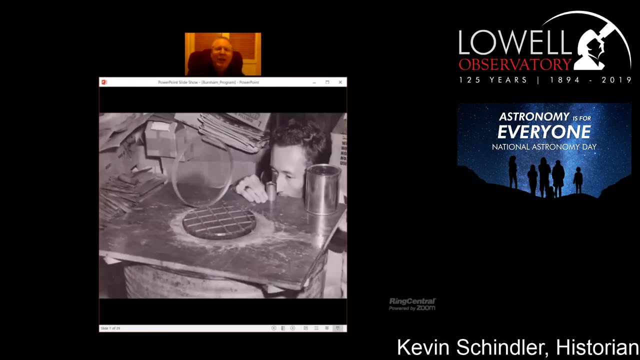 His classmates called him the professor, His family members they call him Cosmo, because he just really loved space And he built his own telescopes. And after he graduated from high school, this is what he did: He stayed at home, He looked through telescopes. 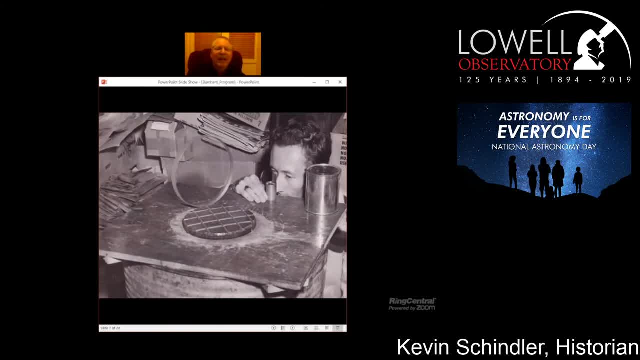 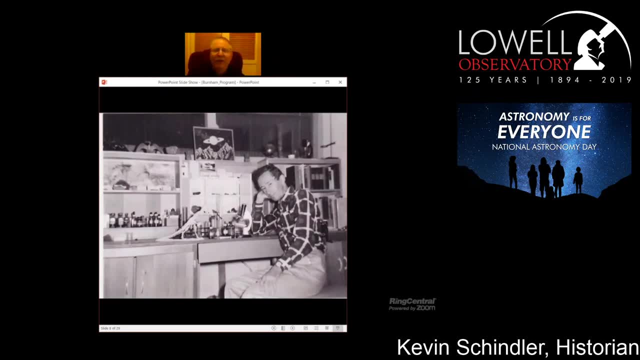 He was really passionate about it. This is him grinding one of his own lenses. He's measuring one of the optical indices of it. He was really interested in a lot of different things, Not just astronomy, but he collected rocks. This is a picture of his homemade. 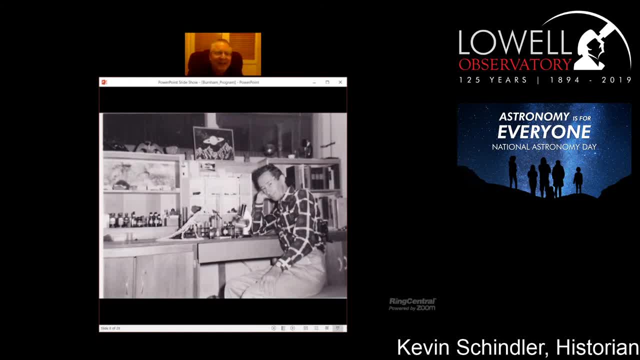 laboratory in Prescott. He's got chemistry studies. He's got some dinosaur models, Rocks and minerals, That drawing of Saturn he did. He was a very talented person And this is what he did for a while. He went to the Air Force for a few years. 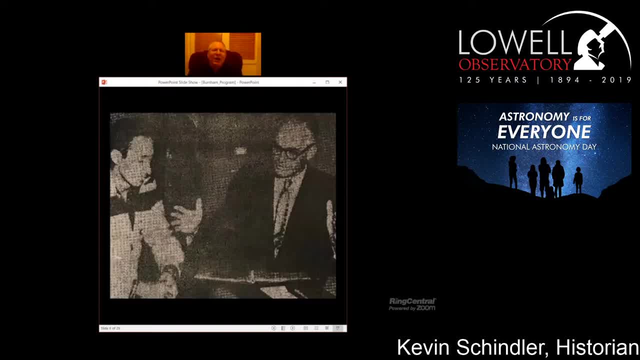 Came back home in Prescott. But then his life changed And I apologize for this quality of this picture. It was from a newspaper article, But from Arizona, my recognized fellow on the right, and that's Barry Goldwater, who ran for president in 1964. 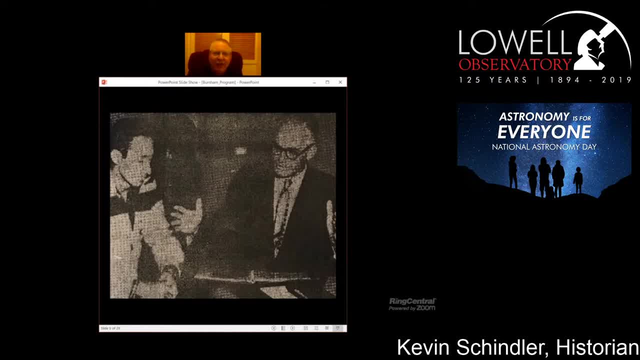 Well, Robert Burnham, 1957, he's using his homemade telescope- that he bounced against the beams on the porch and looked up at the sky. He had become very knowledgeable about the night sky And he discovered a comet And this is pretty great news. 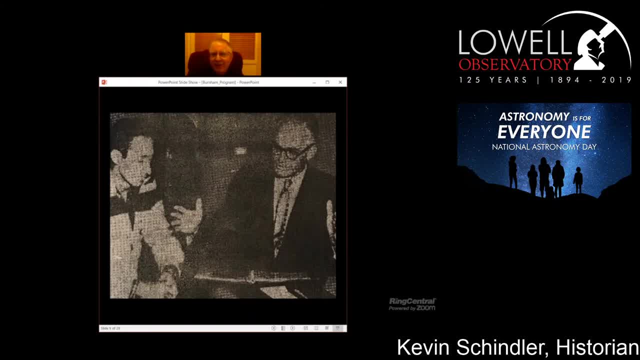 This self-taught guy discovered a comet, And this is December 1957. This is just a couple months after Sputnik went up and really got the attention of Americans that- my gosh, the Russians, they're getting superiority in space. 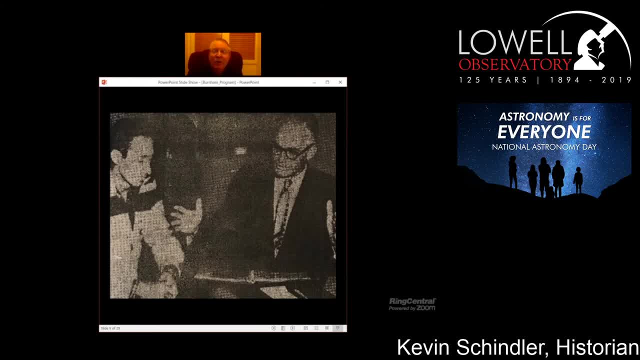 So Barry Goldwater, Senator, who had ties to Prescott, saw this young fellow discovering a comet and thought this was really great. This is a good example of American know-how- People teaching themselves and making great discoveries. So he came to visit Robert Burnham. 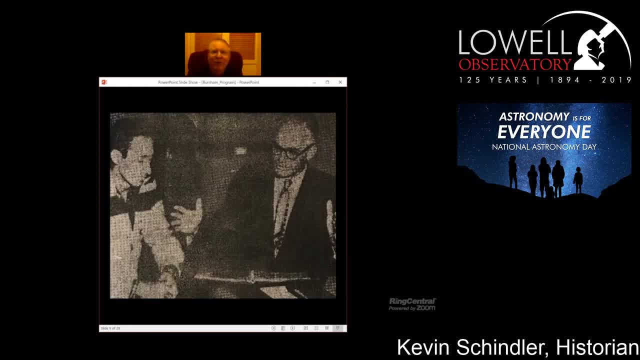 And he even gave him a telescope that his family had owned since the 1800s, And this really got a lot of notoriety from Robert Burnham. Plus, his mother wrote letters to the editor all the time to Prescott, So there's always something. 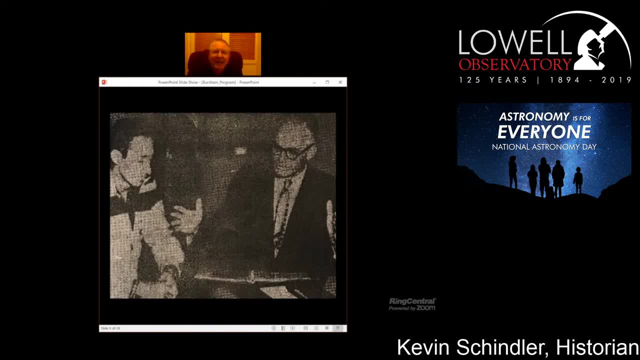 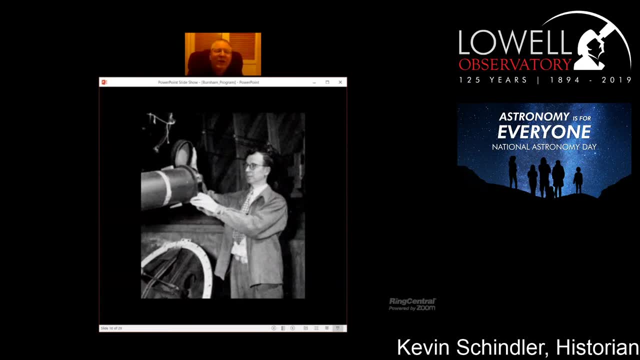 about her views of the paper. Well, she wrote that her son had discovered this comet and it got some views, not just in Prescott but elsewhere. There's a fellow named Henry Giklis, an astronomer, here at Bull Observatory, And here he is using 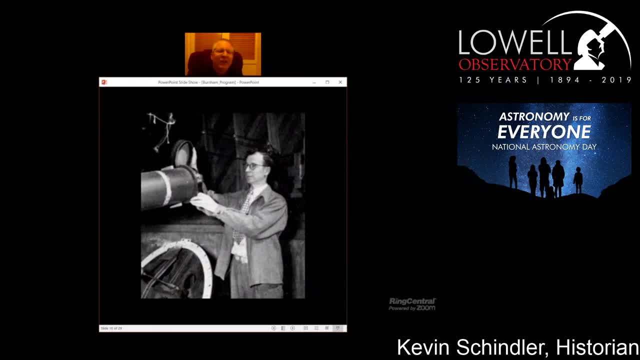 the telescope used to discover Pluto, which is a dive scope on there, And Henry Giklis was just beginning a program called Proper Motion, And it was using the data that Clyde Tombaugh had taken. Tombaugh worked 14 years at the observatory. 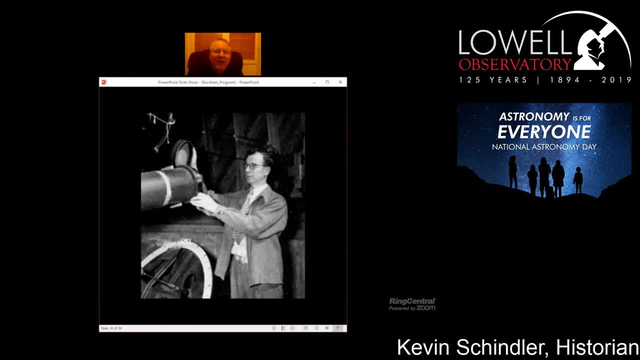 He scanned, I don't know, 80-90% of the sky, And Giklis had this idea: let's photograph the sky and compare the motion of the stars from back when Clyde Tombaugh did it to a few decades later. 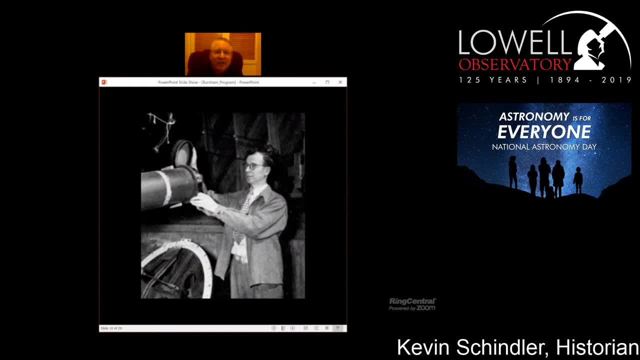 in what's called Proper Motion. And so, just as he's starting this program, he sees: hey, there's this kid who discovered a comet. He must be pretty familiar with astronomy. Let's hire him, Let's bring him on to the observatory. 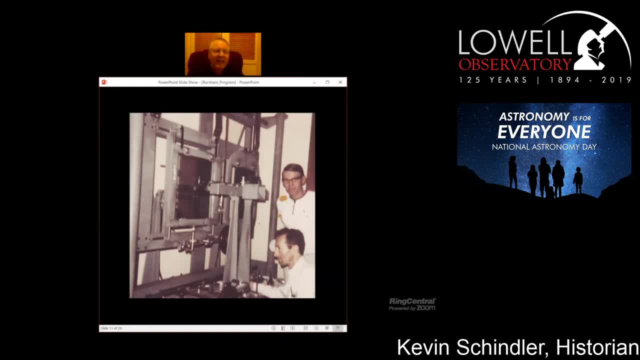 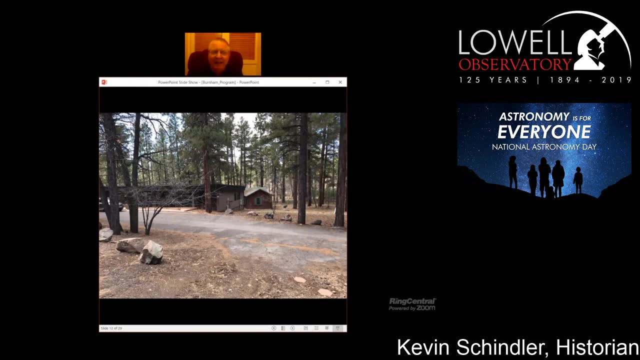 So Robert Burnham, who's in the lower right there, he came on Well modern for the 1950s blink comparator And he would spend two decades here on this Proper Motion survey, And you know two decades is a lot of time. 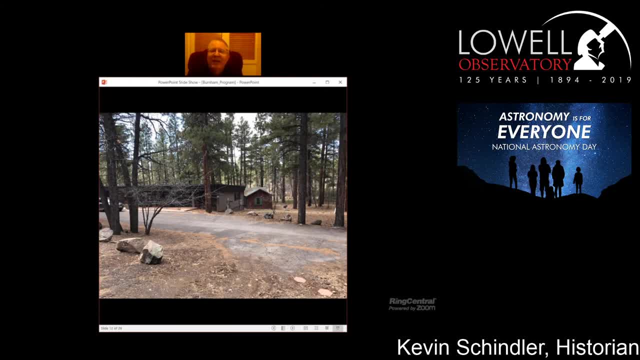 to work at a place He loved it. But there's something we have to mention with Robert Burnham. He was an introvert, He was socially awkward, And so it seems like this was a good position for him. He could do his thing. 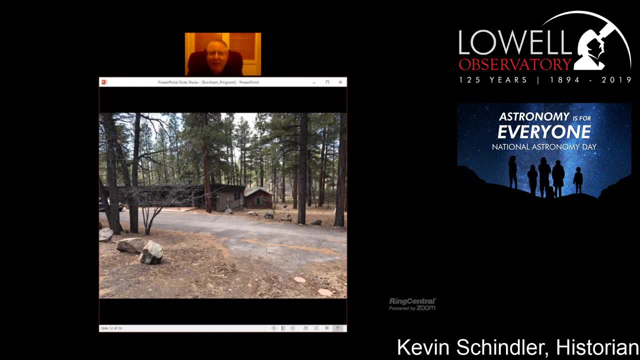 He liked giving tours, but he was also very shy. If you didn't know somebody, there's a lot of complexities to his personality. So he's working up here a year And, as you've been up to Lowell Observatory, as you're coming up the hill, 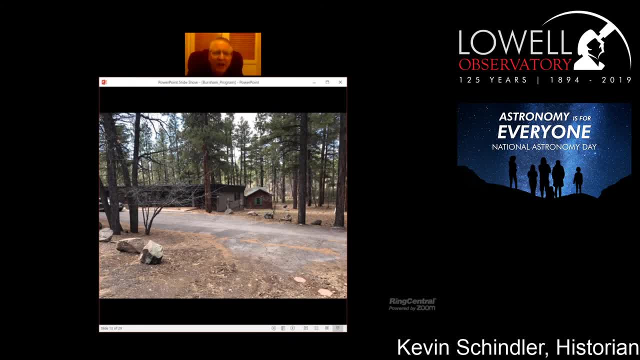 right before you get to the visitor center, on the right, there's a building. on the left, And this is now our business office, And right behind it is a little cabin, And that little cabin is where Robert Burnham lived for most of his time here. 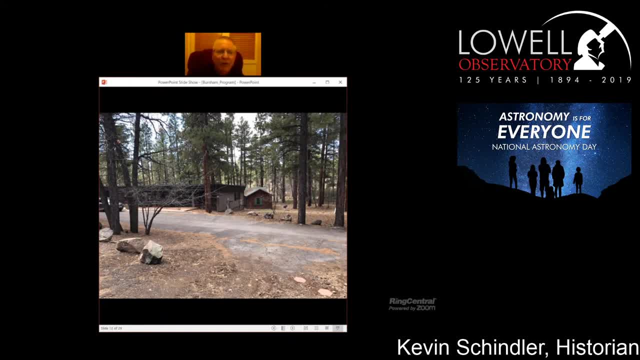 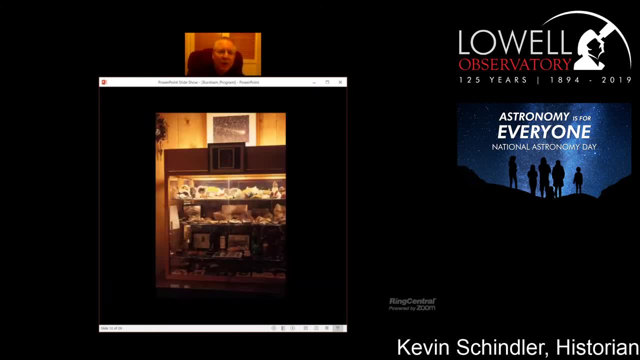 He lived in that little cabin, And that little cabin has three rooms. There's not much to it, But that's where he lived. So his life was doing astronomy. He would work on the proper motion survey. This is a picture inside the cabin. 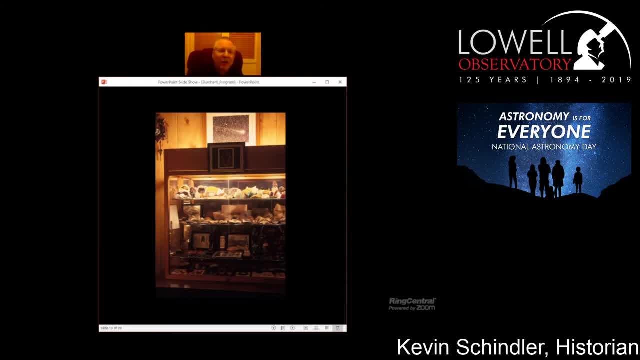 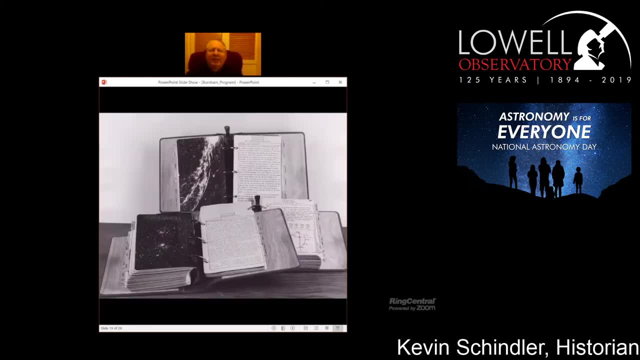 He continued to collect rocks, fossils and coins and other things. He continued to make drawings, But one other thing he did in his spare time was something that is just really remarkable: For a decade he had been compiling information on every constellation. 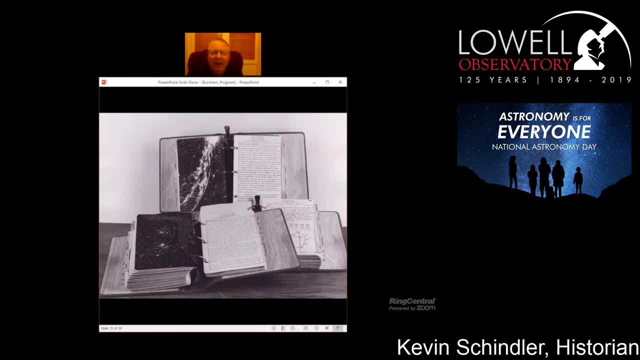 every of the 88 recognized Greek Roman constellations And he wanted to create what he called a celestial handbook, And he did this over time. So many of the pictures in here were taken with the Fluid Discovery Telescope When he wasn't doing the proper motion survey. 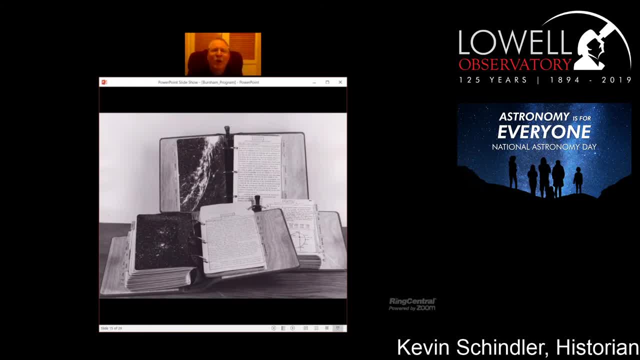 he would work on this And he compiled 2,000 pages And then he put these together page by page in loose-leaf binders and the kids who worked up a bowl helped him, Some other astronomers helped him And he created what we know today. 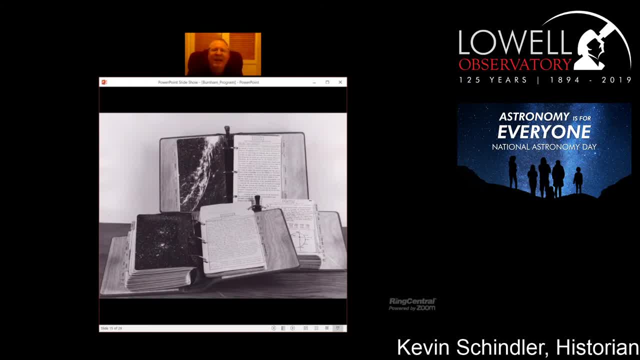 as Burnham's Celestial Handbook And on National Astronomy Day or International Astronomy Day. you know we have to talk about Burnham because this handbook has inspired so many people about astronomy. You know it's been years since it was published. 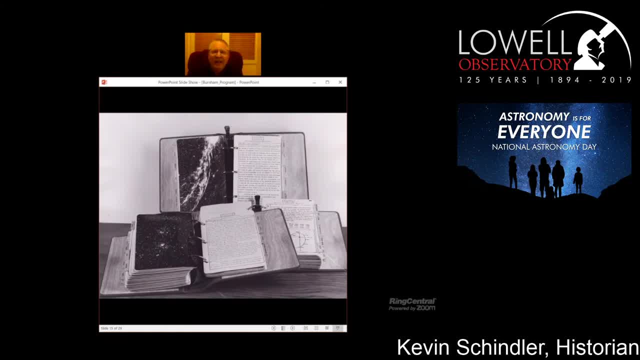 But the information, a lot of it- is a little outdated, like distances and technical information. But remember the background. he had this interest in geology and paleontology and mineralogy and collecting coins. He incorporated all this stuff. So these handbooks are not just data but stories. 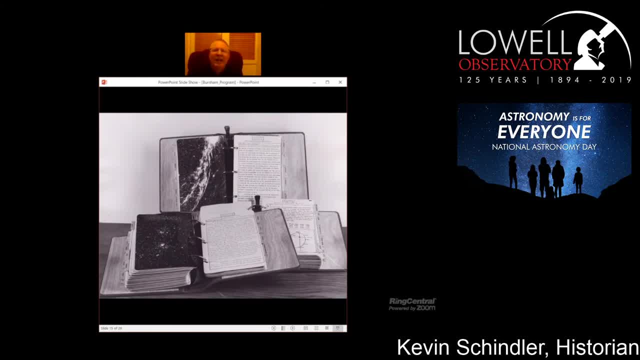 and ties to art and music and other history, And so if you want to find somebody who's passionate about astronomy and feel it yourself, go to a bookstore when they're open and get a copy of Celestial Handbook. Information's out there, but it really captures. 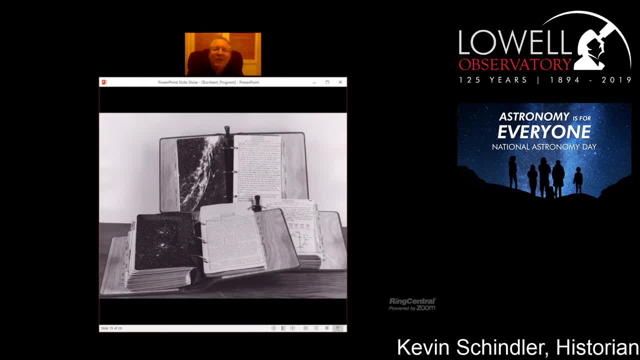 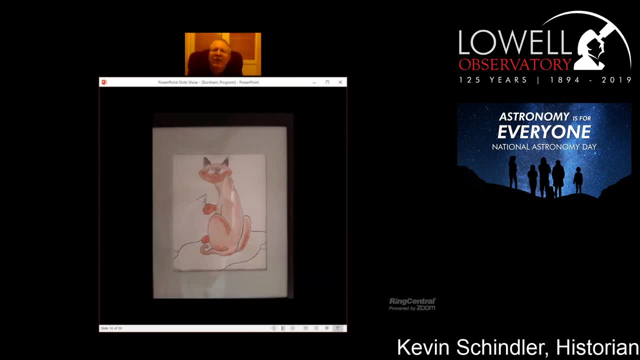 the imagination and the awe of astronomy. So Robert Burnham really became a legend in astronomy. But, as we talked about earlier, there's a tragedy to it, because he also his personality was such that he was an introvert. He had trouble with change. 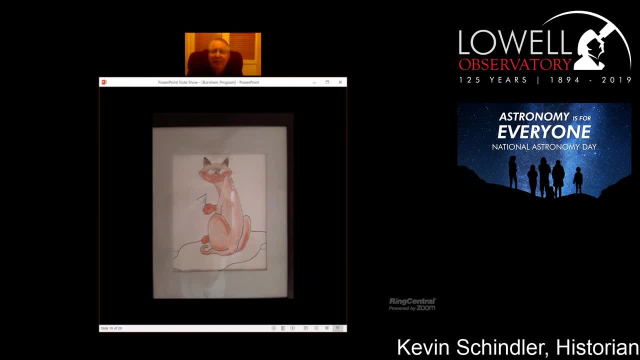 as it looks like, He left Lowell. There's no money for any more projects, So he went to Phoenix for a while and lived with his sister, But then he disappeared And his sister never saw him again. He ended up in San Diego. 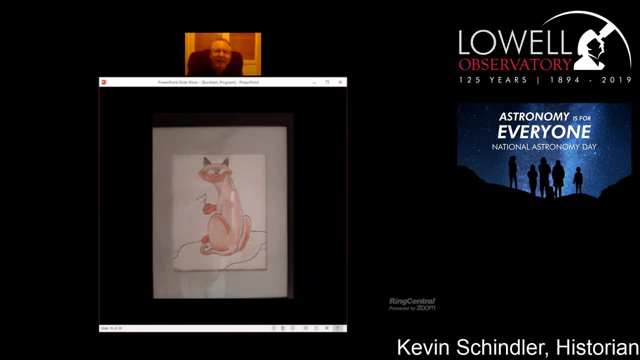 in Balboa Park painting pictures of cats and selling them, And he did have a place to live, but he died destitute, 61 years old, And it's just such a fascinating story I'm not just giving a brief introduction to it, but 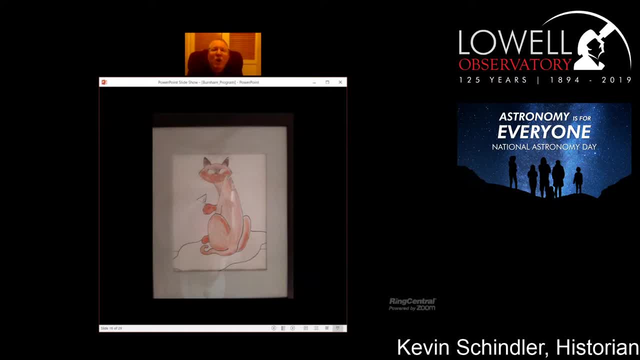 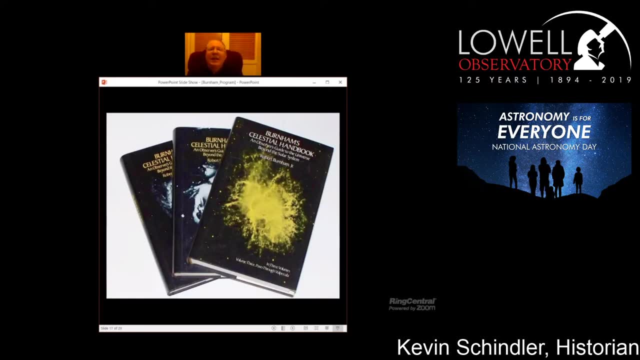 this guy, who made one of the most important contributions to promoting astronomy and our excitement, really died tragically. But be that as it may, his legacy reminds us of what you can do with a passion. Percival Lowell founded the observatory Clyde Tombaugh. 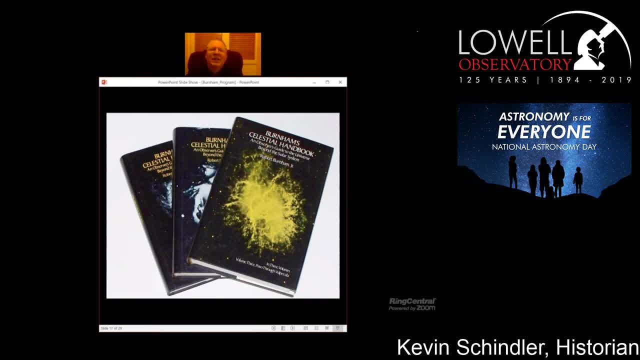 discovered Pluto. Robert Burnham wrote this 2,000 page encyclopedia, as it were, and is still revered by astronomers today. And we heard about from our astronomers and educators and others earlier in our program tonight that passion that everybody has for space. You don't have to have special equipment. 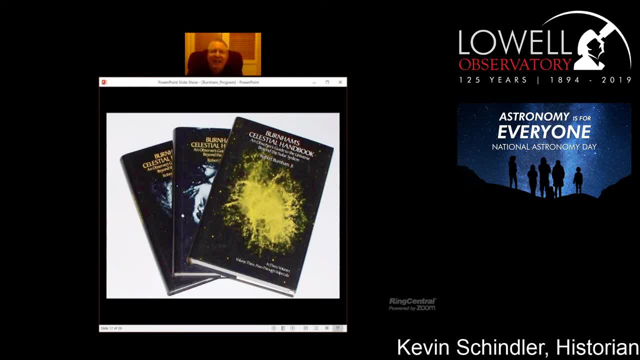 to look up and enjoy the sky. If you get special equipment you can see more, but there's so many different ways of enjoying the night sky and so many ways to feel that passion. I think it's a really neat thing. Let me end with that. 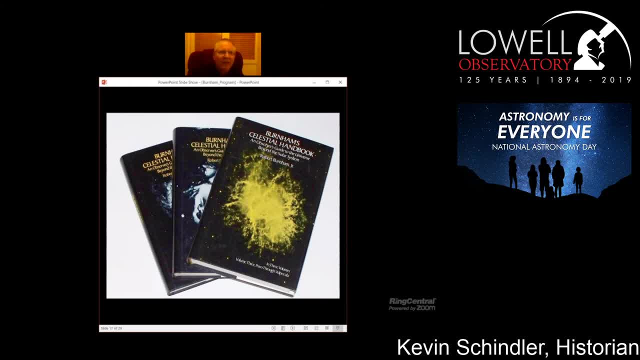 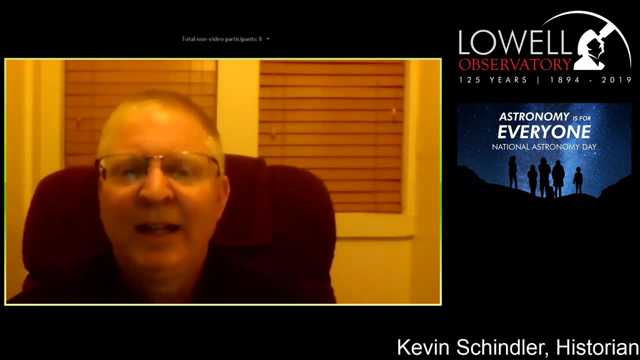 If there are any questions, I can take those. Let me just get out of here. We could talk all night about Robert Burnham. It's just really a classic publication he did, and on National Astronomy Day we of course have to talk about it. 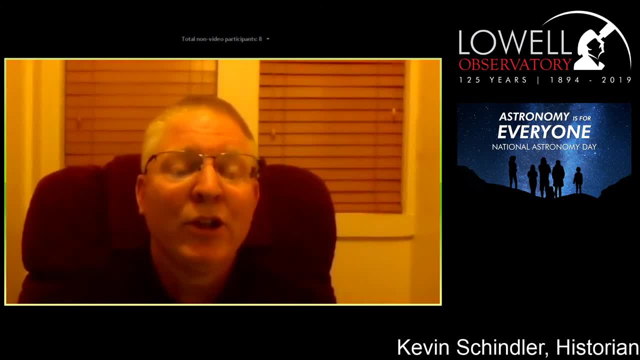 So if anybody has any questions, we'll take those now. Otherwise, I want to give a heads up. Originally we were going to be opening a display about Robert Burnham today for National Astronomy Day, but because of the coronavirus and us being closed, we're going to put this off. 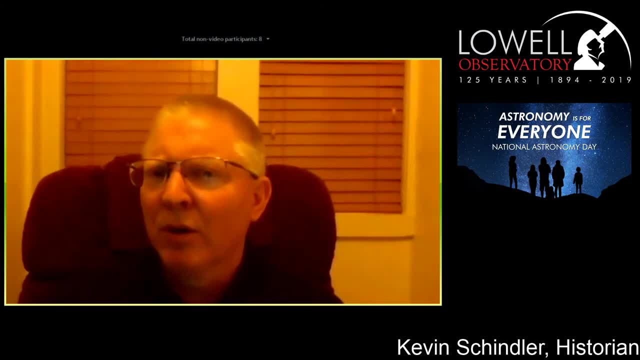 until Astronomy Day in the fall. So on that day in September, or whatever it is, we'll be opening this display and talking more about Robert Burnham and his incredible contributions for astronomy. So thanks everybody for joining me, and I'll turn it back over to Sarah. 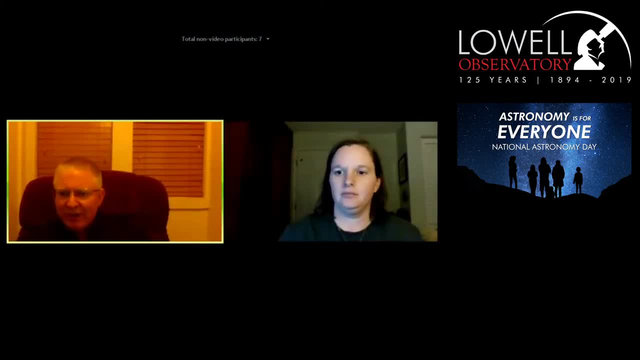 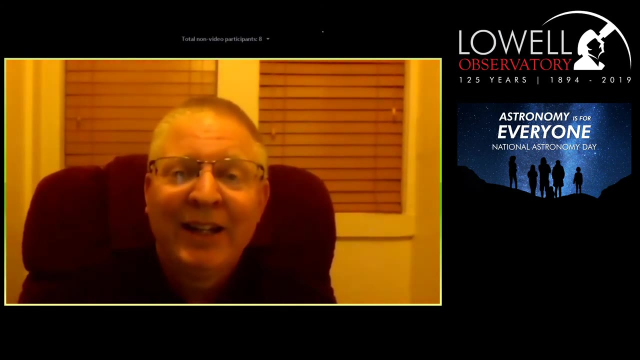 It looks like you have a question for you. It just came up. It's from Summer Brown. What part of this history is your favorite and why? I think it's one of the things I talked about tonight, which is why I talk about it. 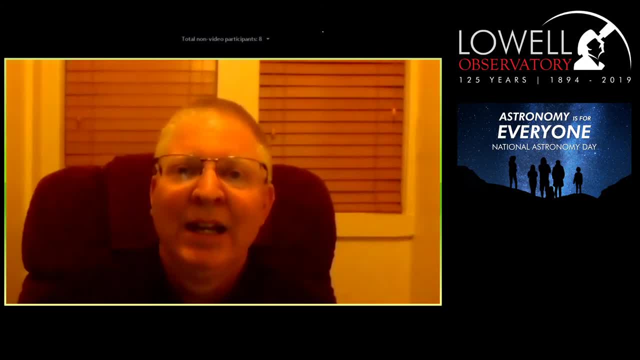 and that's the passion people have for doing science and astronomy. I think of myself as an ambassador to share this excitement, and when I listen to somebody like Phil Massey talking about being on SOFIA or going to Chile to observe, or Gerard or Melissa. 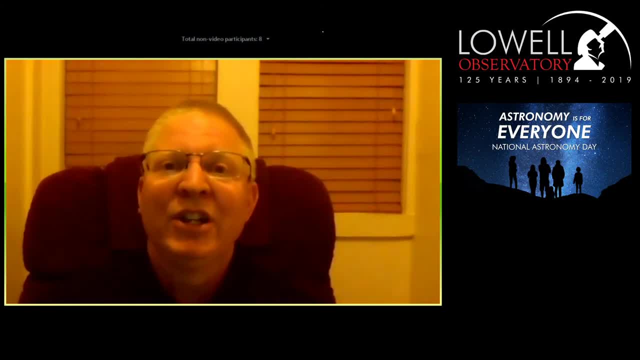 who, as she mentioned, we met in the Grand Canyon and just shared a passion for the universe around us. That's what I like. It's fun to share this. We're all human. It's part of our essence. We're explorers. 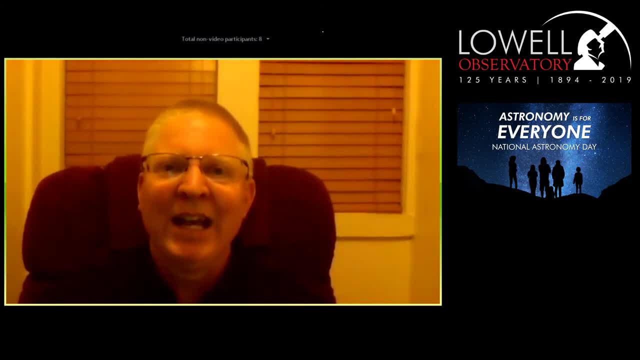 And that's what Loebs and Ruttori does. We explore the universe, Our astronomers go on expeditions to Chile and we think of expeditions like Lewis and Clark, but our astronomers are still doing that kind of stuff today and I think it's really pretty exciting. 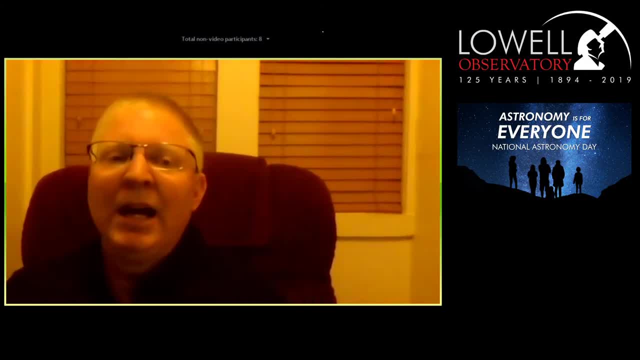 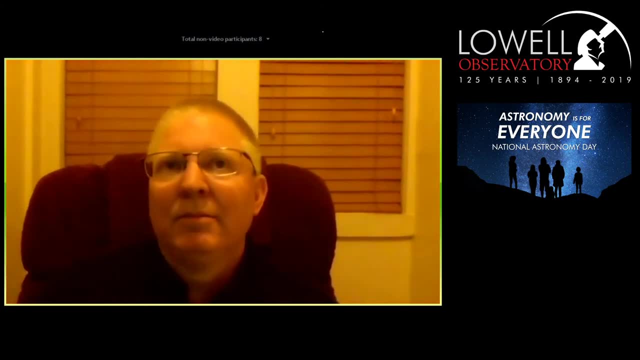 There's another question: Is the handbook, three books? Yes, When Burnham first did it, he created multiple loose leaf printouts and then eventually he sold the rights to Dover and Dover created this three volume set which I have right here and gosh, if you live in Flagstaff. 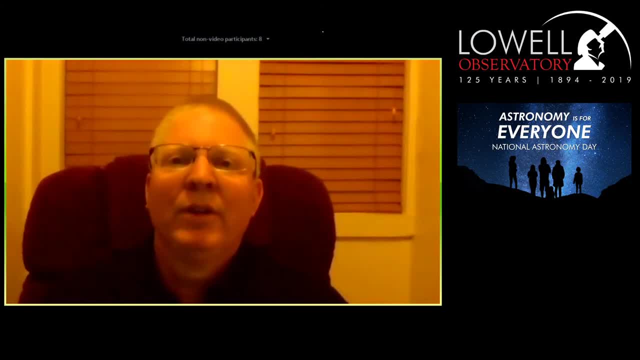 or Tucson or Phoenix. every time I go in there there's a couple copies of the three volume set, but it's really. you're not going to read the whole thing unless you really have a lot of time. but I use it a lot in writing, for instance. 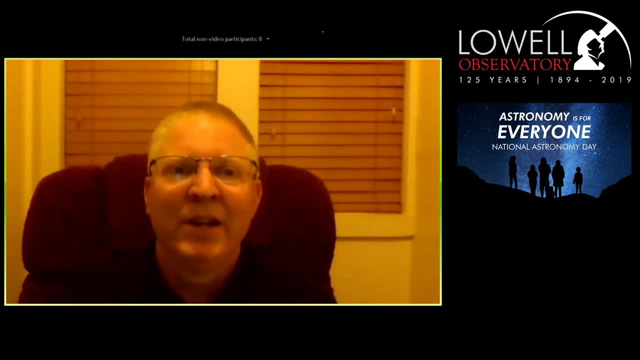 about constellations and every time I read it there's something I pick up, and I've talked about so many different things: mythology, science, of course, how it ties into Roman history of each constellation. it's really fabulous so I highly recommend people getting that. if you don't. 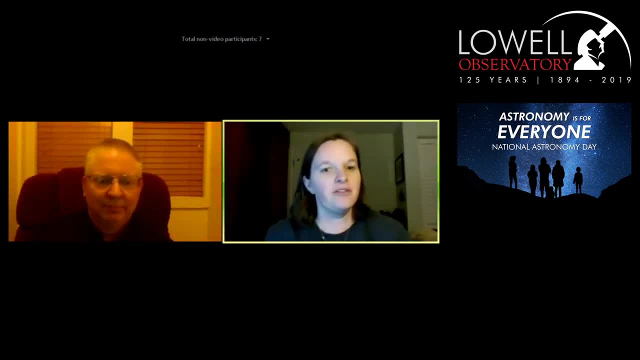 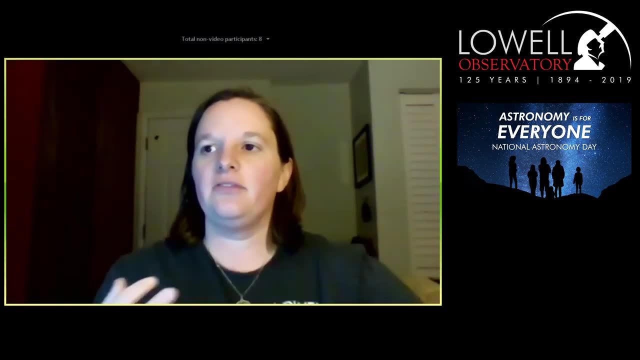 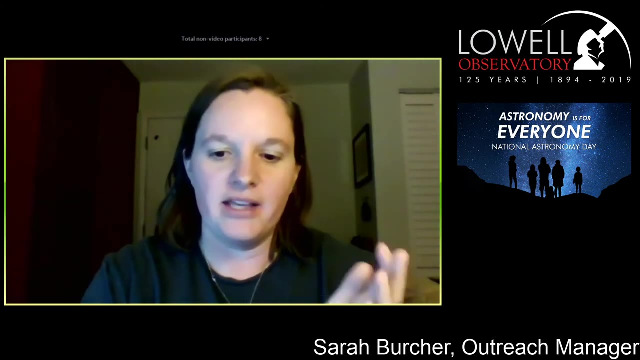 Alright, I think that's all the questions, so thank you for your time, Kevin. So we've spent a lot of time tonight talking about kind of the how our people got into astronomy and how we were all inspired to do this, and so now I want to shift to the more 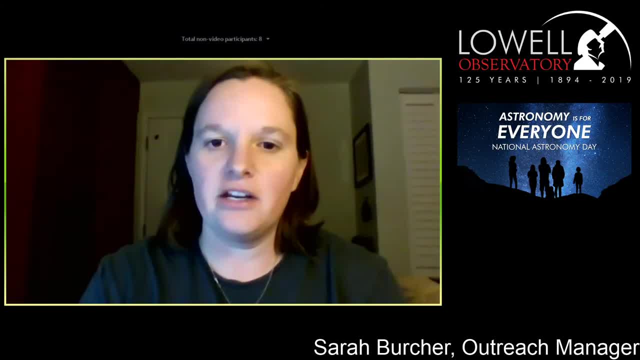 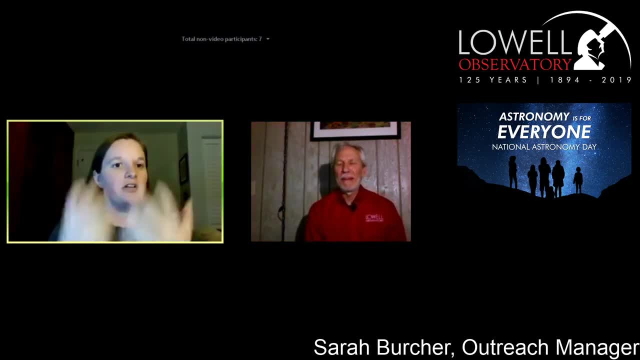 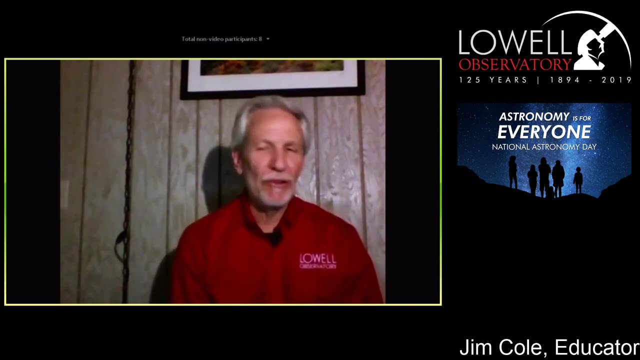 practical way of doing things, and so our educator, Jim Cole, will hopefully pop in and he's going to tell you about how to get started, how to start your own astronomical journey. so, Jim, take it away. Thanks, Sarah, thanks everyone for joining us. my name is Jim Cole. 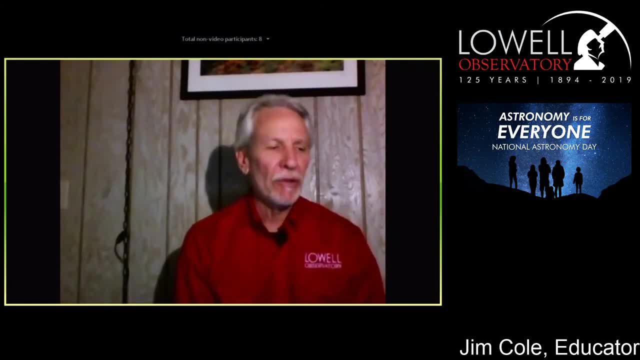 and I am one of the educators here at Lowell Observatory- and in referencing something our educator, Melissa, said a while ago, is that it doesn't matter how old you are when your interest in astronomy is hicked, and I was 40 years old when I received my first telescope. 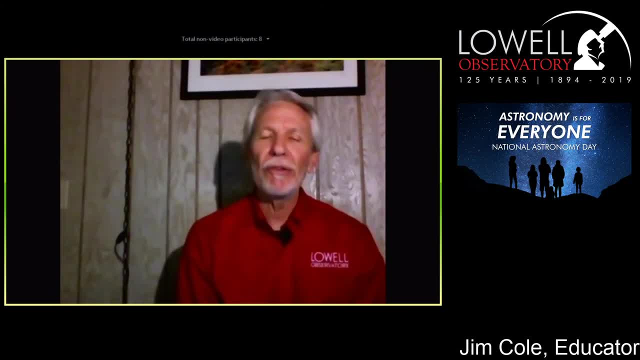 I've been an astronomy enthusiast now- or a backyard astronomer- for going on 30 years, and it really was that first telescope I got, not having any idea how to use it. they caused me to join a local astronomy group. I ended up for a few years being president of that group. 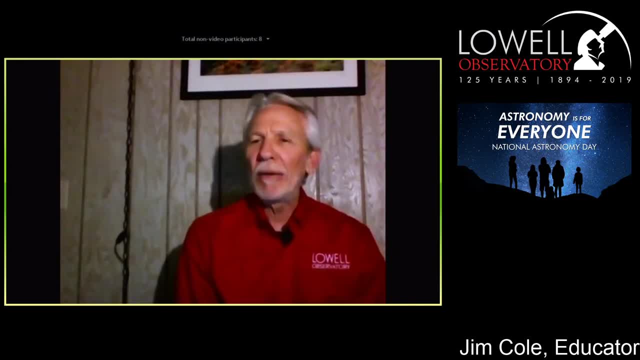 a little bit further down the line, but it didn't take me long at all, once I got involved with a bunch of people that understood what the night sky was all about, to feed me that interest and get me going and, as I said, now it's been about 30 years. 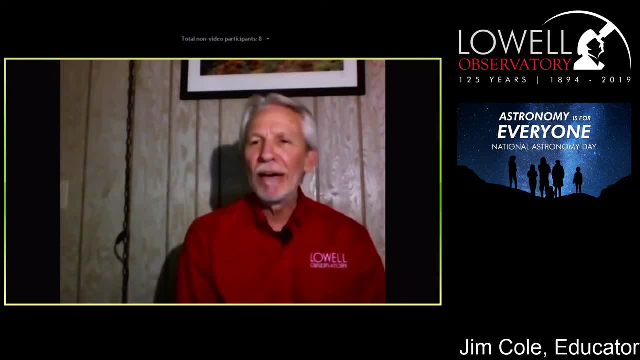 it is the hobby of my choice and I was fortunate enough to actually get a job as an educator at Lowell Observatory to carry that enthusiasm to new generations of people. so in reference to Kevin's talk, he just did too. in the mid 1990s I bought my first three volume set. 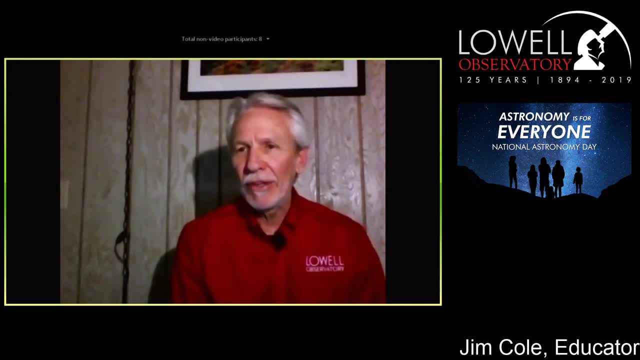 of Burnham's Celestial Guide. it is still, to this day, one of my most treasured volumes. so indeed, most amateur astronomers, if they've been around for any few years at all, usually have a copy of Burnham's book. it's a classic in your local used bookstores. 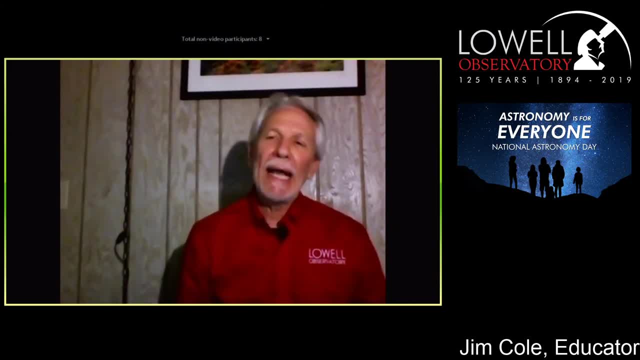 so what I want to do is talk about how to get started as a backyard astronomer, and, before we jump into that aspect, I want to remind everybody that there's a lot of different ways that you can learn about astronomy without having to do this on your own. 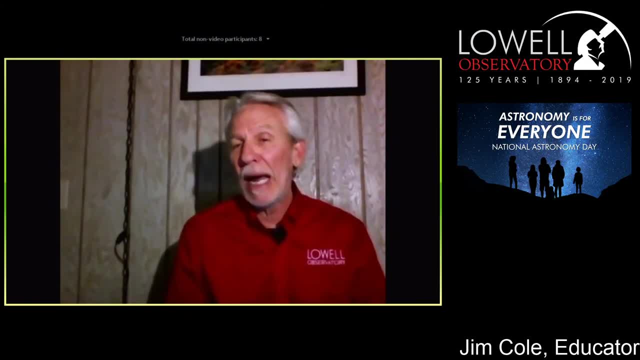 we have like, for example, at Lowell and other places. there are summer camps for kids. so if you're younger you can do these in astronomy camps and get your first taste of how the universe works around the country and around the world. regionally, there are star parties. 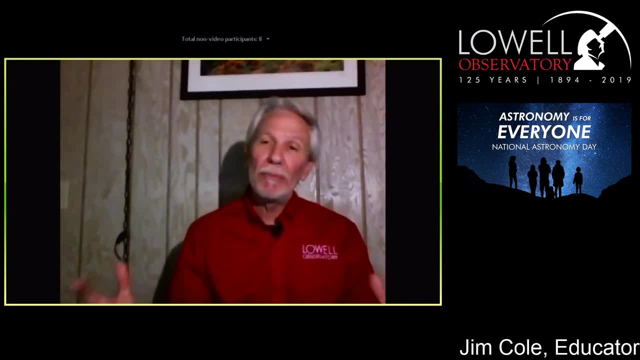 where amateurs get together. sometimes hundreds of them set up telescopes and the general public is invited and the general public gets to get their first views at the universe through these telescopes. it's a pretty awesome thing and a great way to break into looking through telescopes. 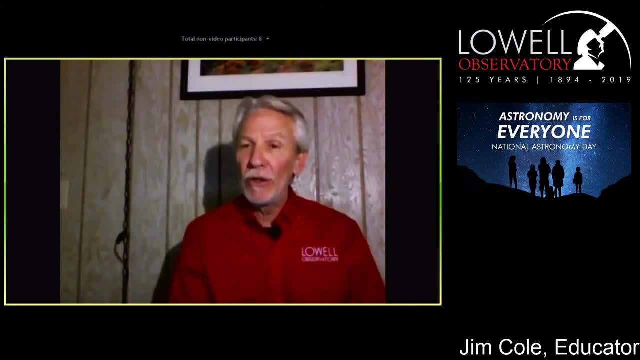 you can visit planetariums and get science presentations on how the universe works. you can visit the great observatories around the world, especially those with public programs, like Lowell Observatory, where you can attend science presentations, get historical tours and look through some of the most incredible telescopes available to the public. 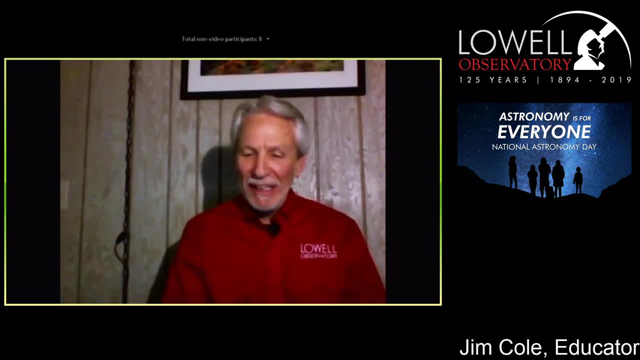 on a nightly basis, of course, when we get reopened after the coronavirus. and finally, you can just go to a library and check out some really cool books on the history of astronomy and actual science and get as deeply into it as you want. so what we're going to do now, though, 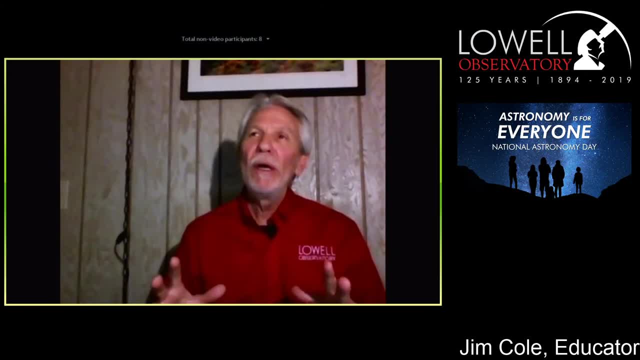 is. I want to get into the practical side of how somebody starts to get into this and, having run telescopes for about five years at Lowell and done constellation tours, the most common questions we get on a very regular basis is: how do you get started in doing this? 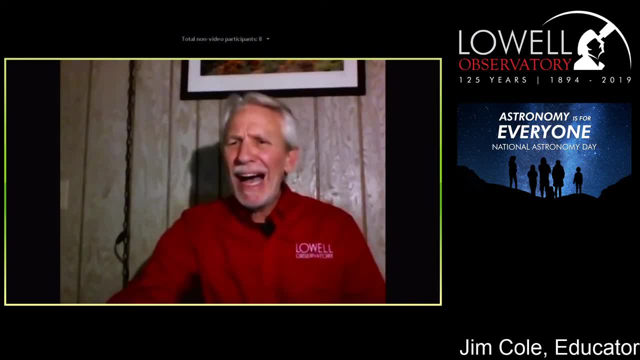 what telescope should I buy my gosh? how did you even find that thing you're looking at? it's like in the middle of nowhere. so we get these questions all the time, and so we're going to try to address exactly that here in the next few minutes. 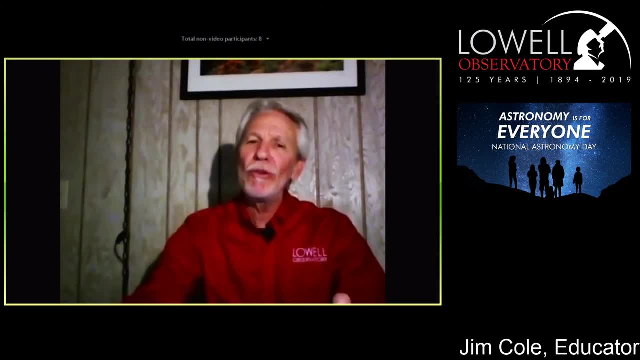 and what I want to do here- because this is a relatively short presentation- is I want to get you started in the simplest, most effective way. I know how, and that does not include the use of a telescope. surprise, that comes later. I'm going to give you a presentation. 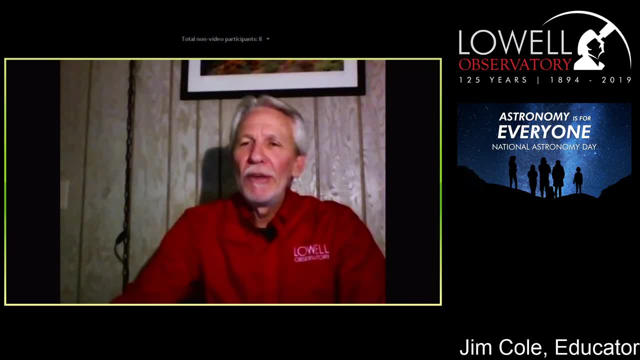 sometime on a future program about how to do that, but tonight we're not going to talk telescopes, so what I want to do here is talk about five things- actually four- that you really need. one is a nice to have to get started in backyard astronomy- you need a place to observe. 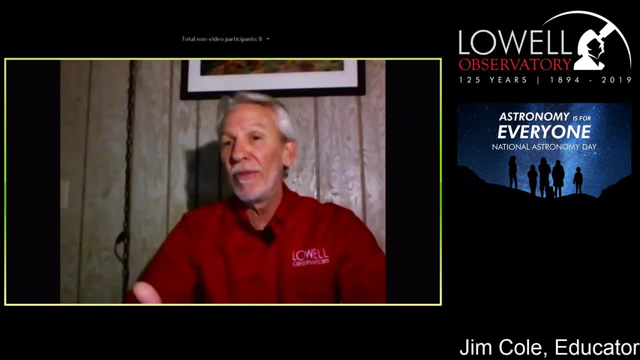 where you can be comfortable and safe. you need a nice, comfortable chair to sit in. that sounds kind of weird, but it's very, very true. we'll get into the details in a moment: all of those stars overhead and how to learn your way to navigate the night sky. 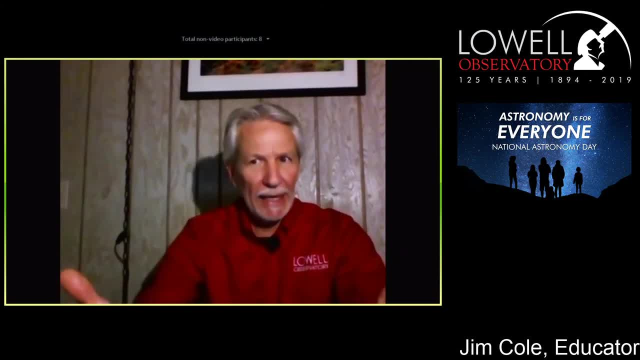 and be able to find objects you don't want to look at. you need a red flashlight that would allow you to look at star maps alright, without ruining your night vision. we'll talk about that in a moment. and the fifth thing: that is a nice to have but not required. 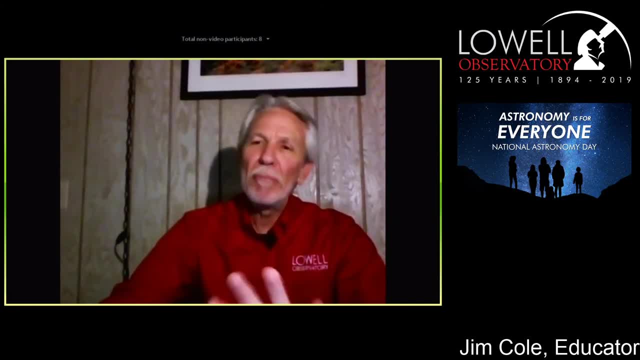 is a good pair of binoculars, and that's sort of the prep to get you ready to start using telescopes. so let's go through these one at a time. we need a place to observe, and the most obvious place for that would be your backyard. 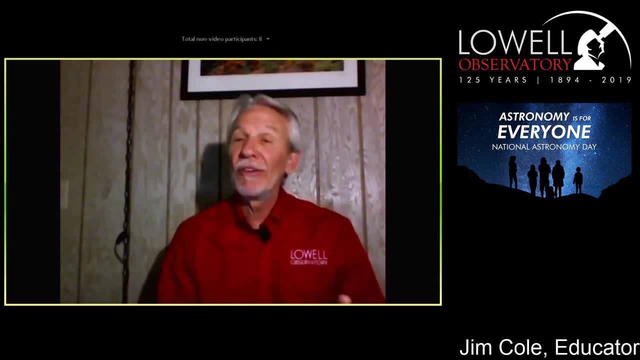 however, the vast majority of Americans, and indeed most people around the world, live in large cities where it's very, very difficult to see the stars, so you need to find an area where you can see at least a couple of dozen stars. that's enough to get you started. 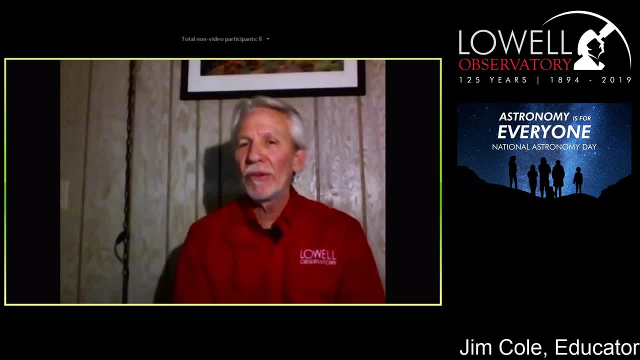 to be able to recognize some of the constellations and to learn your way around the sky. alright, we're lucky here in Flagstaff. I can walk out of my backyard right here. it's one of the reasons I moved here and look up in the night sky on a moonless night. 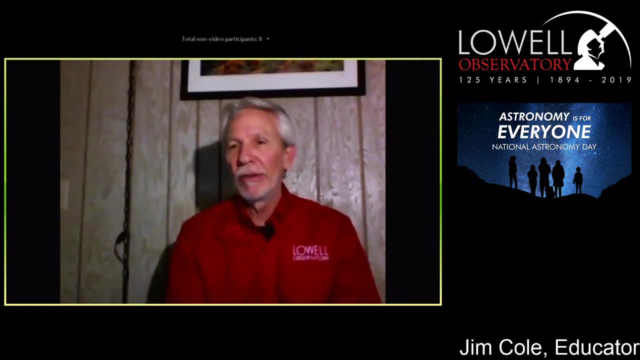 and, on a good, transparent night, see about 3,000 stars. most people in big cities are lucky if they can see a couple of the bright planets- maybe a bright star or two and the moon, so it's quite an incredible experience to live here in Flagstaff. but most of you don't have that benefit, and so if you do, if you are lucky enough to live in a place where you can walk out of your front yard and your backyard and look up and see at least a few dozen stars, that's a perfect place. 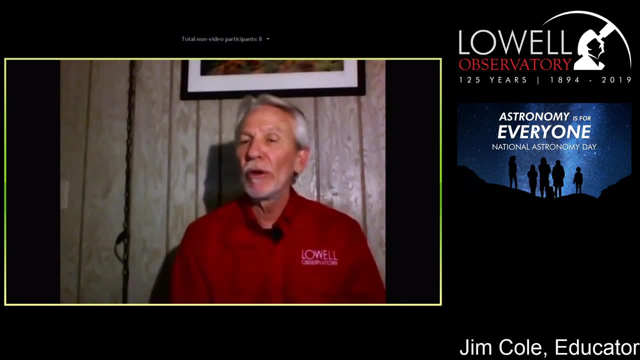 it's comfortable, it's easy to walk outside. you don't need to commit an hour or two hours to learn astronomy. you can go out for 5 or 10 or 15 minutes at a time and learn something new for the night. all quick and go in and go to bed. so your backyard, front yard, first choice, and you can't really see any stars. or even if you live on the edge of the city or in rural areas and you have neighbors that like to light up their yards and, unfortunately, as a result, light up your yards. it's very difficult to see stars. you might want to check out local neighborhood parks or community parks, where they sometimes are located just outside the city limits a little bit or outside your neighborhood where the sky might be a little bit darker. that's a next choice. third choice requires to drive out of the city. 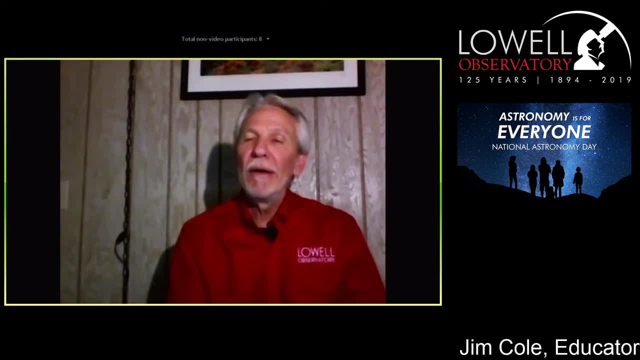 sometimes you just don't live in the right spot, and so you throw what you need into the car and you drive a half hour or an hour to get out of town someplace that's a little bit darker, and then worst case scenario- and not necessarily worst case scenario- 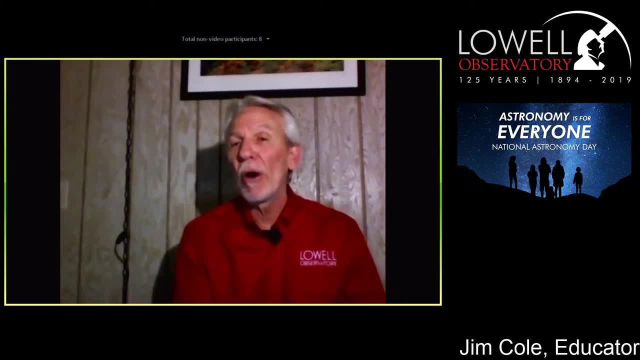 these are awesome places, the United States and around the world. there are national parks and other parks that are available to the general public, where the lighting is a little more controlled and you can get to some of the darkest skies, especially in this country, so sometimes overnight camping trips. 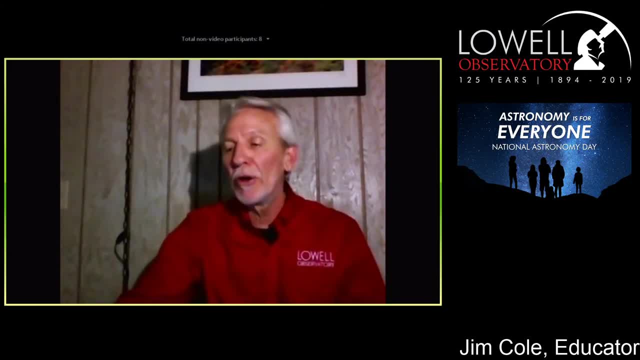 might be necessary. if you're lucky enough to use your front yard or your backyard, you've got it nailed and it's as easy as it gets. so that's the first thing. let me get a sip of water is to make sure you have a nice, safe location. 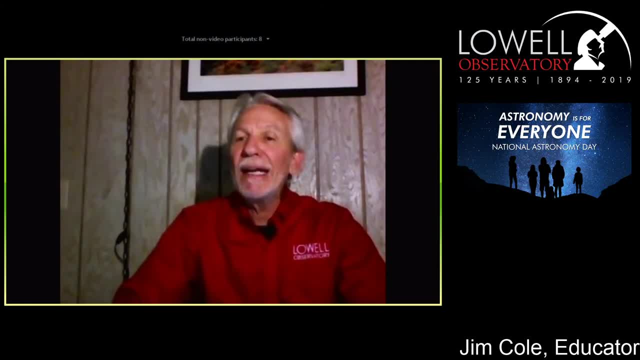 where you can spot enough stars to be able to learn your way around. the second thing that you need is a good, comfortable, adjustable patio style lounge chair. lot of words, so the whole idea of a relaxing reclining chair is it allows you to put yourself and your head. 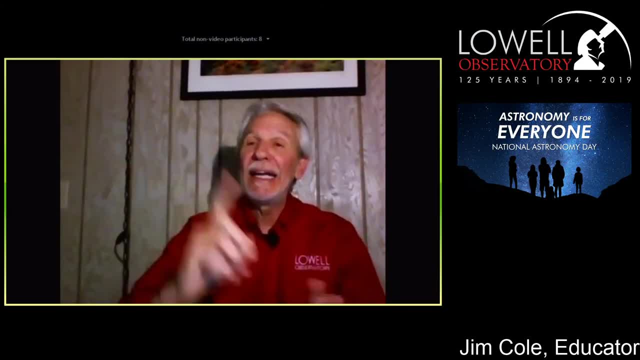 comfortably relaxed and point yourself at different places in the sky, including straight up, without getting tired or straining your neck. it also helps to maintain your body if you decide you want to use a pair of binoculars, and it's easier to steady a pair of binoculars on your face. 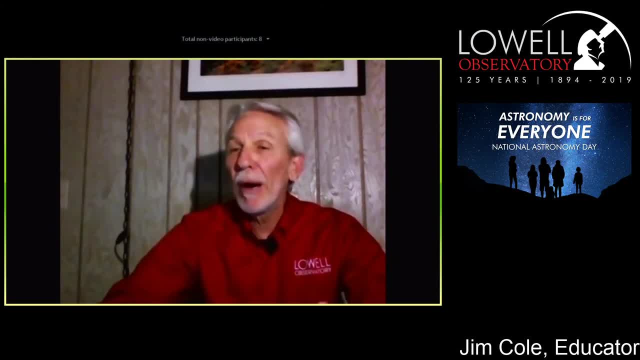 if you and your head are supported, you can use a regular chair among astronomers or amateur astronomers, I should say. it's a brand called Zero Gravity and it's because it's a really comfortable lounge chair. it's got mesh over a metal frame. you can put it in all kinds of different positions. but it's the way the mesh supports you. that makes it very comfortable to sit on or lay on for long periods of time, and the Zero Gravity is not necessary to buy that brand. there are many, many copycats now in the market and I'll just make this point. 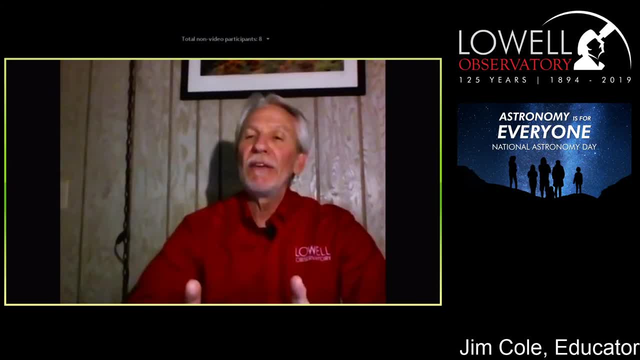 that there is nothing more uncomfortable than standing and looking at the night sky with your head bent back like this. it becomes fatiguing very quick and astronomy will literally become a pain in the neck. you won't want to do it, so you want to make yourself comfortable. 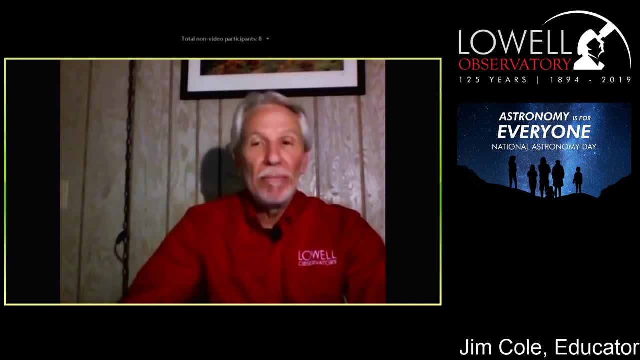 lay down on cold nights, take a blanket and sleeping bag out with you and make yourself comfortable. so you need to have a good observing spot. it's safe to do it and it's dark and you want to have a nice, comfortable chair, alright. third thing, we want to have a good map of the sky. 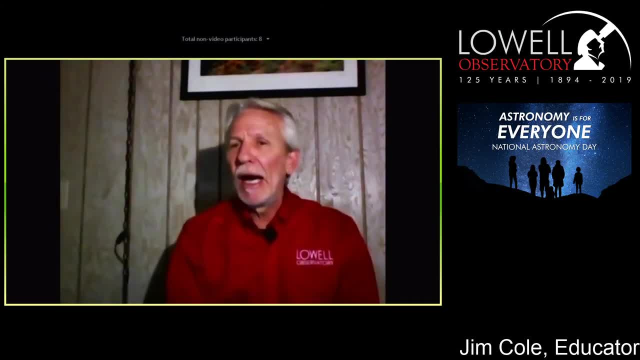 all of us can just look up at the sky and marvel at the stars, but part of the understanding is to realize that there's relationships, historical relationships, between a lot of those stars. we call them constellations and learning the constellations, at least the major ones, that change throughout the year. 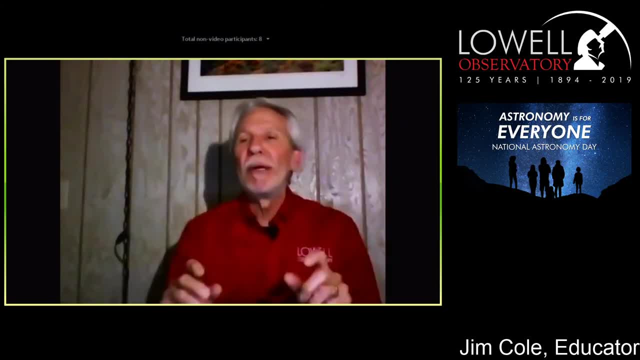 helps you to get a grip on the sky, what's up and how to find things, and so the very first step is to just start learning your way around the night sky, and to do that, you either need a tutor or a teacher, or you need to have a good star map. 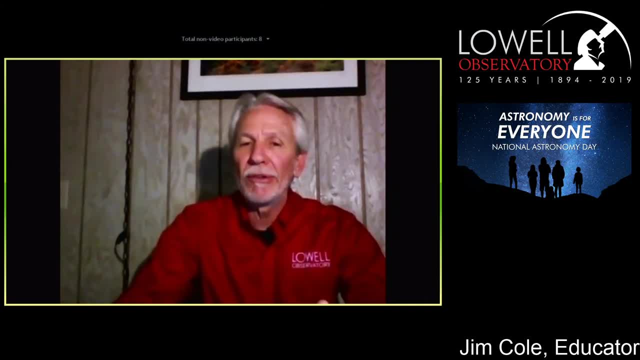 that allows you to look at the night sky and relate it to something in print. alright and right off the bat, I'm going to suggest that, even though we're in the modern age here of devices and phones and iPads, I want to recommend against using those kinds of devices. 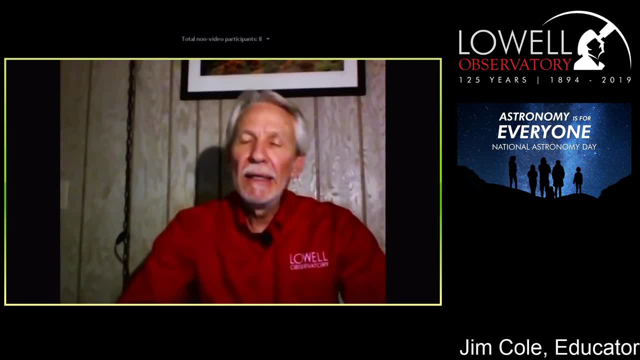 with astronomy apps on to learn your way around the night sky. unfortunately, most of those apps bleed a lot of light even though they have a night mode, and your night vision, which we'll talk about in a few moments, will be ruined and will make it harder and harder. 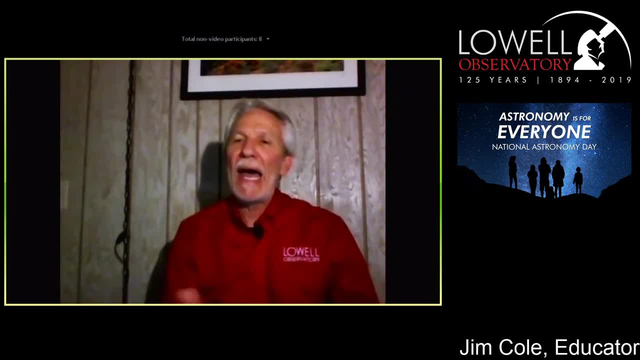 for you to see things. so my philosophy is to leave those things at home, in the house, in the car, wherever you happen to be, and don't take them out with you. it can ruin your night vision and make it very, very difficult to see things. 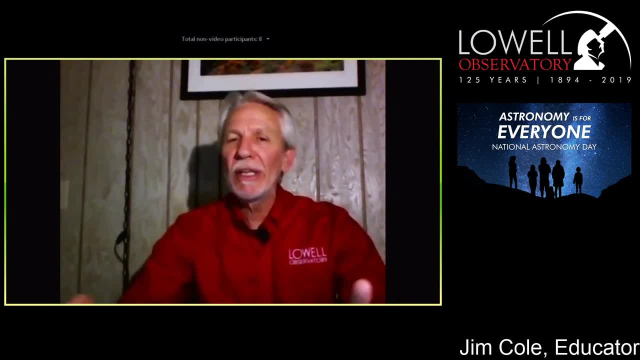 alright, so at this point you're learning. you basically want to learn to explore, discover and understand new things about the universe. alright, so you want to keep it simple. the way I started was a star atlas, even though I had a telescope for the first couple of months. 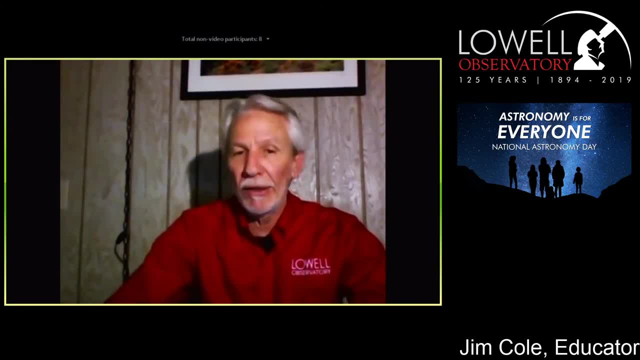 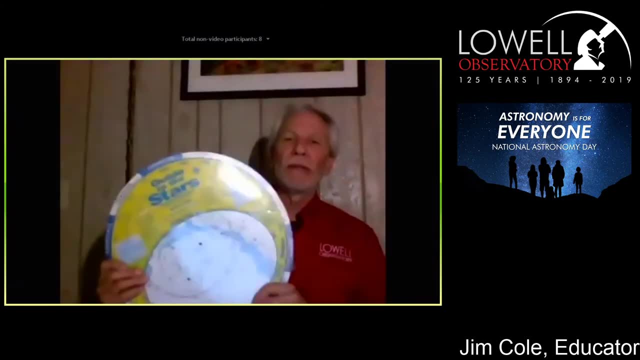 I didn't use it much because I didn't know how to use it, but I learned my way around using a star atlas, so you learn your way around the sky. alright, we're talking about things like. this is a planisphere. it's called this particular one. 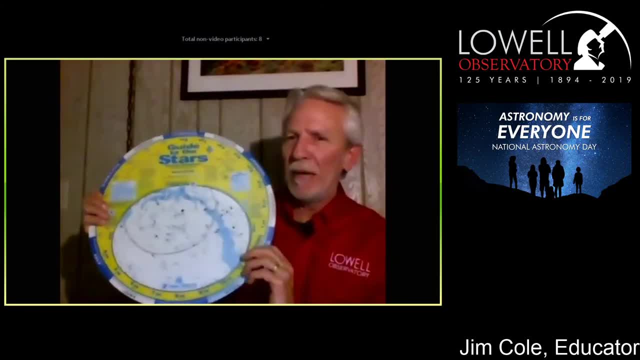 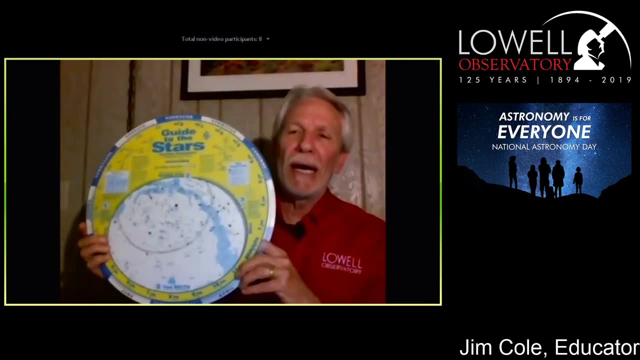 is called Guide to the Stars. alright, and this is a big classic thing. you can buy at most bookstores like Barnes & Noble. you can buy it online at Amazon. you can buy it at the Starry Skies shop at Lowell Observatory and many other places. 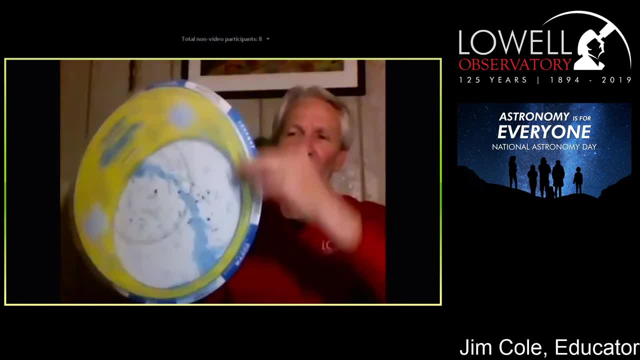 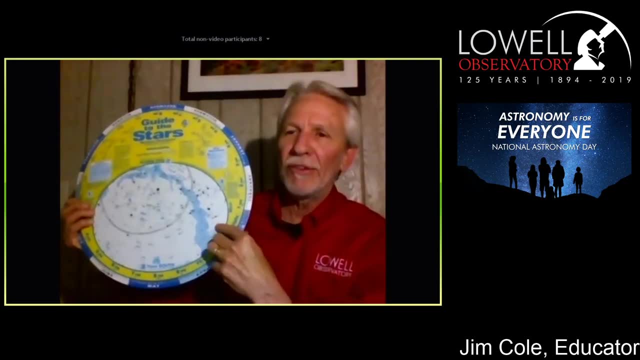 but it's basically a two-parter and there is an outer dial that rotates like this and an inner dial that shows in this window, and this is what you see as the night sky, and you can see that there's stars. the light's not too good. 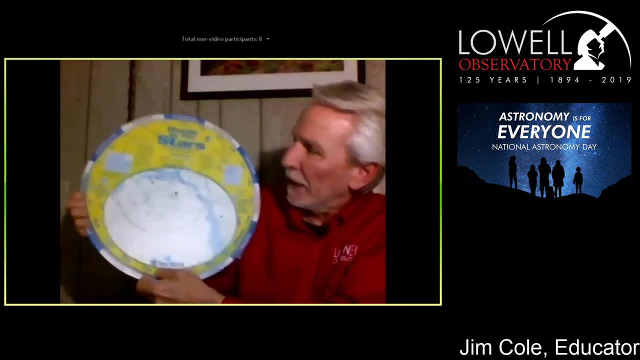 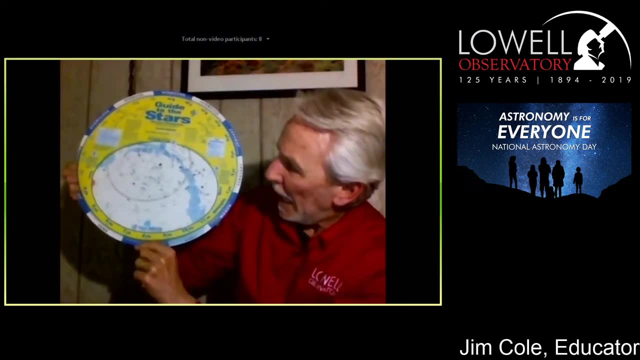 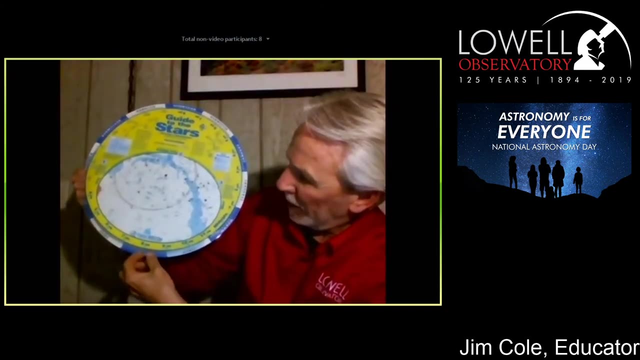 when I get too close. I apologize for that. the really cool thing about a planisphere, though, is on this rotating ring there are times for the 24 hours, and on the fixed part of it are the months of the year all the way around. so, for example, 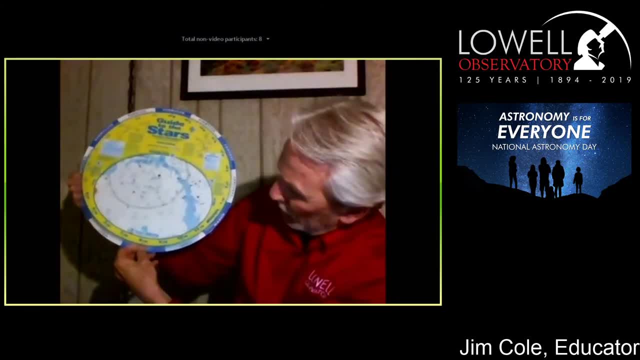 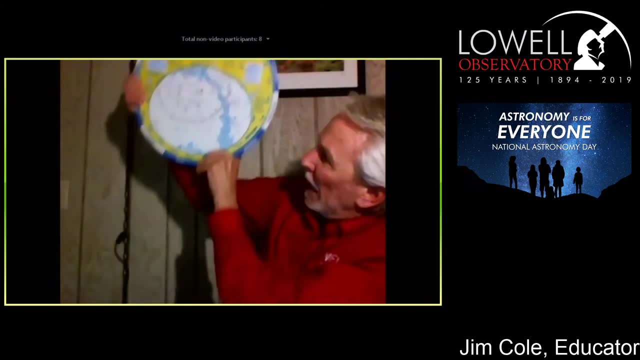 if I go outside it's about 8.30. I could put the 8.30 mark right on May 2nd and then hold it, and when I go outside and face south and put this over my head, it shows me the entire night sky. 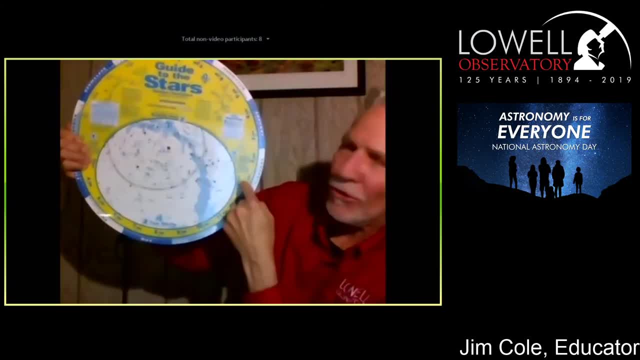 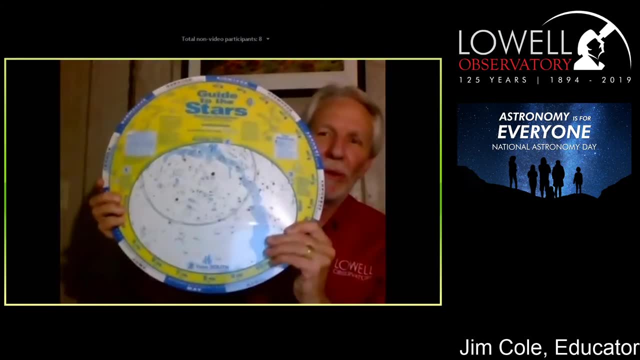 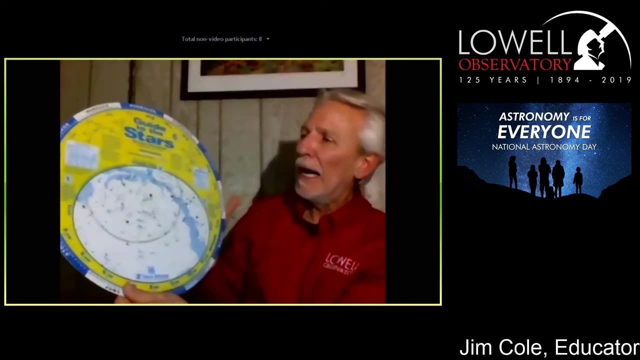 exactly like it's going to be. when you walk outside, you can see all the way down to the eastern horizon, the western horizon and the northern horizon. the benefit of these is that they're infinitely adjustable for any place in the northern hemisphere, usually around 35 degrees north. 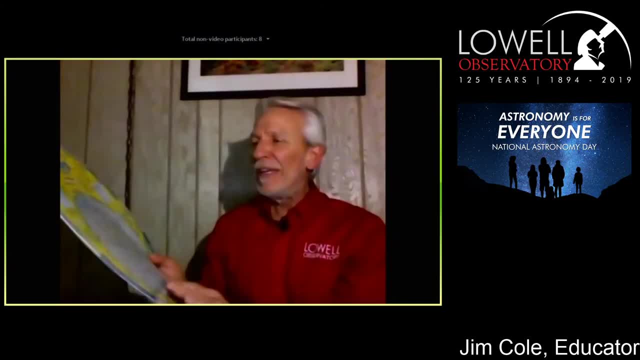 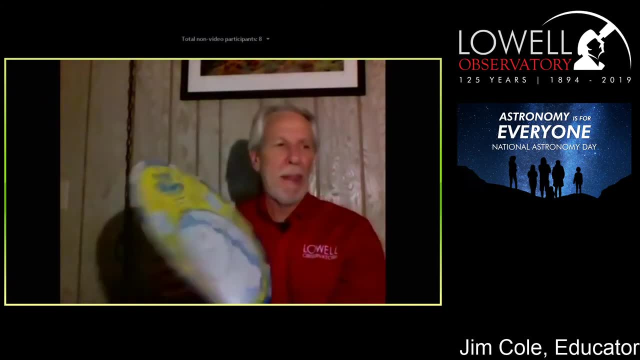 and the time and the month of the year will show you exactly what's in the night sky, and these are great for being able to see the big picture and start to relate patterns in the sky to the constellations. that's called a planisphere, available anywhere 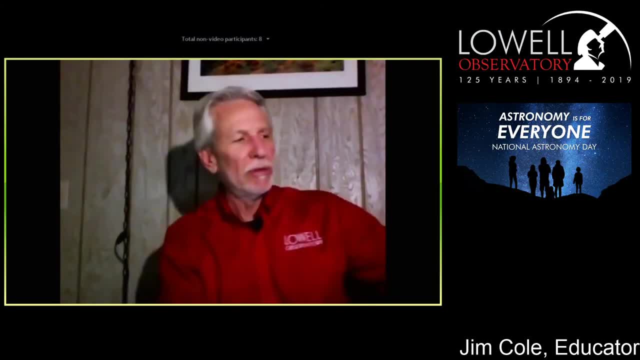 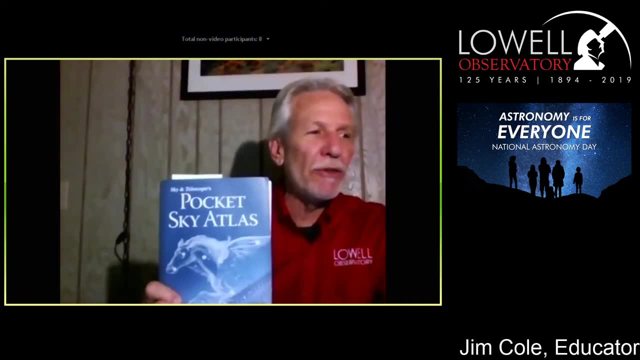 there's smaller ones too, but I tend to like the bigger ones. they're easier to see and no, it doesn't have to do with my age- although it could they have this either- but it goes along very nicely with the planisphere. this is a book called the pocket atlas. 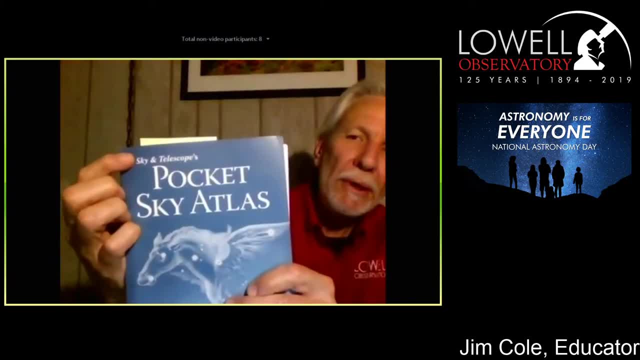 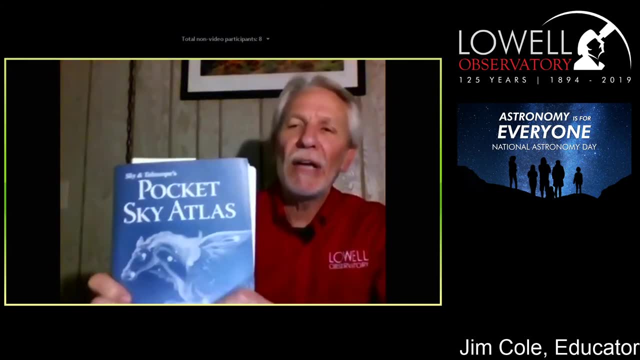 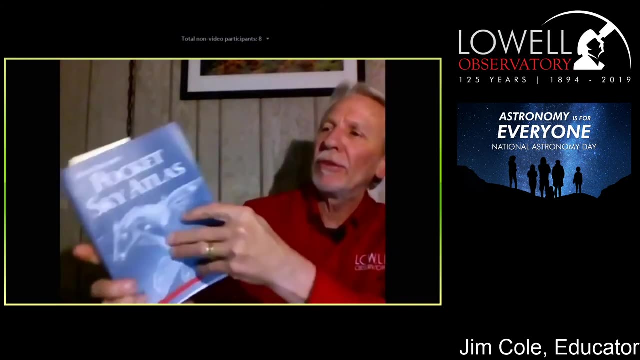 pocket sky atlas. it's by sky and telescope. these are about 20 bucks, as is the planisphere, and this is a more detailed sky atlas available through sky and telescope itself and also available through the starry skies gift shop at Lowell. but the idea here is it goes into 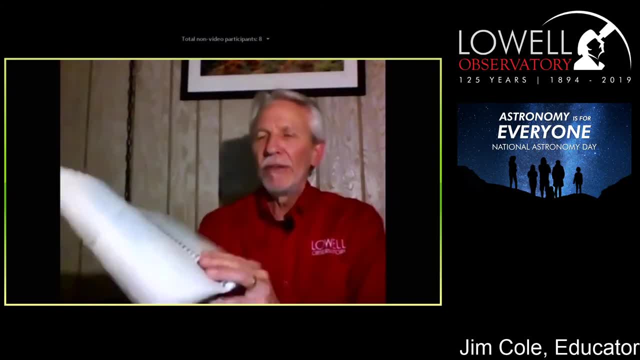 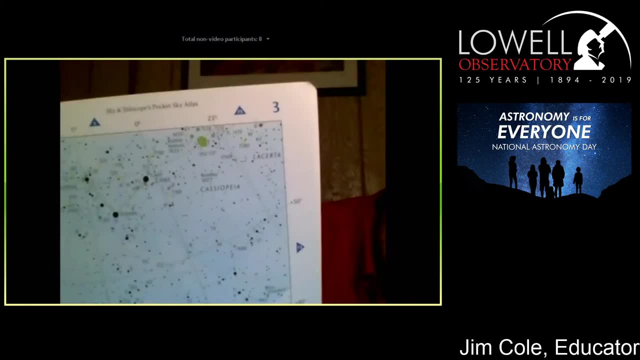 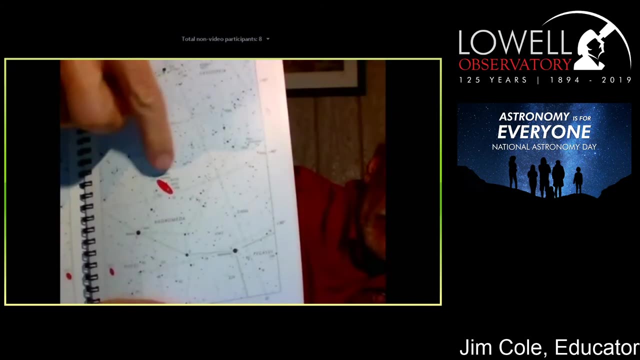 much more detail when you're looking at this. so within a particular constellation I can look- and this case is Pegasus- and I can see a whole bunch more detail than I can see on the planisphere. and it starts to point out quite a bit of detail where some of the 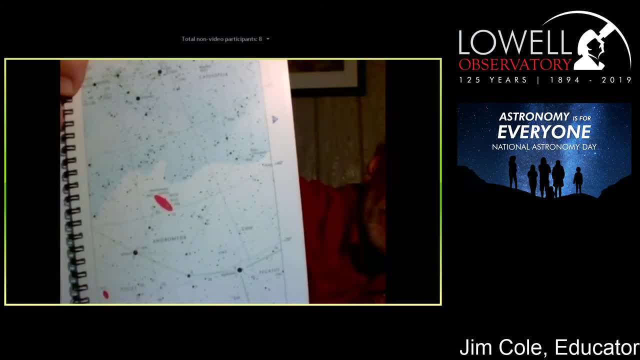 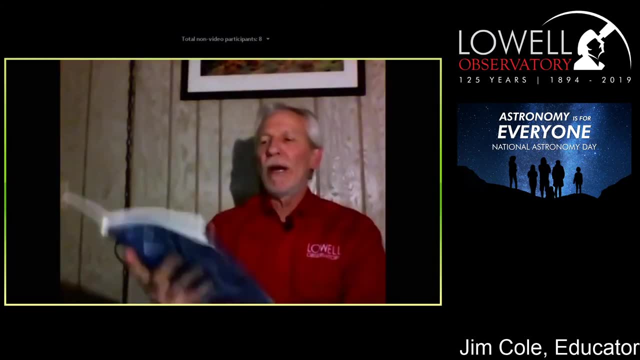 large galaxies are, and things that I can find through my binoculars and even naked eye if I wish. so this is kind of stage 2, and it's small enough to sit in your lounge chair and look at it without being too bulky. alright, so you need to have a map of the stars to go along. 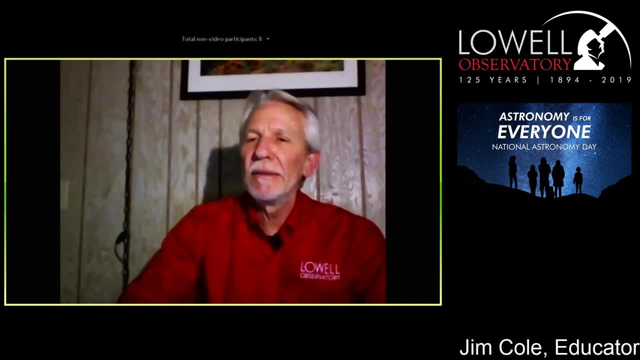 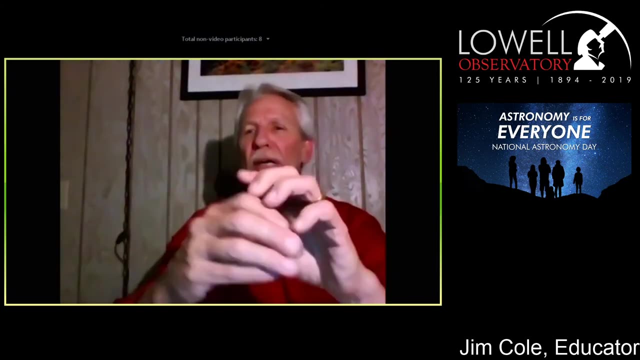 with your comfortable chair in a nice, safe, dark place to observe. so either one of those, or both together, make very good additions to your learning experience, and they're relatively cheap. alright now, fourth thing that you absolutely have to have this is a red flashlight. I'll turn it on in a moment. 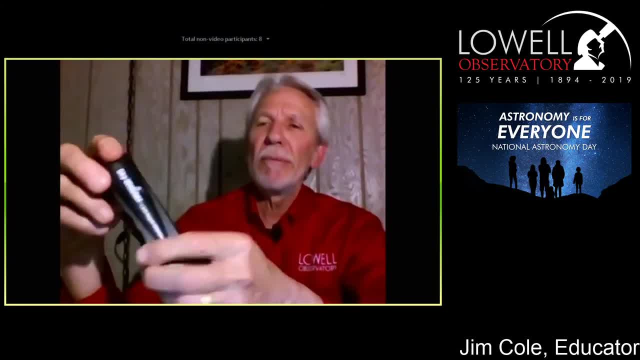 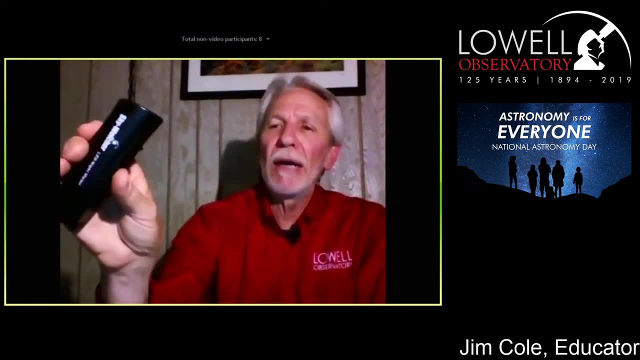 this particular one is by skywatcher. these generally run about $15 to $30. you can buy them in online stores, online astronomy stores. you can buy them at the starry sky shop at Lowell. you can buy them in many, many, many different places and there's many different. 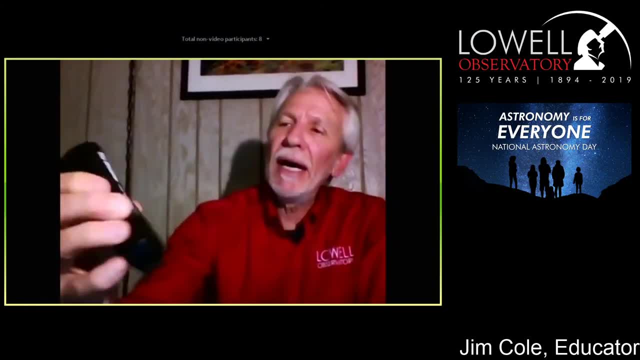 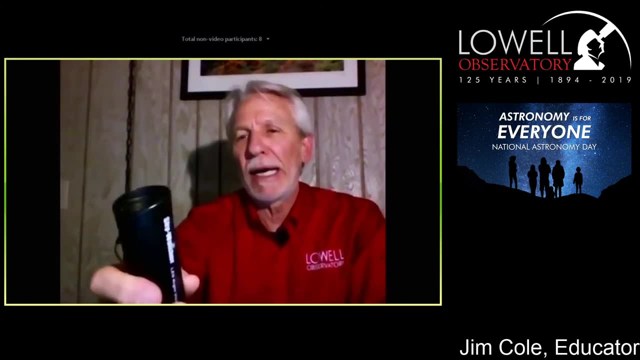 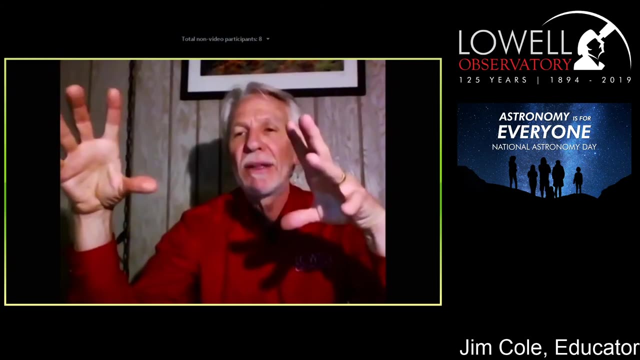 variations on red flashlights. alright, so the idea of a red flashlight here is that it won't destroy your night vision, and let's talk about that for a second. so when you walk or when you leave an area of bright lights, like most big cities, and drive out of the country, and you step out of your car and those car lights come on and you're kind of temporarily blinded for a minute and you throw a blanket on the ground. you look up at the night sky in about 30 to 40 minutes, the number of stars you can see. 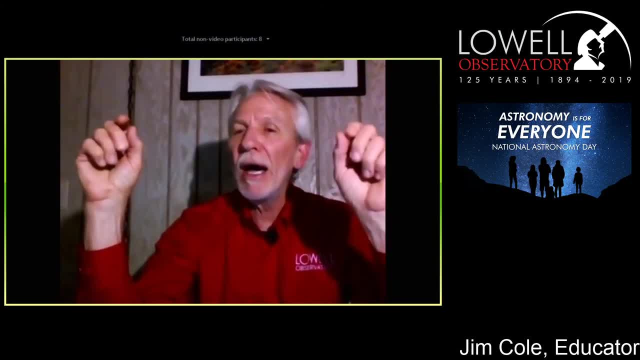 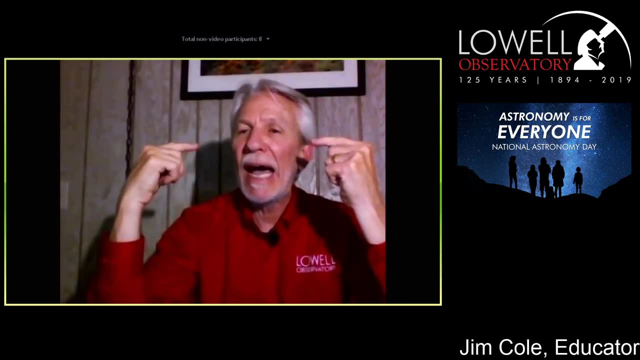 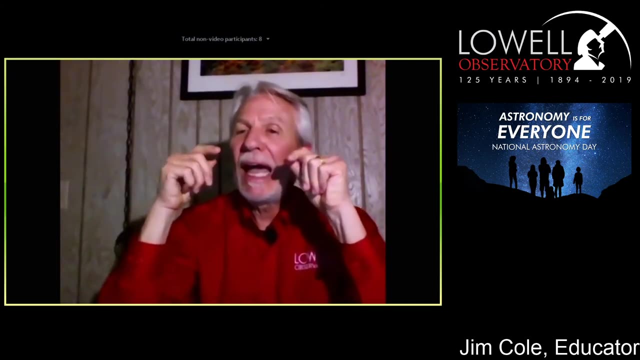 is incredibly larger, so your eyes, when you get away from bright lights, undergo a chemical process and it takes about 30 to 40 minutes for that to happen and basically the sensors in your eye that are responsible for daytime color vision are turned off and the other sensors. 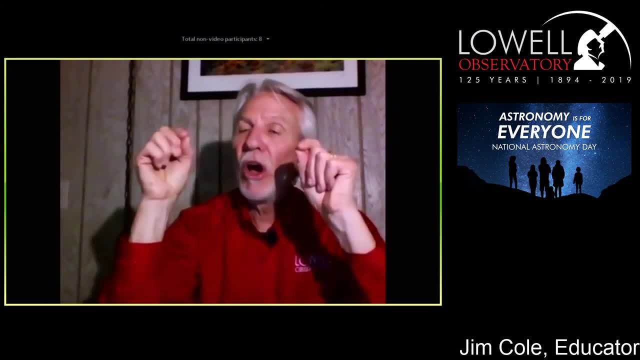 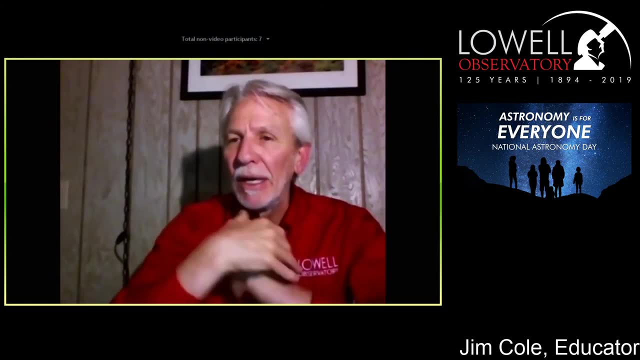 that are many thousands times more numerous are turned on, and these are very, very much more sensitive to light than your daytime vision, is indeed alright, they can see about a thousand times dimmer than your daytime vision can. so this is called your night adaptation, or your night vision. 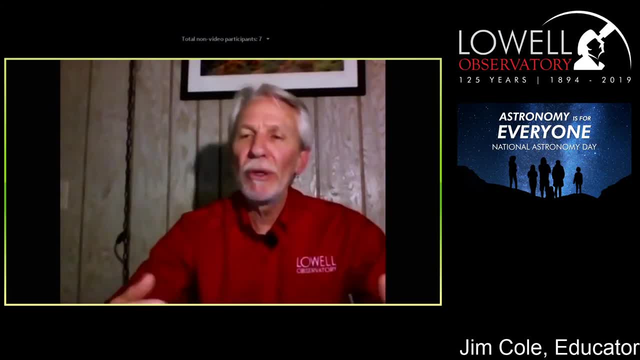 and this is one of the reasons I didn't want you to use devices. when you go out to learn the night sky, you're looking up at the sky, you turn the device on to look at the map and boom, the light comes on and you're blinded and that chemical process. 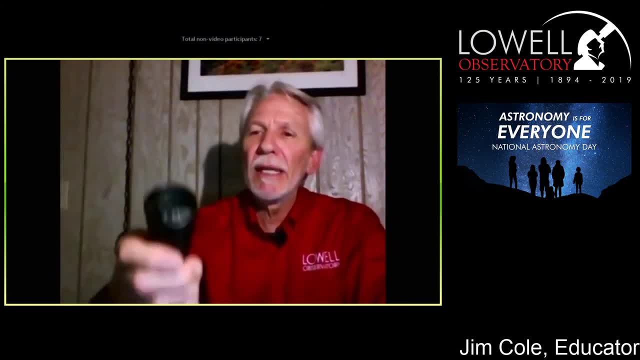 has to start all over again. so the thing about using a red light is that those low light sensors in your eyes, we call the rods, are less sensitive to dim red light. and I say dim for the following reasons: you can have a red light and if you have a dimmable, 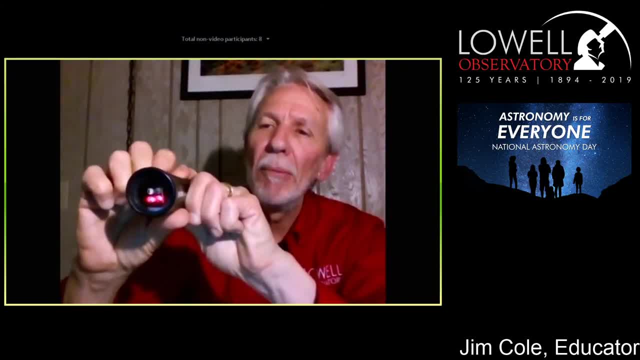 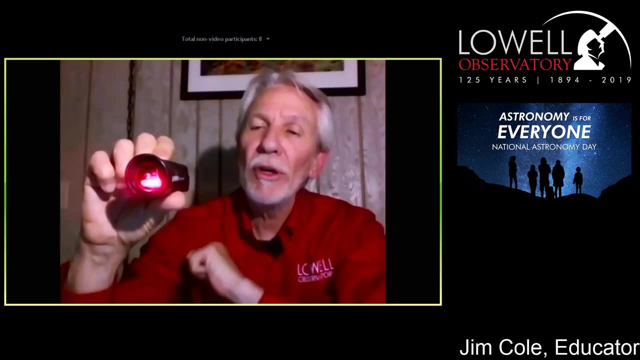 one. you can turn it on very, very dim and you can roll it up to a very, very bright light. now, if you're dark adapted, this is bright enough and it doesn't look that bad, but it's bright enough to actually activate your cones again and ruin your night vision. so you want. 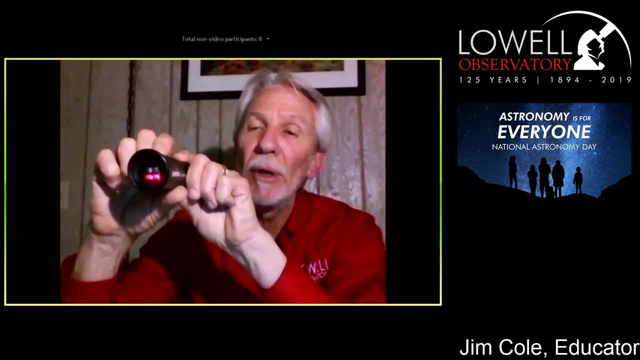 to have a light that you can dim way down, make it just barely bright enough to be able to read star charts and be able to still look up at the night sky and see the stars. so you really need a red flashlight to be able to read your charts, alright, so 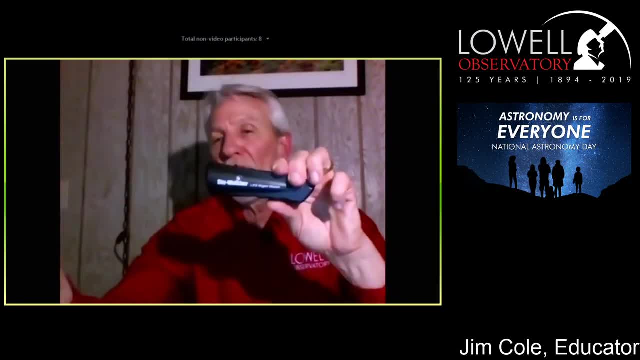 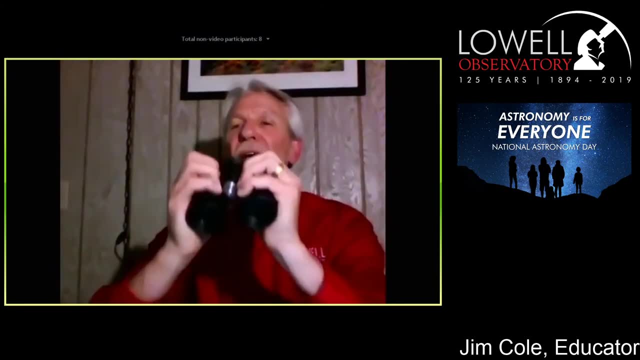 you need a location, you need a comfortable chair, you need a set of charts to show you where the stars are in the sky, and you need a light. finally, and this is the thing, that is not necessary for you to start learning your way around the night sky, but once you, 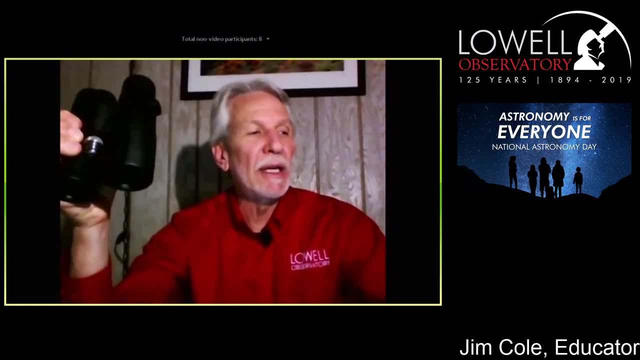 start to learn the constellations, you'll notice that when you look on the pocket sky atlas or on the planet sphere itself, there's lots of little cool things that are marked, little star clusters and galaxies and things like that that you can't really see too well with your naked eye. 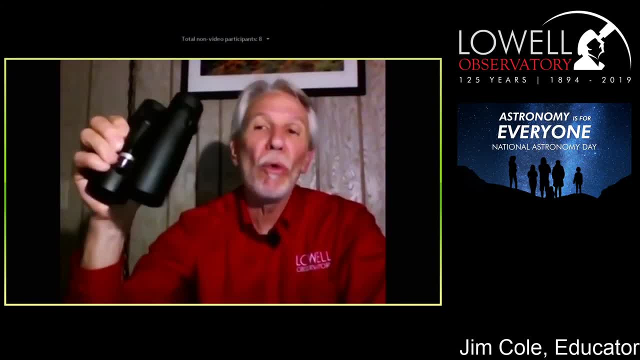 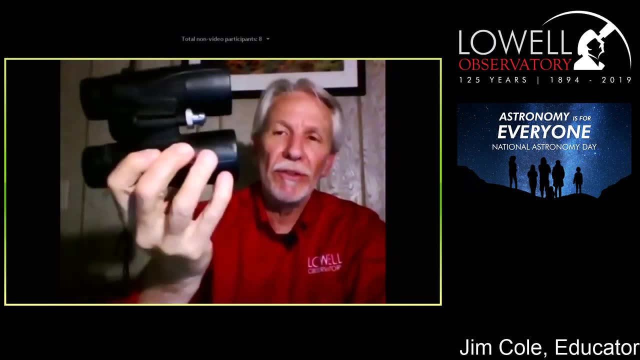 binoculars allow you to see about 40 times more stars than you could with your naked eye, and I'm talking about small binoculars. these are called birding binoculars. it's not a brand, it's just the type. once you see most people walking. 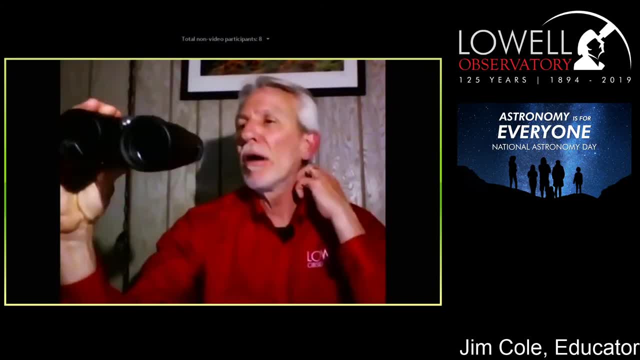 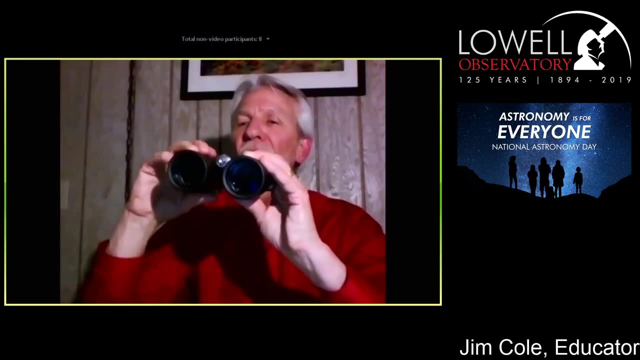 around the forest looking at birds with. these are an 8 by 42 version. the magnification is about 8 times 42 is the size of the optics in the front. the idea is to get something lightweight that you can still see much more with. it'll magnify enough to. 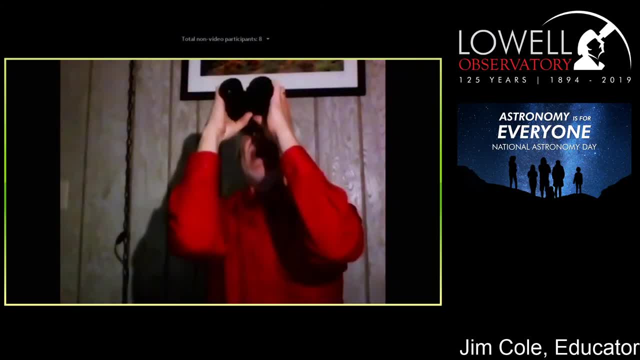 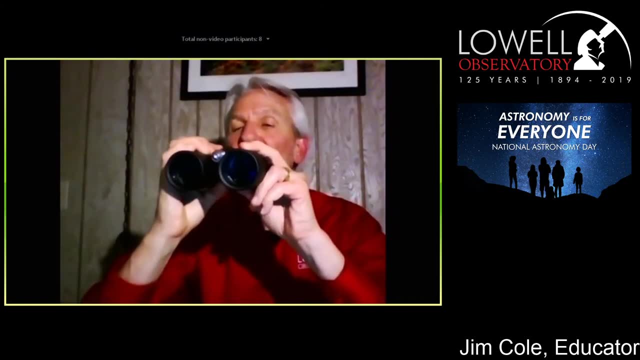 see incredible things in the night sky, but yet when you're laying back, your hands and arms can support them, while you're supported on a nice comfortable chair and you can sweep the night sky for hours with lightweight binoculars. many astronomy binoculars are too heavy. 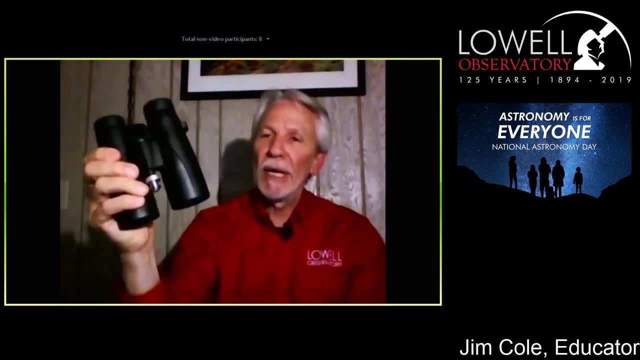 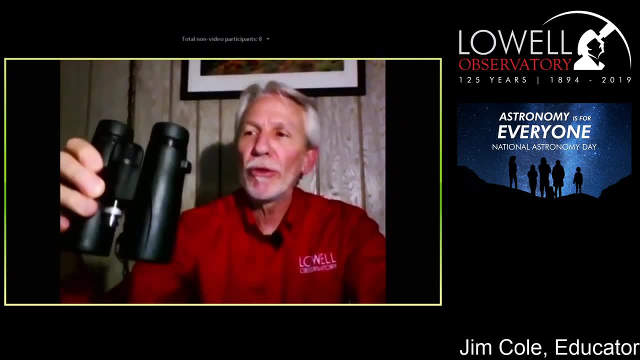 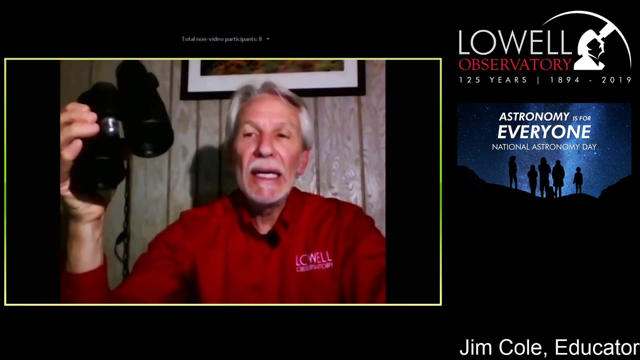 to actually hold comfortably. so the binoculars you can add, and binoculars from a good pair to a very good pair, from about $150 to about $300. you can spend thousands on binoculars. it's not necessary you want to stay away from the most inexpensive. 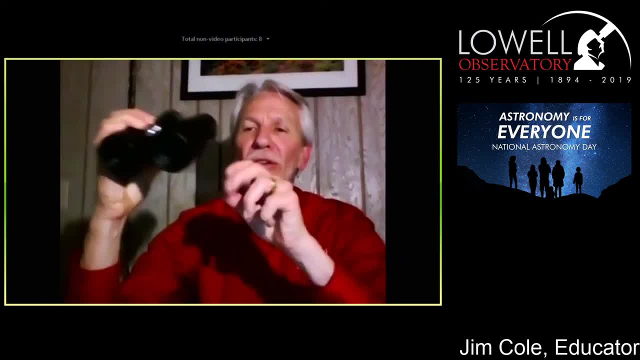 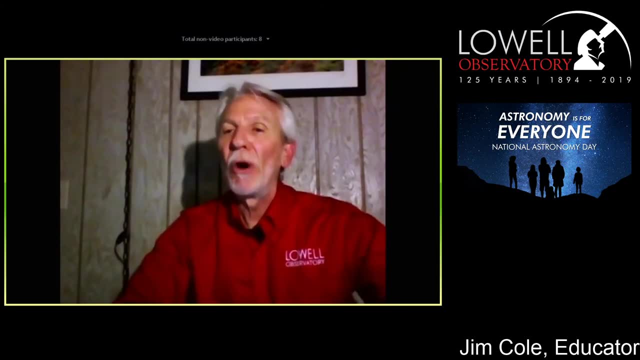 ones, because they're very difficult to see through and there's a lot of aberrations and they don't look very good. but in that $150 to $300 range you can get a very, very nice pair of binoculars. so now you've got your. 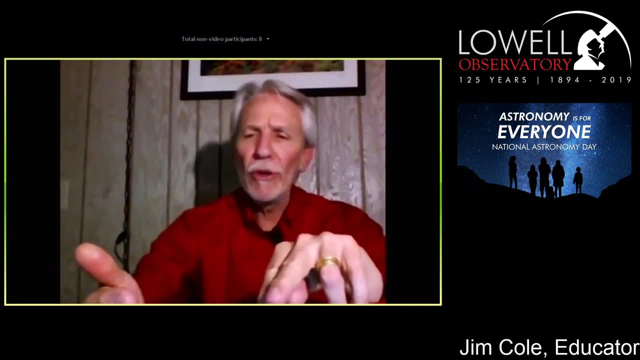 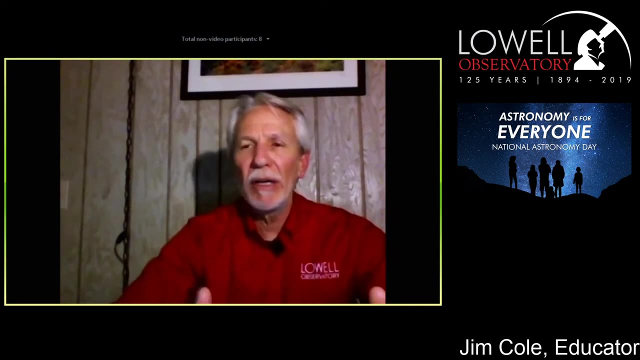 observing sight. you've got your atlases, you've got a comfortable chair, you've got a red light to read your atlases and you've got a pair of binoculars. at this point, you just want to go out as often as you can if you're using your own backyard. 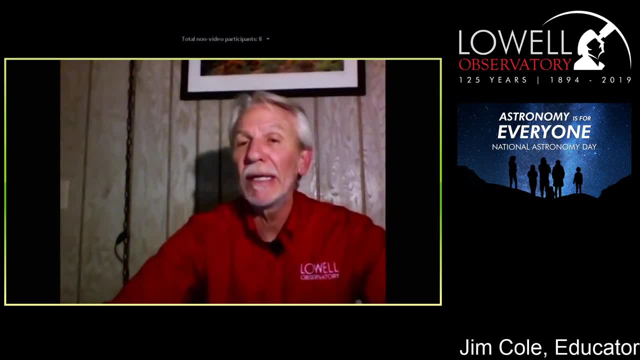 it can be a nightly or every other night, whenever you have 5 minutes or 10 minutes if you have to drive somewhere or walk somewhere. it's going to be a little less often than that, but the more you go out, the more you'll learn. so what you want to do initially is 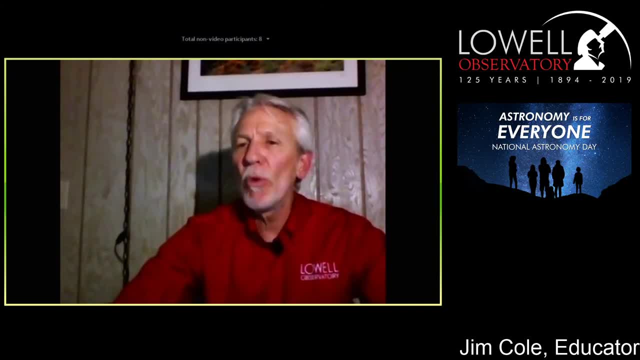 to learn. the brighter constellations and the more you go out, you can start to see the hourly change in the way the stars move across the sky due to the turning of the earth on the day- night cycle. you'll see that the monthly changes in the stars that are up. 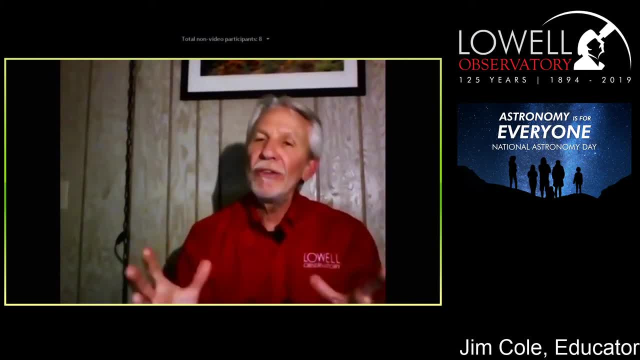 because of the earth going around the sun. you'll see seasonal changes where the changes are even bigger, and you'll be able to start to map all this stuff in your head and start to see how our solar system works and why the sky looks different all the time. 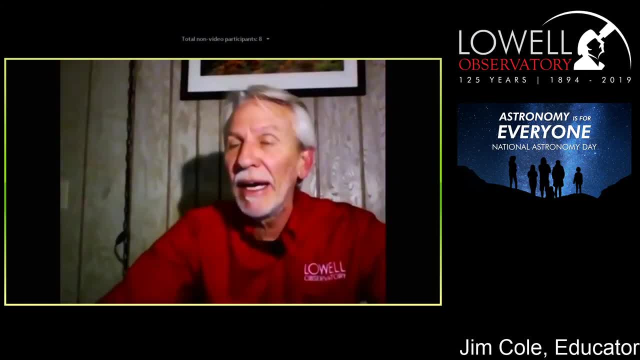 don't forget to look at the moon- it's the brightest thing, easiest thing to find, naked eye or with your binoculars- and don't forget to notice how it changes. and this is an every night thing. so the phases change every night. some nights the moon's not even up for several days. 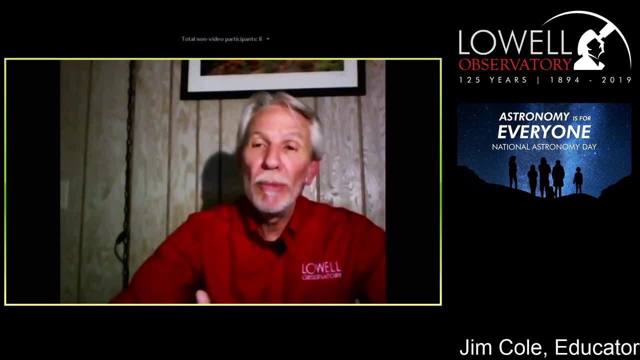 and other times it's up in full moon mode and it's very bright and makes it very difficult to see other stars. most importantly, and I'm going to leave you with this, have fun and learn, read, go to science presentations, visit museums, visit observatories, visit planetariums. 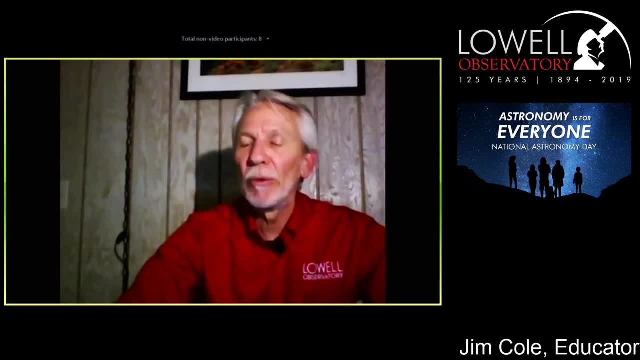 go to star parties, join a local club and just have fun with it. as I mentioned earlier, I was 40 years old when somebody gave me my first telescope, and it's been a life long passion of mine. I'll go back to that word that one of our astronomers used. 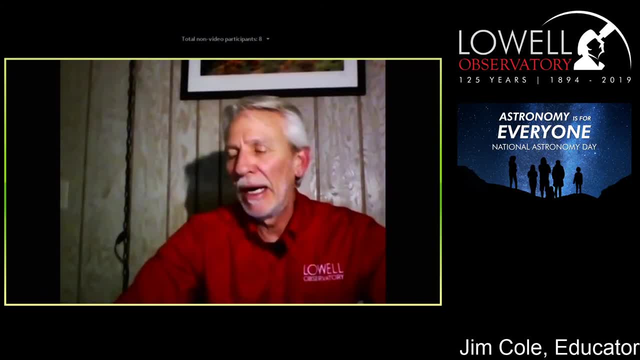 a little while ago, Michael West, it's all about passion, or was it? Kevin Schindler? can't remember where that came from, but anyway, it's all about the passion. I'm going to leave it with you and I think I'm going to go back. 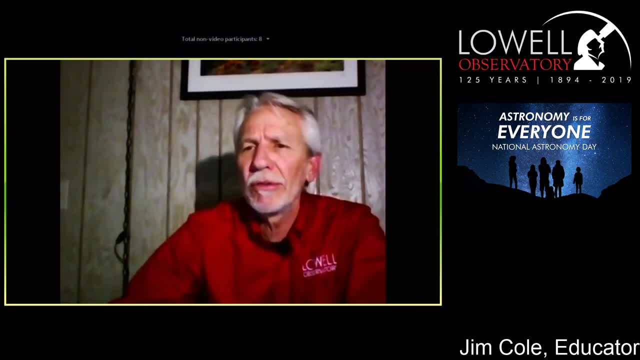 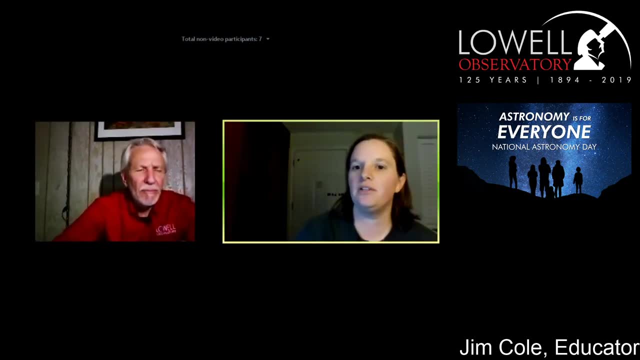 I think Sarah is off right now and we've got Curtis. that's going to be the emcee, if I read that right. oh, Sarah's back. it's still me, Jim, but you do have a couple questions, so I'll leave you with those. alright, so let me get. 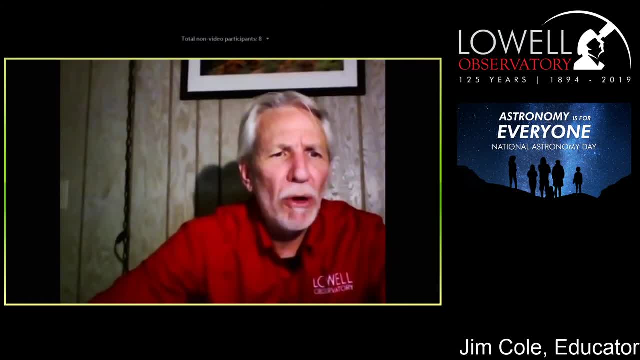 down here, alright, Summer. hi Jim, what in the night sky are you most passionate about, and why? um, I have to say, well, gosh, there's a lot. that's one of those bread questions. they're all good, but I'm going to call out three real quick. 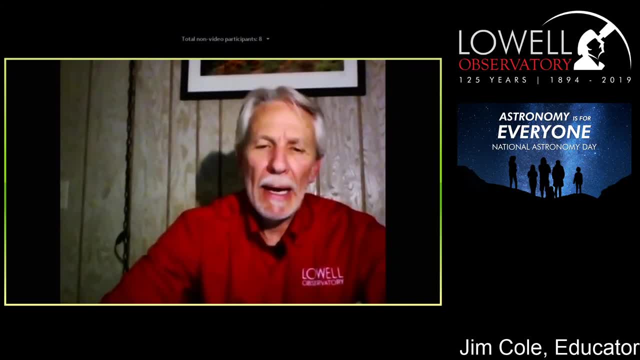 I love looking at places- star nurseries like the Orion Nebula, where stars are being formed. we call them stellar nurseries, and that's what's happening as we look there. I love looking at things called globular clusters. they're probably my favorite visual thing to look at. 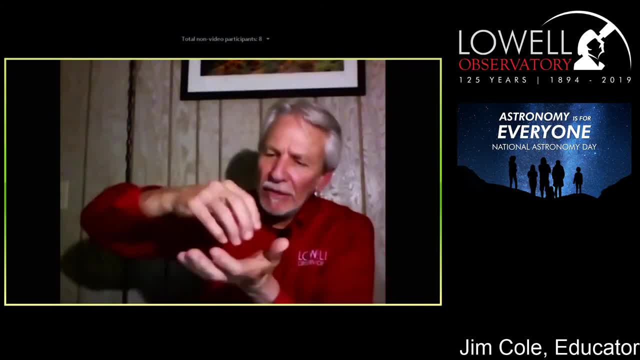 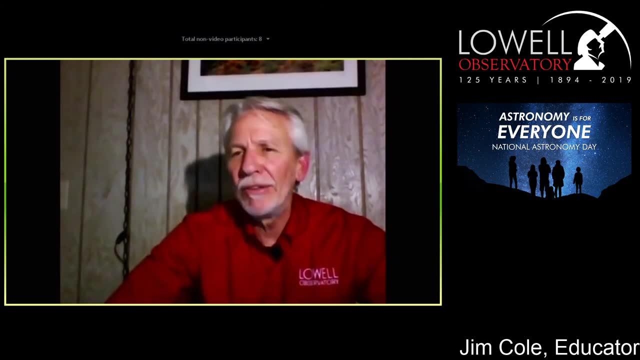 balls of hundreds of thousands of stars in really small places. it looked like diamond dust sprinkled on black velvet when you looked at them through a binocular or a telescope. and then, of course, galaxies other than our own. Milky Way, just understanding how far away you're seeing. 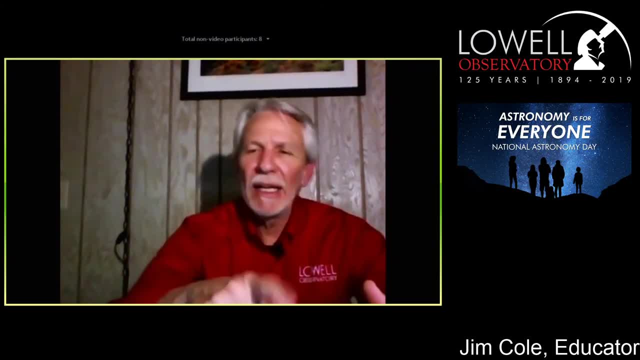 the light travel and the entire galaxy in your Milky Way fitting in your field of view as you investigate these things. so all three of those are really my favorites. alright, thanks, Summer for the question, and David, how can we make a telescope at home to see a normal eclipse? 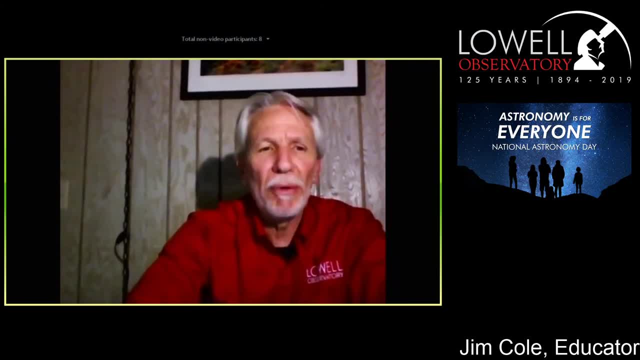 okay, that is a little bit beyond the scope of this talk, but you can actually watch a solar eclipse with a hole punched in a cardboard, piece of cardboard and project that goes down to the ground. so there's many, many simple ways to do that. maybe that's something we can address. 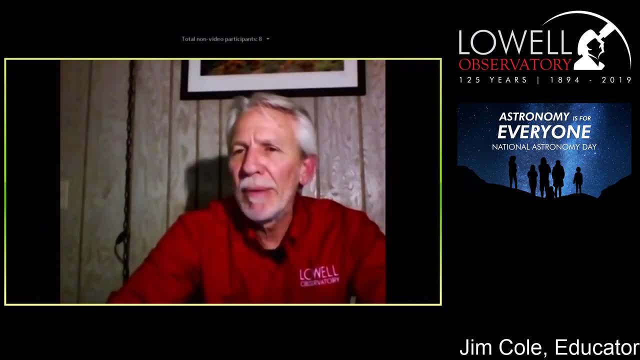 in a future episode of this, but it's a little bit tough for me to get into that right now with the amount of time that we have allotted, but it's a very, very good question. hopefully, if you Google that or you get onto places, there's a good website. 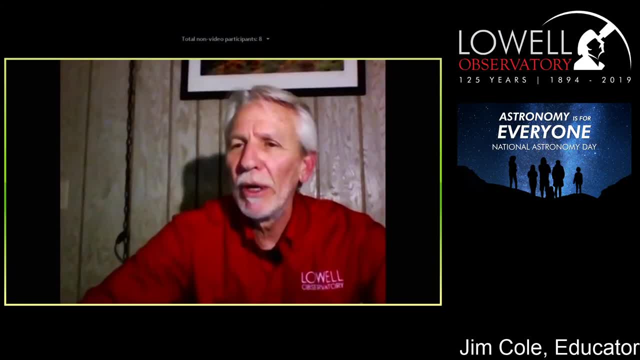 the largest astronomy forum in the world is called Cloudy Nights- kind of a play on words, because when you can't be outside observing, it's usually because it's cloudy. it's not about amateur astronomy. there's a lot of information on cloudynightscom and I invite you to join in sign up. 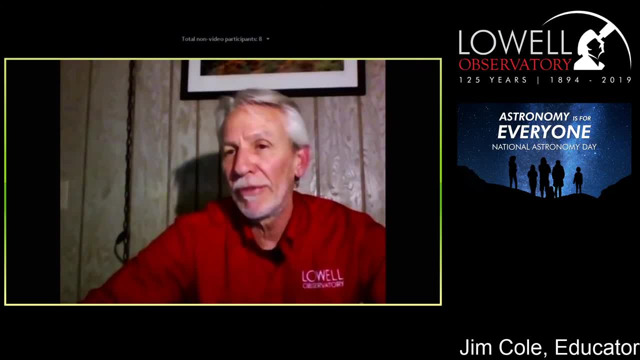 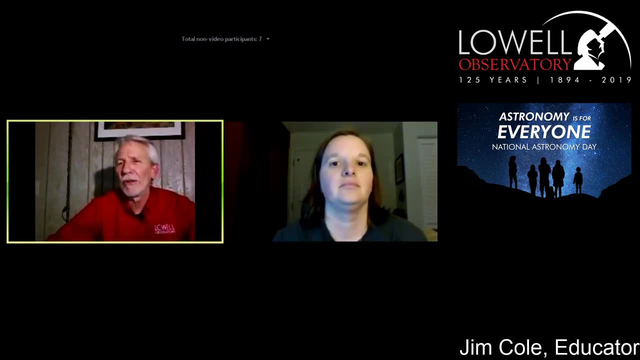 and go onto some of the beginners forums and start learning all kinds of cool stuff there. so, and let's see here, and a little note: don't look at the sun with a telescope unless there's proper filtration on it or the telescope is designed to do specifically that. and that was a good call on your part. 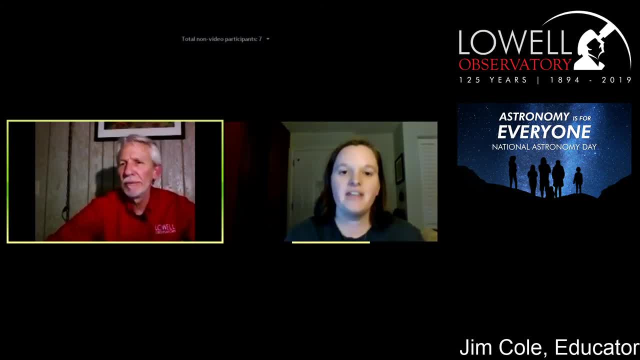 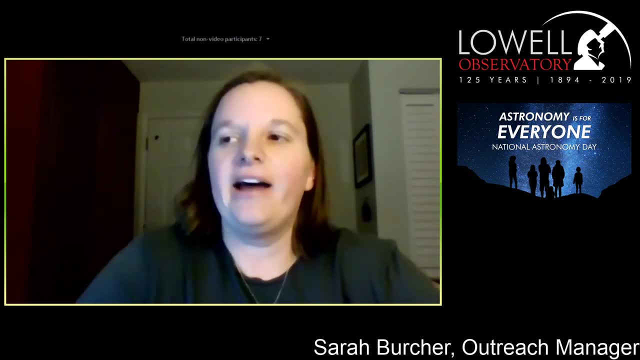 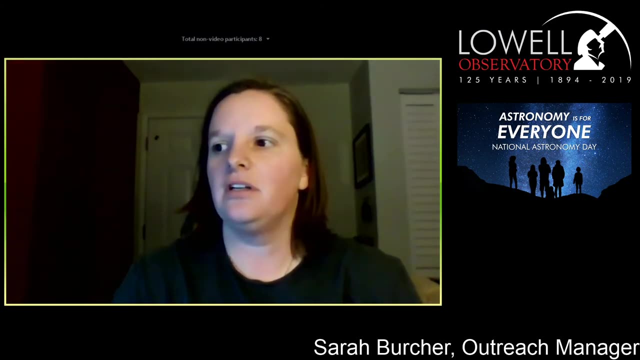 thanks a lot. any other questions? I don't think so. thank you for your time. Jim, you're welcome. alright, so I am now going to turn it over to myself and I am going to give you guys another activity. we learned from Kevin how to turn your. 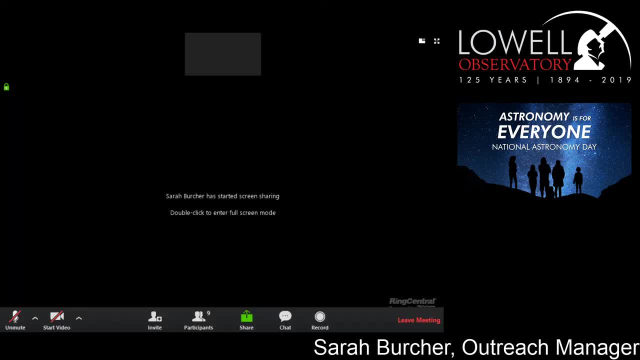 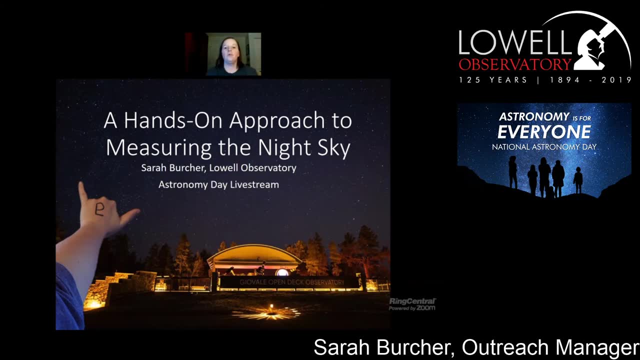 how to turn a simple plastic cup into a into the night sky, but I am now going to talk to you about how to use your own hand to measure the night sky. alright, I won't let you see that this is going to be a presentation wrought with poorly drawn illustrations. 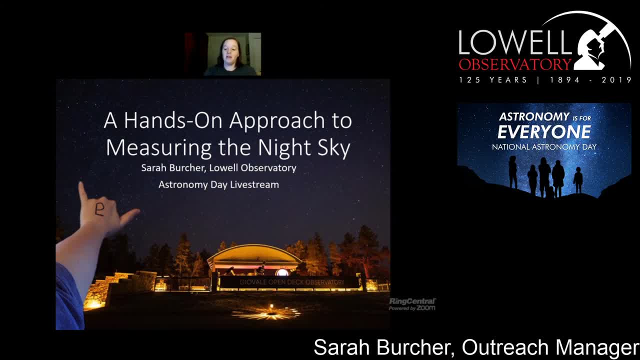 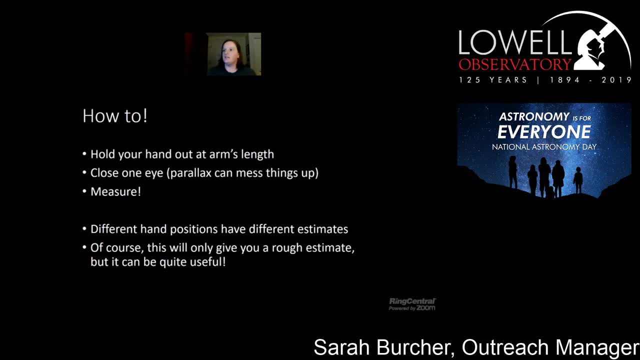 and poorly shot, poorly photoshopped photos. so bear with me there. so what do you do for this? what you do is you hold your hand out at arms length. you then close one eye. parallax can mess things up, and then you measure different hand positions. different ways you can arrange your hands. 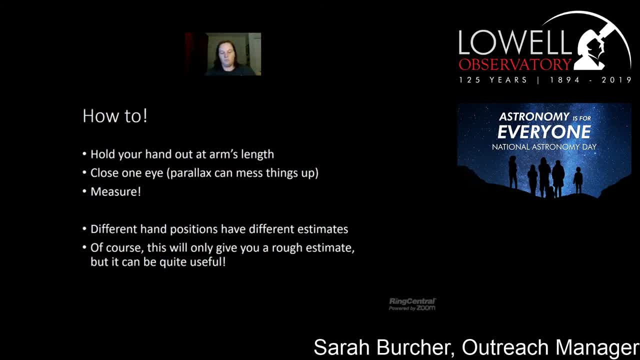 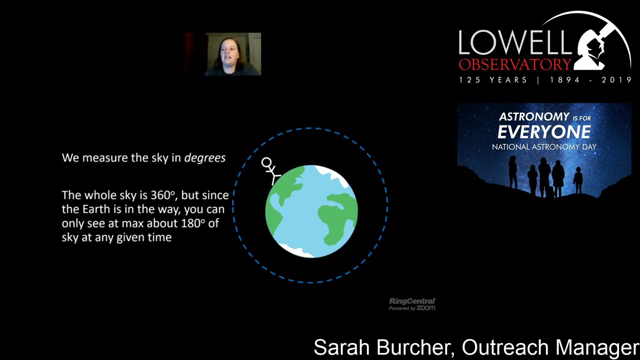 we'll have different estimates, but we'll get to that in a second and, of course, this is only going to give you a rough estimate of the night sky, but it can still be pretty useful. so let's first get some background. we, we being astronomers, we being people. 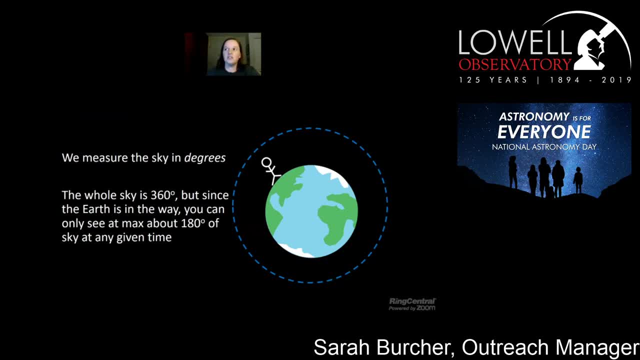 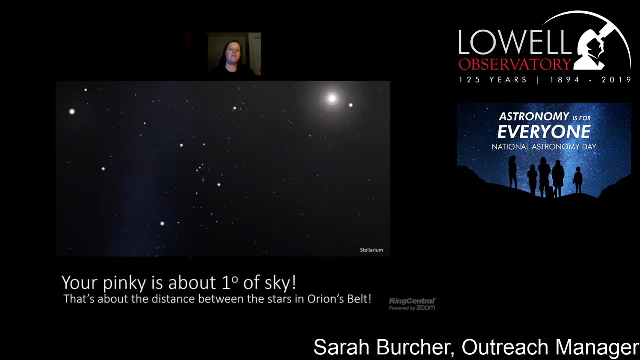 measure the sky in degrees. the whole sky is 360 degrees, but since the earth is in the way, you can only see a max of about 180 degrees of sky at any given time, right? so if you take your hand, hold out your pinky, your pinky is about one degree. 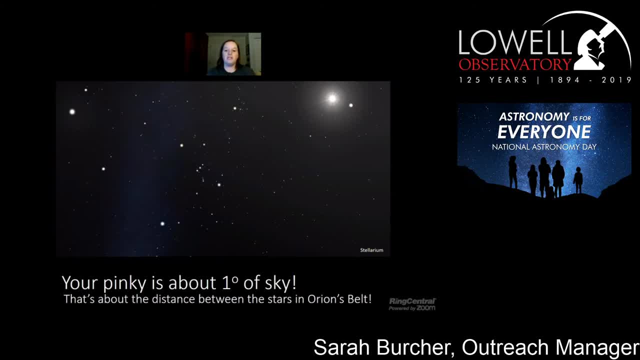 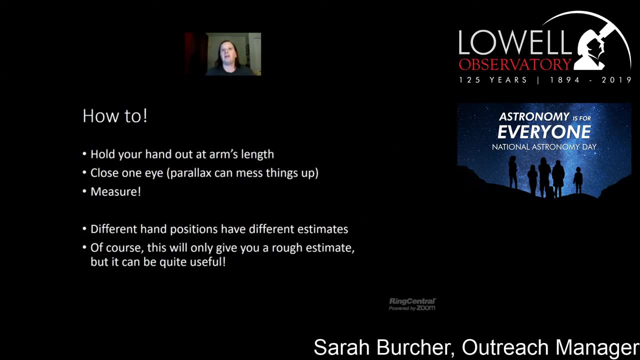 of the sky, which, by the way, is about the distance between the stars and Orion's belt. I did. I want to go back real quick, though, to talk about parallax. so I tell you to close one eye here, and that's because if you hold out, say your pinky. 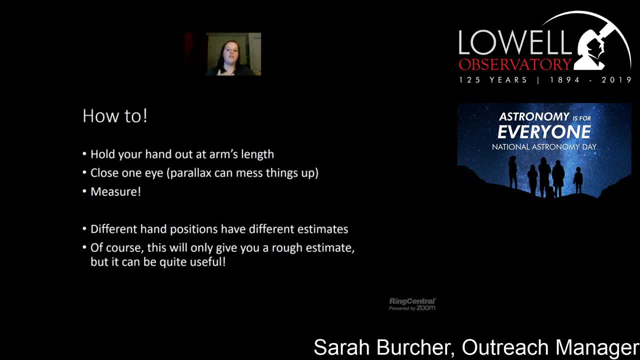 and blink from one eye to the other. your pinky actually moves from your perspective because you're shifting slightly from where your pinky goes, so make sure that you're always looking out of the same eye when you're measuring something. so your pinky about one degree of sky. 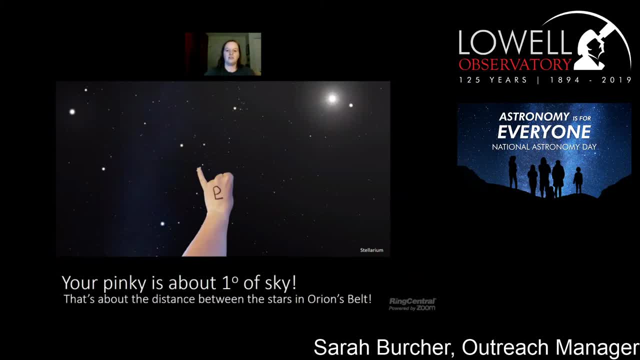 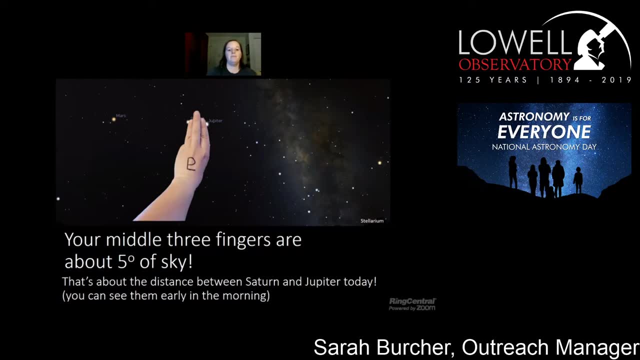 which is not a lot of sky, between the distance between the stars and Orion's belt. your middle three fingers are about five degrees of sky, which right now is about the distance between Saturn and Jupiter, and later on we're going to watch a video that's going to talk to you about what Saturn and Jupiter. 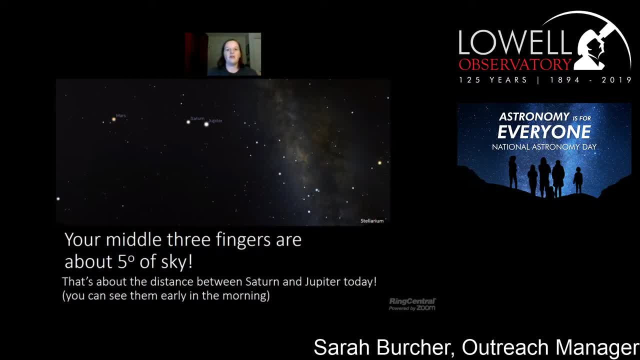 are doing. that's kind of fun. they're moving kind of closer together over the next year but right now, well, actually it'll be a really fun thing to do to continue to measure them over the next couple months up until about December, as they get closer and closer. 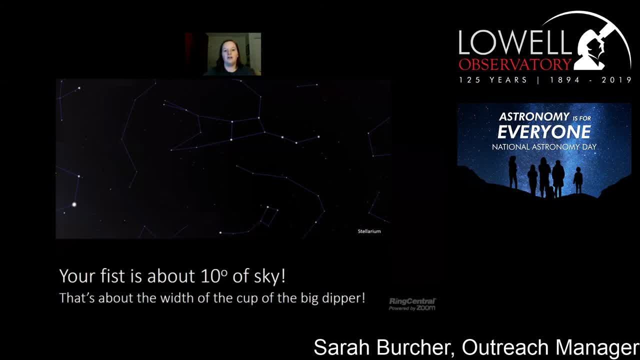 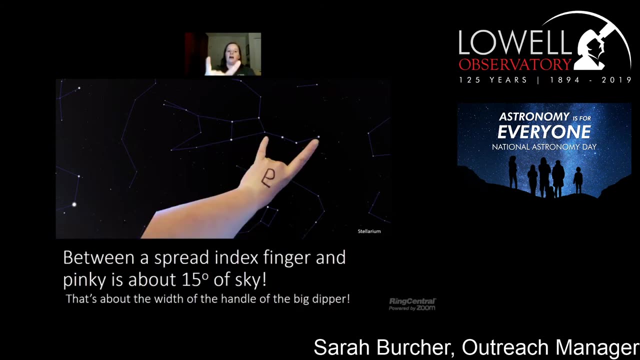 but right now in the morning they are about five degrees moving on. your fist, held out at arm's length, is about ten degrees of sky and that is about the width of the cup of the Big Dipper. cool, you can do another one if your spread index finger and pinky. 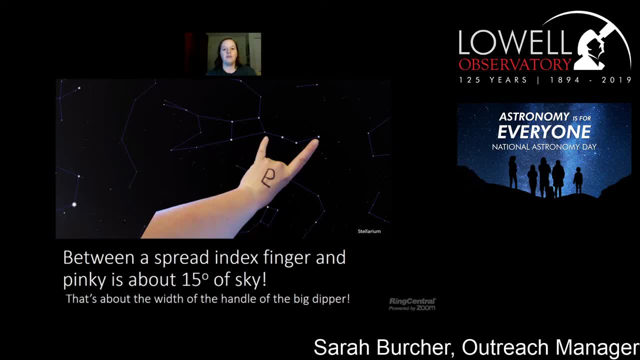 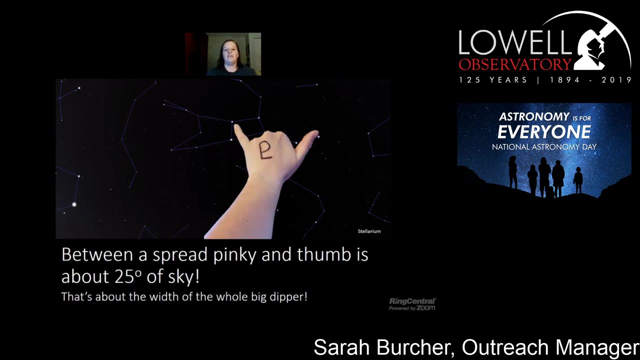 is about fifteen degrees of sky, which is actually about the width of the handle of the Big Dipper. I picked the Big Dipper because it's easy to find and everybody can do it. now, if you put those together between a spread, pinky and thumb is about twenty-five degrees of sky. 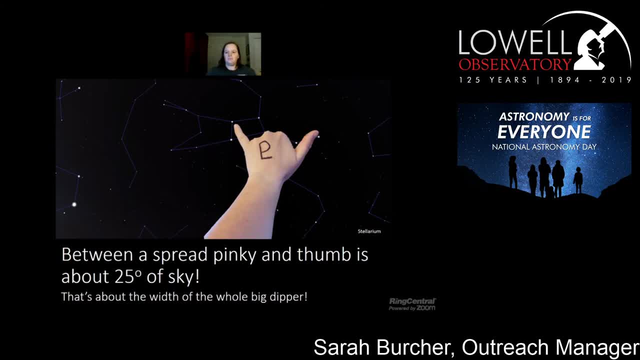 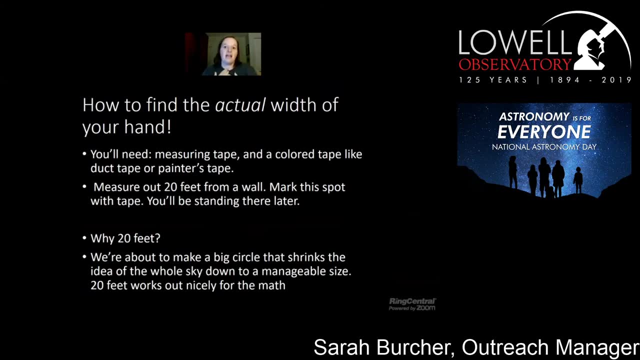 and that's about the width of the entire Big Dipper. cool. so you may be thinking to yourself: well, maybe my hand size is different than somebody else's hand size, maybe my arm length is different than somebody else's arm length, and how do we reconcile that? 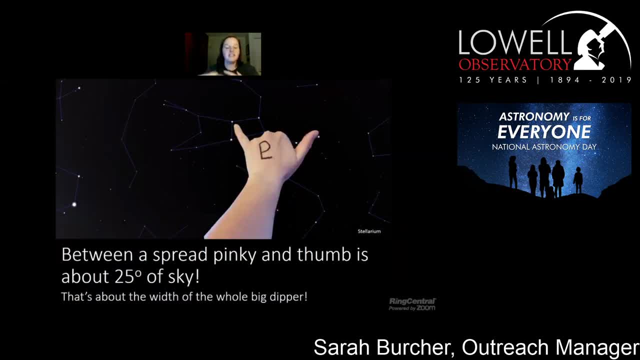 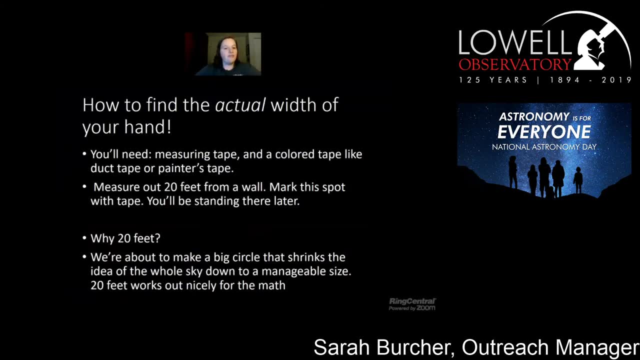 well, these estimates I give you are actually pretty good for a lot of people, even kids. but if you want to get more particular with it, we are going to do a fun little activity now, or I'm going to explain to you how to do a fun little activity. 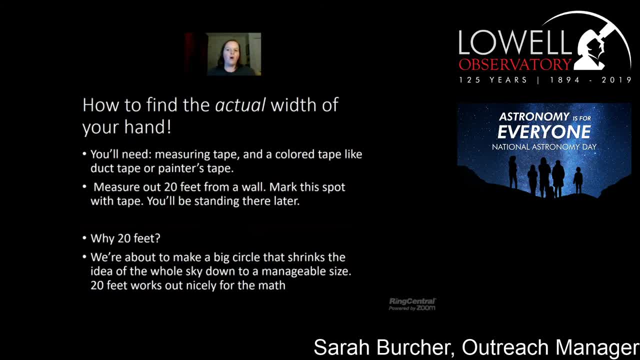 first thing you'll need is some measuring tape and just something you can stick on a wall, like colored tape, duct tape or I used painters tape. the first thing you're going to do is measure out twenty feet from your wall, mark that spot with tape why you're going to do twenty feet. 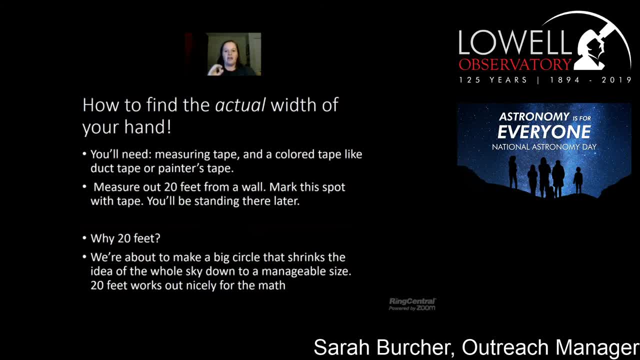 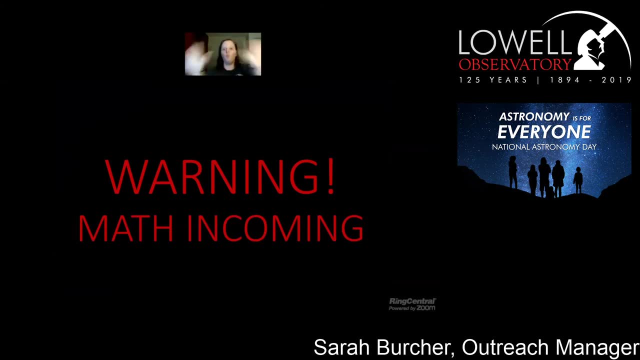 is that we are about to make a big circle and that big circle is going to shrink the sky, the big circle of sky, down to a manageable size, and twenty feet is good for the math. now there is math upcoming, so be warned. you can tune this out if you like. 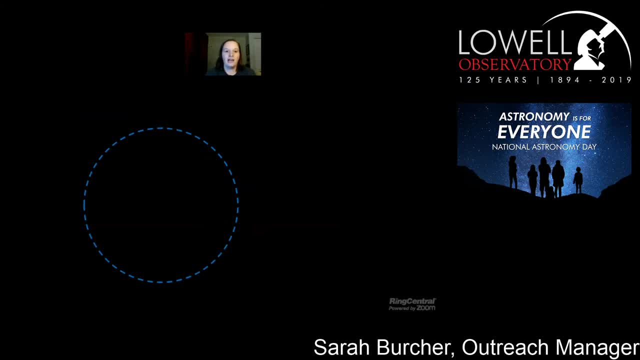 and just take my word for it later. but here is our sky: big, big, big sky. but this time our sky is only twenty feet in radius instead of billions of miles, so you are going to stand twenty feet away from your sky, or from your sky, which is now the wall. 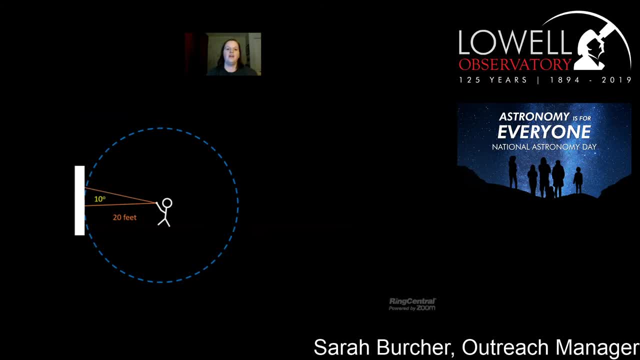 what we are going to do is we are going to carve out a ten degree swath of sky wall, but what we have to figure out now is how much of your wall is ten degrees of sky? alright, so let's get to the math. let's calculate the circumference. 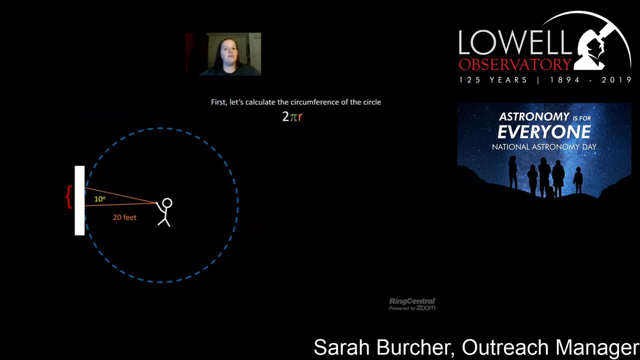 of our twenty foot radius circle. if everybody remembers from geometry we have two pi r, r being the radius. so two times three point one, four, one five, nine, carry on times twenty feet, which brings us to about a hundred and twenty five point six, six feet, and that encompasses 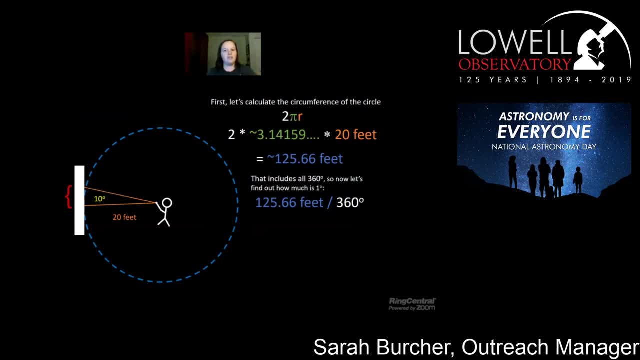 all three hundred and sixty degrees of our circle. so let's find out how much is just one degree of circle? we have point three five feet for a degree, but we want ten degrees. so let's multiply that by ten. per degree times ten degrees equals three point five feet. 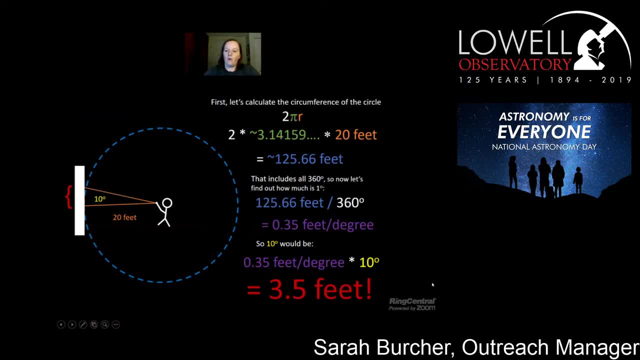 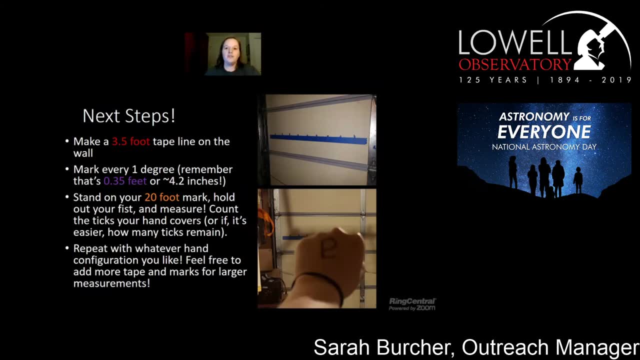 that's what we are going to do and mark that on our wall. so there was not a space in my house that was twenty feet apart from anywhere else, so I used my garage. so you can see that I have made a three point, five or ten degree. 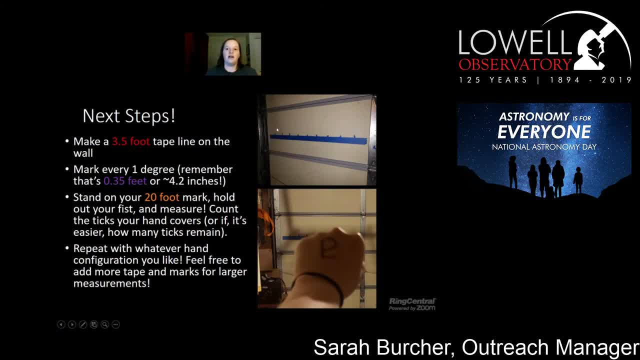 foot tape line in my garage, and what I've also done is marked every degree, which we've already done. that math, that's point three, five feet or four point two inches, more or less. so all you have to do, stand on your twenty foot mark, hold out your fist. 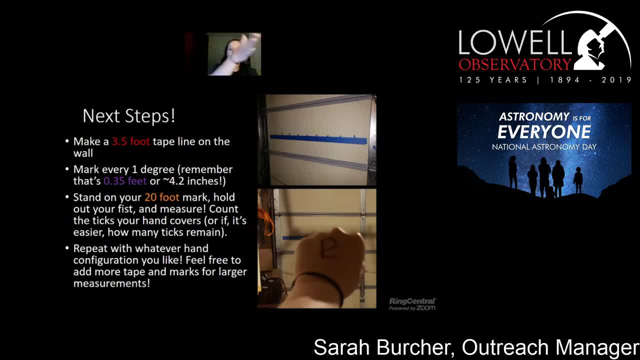 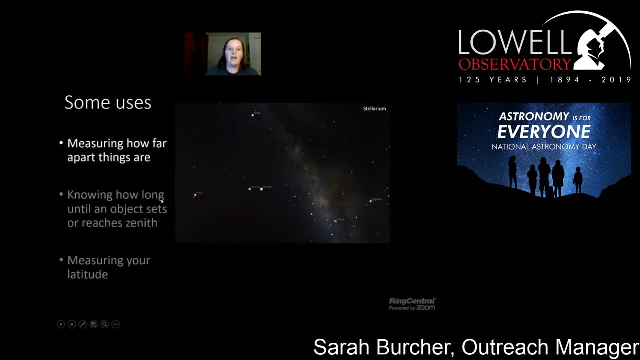 or whatever bit of your hand you want to measure and count the ticks that your hand covers or, if it's easier, how many ticks remain. so then you can repeat with whatever, whatever hand configuration you want. you can make your your thing longer if you need. you may also be. 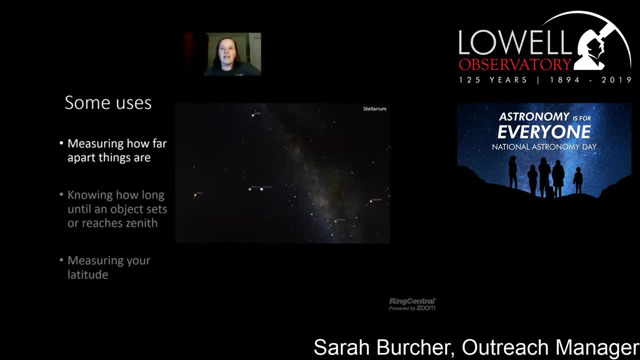 thinking. alright, now you've shown me that I can use the sky, or use my hand to measure the sky. what good is that to me? well, you can measure how far apart things are in the sky. I've already used Jupiter and Saturn, but what if you wanted to measure between Mars? 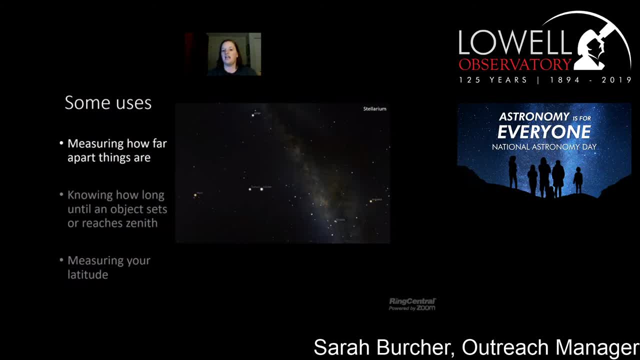 on the left there and not Mars, which is Antares on the right there. so you can just start measuring. I've got my approximately twenty five degree spread out and just keep going. ends up about eighty degrees right, and of course, the more times you do this, the more. 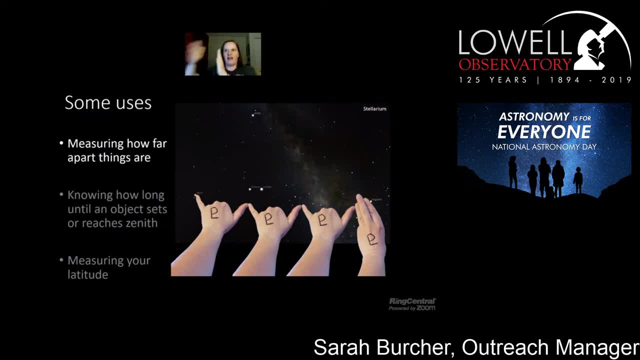 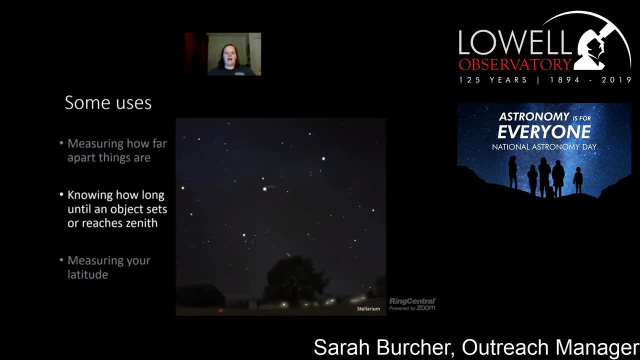 the farther apart something is. it's going to get less and less precise because you're adding a whole bunch of uncertain numbers onto each other. but it's a pretty good estimate. you can also know how long it is until, say, an object sets or an object moves a certain distance. 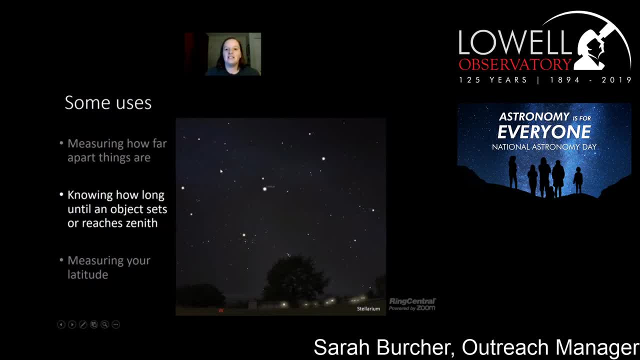 across the sky. so let's do a hypothetical. let's say Venus here is setting in the west and you have some friends coming over, but they're running a little late and you're scared that you're not going to be able to show your friends Venus through your binoculars or your telescope. 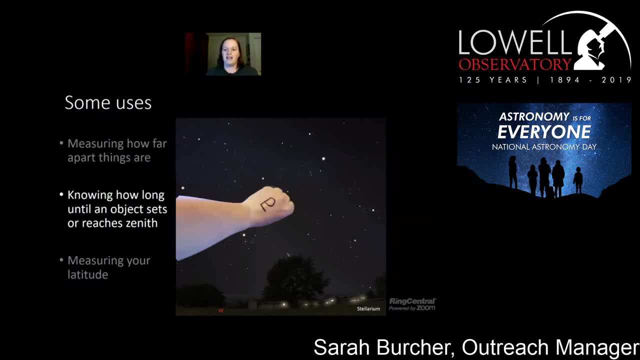 and so what you need to do is you can hold out your hands and measure that Venus is about twenty degrees from this tree in my backyard now. you may know just from personal experience that the earth rotates once every twenty four hours, so that means you, standing in any place, will go through. 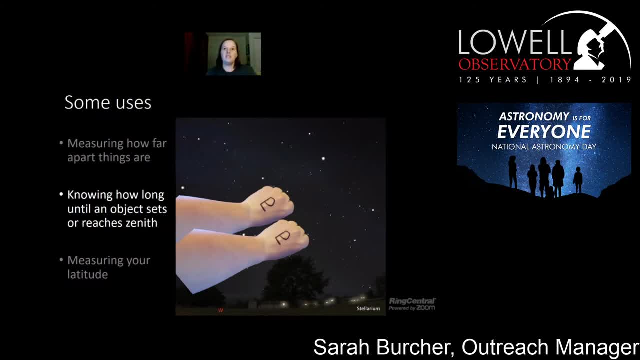 three hundred and sixty degrees of sky in twenty four hours, which means that it travels- the sky from our perspective travels at fifteen degrees per hour. so we know, by measuring twenty degrees, that I've got an hour and change for my friends to get there before Venus falls below these trees. 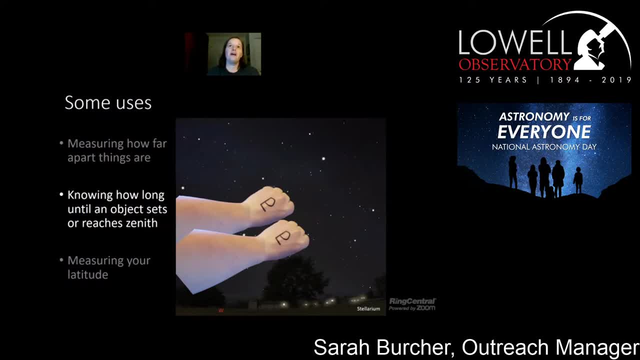 you can do the same thing for anything anywhere in the sky. if you want to measure for how long something reaches zenith, that's important. the best time to observe something is when it's right above you, so you might want to measure how long it is until something gets there. 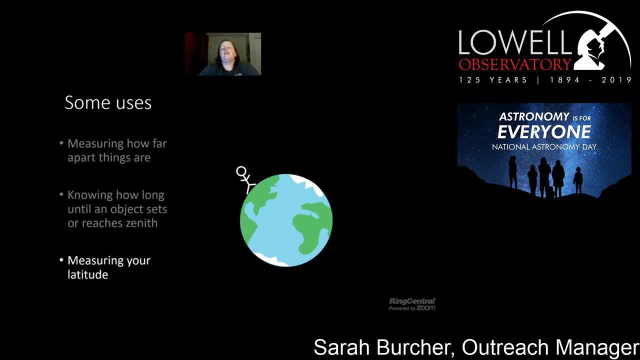 possibly the most useful thing out of this measuring is measuring your latitude. now I'll get to the latitude part in a second, but I want to talk to you first about the axis of the earth. so the earth is tilted at twenty three and a half degrees, or whatever that is, and the axis 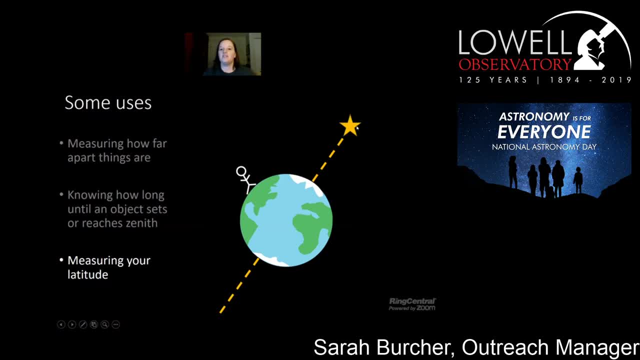 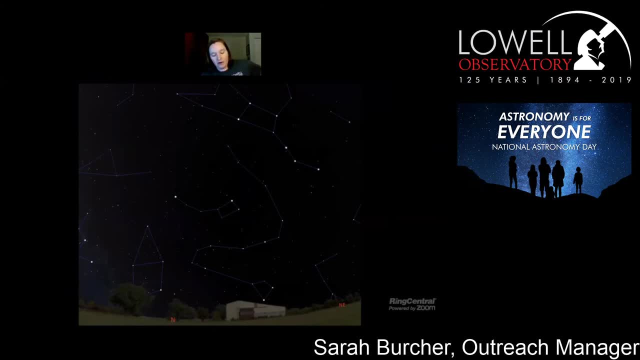 of the earth points directly at a star, and that is our north star, and its name is Polaris. now you may have heard that the north star is the brightest star in the night sky. I don't know where that comes from. it is very wrong. the north star is the fifty fourth. 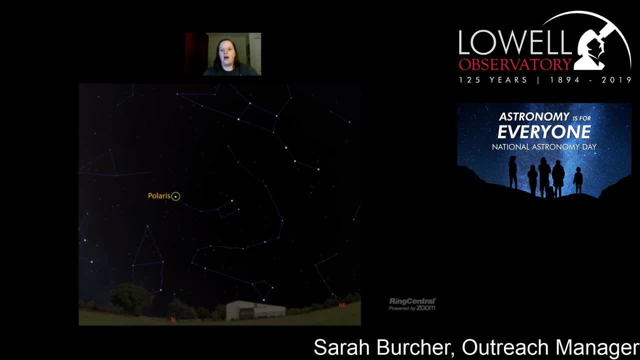 brightest star in the night sky and it is named Polaris. yeah, so it's not even in the top fifty. if you followed the brightest star in the sky tonight, you would end up pretty due south. so I would not recommend that anyway, because it's so dim. Polaris isn't particularly 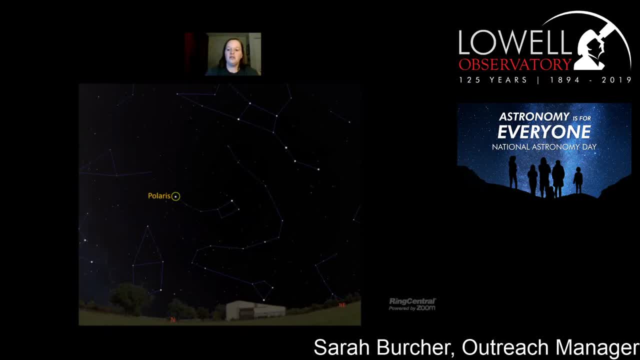 easy to find. so what you can do is use the big dipper- which anybody can find, the big dipper- and use the two stars at the end of the cup of the big dipper. draw a straight line out of that cup and you will run right into. 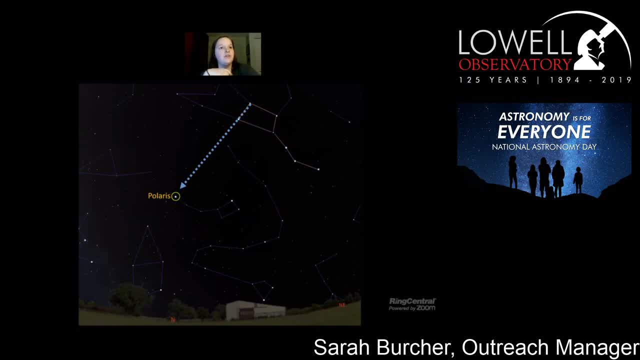 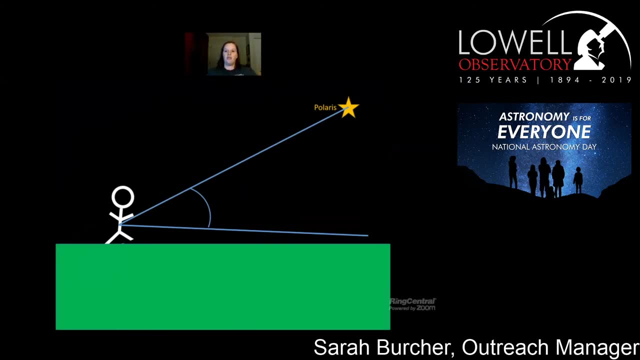 Polaris. now, what does Polaris have to do with your latitude? well, you can tell from my gorgeously crudely Microsoft powerpointed drawing that your latitude is actually the angle that is created between the north star, yourself and the horizon. so if I draw that angle out there, that angle, 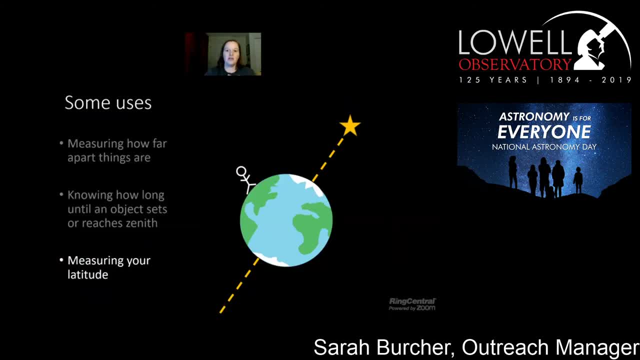 is your latitude. and so here in Arizona, right at 35 degrees latitude, the angle between the north star us, and the horizon 35 degrees. if you were, say, up at the north pole, that angle would be 90 degrees because Polaris is straight up and the horizon is straight out. 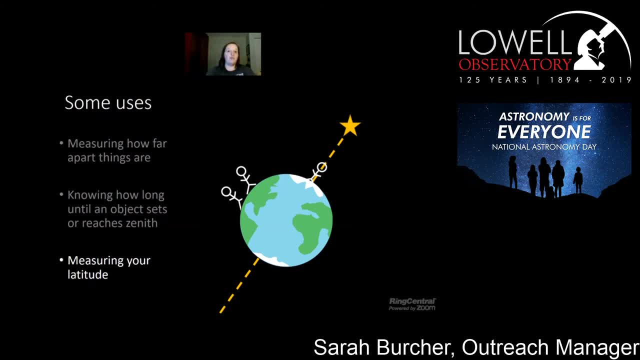 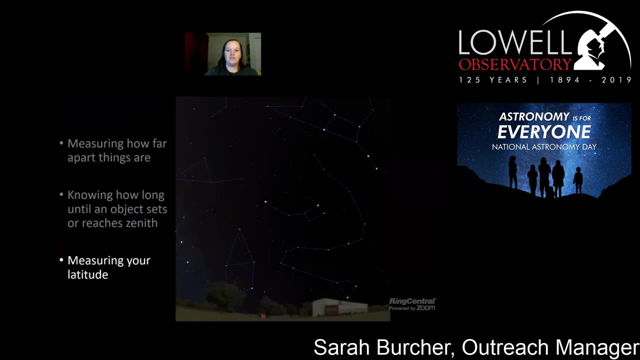 if you were at the equator. that angle becomes 0 degrees because the north star is just sitting right on the horizon. so now you know how big your hands are, you know how many degrees you are, you can measure what your latitude is, right. so here's a picture of the sky. 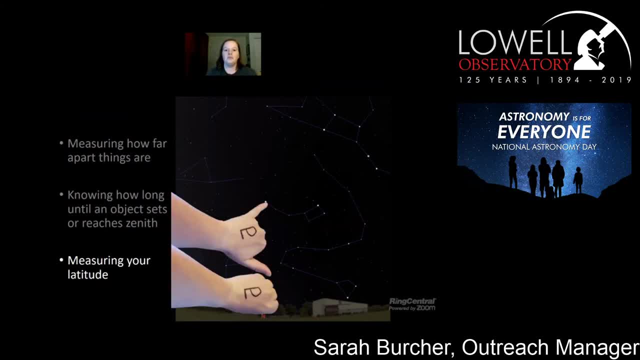 from Arizona using the stellarium, and so if I just do two, I can do a little 25 degree and a 10 degree, giving me about 35 degrees, cool. so I'm going to open it up for questions. so go ahead and start typing your questions. 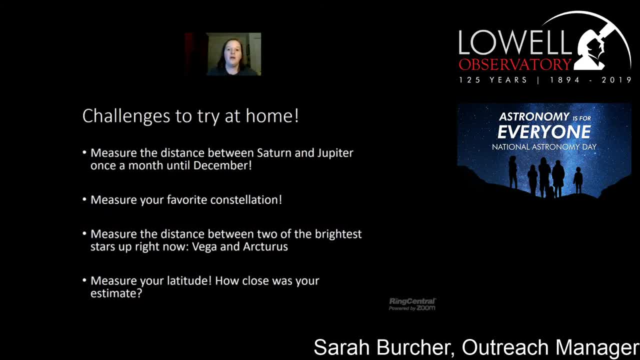 if you have them- and I'll go into challenges to try at home- you can measure the distance between Saturn and Jupiter just from now until December, because they're they're going to keep changing. it's going to be pretty fun. you can pick your favorite constellation, just measure it out. you can measure the distance between bright stars. the two easiest ones to find right now are Vega and Arcturus. Arcturus is kind of up higher right now, Vega a little bit lower down in the east, but you'll be able to find them no problem. 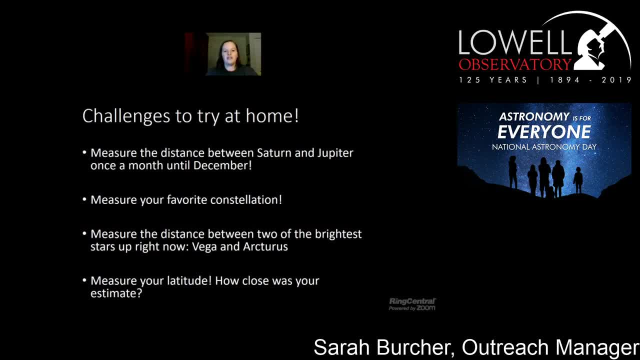 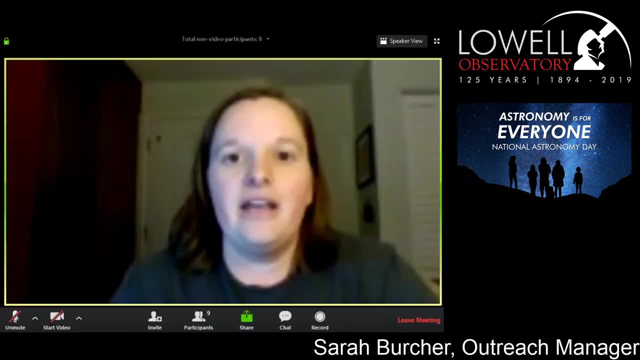 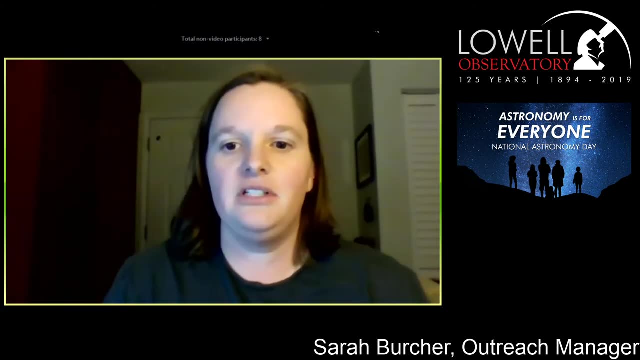 especially if you have one of Jim's planispheres, and I want you guys to try to measure your own latitude. it's going to be different for every single one of us, right? so, yeah, alright, so now, after that wonderful whirlwind of how to use your, 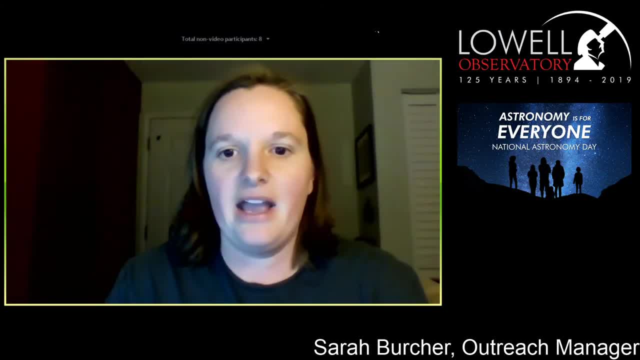 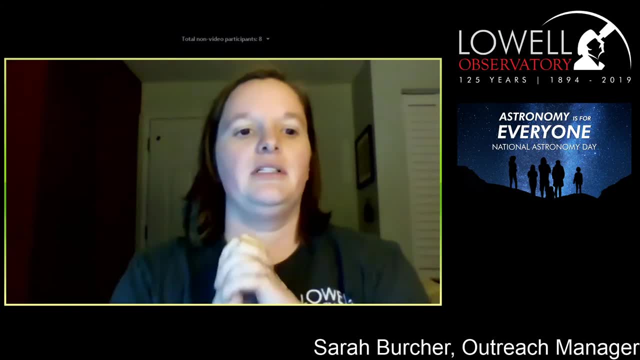 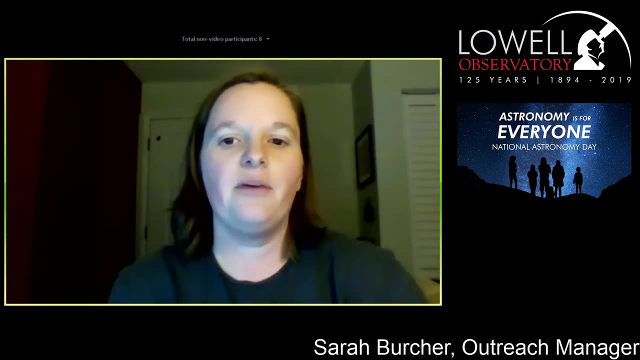 hand to measure the night sky. I'm just going to hang out and see if we have any questions, um, but yeah, what was I going to talk about? I don't remember, so I hope you enjoyed my poorly photoshopped thing and I wanted to prove that I wasn't. 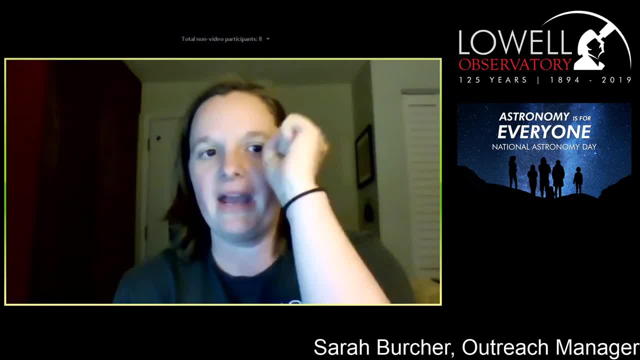 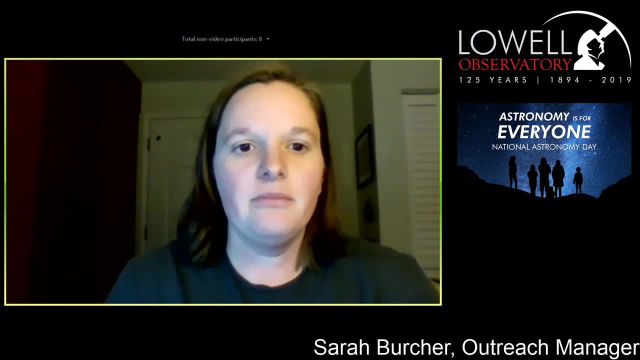 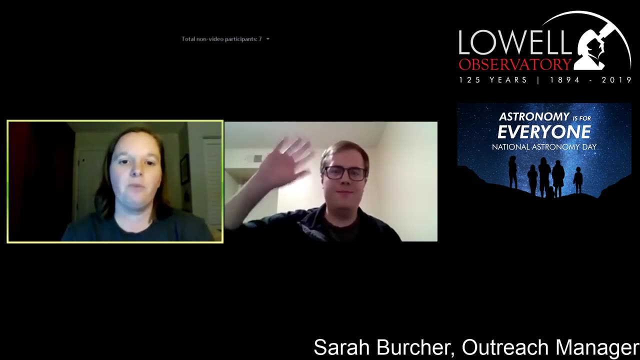 using stock photos for this, so I drew a little kundo on my hand, but I'm sure you enjoyed. so it doesn't look like I have any questions. so I am going to turn it over to Curtis Dancoff, who's going to kind of wrap up the live portion. 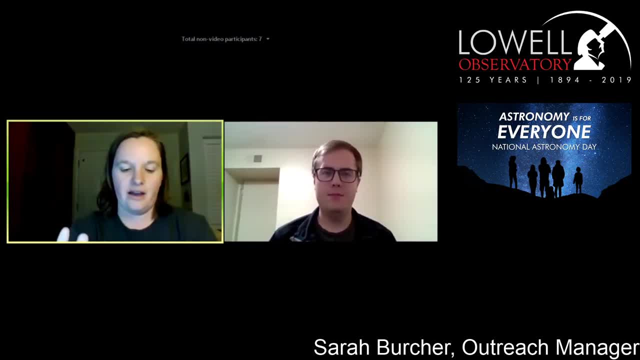 of this, of this- whatever term- of this stream, and we'll wrap up the whole stream with some premieres of some of the new video series that we're going to get into. but let's actually turn it over to Curtis, who's going to talk a bit about. 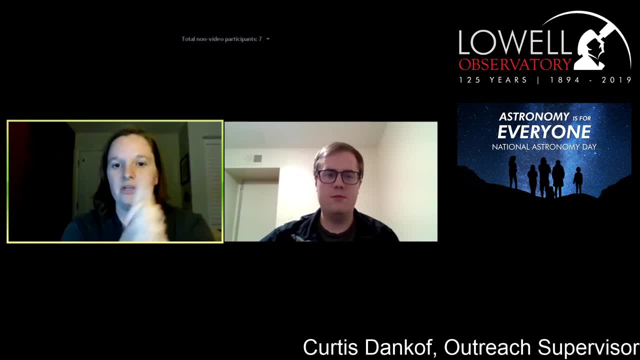 the connectivity of astronomy and real quick. we just got a question- what's going on with Saturn and Jupiter- and I'm going to leave that to the video that we're going to show later. it's going to end. I'm going to answer that way better than I ever could. 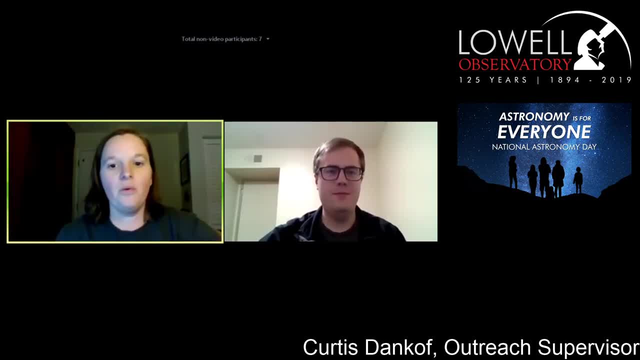 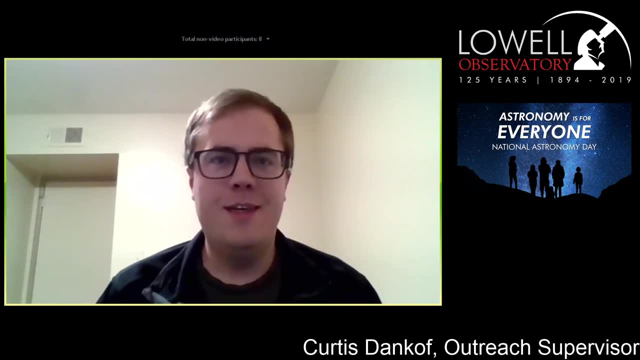 so I'm going to continue to turn it over to Curtis Summer. don't worry, your question will be answered. alright, Curtis to you, alright. thank you, Sarah, for that. I'll actually be referencing back to the presentation about how to find your latitudes. that was perfect set up. 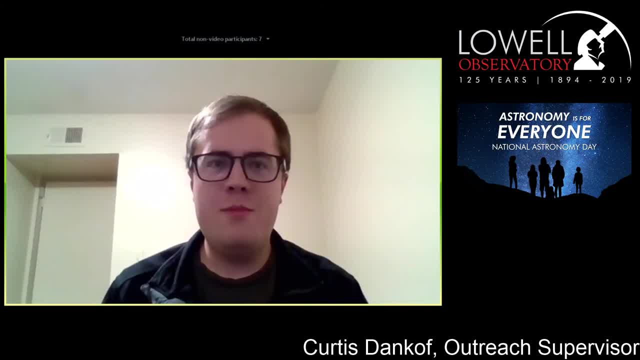 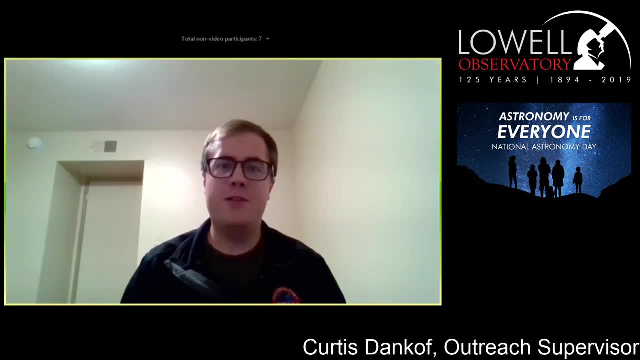 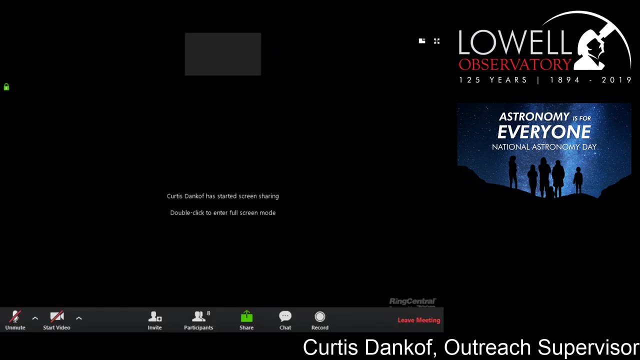 and I'm going to be talking a little bit about how astronomy connects us. it's one of my favorite parts about astronomy in general is that it connects everybody. particularly the night sky is what connects us, so I'm going to go ahead and share my screen here. 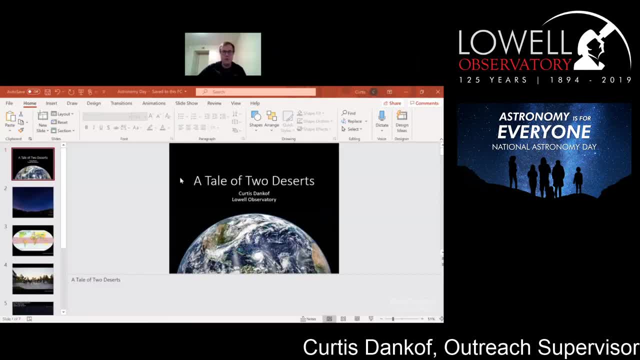 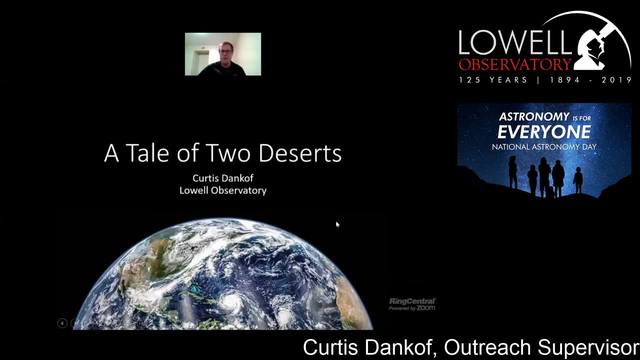 alright, and we are going to start this presentation alright. so I'm talking about a tale of two deserts and we'll actually kind of get into into this why it's two deserts in just a little bit. but I want to set this up, set the stage first. 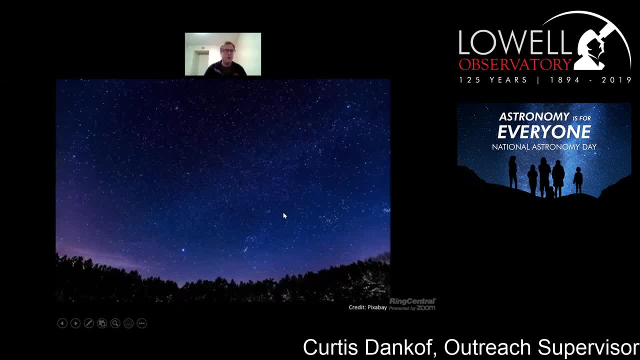 so what I love just so much again about astronomy is that it connects us all. the night sky is there for everybody. no matter where you are in the world, you can have access to the night sky, and not just anywhere in the world, but anywhere through time. so when you do look up at the sky, 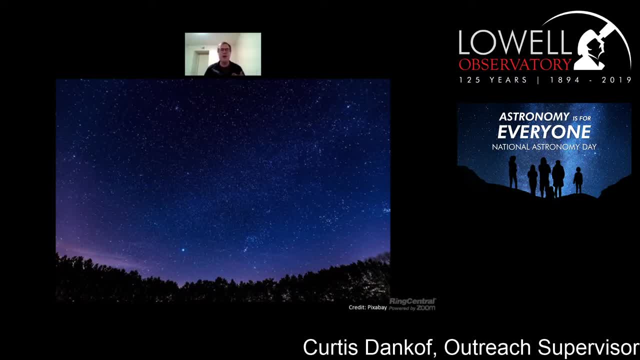 you're sharing that same view with people throughout time, throughout history and around the world, and you know, people have lived their lives having never seen mountains or the oceans, but the night sky is there for everybody, and so that's why we see it as such an important factor. 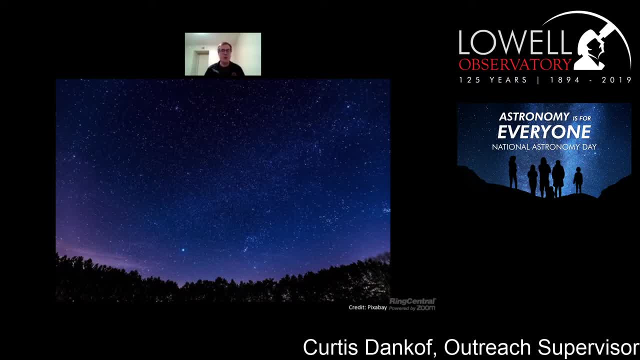 in our culture, our constellation stories, our architecture throughout history can be very, very centered around astronomical phenomena so incredibly important to us as a species, as a civilization, and so when I say that you can look up at the sky and see the exact sky as somebody else, 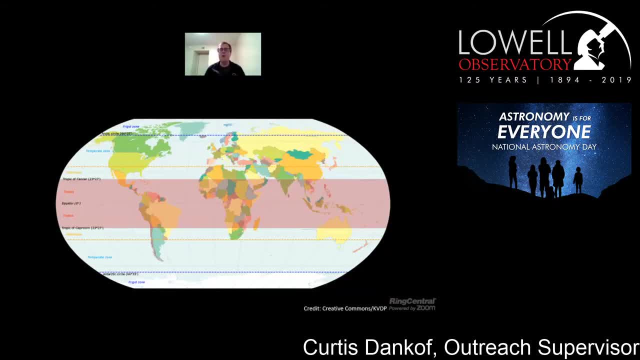 I mean it. so, depending on where you are in the world, your latitude, you will actually view the stars a little bit differently, and we'll see an example of this in just a little bit and, like Sarah mentioned in that last little presentation, where the north star is, 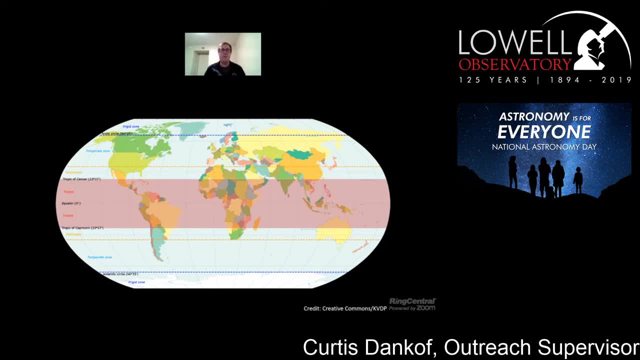 in the sky, how far it is above the horizon, depends on where you are in the world, what is your latitude. and so say, for instance, if you live along the US-Canada border up here and you follow that line of latitude all the way across, you kind of cut through France. 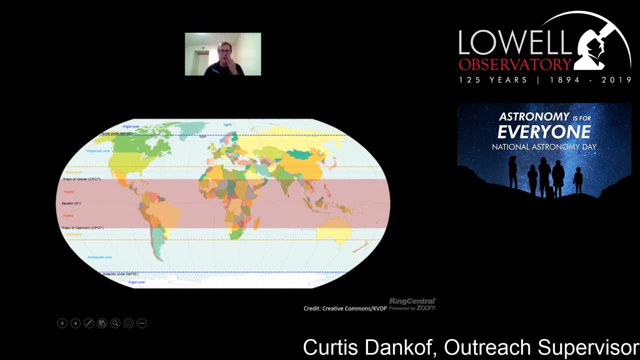 maybe Germany and over here through Asia and those people that lie along that latitude line will have the same exact night sky as you. for us down here in Arizona there's this really nice dashed line that goes right across, basically right in Arizona, and you can see that we kind of cut across. 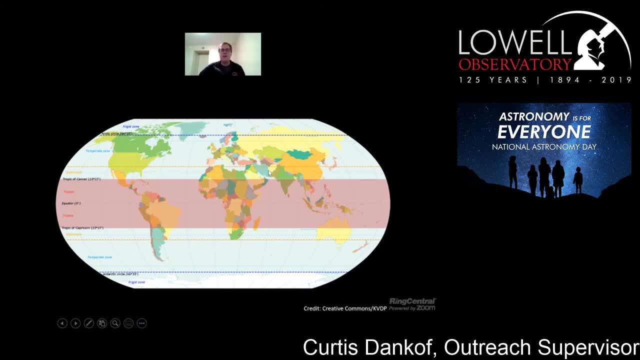 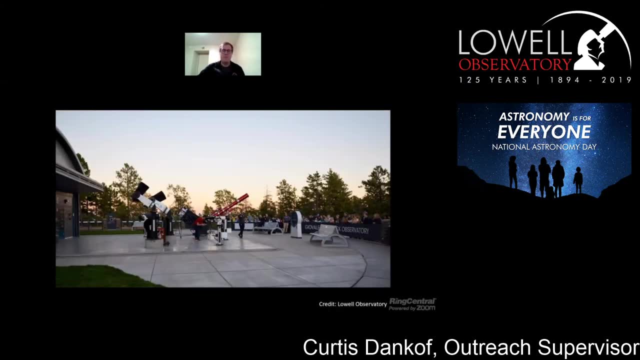 from Northern Africa, the Mediterranean, through some of the Middle East and, particularly, we end up in Afghanistan, which I will go into in just a few minutes. so one of my favorite parts of working at the observatory is interacting with the public and hearing the stories of how 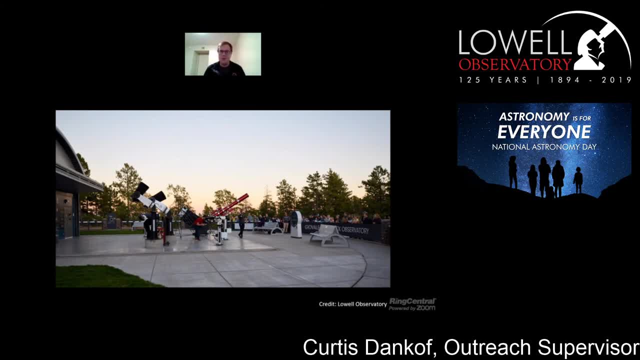 astronomy, how the night sky has impacted certain people, and these are people that come from around the world, and they all have different, unique stories. it's really, really incredible, and so just- oh, it was about a year ago- I was at one of the telescopes that we offer to the public. 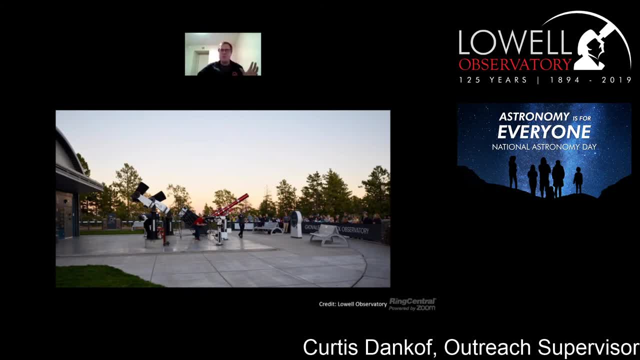 and it was such an incredible experience that I had with this one particular guest, and this guest was visiting from Phoenix, just about two hours south of Flagstaff, and he was telling me how much he loved astronomy. he grew up just fascinated with it and he became very knowledgeable. 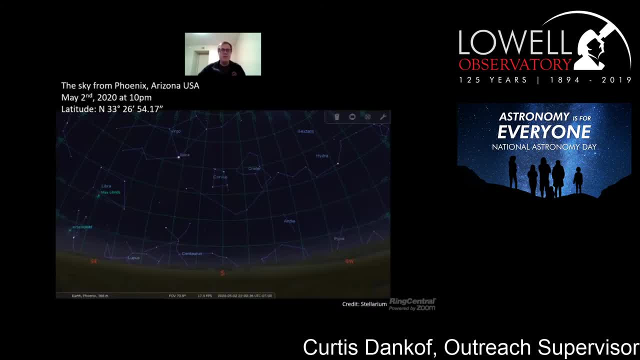 with the night sky, he knew the constellations, and so if he was to go outside on a night like tonight, for instance, and he's sitting in Phoenix at about latitude 33 degrees, he would see the sky and he would see, say, Spica, here a little bit over. 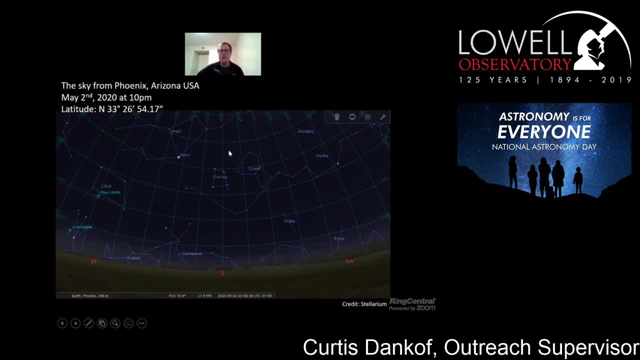 30 degrees above the southern horizon, he would see Corvus, the crow Crater, the cup Hydra snaking along the sky, and he would even see Scorpius down here just rising- and this is at 10pm tonight, by the way, and so he became very, very, very familiar. 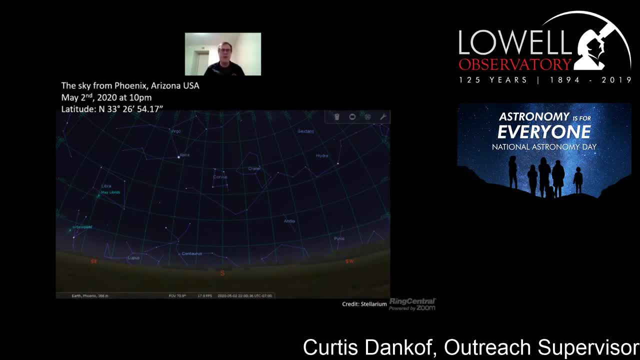 with the night sky and this man then went on and joined the military and he was deployed to Afghanistan. and while he was in Afghanistan he found himself looking up at the sky and he noticed it was a very similar climate to Phoenix, so it felt very desert like. 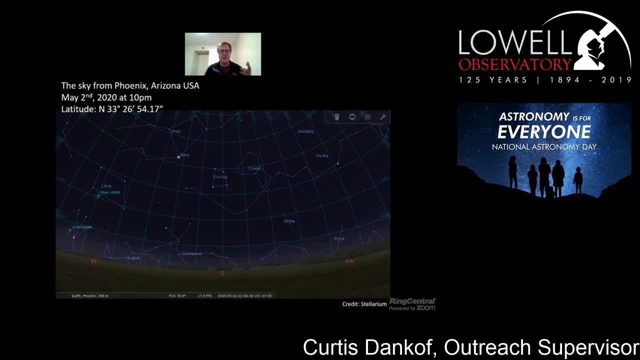 so this is the tale of two deserts, if you will. and when he was laying there, he looked up at the sky and noticed that it looked the same, the stars were in the same spot, and so, if I go to this next slide, here we have what it looks like. 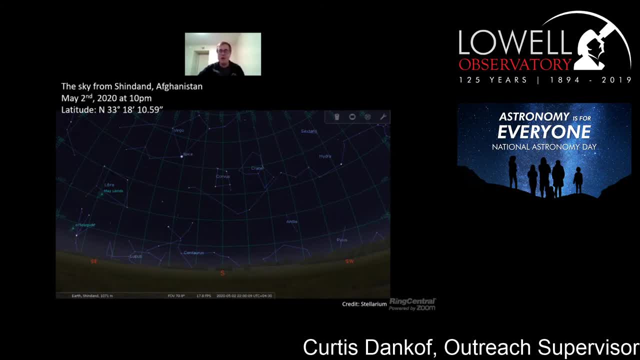 from a town called Shandong, Afghanistan. they actually have an air force base there as well, run by NATO and the Afghan air force, and so they are at a very similar line of latitude to Phoenix. they are within the same degrees, just a few arc minutes off, which is one of the 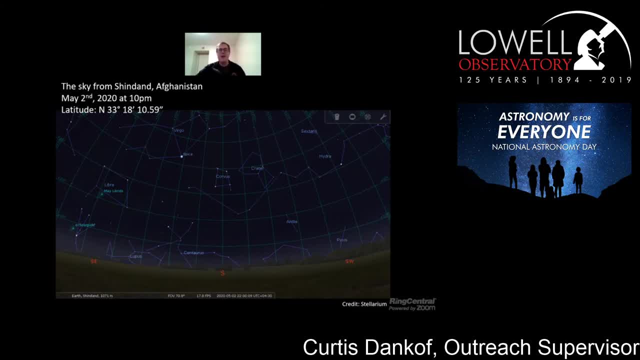 measurements of the sky a little bit finer than degrees, and so if we go back and forth between our Afghanistan sky to Phoenix, we see that the sky doesn't really change much. this is at 10pm local time for each of these locations and it looks almost identical. 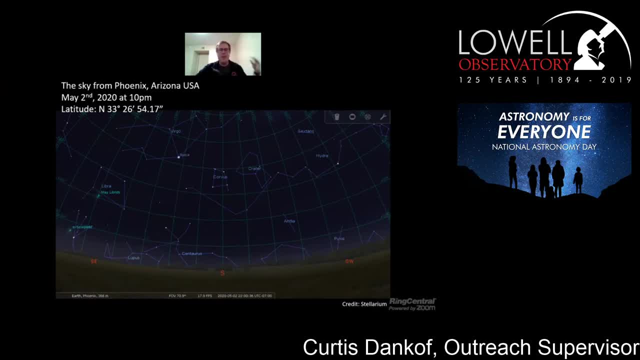 and so this soldier, deployed 8000 miles from home, could feel this incredible connection to his family back in Phoenix. he knew that he could go outside, look up at the night sky and see the same exact thing as his family back home. it was just this really incredible moment. 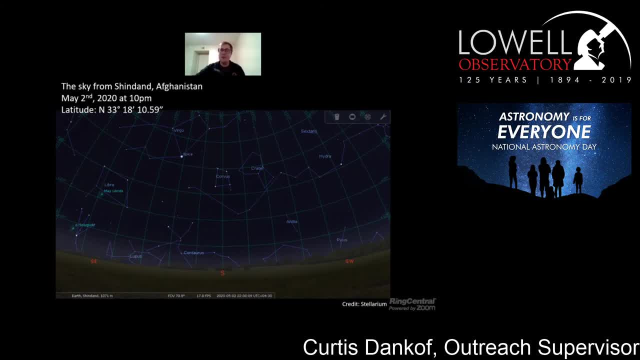 that still sits with me to this day. just by the way, I am using a program called Stellarium, which we have seen throughout these presentations. it's free, it's on the desktop. it's a great way to go to different places in time in the world. 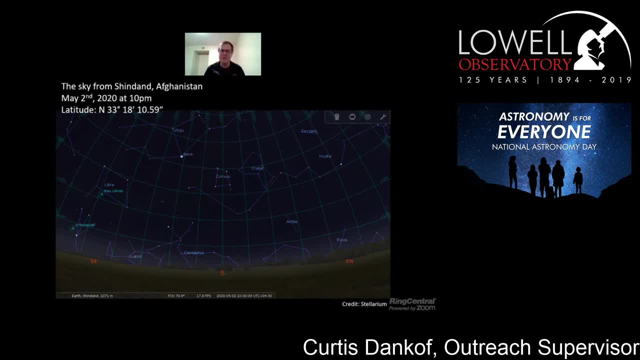 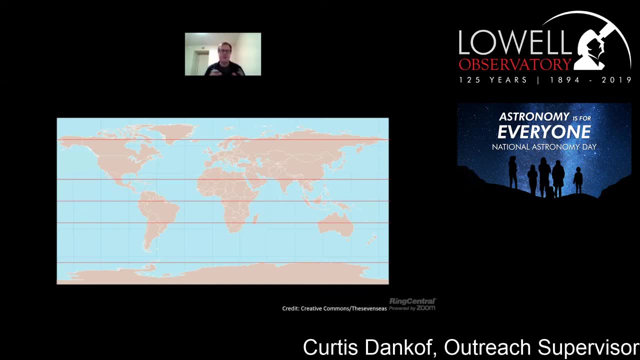 to kind of see what the sky looks like from that location and that time, and so astronomy and the night sky again has this incredible way of just connecting people. when you look up at the sky tonight, go outside or any night you can go up and just look up. 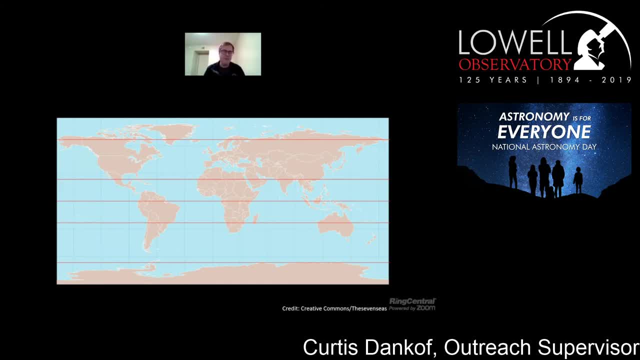 and think about all the people throughout the world that you are sharing that same view with and throughout time as well. so I urge you to grab out an atlas or a globe or go onto a google earth type page and look at where you live and look right along your 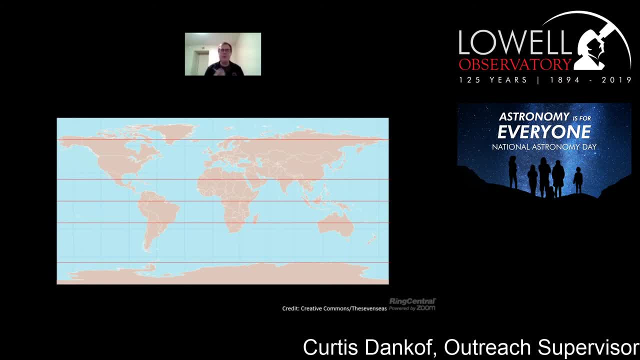 line of latitude and take it all the way around the globe and just see who is along that line, which cities, which cultures, which constellations, and just really see that we're all connected under this beautiful, beautiful night sky that we all have access to in some way. 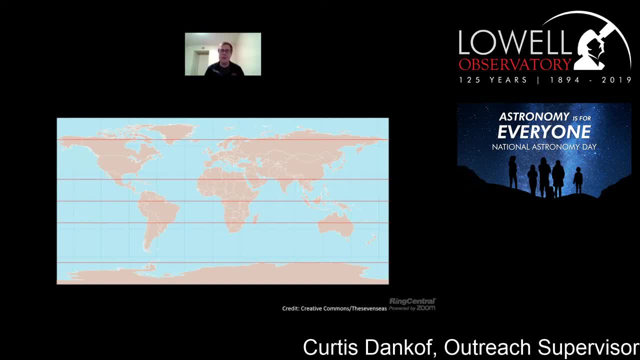 it's always up above us. so if anybody has any questions at all, please ask away. I'm happy to answer any questions. I'll be looking for them in the chat. alright, I don't see any questions yet, but we'll stand by for just another few seconds here. 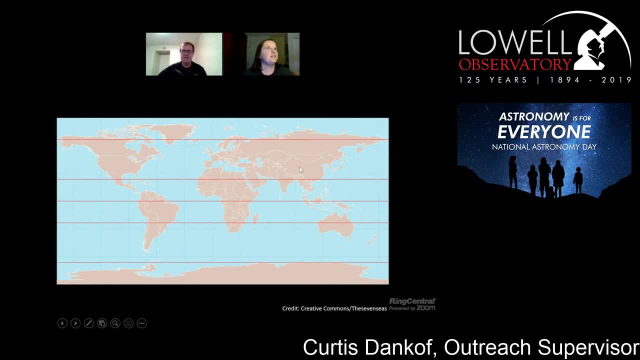 don't want to miss anybody's questions. it's amazing how many stories we get like that on a regular basis. you know just so many people talking about how the night sky, they feel so connected to the rest of the world. yeah, it's really incredible. 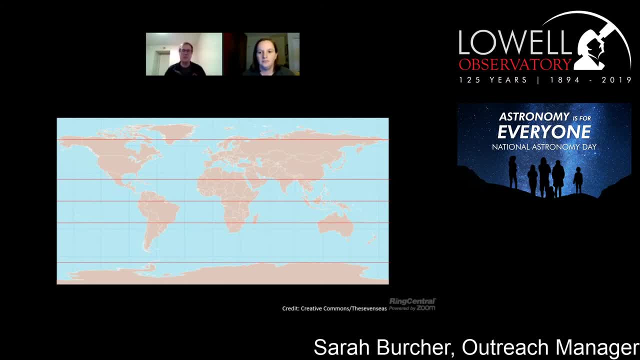 it makes you feel small but also big at the same time. it's this really interesting feeling that so many people get. it's really really cool. it's not just a feeling that I have or you have. it's that most people in the world have some sort of reaction to the night sky. 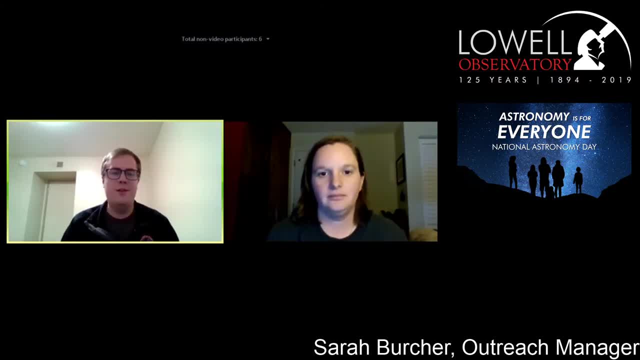 I don't see any questions, but thank you all and I hope sometime you can maybe all come up to Lowell, if you get a chance, and share some of these stories. I can talk for hours with people about their stories of how astronomy has impacted them. okay, thank you, Curtis. 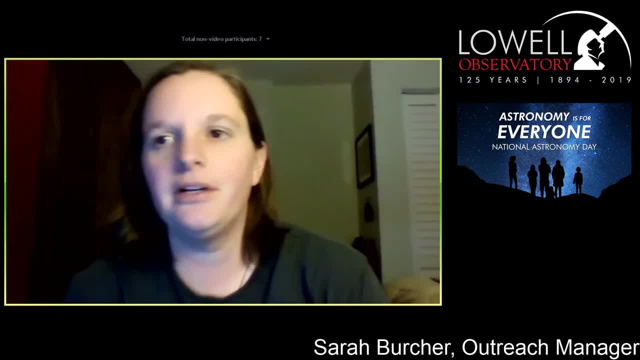 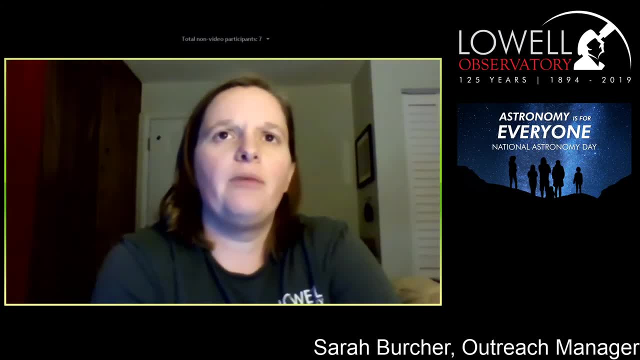 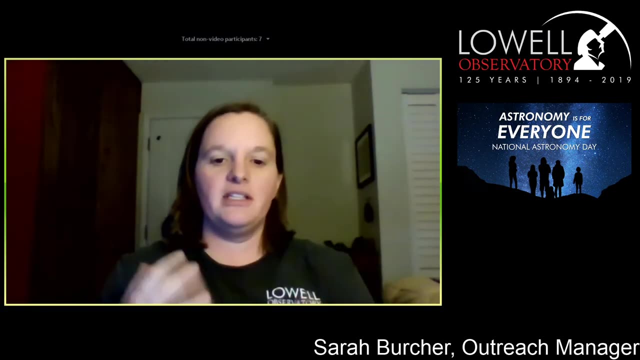 so that does conclude the live portion of our stream for you tonight. so we're going to do something special. we're going to premiere two of our new web series. the first one is called the Mars Hill Almanac, which will show you what's coming up. 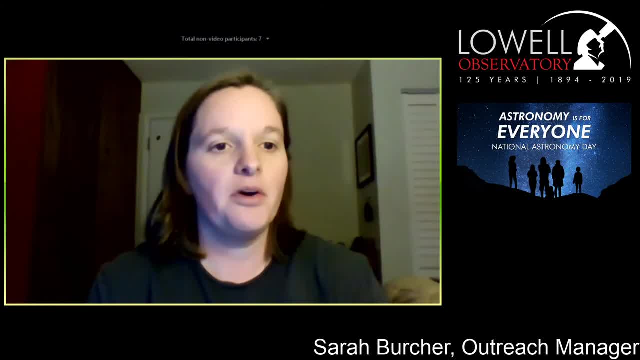 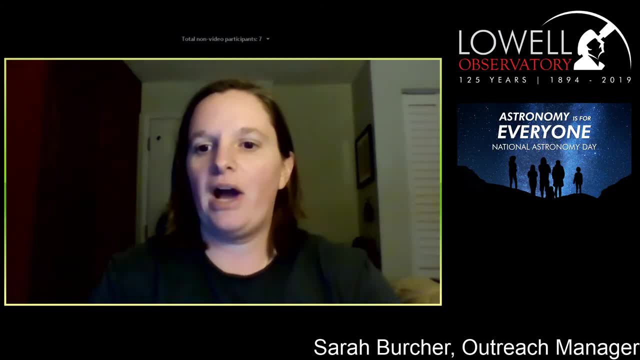 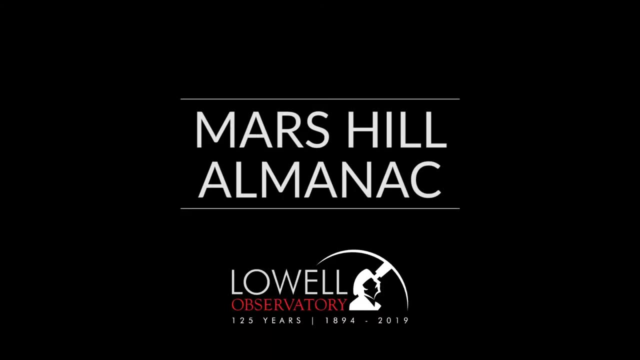 in the sky the coming week, and this particular one focuses on planets, both in the evening and in the morning, so I believe I'm going to turn it over to our video master, who will start playing that for you. Hello everyone, I'm Rezi from Lowell Observatory. 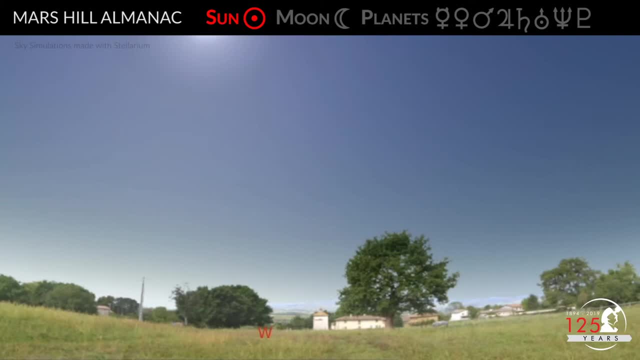 and we're going to take a look at what's in our sky tonight. let's start with sunset. the sun is going to set tonight just after 7pm. slightly north of west along the horizon, we're nearing the solar minimum in our 11 year solar cycle. 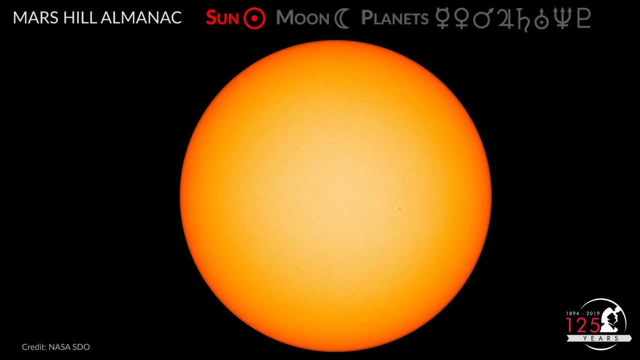 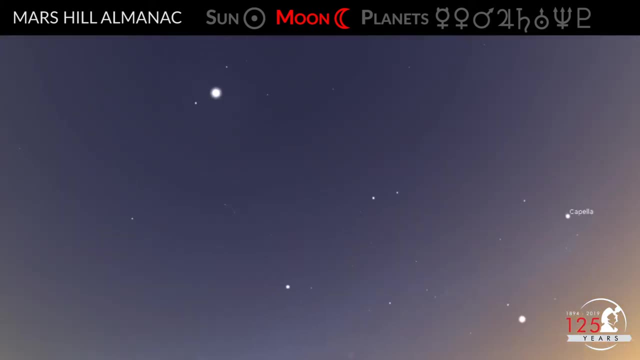 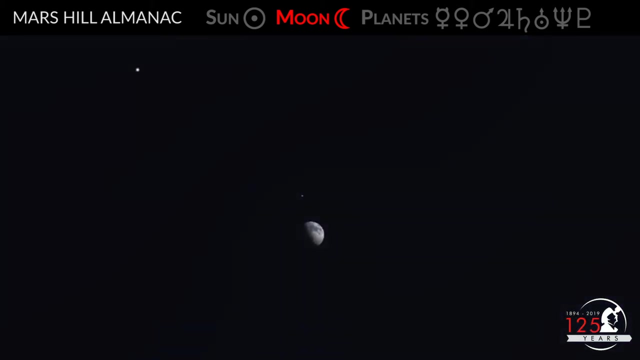 so there's not too much to look at on the sun up close for any of you solar observers. the moon is clearly visible high in the sky in its half waxing phase, just after sunset. for those of you who are observing every night this week, or a few nights this week, 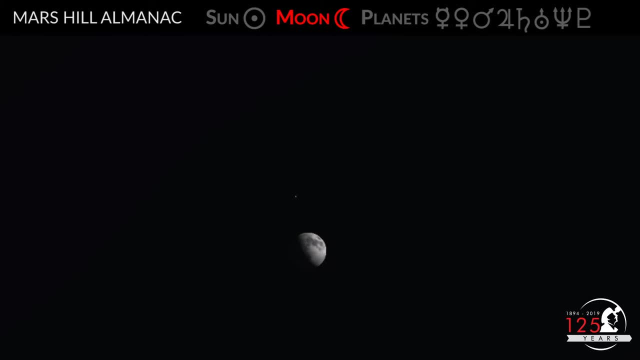 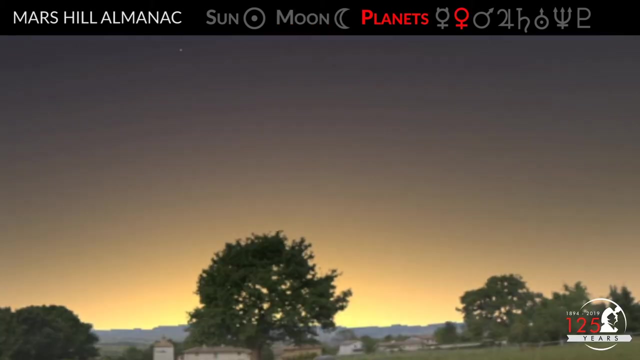 you will notice that as the moon gets fuller and brighter, you're going to see fewer stars in the night sky, as that moonlight creates some natural light pollution and drowns out the light of those stars. Venus is high in the sky tonight at about 45 degrees above. 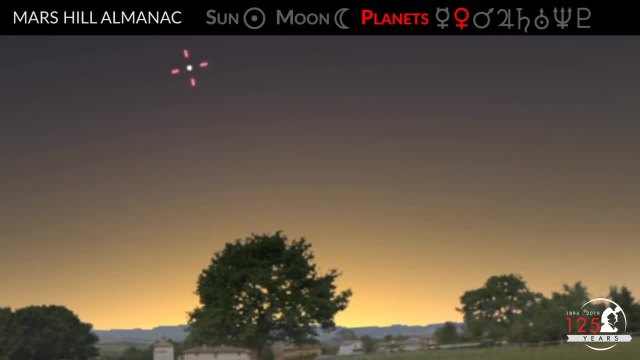 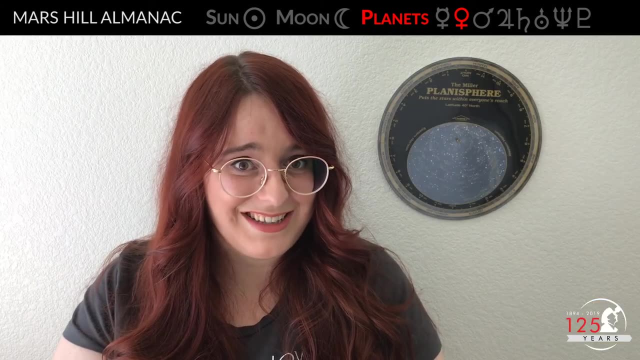 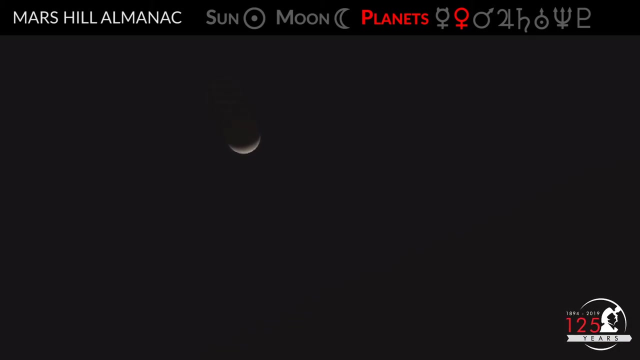 the western horizon. aside from the moon, it will be the brightest object in the sky tonight, making it an easy target to spot with the naked eye. for those of you with a backyard telescope, Venus makes a fantastic target. looking at Venus tonight through a telescope, you will be able to observe. 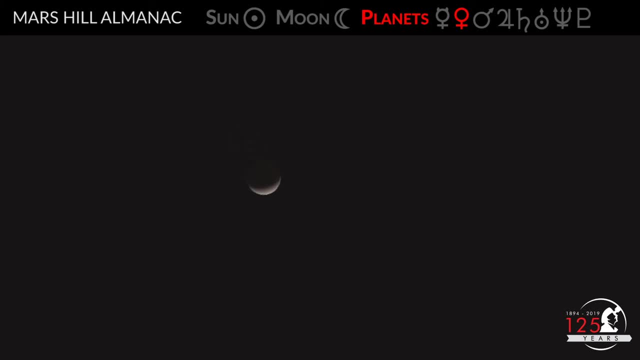 Venus in its crescent phase. Venus sets just after 10pm and for a couple of hours there will be no planets in tonight's sky for any early morning observers. Jupiter rises at 1.30am, with Saturn trailing just behind between the constellations. 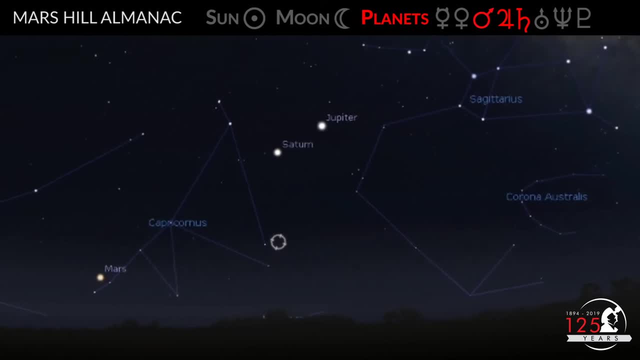 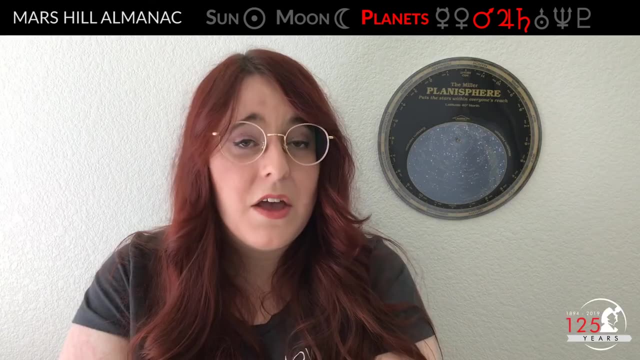 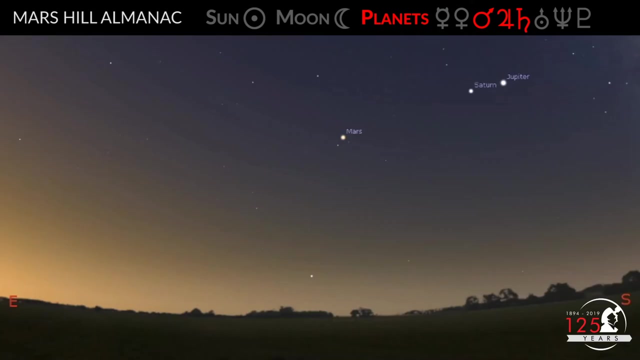 Sagittarius and Capricorn. Mars follows these two planets just a couple of hours later, at 3am, on the other end of Capricorn. for those of you who wake up early, looking up in the sky at about 5am, you will see all three of these planets. 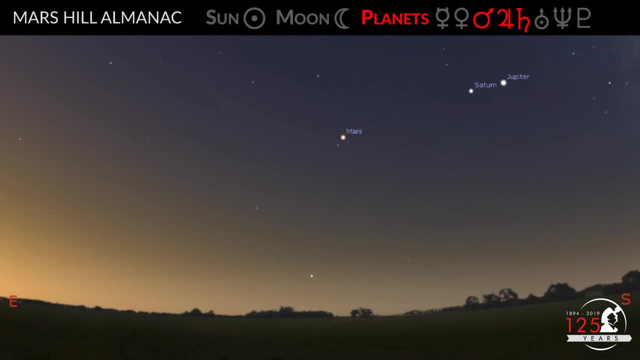 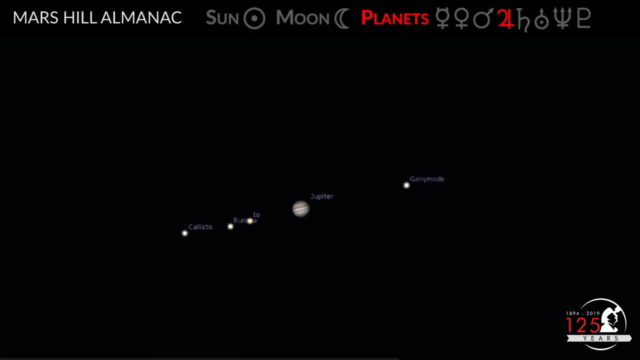 Jupiter, Saturn and Mars. in a line above the eastern horizon, Jupiter and its moons make a great telescope target. for those of you with a very good pair of binoculars, you may actually be able to challenge yourselves to point at Jupiter and see it alongside its largest and brightest. 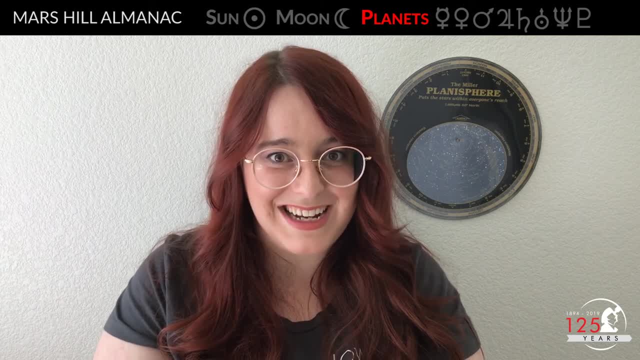 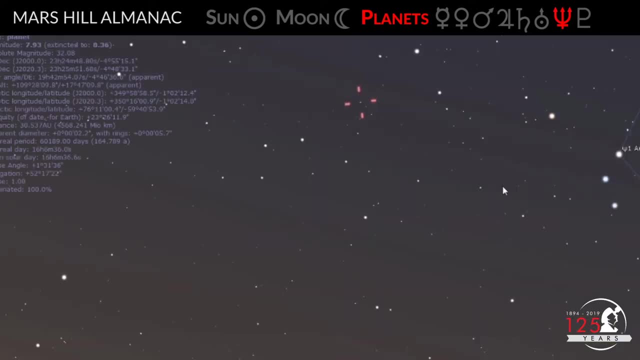 moon Ganymede. for those of you interested in a deep sky challenge this week, let Neptune a try. early birds may be able to view this elusive ice giant just before sunrise, between about 4.30am and 5am, just under 20 degrees above the eastern horizon. 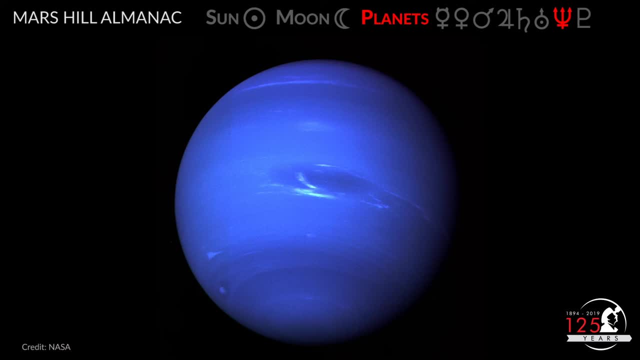 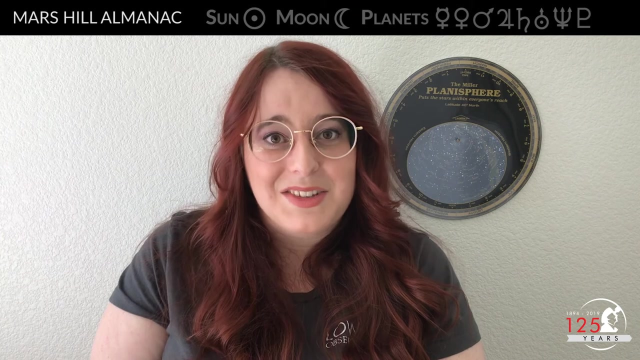 though it is very large, about 4 times the size of the earth. Neptune is so far away that the sunlight on Neptune at noon is about as bright as the sunlight is at twilight here on earth. we're interested in hearing from you in the comments. go ahead and. 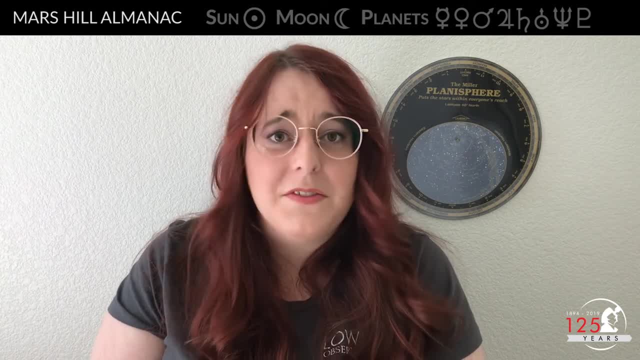 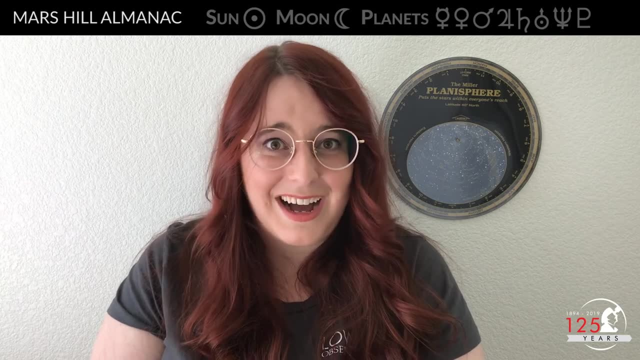 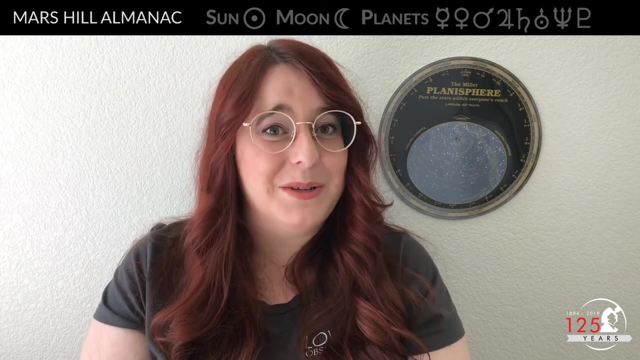 tell us your favorite experience observing the planets. if you've never observed the planets before, that's fine. tonight's a great time to start. we'll be combing through those stories in the comments and picking our favorite to share in next week's update. until then, my name is Rezi from Lowell Observatory. 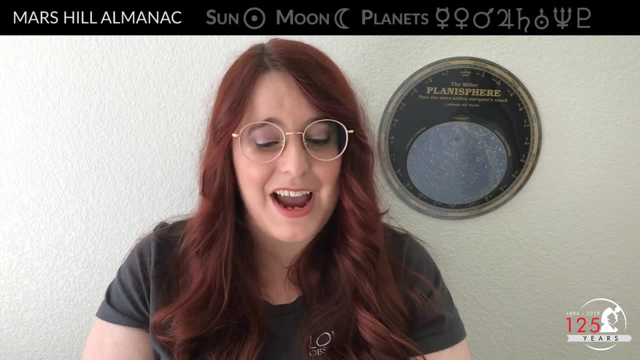 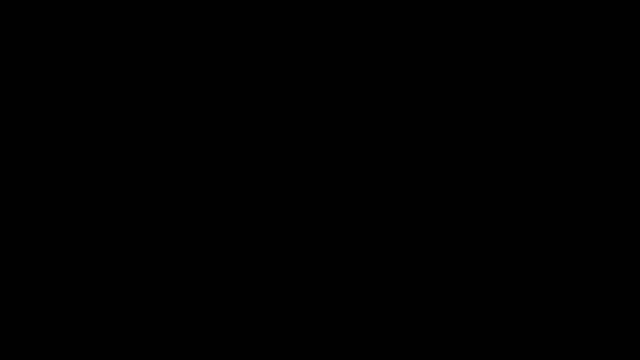 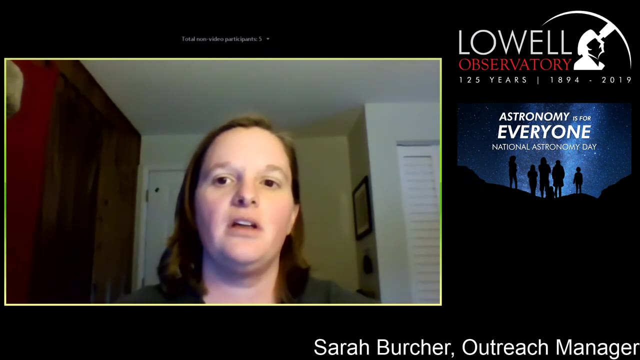 thank you so much for following along with us tonight. I hope you guys have a great time with your backyard observing. that was the end of our video. I'm going to set up our next video, which is actually a bit of a different take. we're going to continue to talk about. 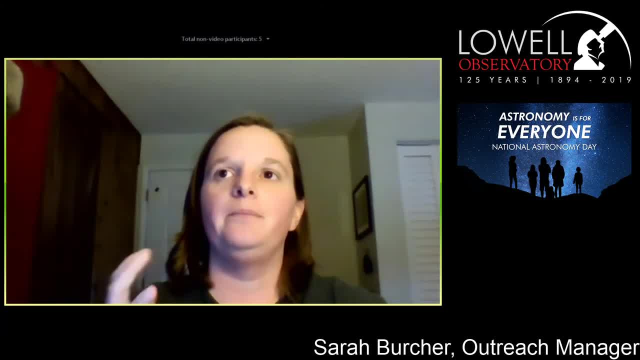 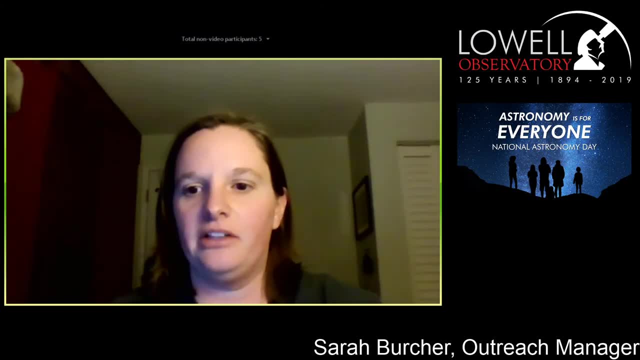 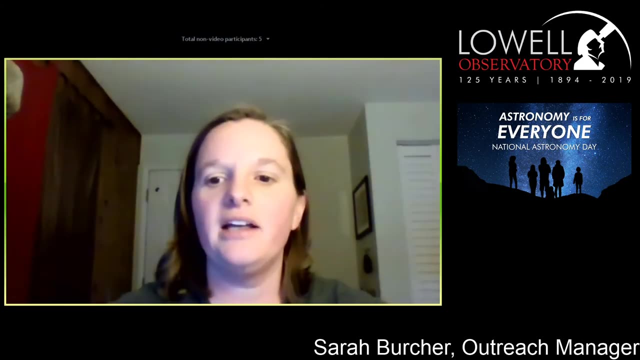 the planets, but we're going to talk about them and talk about their importance throughout history and tell some of the stories in a whole bunch of different mythologies. so if we're ready to go, let's go ahead and go to the Sagas in the Sky. 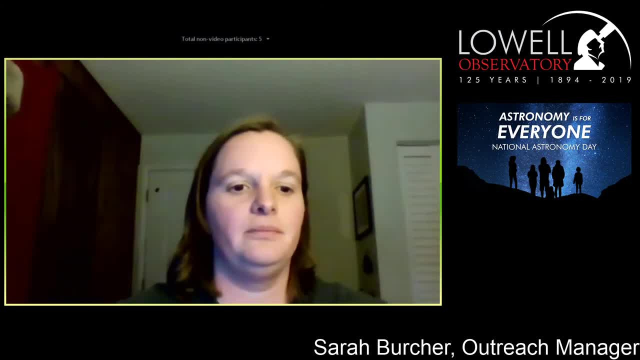 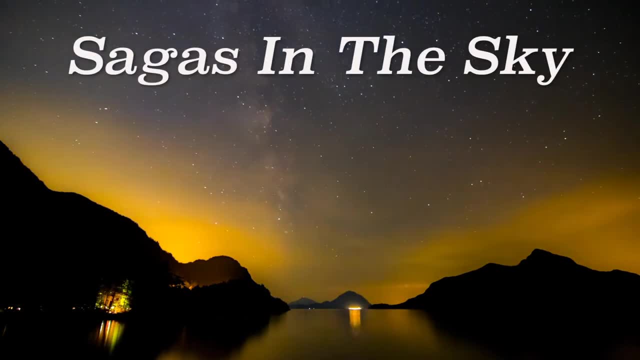 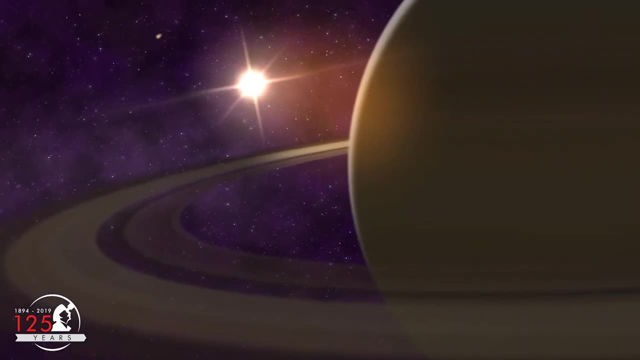 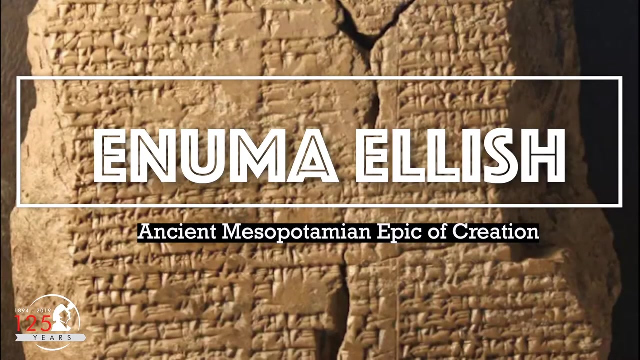 that will tell us some of these stories. how did the planets get their names? well, that's a story that goes back to the very cradle of civilization. one of the oldest surviving stories of creation is the ancient Mesopotamian Enuma Elish in this story. 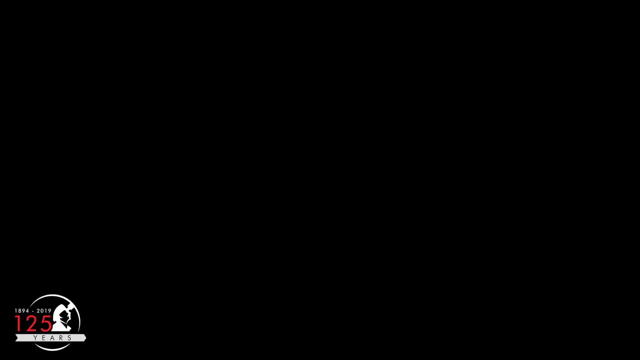 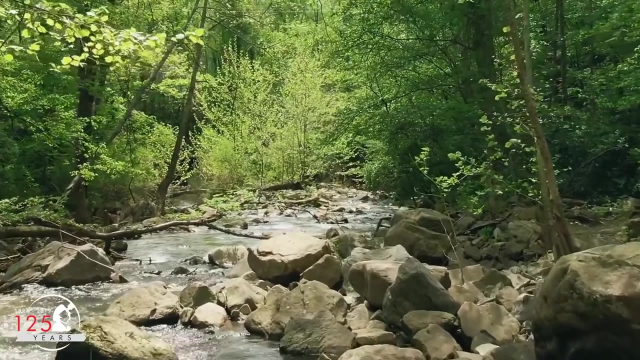 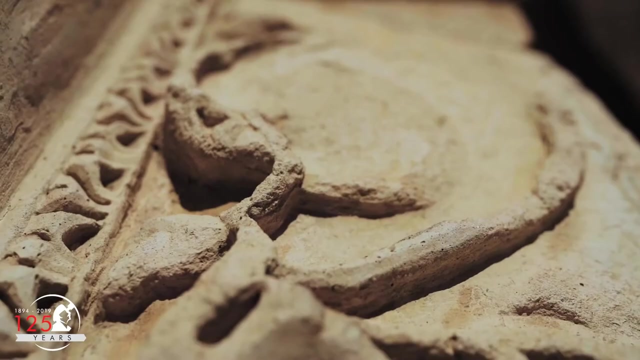 the universe begins with two primordial beings: Tiamat, who is chaos and the saltwater oceans, and Absu, who is the fresh water, rivers and streams. Tiamat and Absu become partners and the gods descend from them, but the new gods are wicked in their ways. 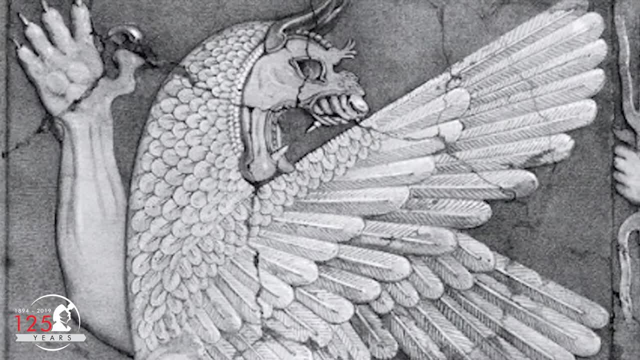 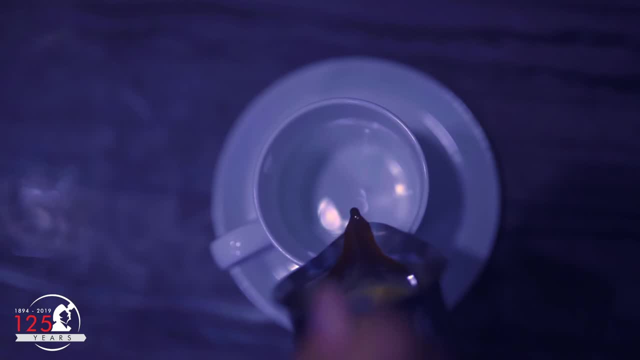 in the eyes of Tiamat and Absu. Tiamat wants to spare the new gods, but Absu decides to do away with them and start over. but the other gods are forewarned. they use a potion to put Absu to sleep. Tiamat is enraged. 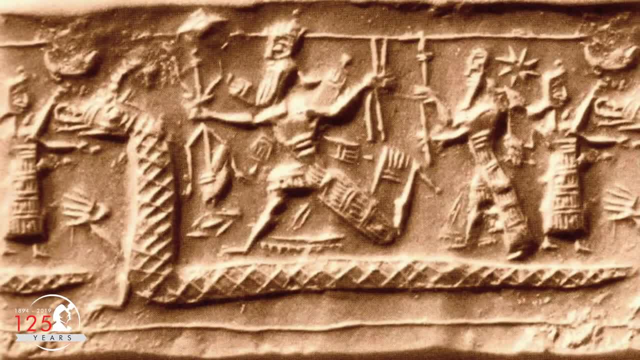 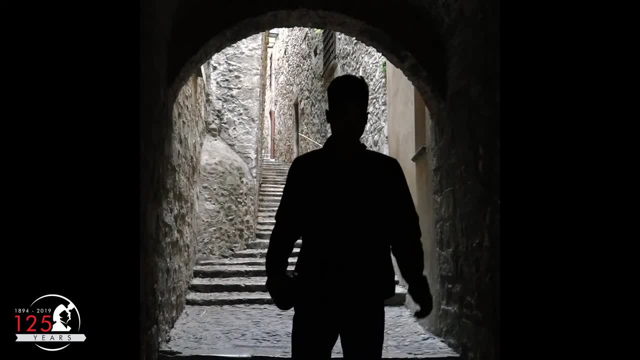 at the loss of Absu, she creates a gigantic army of monsters and rampages across the cosmos. no one can stand against her until one of the youngest gods comes forward, Marduk, the god of storms. Marduk agrees to fight against Tiamat. 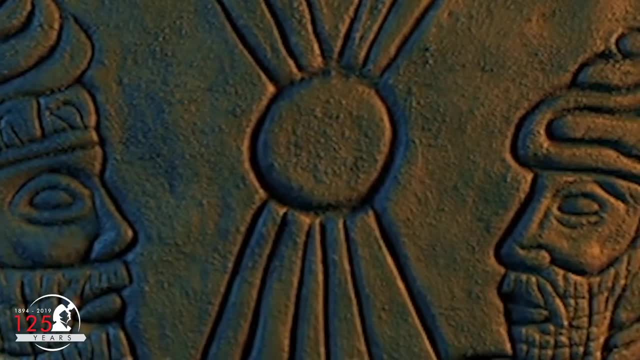 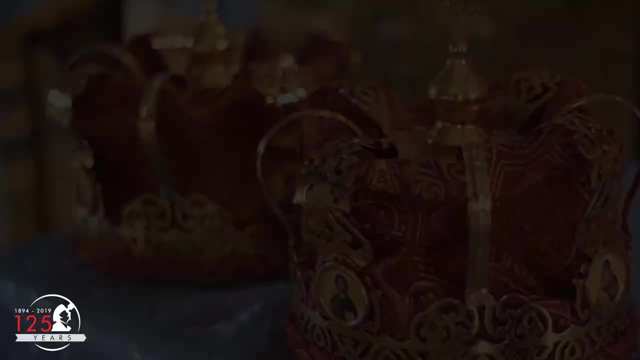 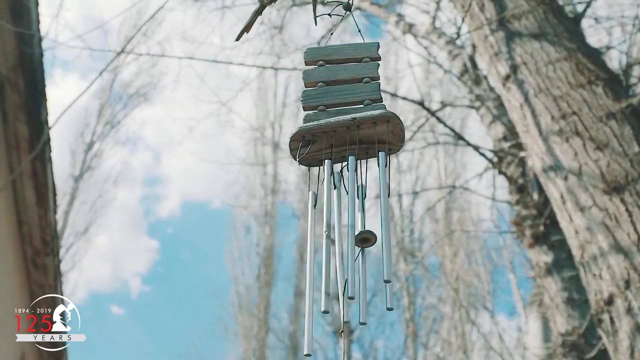 in her army, but only if the other gods agree to lend him some of their power and only if Marduk is made king upon his victory. the other gods agree. Marduk uses the winds and power, including the power of the wind. it's a fierce battle. 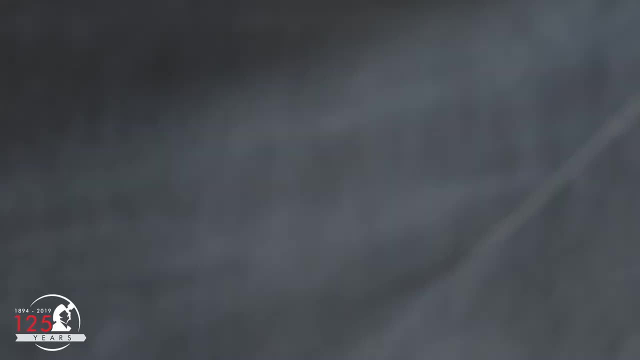 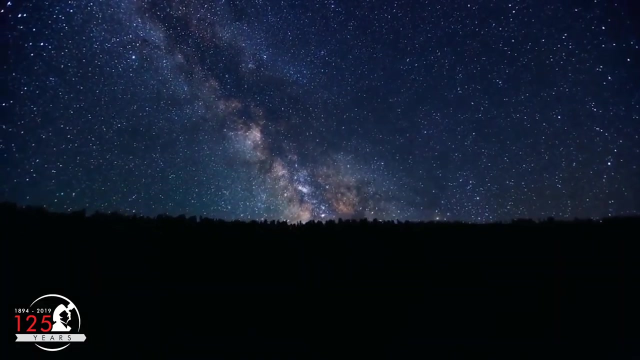 but eventually Marduk uses the winds to trap Tiamat and slay her. Marduk uses Tiamat's body to create the sky and to make it firm, and across the sky he makes shrines and likenesses of the other gods to honor them. 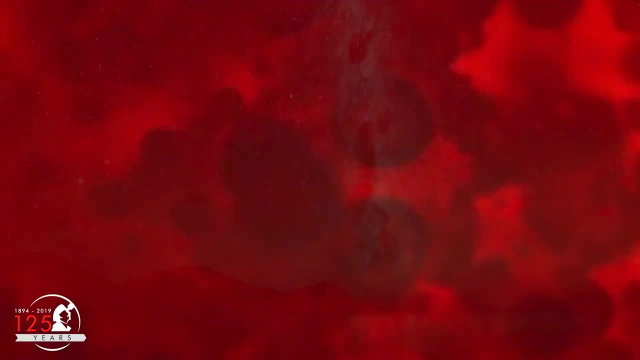 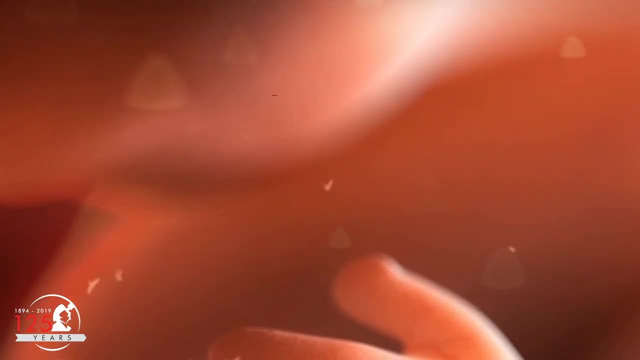 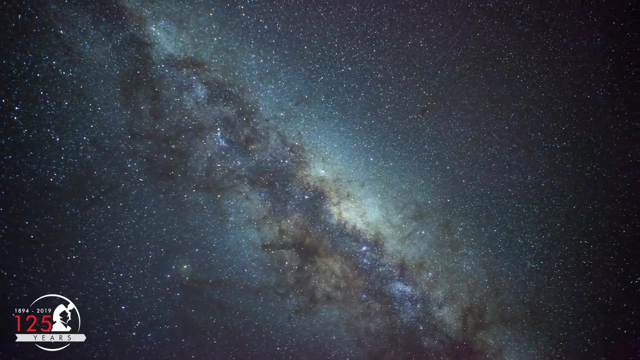 and he stations 300 gods in the sky to protect it. then he uses the blood of the most powerful monster of Tiamat's army in order to serve the gods and to help protect the natural order of the gods who live in the sky. seven are particularly important. 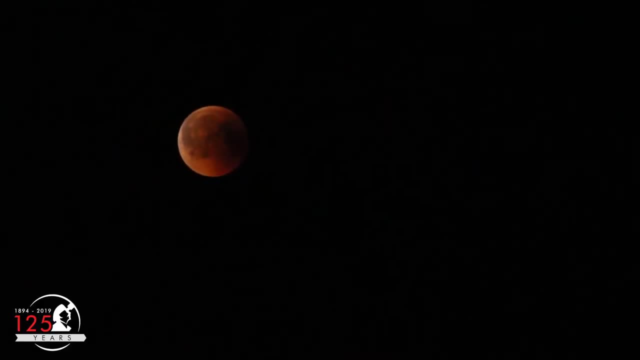 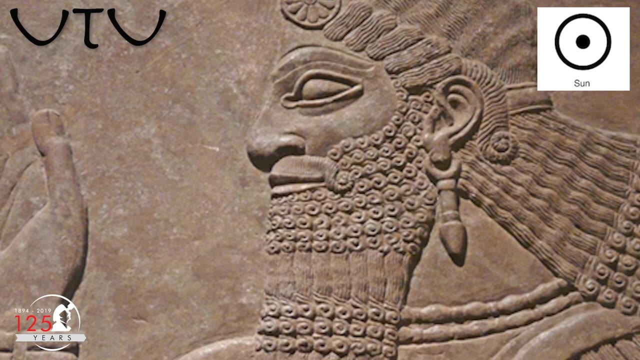 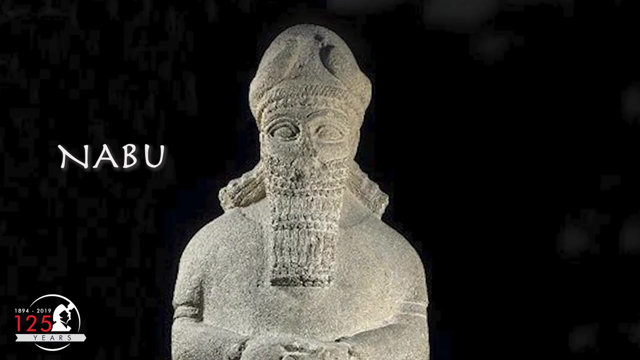 unlike everything else in the sky, these would move across the sky from night to night. Utu is the god of the sun. he is all-seeing and represents truth and justice. Nana, the lord of wisdom, is god of the moon. Nabu, the god of writing. 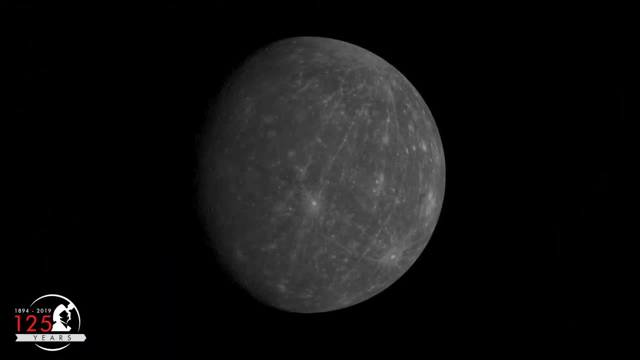 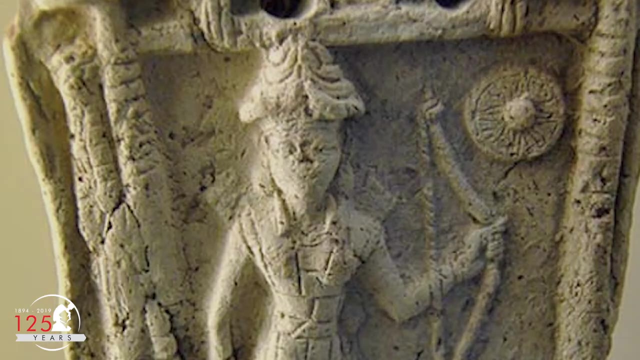 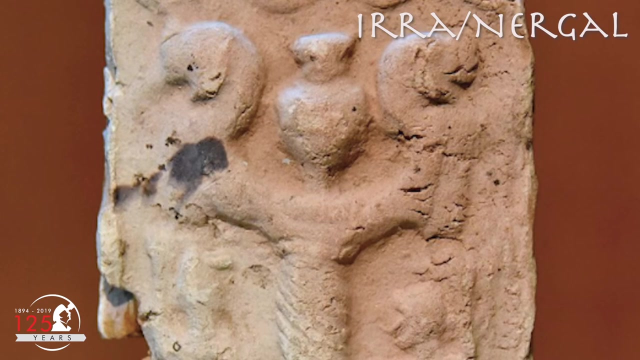 and of scribing would later come to be known as Mercury the messenger, Inanna or Ishtar, the goddess of love and war, who would come to be known as Venus the goddess of love, Ira or Nergal, the god of destruction and the conqueror of the underworld. 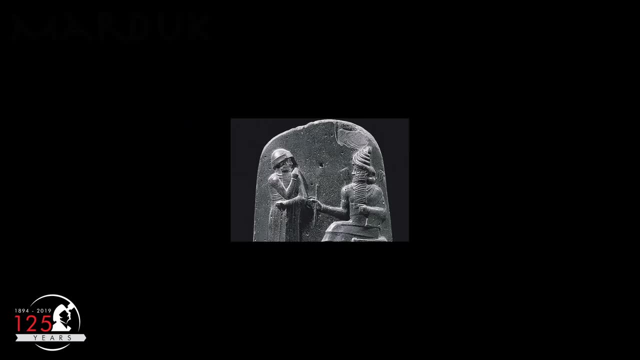 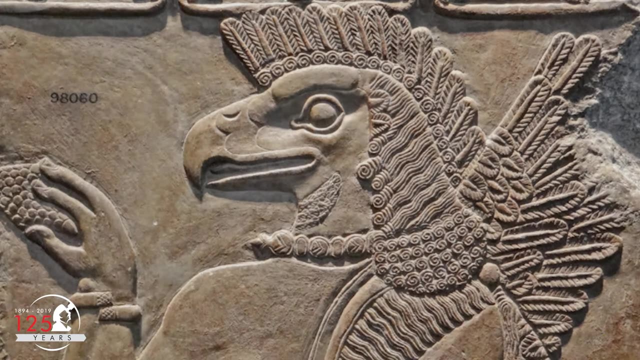 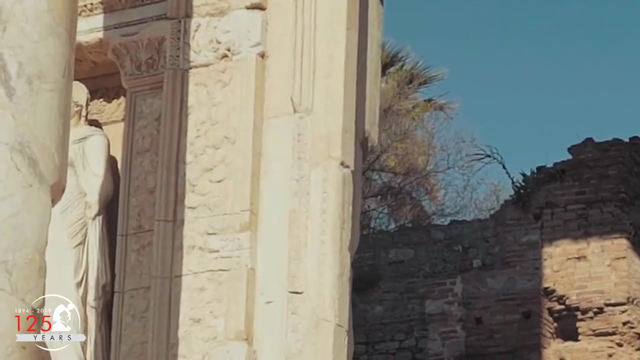 would become Mars, the god of war, Marduk, the god of storms and the king of gods, would become Jupiter, and Ninurta, a patron god of farmers and the god of agriculture and renewal. the most well-known versions of these stories of the planets and the constellations. 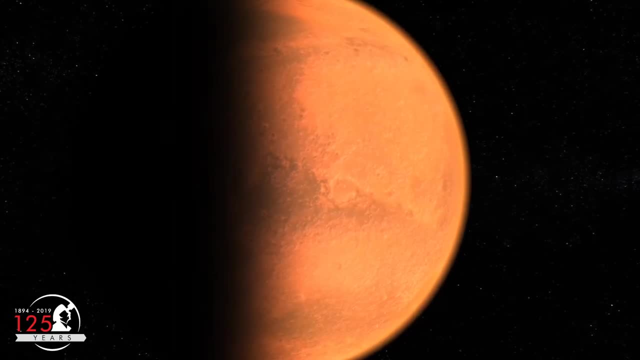 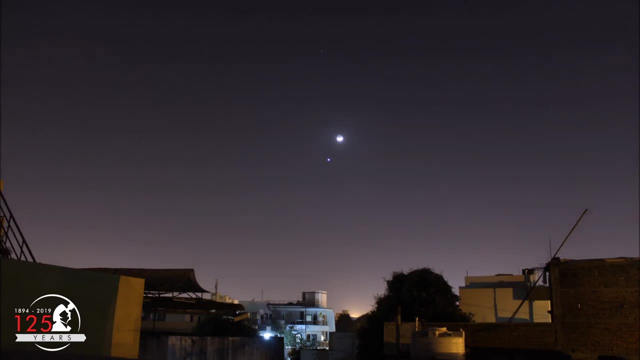 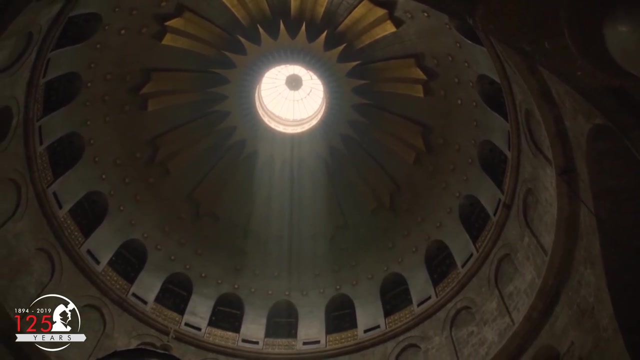 are those of the classical Greeks. it's actually from ancient Greek that we get the word planet, which literally means wanderer, for those special objects that appear to wander across the sky. the Greek gods have countless adventures and misadventures, but their story begins with the earth. 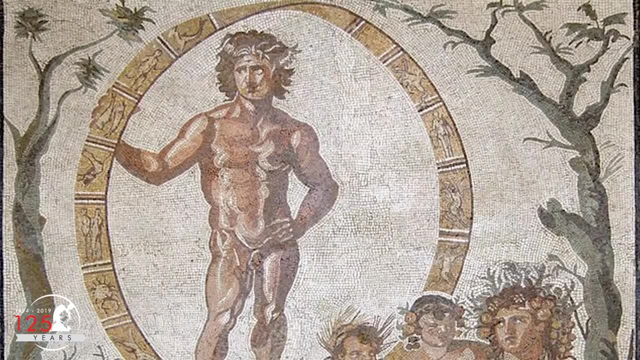 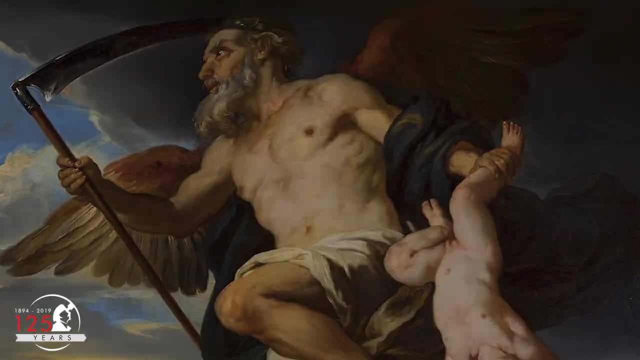 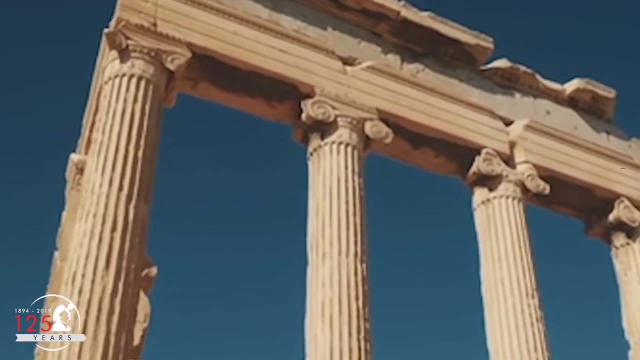 and the sky, personified by Gaia and by Uranus. this couple begets the titans, one of whom, Cronus, overthrows his father and takes dominion over the cosmos. Cronus rules wisely and for time. untold, he oversaw a golden age. 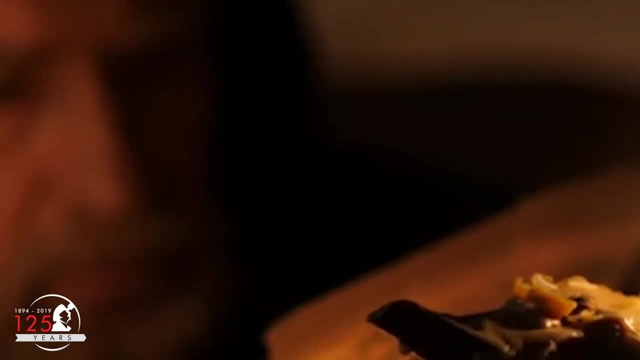 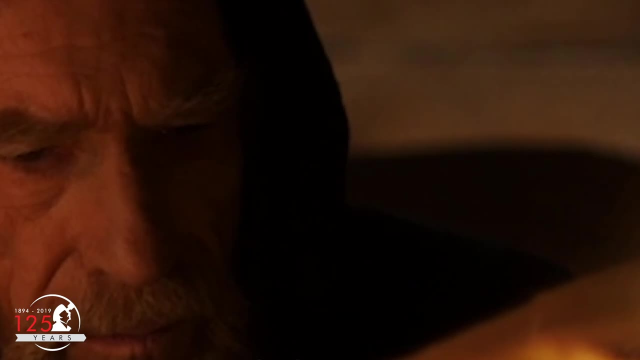 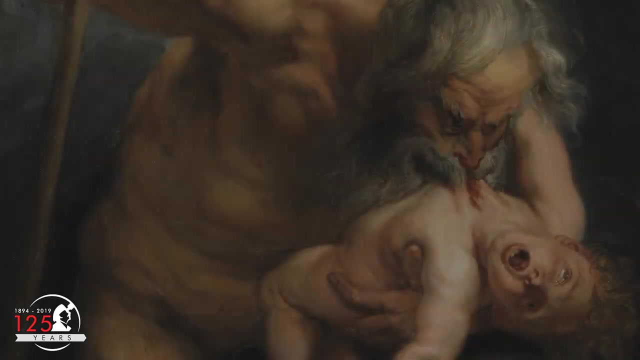 without war or famine, or even a need for laws. but eventually Cronus heard from his deposed parents that they prophesied that he would overthrow his father. eventually, Cronus would be overthrown by one of his own children. in order to prevent this, Cronus would devour each of his children. 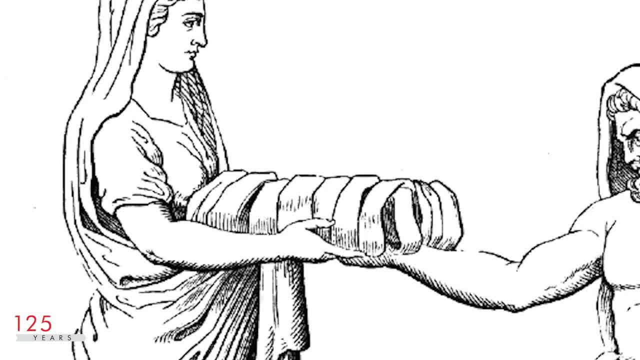 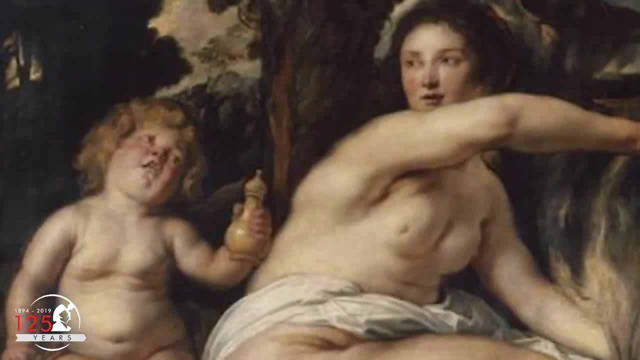 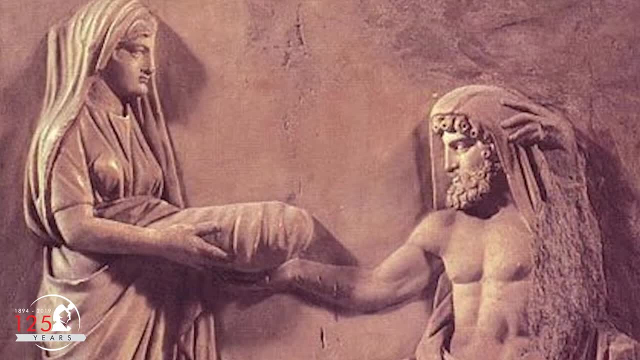 when they were brought to him, but Cronus' wife, Rhea, was not happy with this arrangement. eventually, Rhea gave birth to his son, named Zeus, but instead of presenting Zeus to Cronus, Rhea disguised a stone as the baby and handed it to Cronus instead. 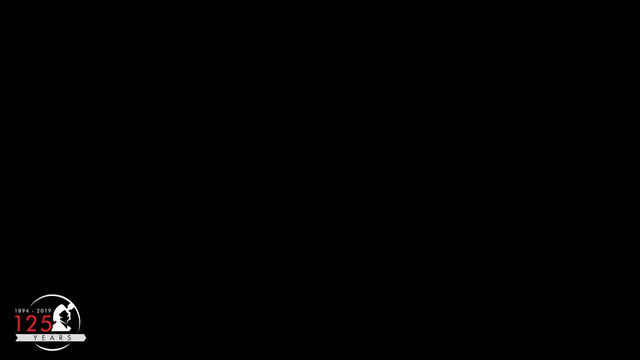 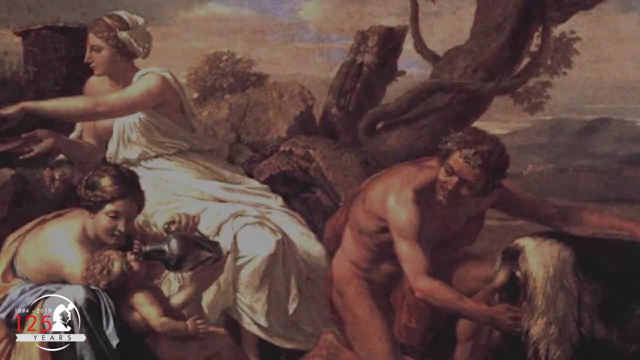 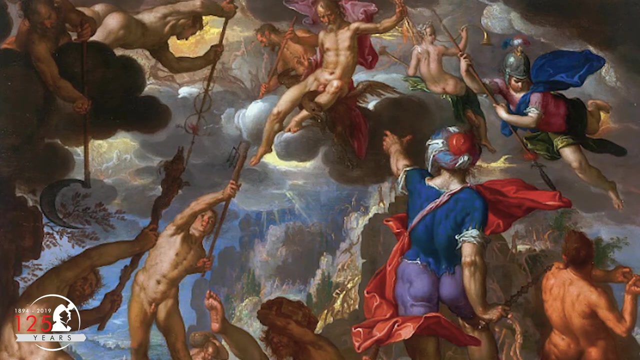 without even looking, Cronus swallowed the stone whole Rhea, then hid baby Zeus away and let Zeus be raised by a goat named Amalthea. when Zeus was of age, he freed his five siblings from his father's stomach, and the six of them waged war. against Cronus and eventually won, this cycle was to repeat itself. it was also prophesied that Zeus would be one day overthrown by one of his own children, but that's a story that has yet to be told. most of the planets as we now know them. are named for gods of Roman mythology, who are usually quite similar to their earlier Greek counterparts. Zeus is the precursor to Jupiter, as Cronus is the precursor to Saturn. Hermes and Ares are children of Zeus, and they are represented in Roman mythology and in the sky, as Mercury and as Mars. 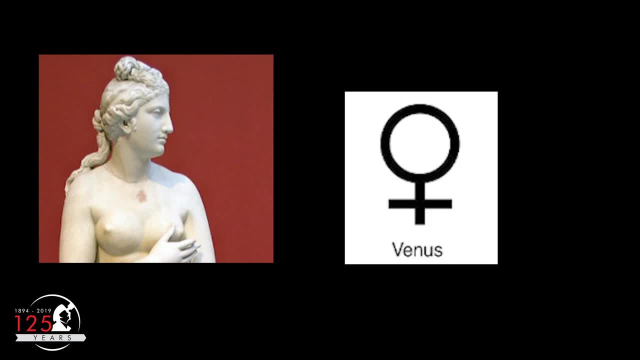 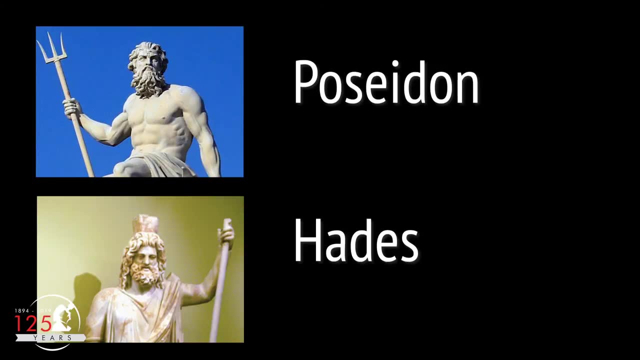 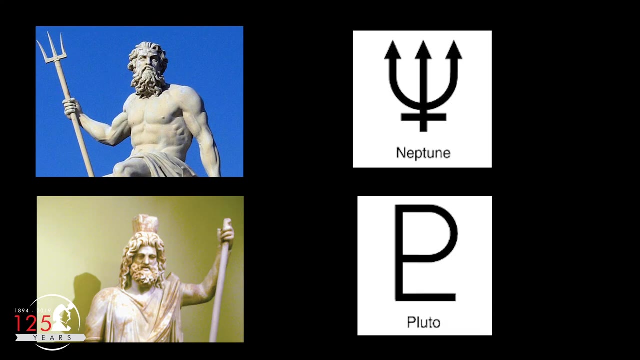 Aphrodite was Romanized into Venus and she was created, and part of Uranus fell into the sea when he battled Cronus. Poseidon and Hades are the classical Greek gods of the ocean and of the underworld and they're Zeus' brothers, and they were Romanized into Neptune and Pluto. 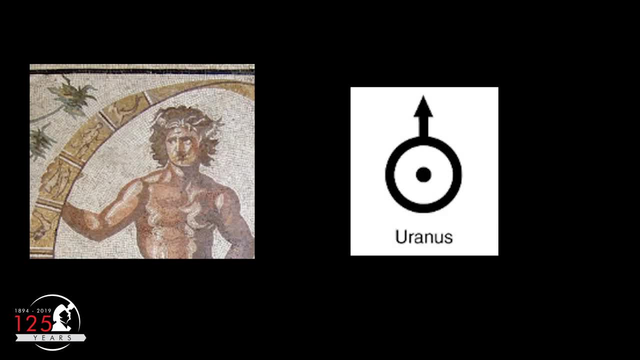 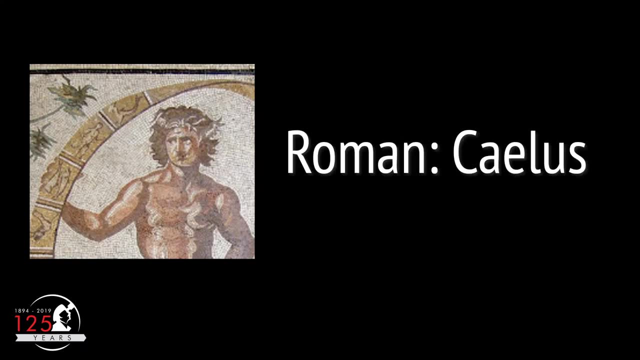 Uranus is the only one of the modern planets to be named directly after a figure of the Greek, rather than Roman, stories. the Roman analog for Uranus is Calus, and remember Amalthea, the goat who raised baby Zeus. she is in the sky too. 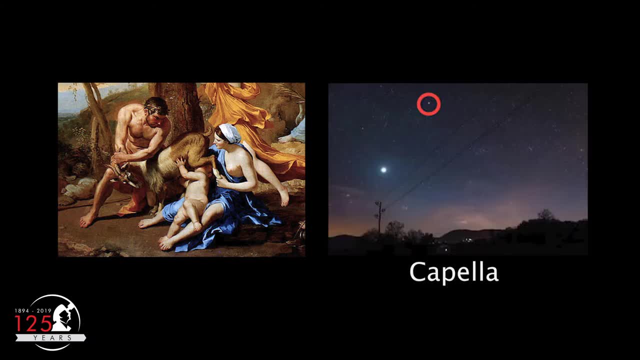 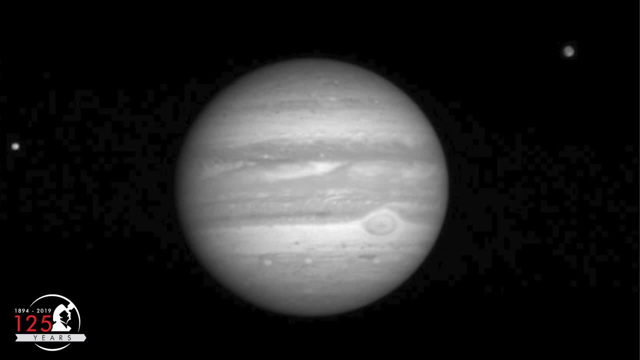 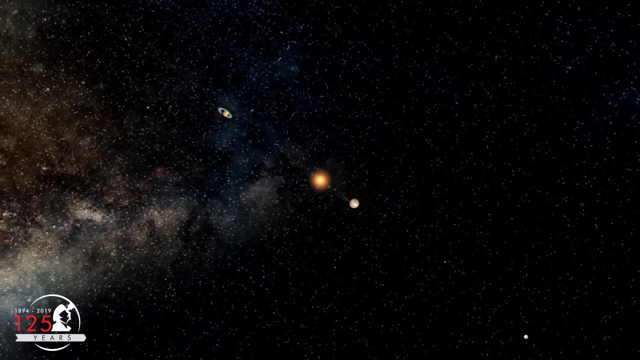 she is traditionally represented by the star Capella, the sixth brightest star in the night sky, and one of Jupiter's moons is also named for Amalthea. incidentally, the seven classical planets, the seven objects that move across the sky, are modern days of the week. 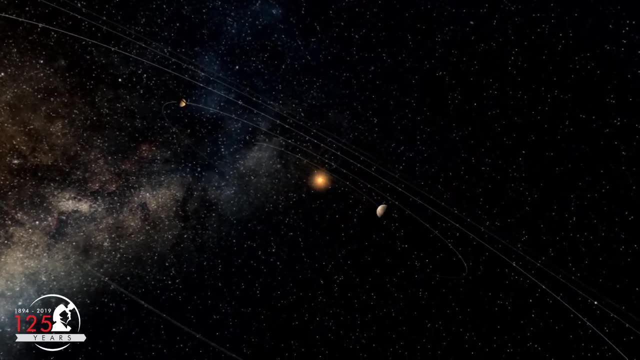 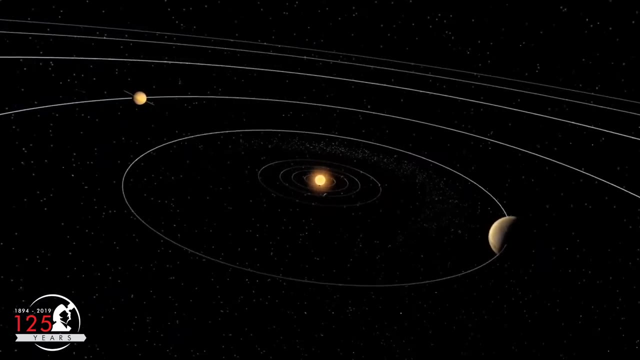 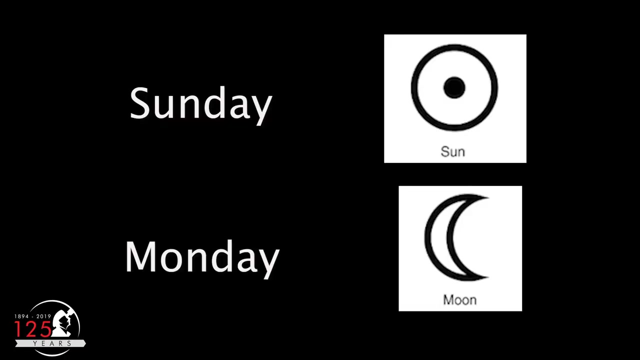 were created in their honor by the Babylonians and even through many changes in how our calendars are organized, the seven day week persisted. our current days are by way of the newer Norse stories. Sunday was named for the sun and Monday for the moon. Tuesday is named for Tyr. 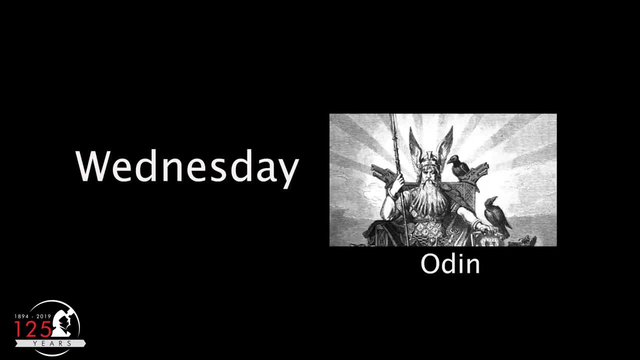 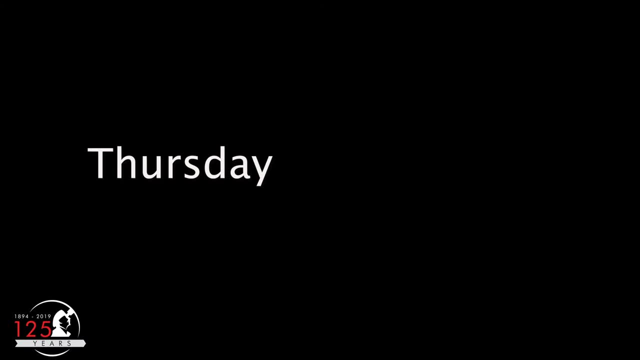 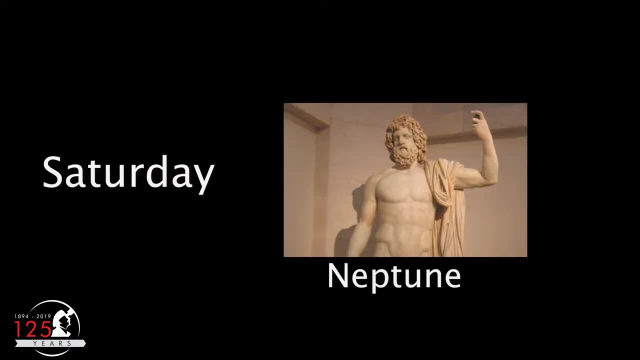 who displaced Mars. Wednesday is in honor of Odin, who replaced Mercury. Thursday is for Thor, who is, like Jupiter and Marduk, a god of storms. Friday is for Freyja, who took over for Venus, and Saturday is- you guessed it- for Neptune. no, just kidding, it's named for Saturn. 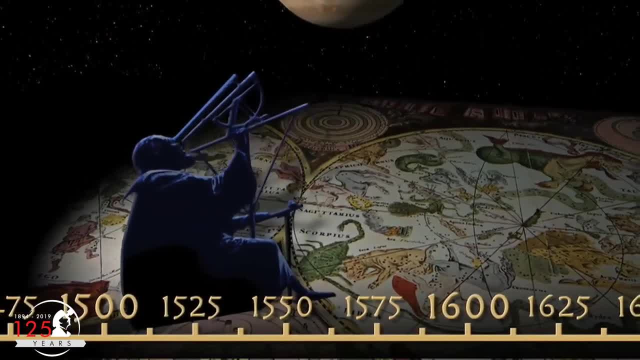 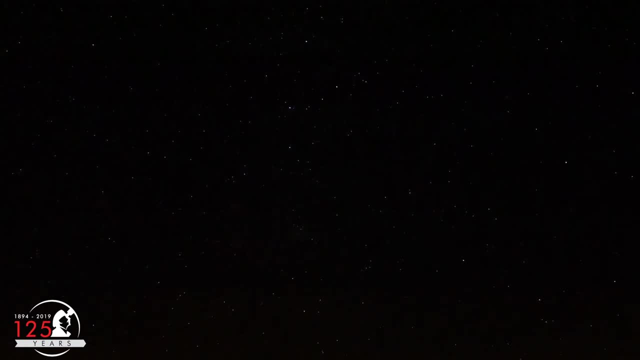 even after thousands of years, our calendars bear the marks of stargazers of ancient civilizations. next Thursday, spare a thought for a stargazer 3000 years ago, looking up and seeing Marduk, the vanquisher of Tiamat and the god of storms.